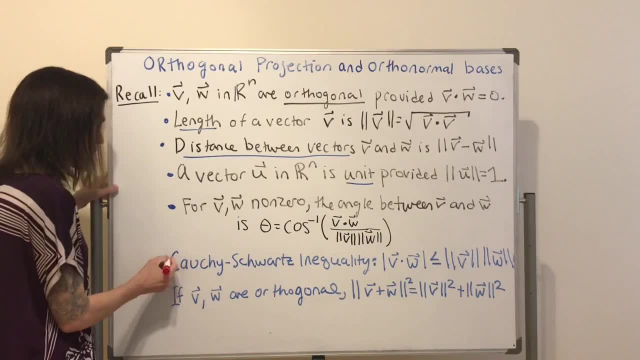 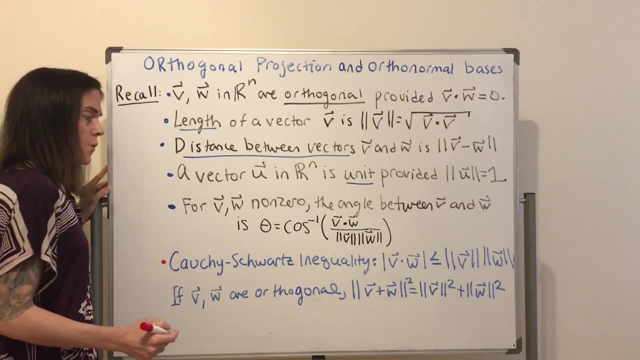 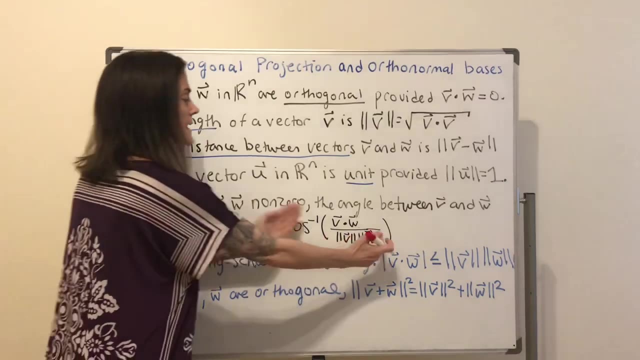 well, I may not have explicitly read it on the board, but we will use this one. I will use in our very last example today: Cauchy-Schwarz inequality. Where does this come from? Well, think about it If you think from the above right. what's in here? and I could have written: 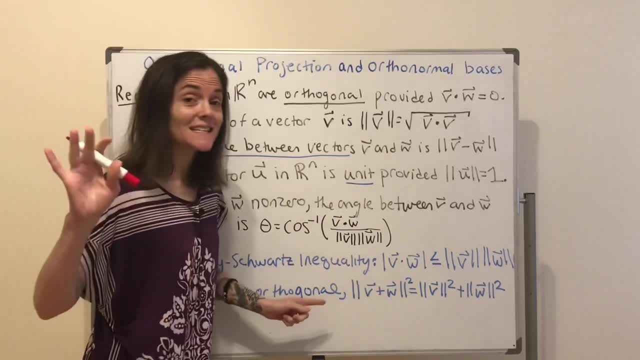 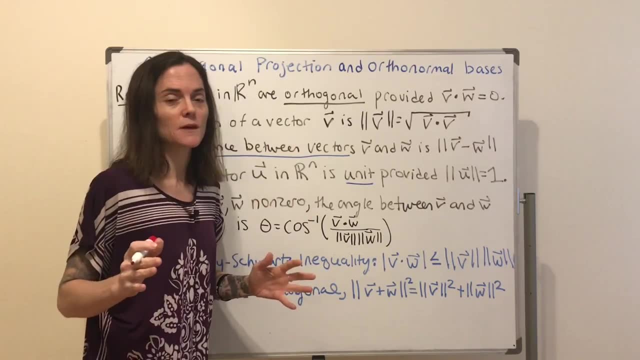 this differently, but what's inside these parentheses is a cosine of an angle. So we know, in absolute value, the cosine is b. well, it's always less than or equal to one in absolute value. And so if you have an absolute value, and you have an absolute value, and you have an. 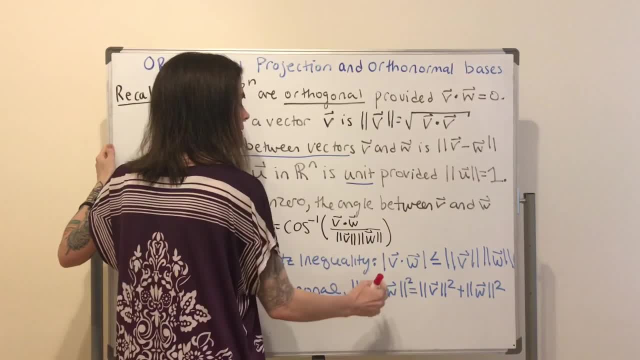 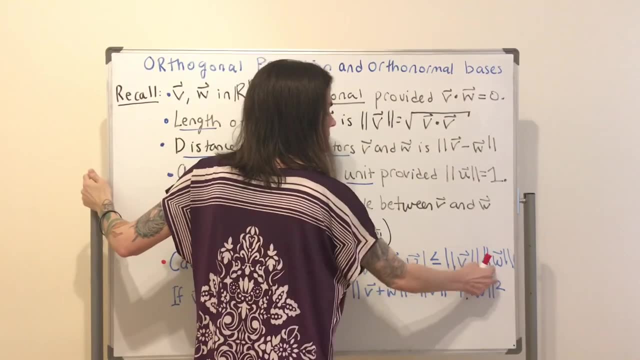 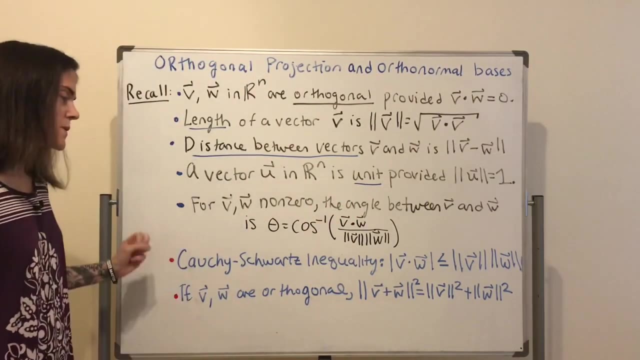 absolute value, this is less than or equal to one. then that would say that the absolute value here is less than or equal to these two products, And these two are always non-negative. anyways, they're lengths. Finally, let's talk about this last one, which we will see maybe in the next or. 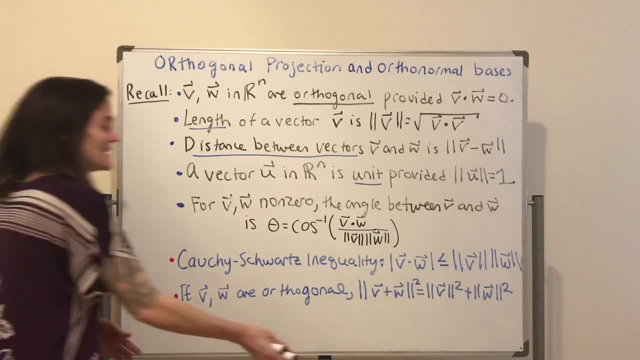 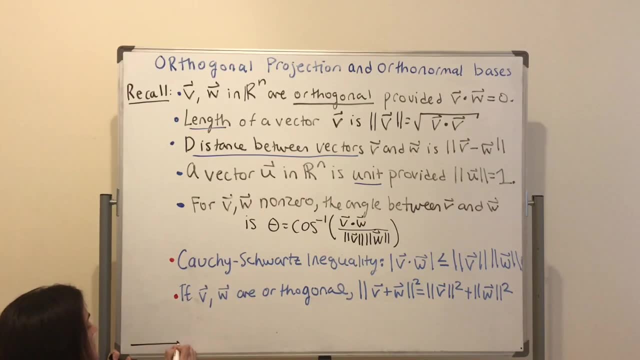 the one after that video. Well, this really just comes from a picture. Suppose this is v, and oh, excuse me, this is supposed to be v. I wrote w. Let's suppose this is v, And then, whatever w is, we know how we add triangle rule, So I put w here. 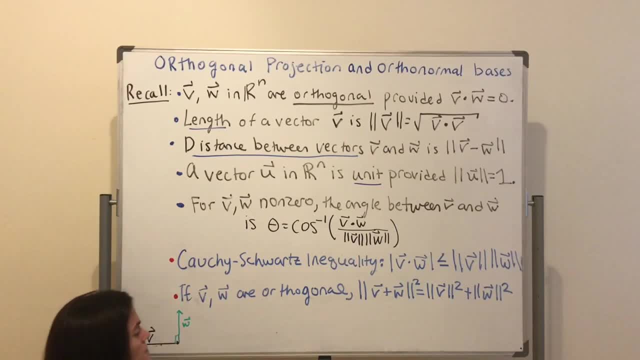 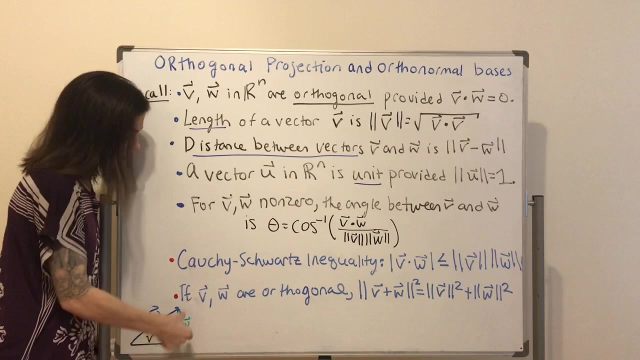 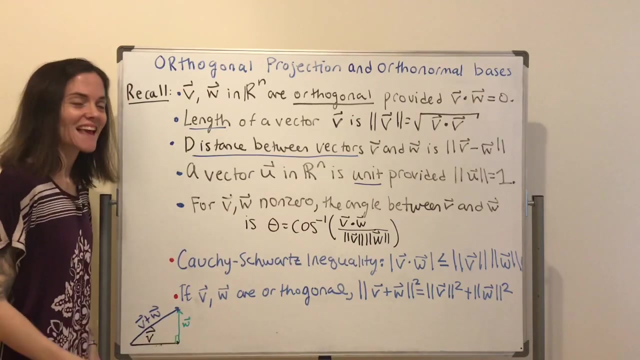 This would be 90 degrees, or pi over two, And then v plus w is here. Oh okay, This is v plus w, And you see, the Pythagorean theorem says that this side squared plus this side squared equals this side squared, And that's exactly what this equation is saying. 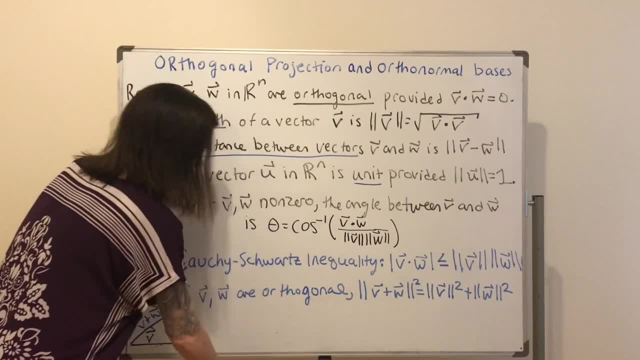 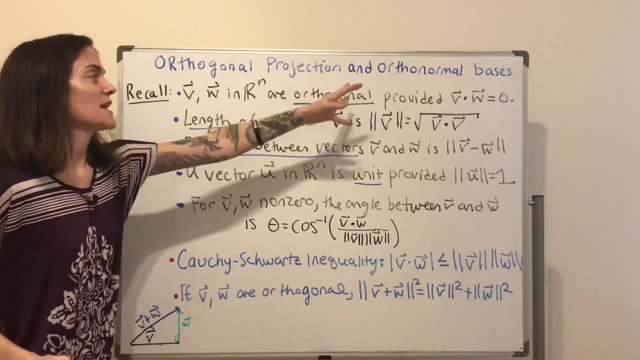 Okay. So now let's do an example. Let's do an example of using some of this before we get into orthogonal projection and orthogonal projection. So let's do an example of using some of this before we get into orthogonal projection and orthogonal projection. 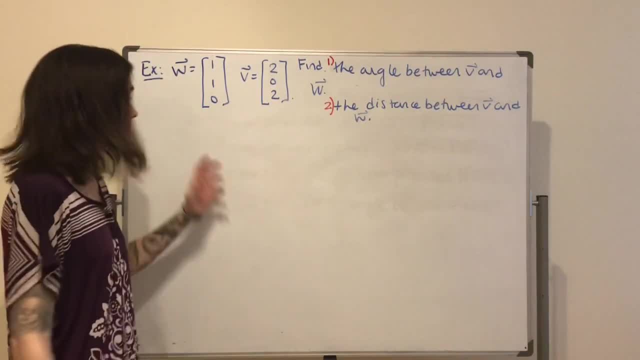 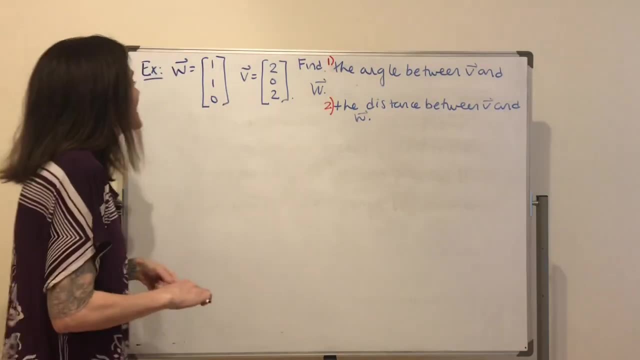 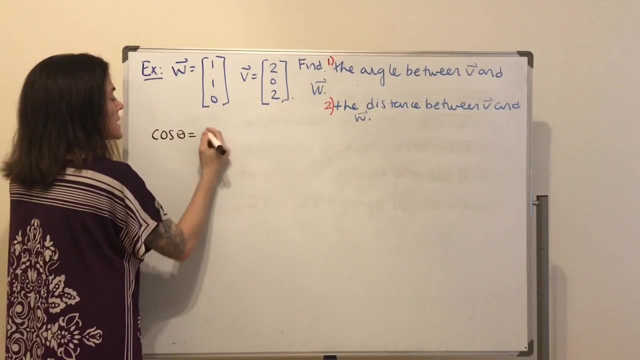 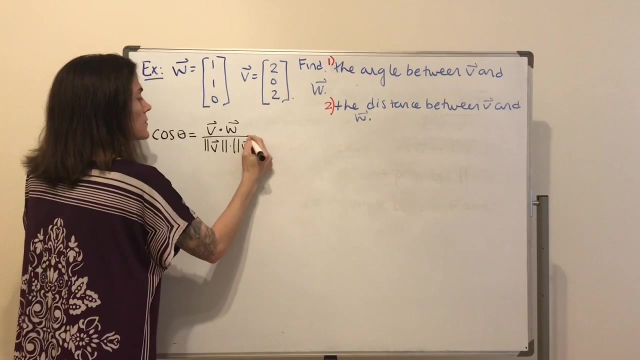 Here are two vectors in our three. We want to find the angle between v and w and find the distance between v and w. Well, let's remind ourselves that we know the cosine of theta is v dot w over the length of v times length of w. And then we know the distance between. 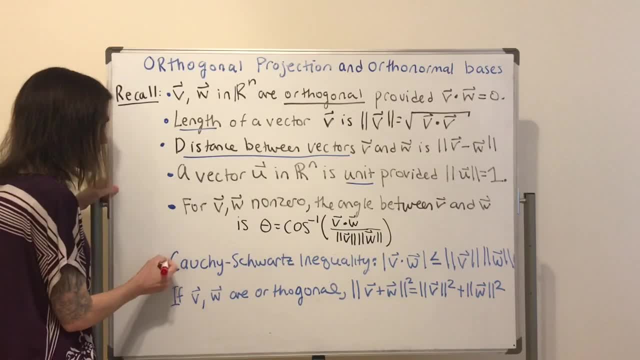 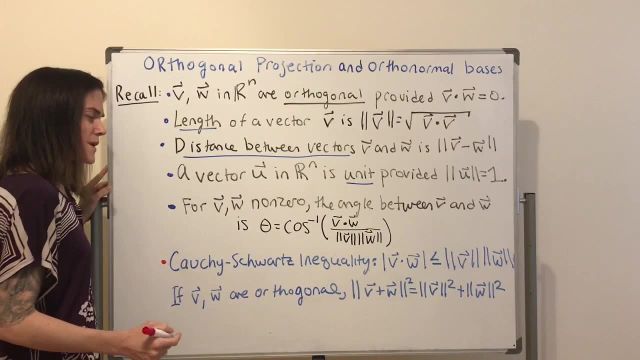 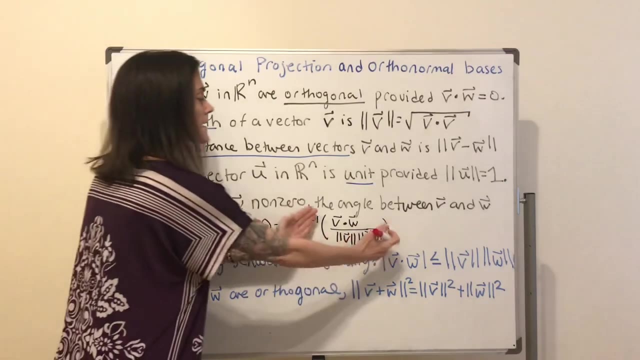 well, I may not have explicitly read it on the board, but we will use this one. I will use in our very last example today: Cauchy-Schwarz inequality. Where does this come from? Well, think about it If you think from the above right. what's in here? and I could have written: 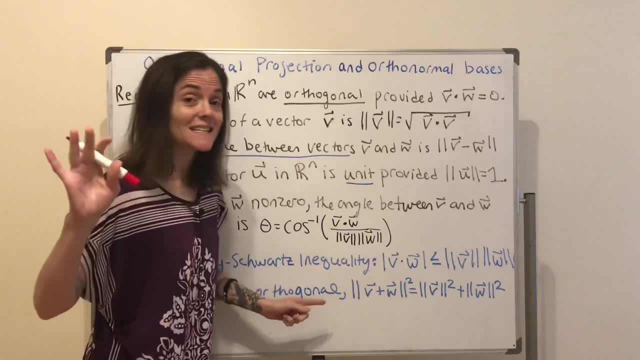 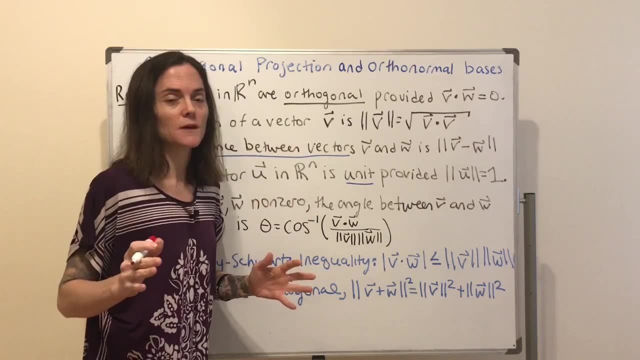 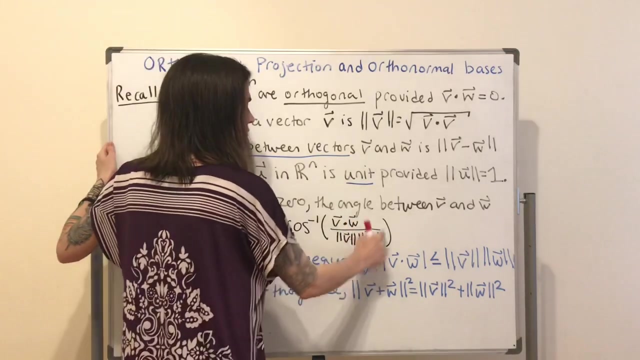 this differently, but what's inside these parentheses is a cosine of an angle. So we know, in absolute value, the cosine is b. well, it's always less than or equal to one in absolute value, And so if you have an absolute value, 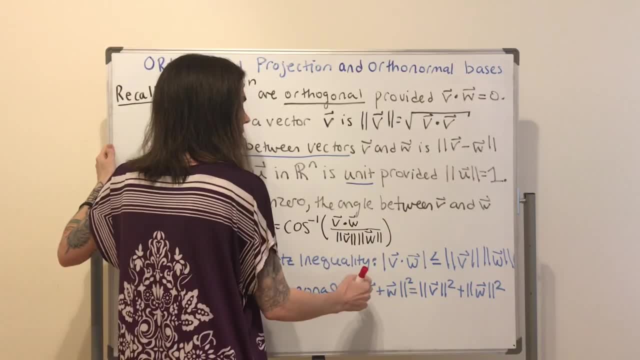 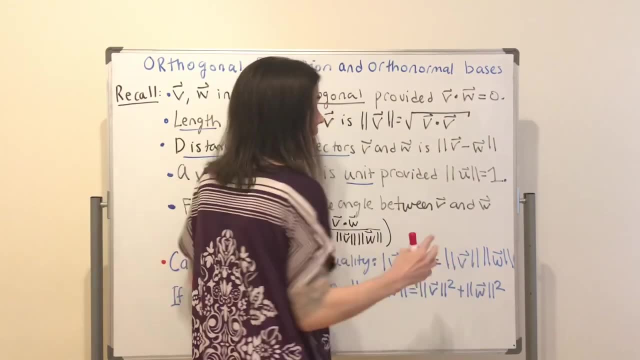 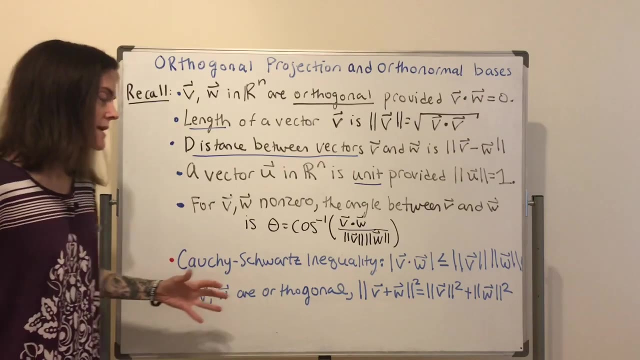 this is less than or equal to one, then that would say that the absolute value here is less than or equal to these two products, And these two are always non-negative. anyways, they're lengths. Finally, let's talk about this last one, which we will see maybe in the next or the one after that. 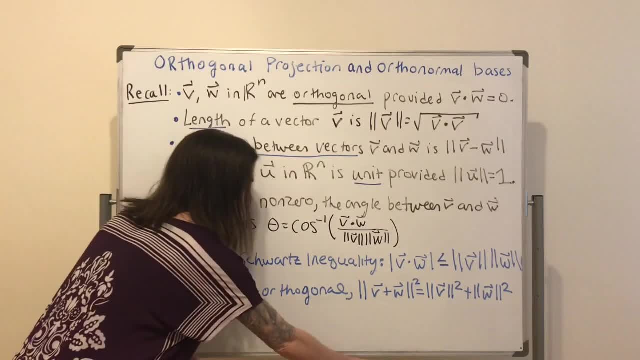 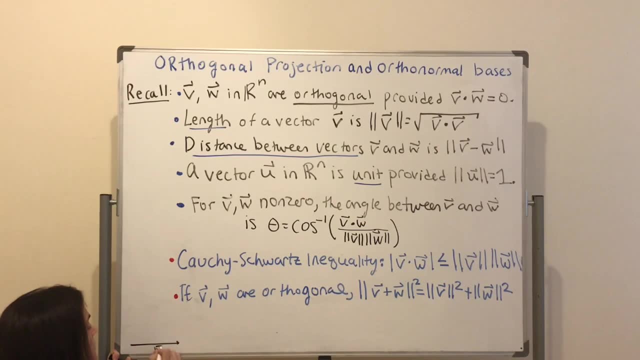 video. Well, this really is the most important part of our program, which is the length of the product. just comes from a picture. suppose this is v and um. oh, excuse me, this is supposed to be v. i wrote w. let's suppose this is v, and then, whatever w is, we know how we add triangle rule. 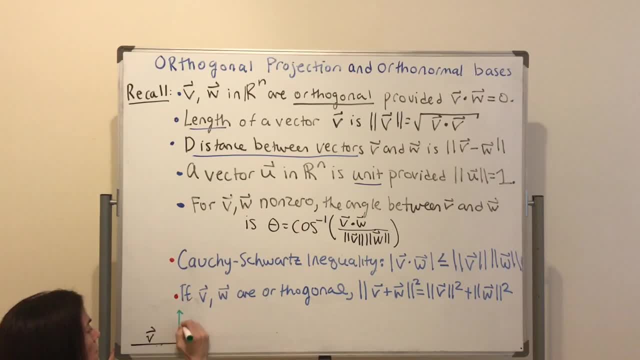 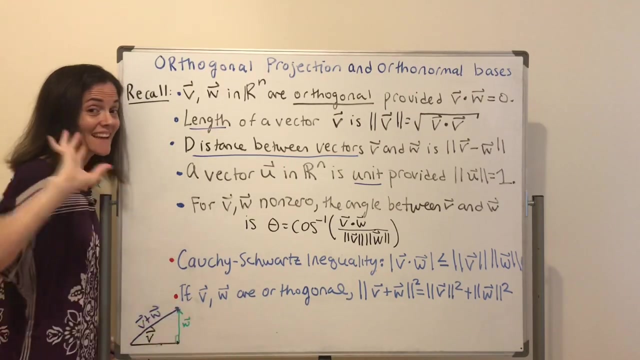 so i put w here, this would be 90 degrees, or pi over 2, and then v plus w is here. oh okay, this is v plus w, and you see, the pythagorean theorem says that this side squared plus this side squared equals this side squared, and that's exactly what this equation is saying. 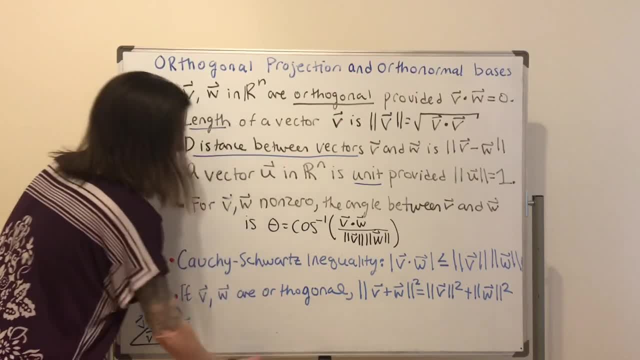 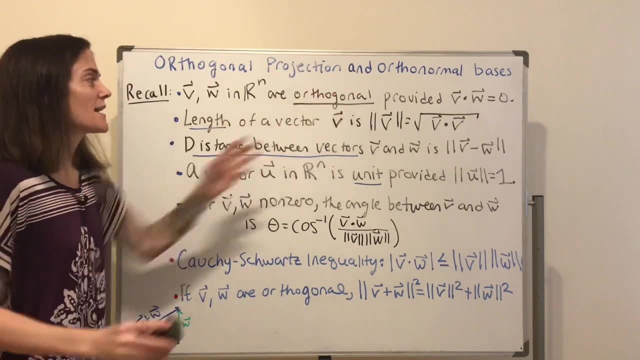 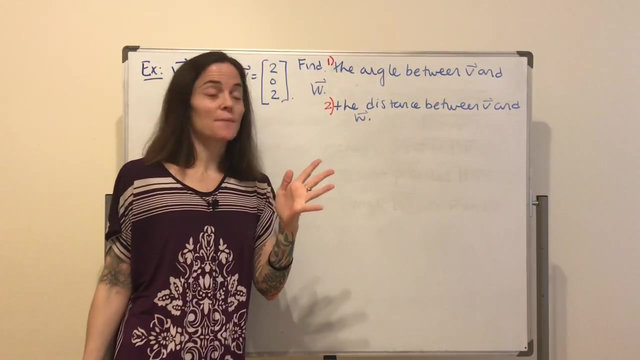 okay, so now let's do an example. let's do an example of using some of this before we get into orthogonal projection and orthonormal bases. here are two vectors. in our three we want to find the angle between v and w and find the distance between v and w. 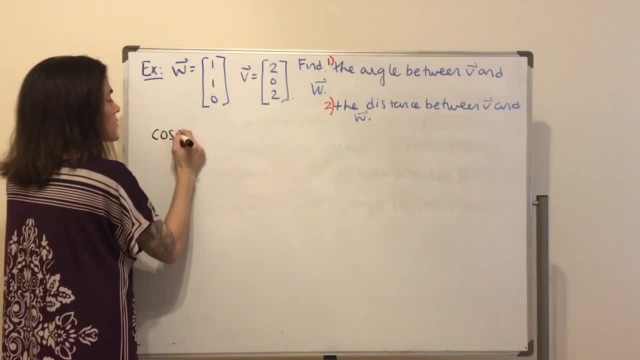 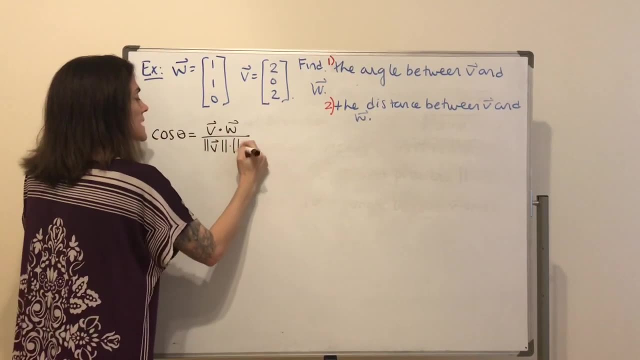 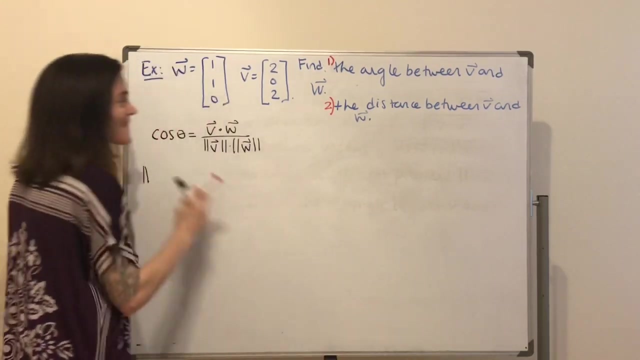 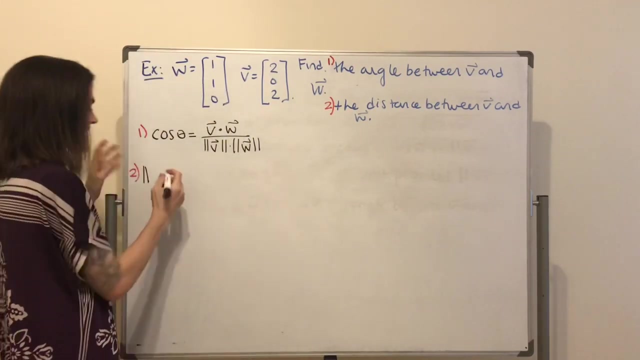 well, let's remind ourselves the we know the cosine of theta is v dot w over the length of v times length of w, and then we know the distance between. so this first part is what we use for number one and for number two, as we just reminded ourselves the distance. 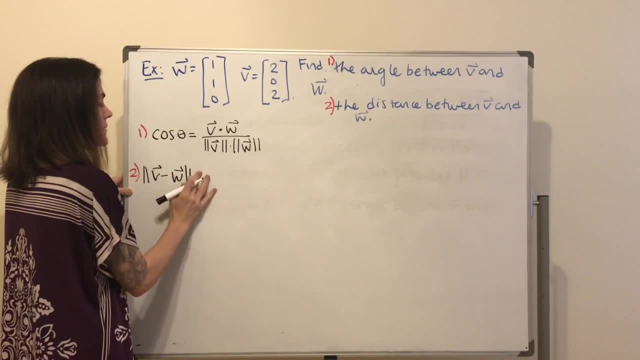 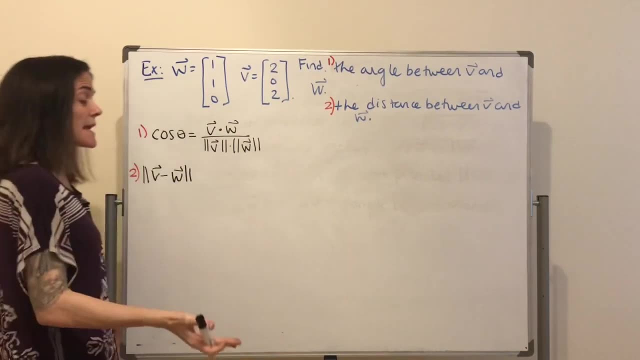 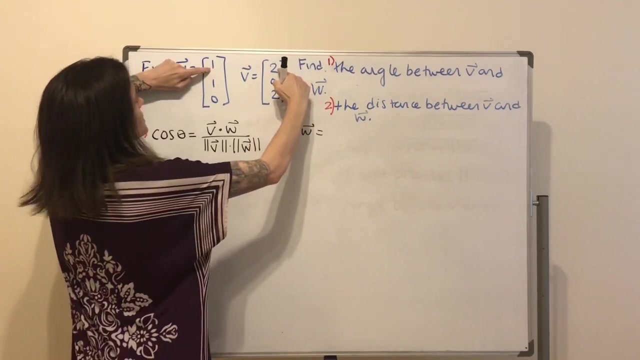 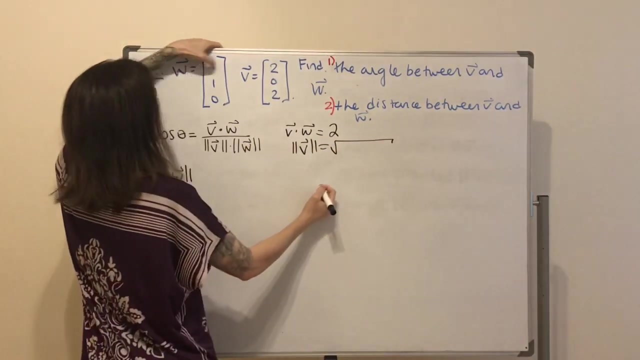 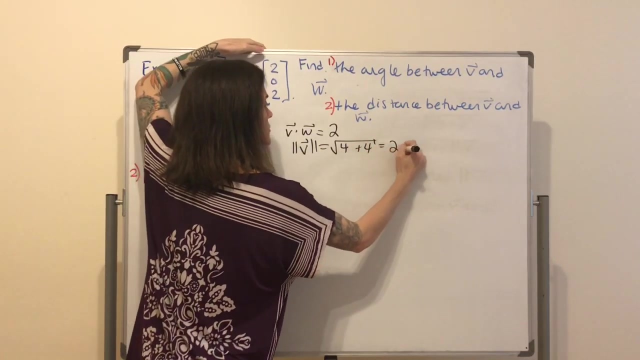 between the two vectors. is this okay? well, let's begin on number one. all the i need. i'll calculate it so we can get rid of all those quantities. and then think about the inverse cosine. v dot w is 2 plus 0 plus 0.. the length of v is the square root of here, 4 plus 5. this is the square root of. 2 square root of 2. the length of w is square root of 1 plus 1 and the group's missing, so probably it doesn't matter. the point is that this is the Lagrangian purpose. so again, if you try to sleeve theraph sodid, you're going to get this unit here. just if you make sure a square root is a square root. of 2. there's no answer you so just make sure that that is the temperature that you're got of these limits. so if we need to separate the product charge several times, then inside the vocês, then this is what we're going to do. okay, so we divide the wystras. 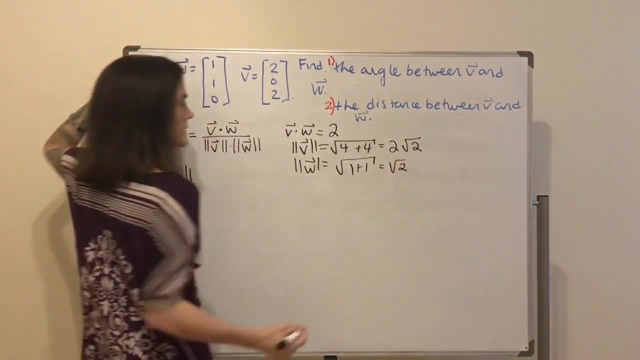 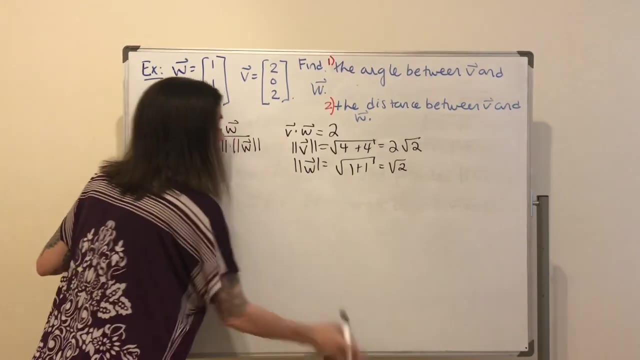 okay, that's m square root and we'll take this variable into buying strength. then we'll go to the plus one square root of two. okay, So we- maybe I need to actually erase this, I will come back to it- finish this problem. 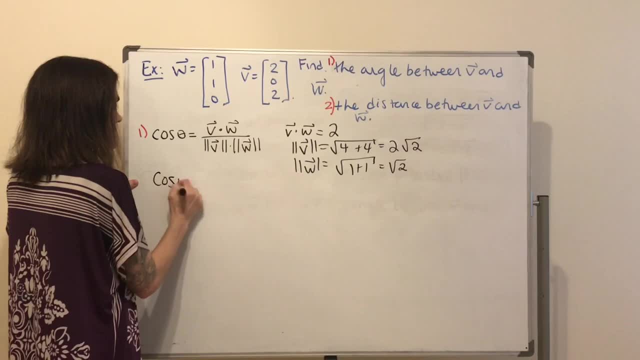 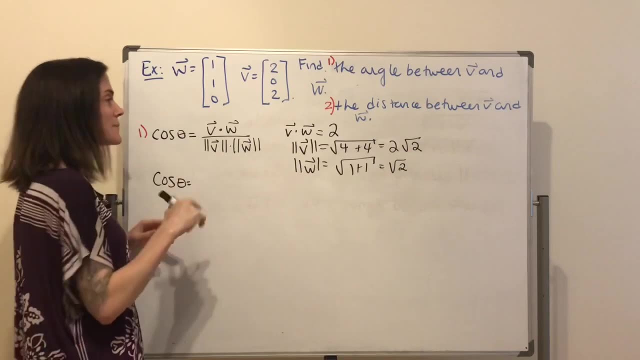 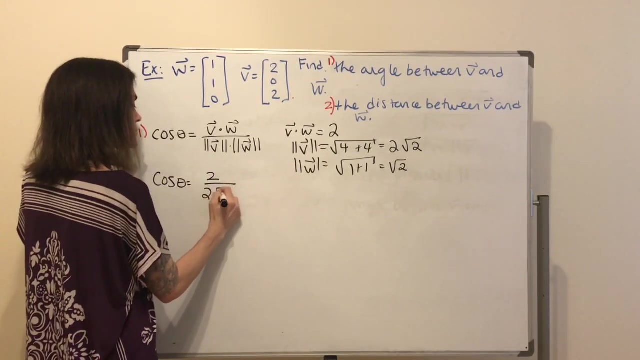 part one and then move to part two. So I know the cosine of theta, where theta is the angle between v and w and always measured between zero and pi, is two over two, square root of two, square root of two times square root of two. 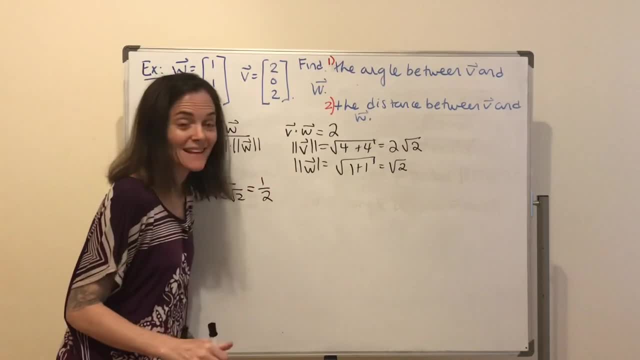 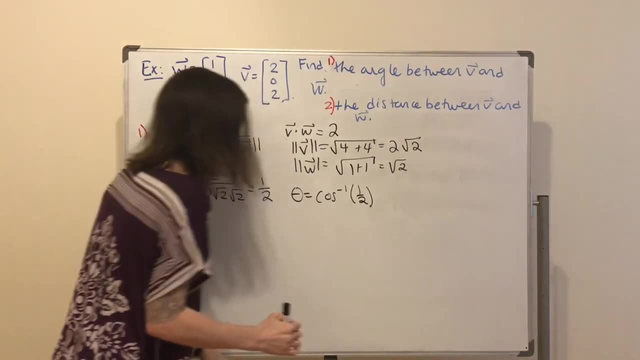 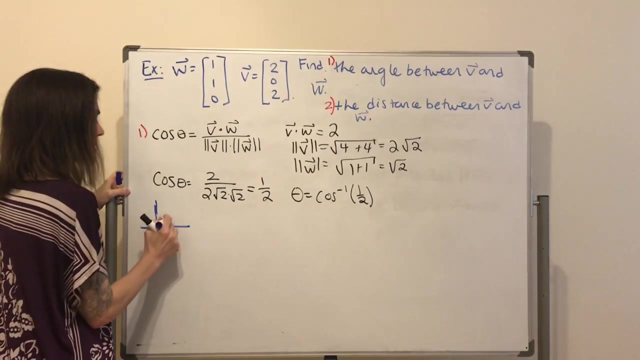 which is one half. Well, now you just have to think a little bit about trigonometry. This is the cosine inverse of a half, and here, if you think first quadrant, I always remember you have these two here: one's pi over six, one's pi over three. 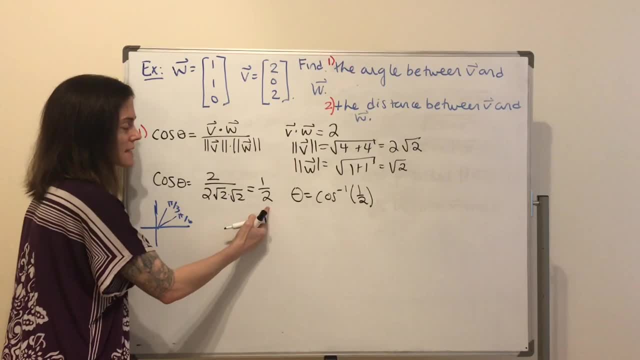 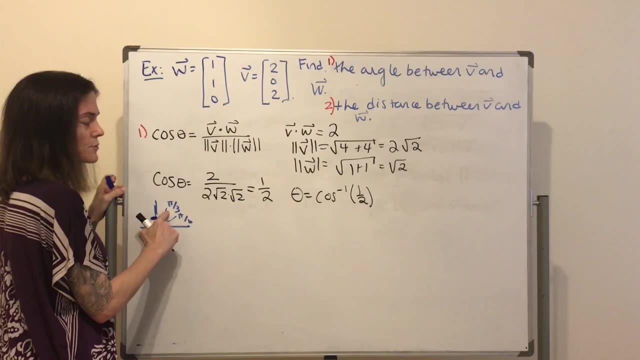 One of them has this as the cosine, one of them has this as the cosine, and one of them has this as the cosine. One of them has this as the sine and pi over six. the cosine is bigger, so that means this angle is pi over three. 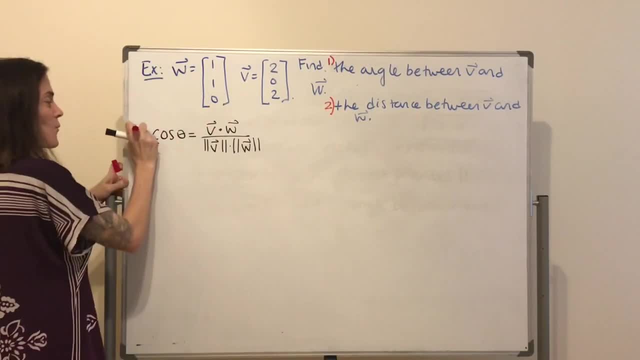 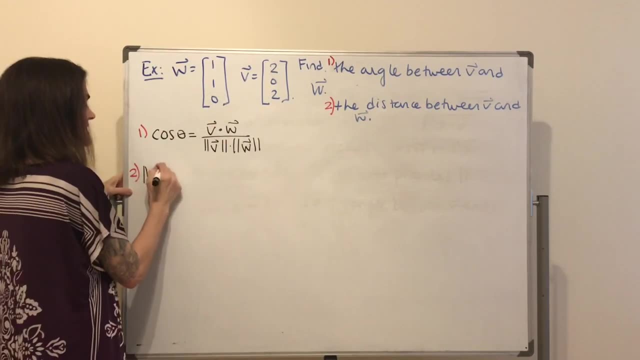 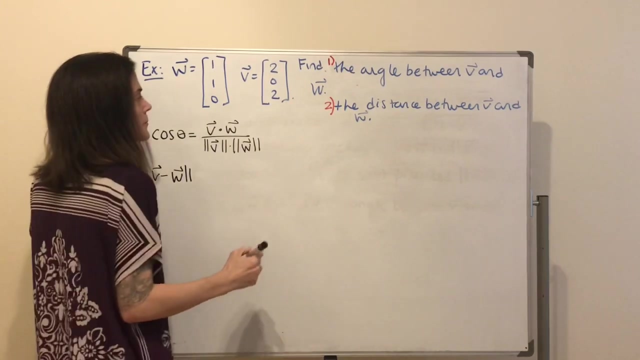 so this first part is: well, we use for number one And for number two, as we just reminded ourselves, the distance between the two vectors is this, Okay? Well, let's begin on number one. All the I need to calculate all these quantities and then think about the inverse cosine. 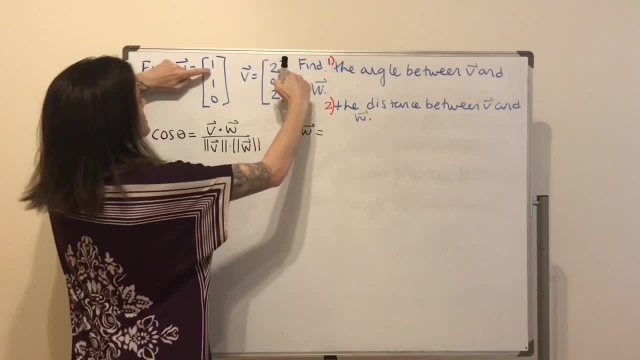 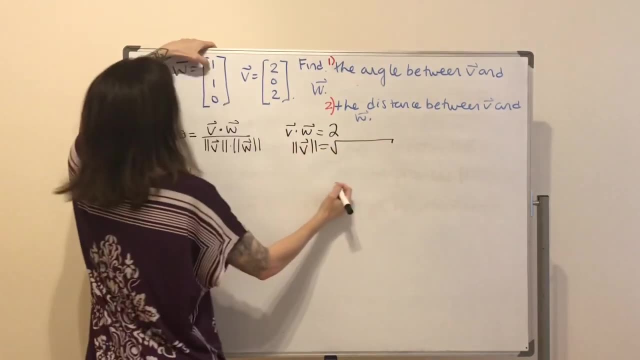 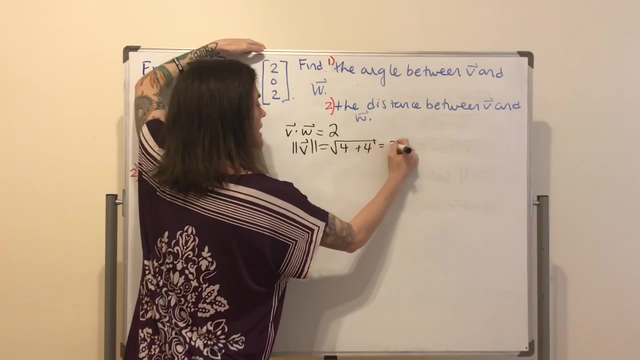 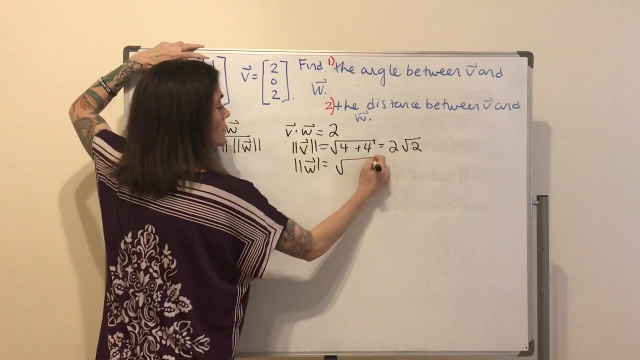 v dot. w is two plus zero plus zero. The length of v is the square root of here Four plus four. This is the square root of eight or two square root of two. The length of w is here square root of one plus one square root of two. 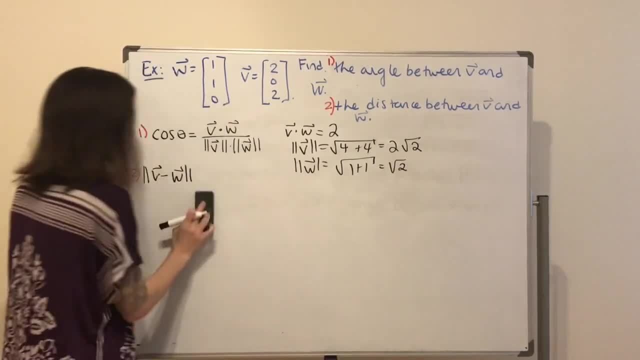 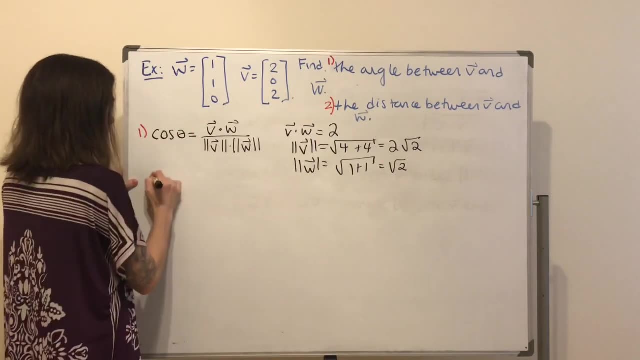 Okay, So we maybe I need to actually erase this. I will come back to it. We'll finish this problem, Part one, And then move to part two. So I know the cosine of theta, where theta is the angle between v and w. 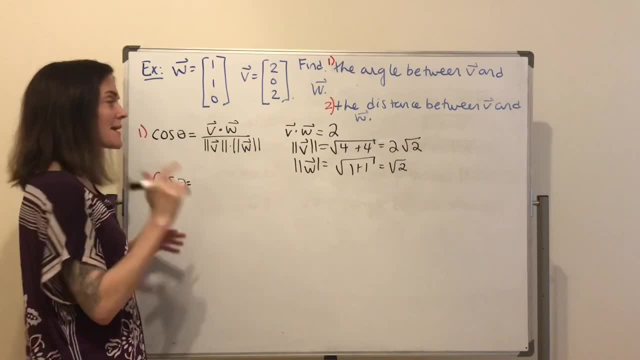 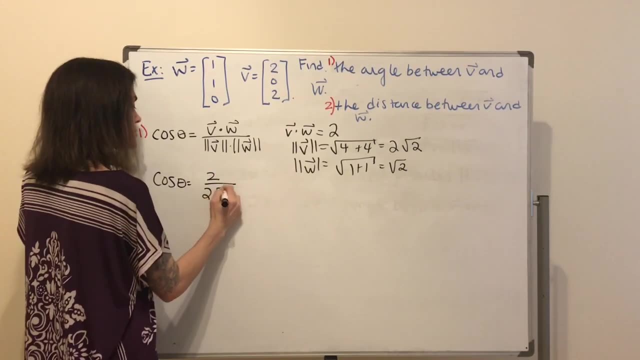 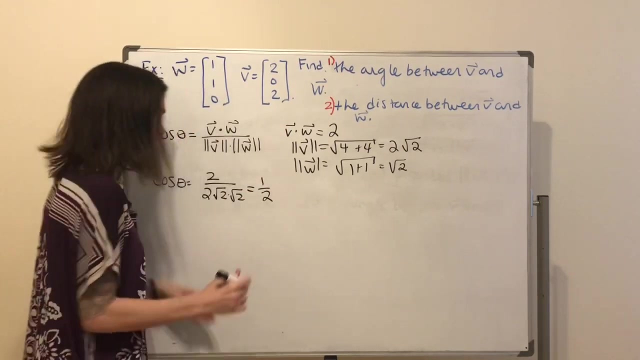 and always measured between zero and pi, is two over two, square root of two times square root of two, which is one half. Well, now you just have to think a little bit about trigonometry. This is the cosine inverse of a half. 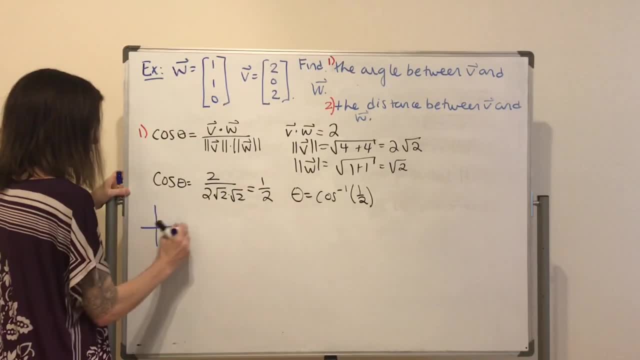 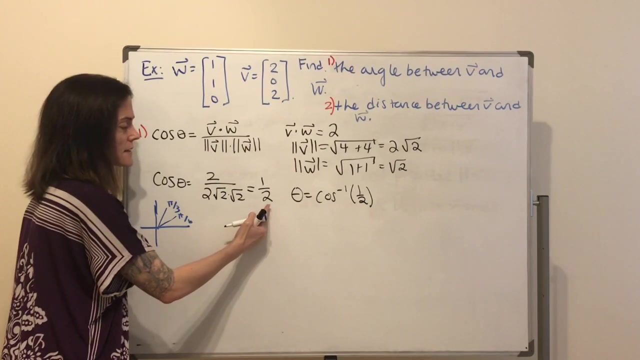 And then you just have to think a little bit about trigonometry. And then you just have to think a little bit about trigonometry, And here, if you think first quadrant, I always remember you have these two here, One's pi over six, One's pi over three. One of them has this as the cosine, One of them has this as the sine. 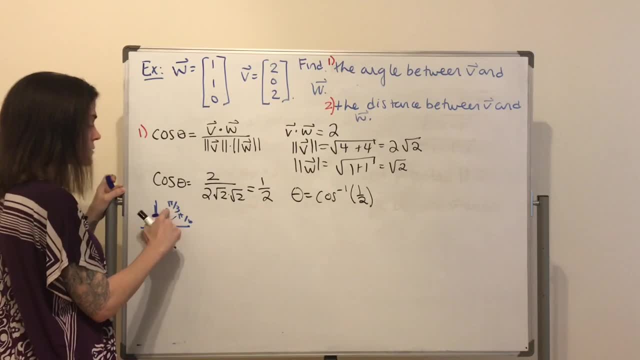 And pi over six. the cosine is bigger, So that means this angle is pi over three, because I know the one that goes with this is square root three over two, So this angle is not pi over six. The cosine is a half at pi over three, So the angle between these two vectors is pi over three. 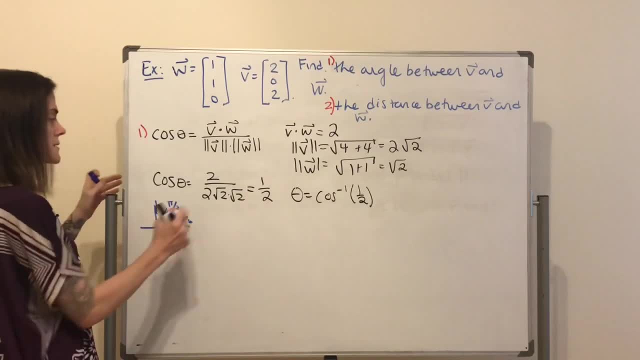 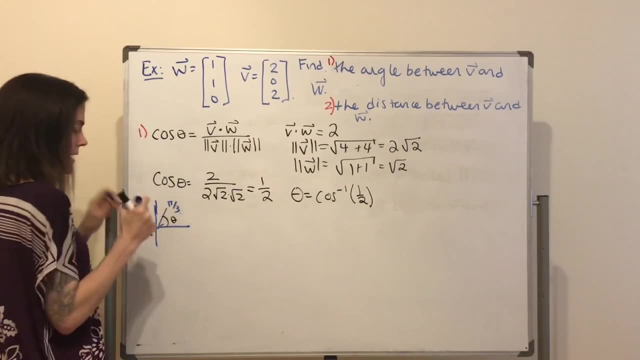 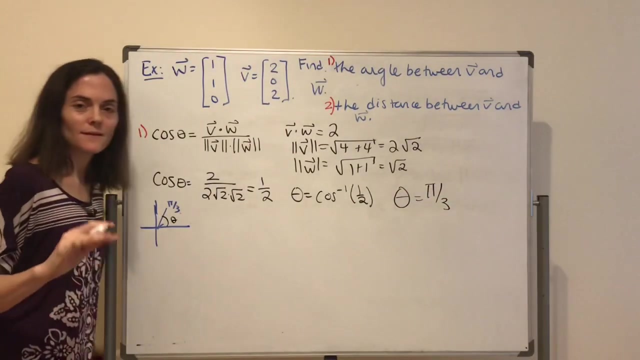 because I know the one that goes with. this is square root of three over two, So this angle is not pi over six. the cosine is a half at pi over three, So the angle between these two vectors is pi over three and this is the number one, okay. 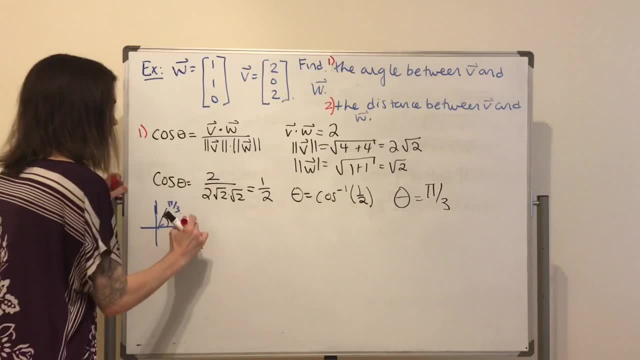 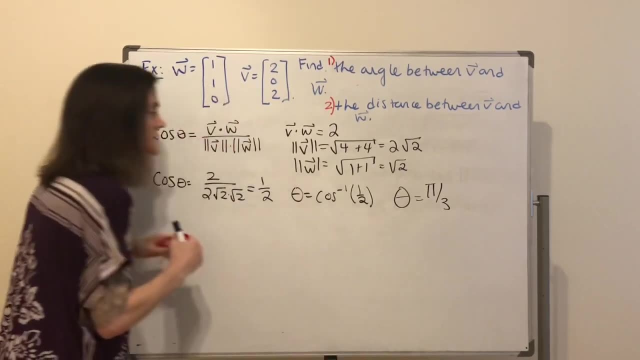 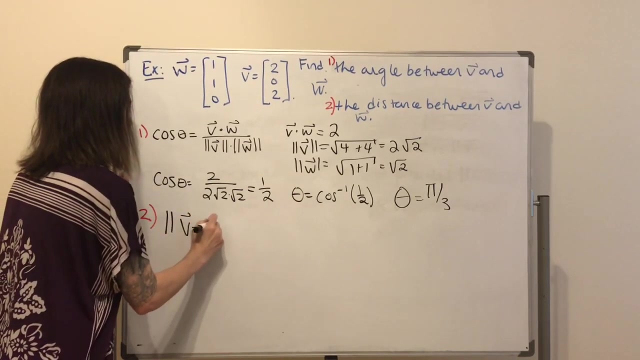 Now let's move on to number two. maybe I'll erase my picture that was helping me think about how to figure out theta. I need this v minus w, and this will just be well. first let's compute v minus w. 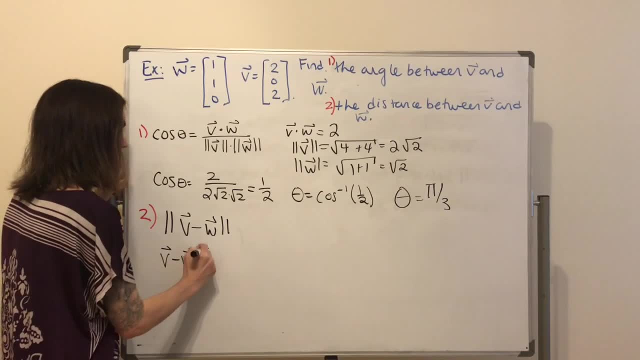 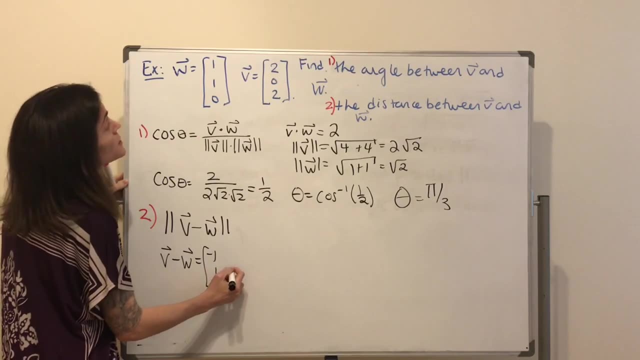 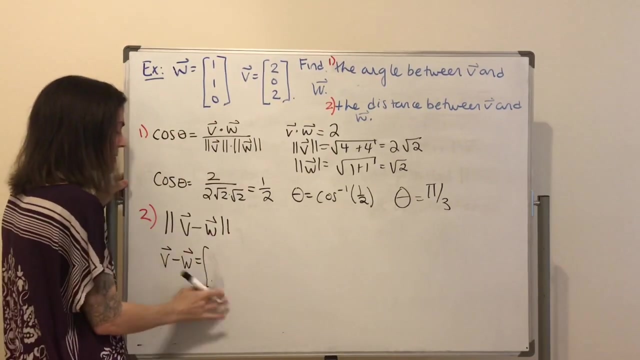 and then I will compute the length. This gives us the distance between the two vectors. This is minus one, one minus two. Oh, I did w minus v. Well, I was looking here, v minus w, pardon me. Reality is I would get the same length. 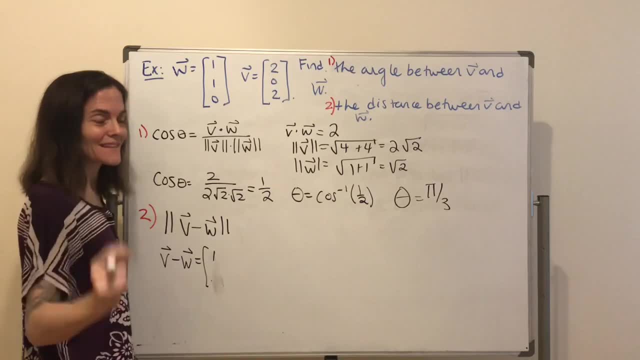 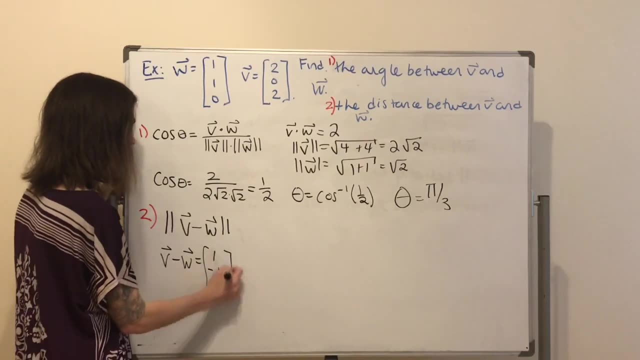 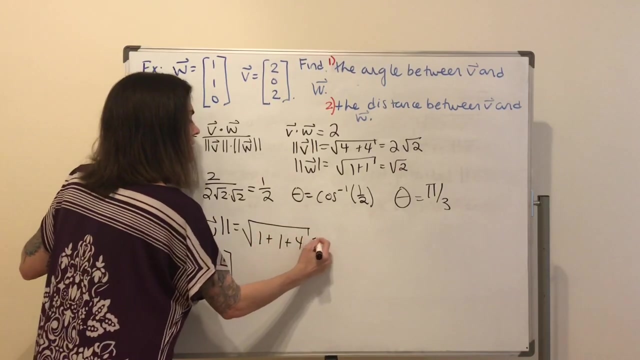 but since I wrote v minus w, let's actually do v minus w. One minus one minus two. Okay, and then this is the square root. It's one plus one plus four. It's the square root of six. 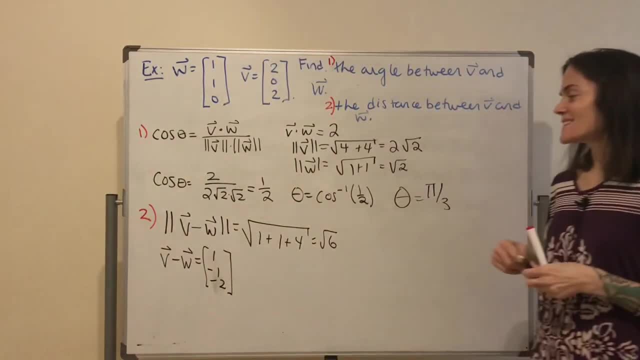 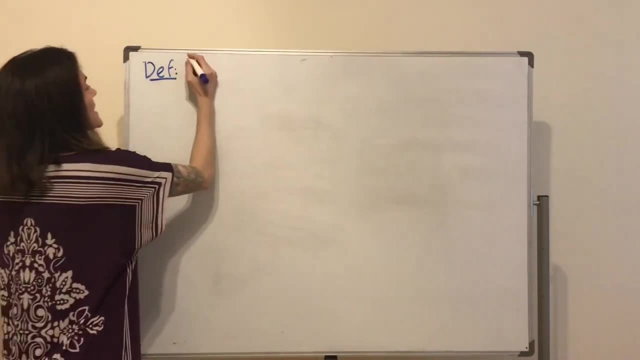 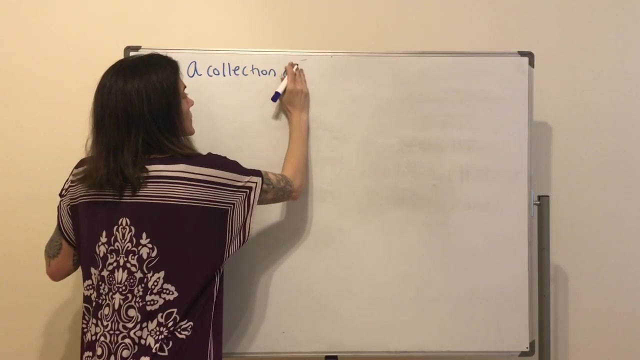 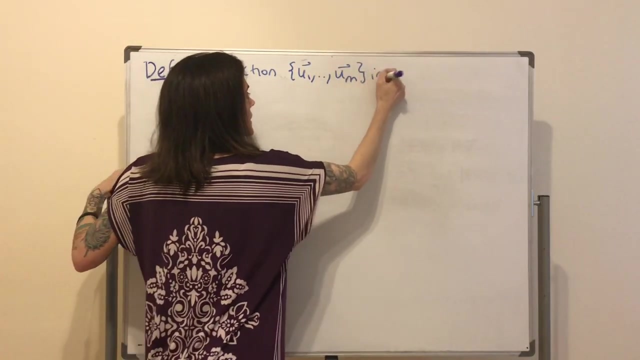 So this is the distance between these two vectors. Now we'll move into the orthonormal bases. The definition: a collection of vectors- let's say I call them u one to u m n r n- is what's referred to as u one to u m n r n. 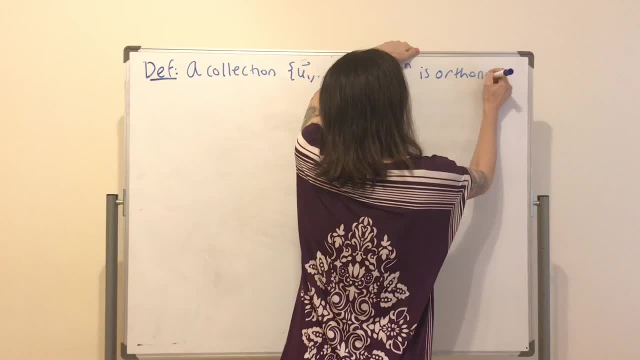 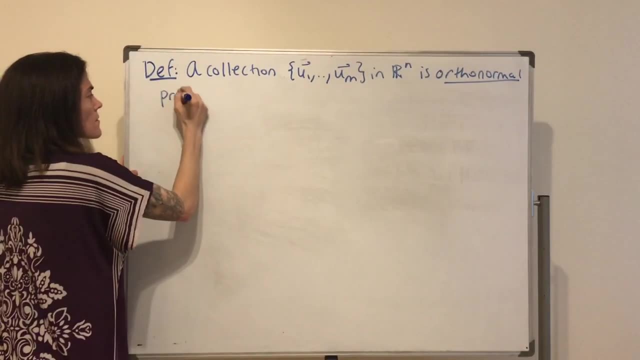 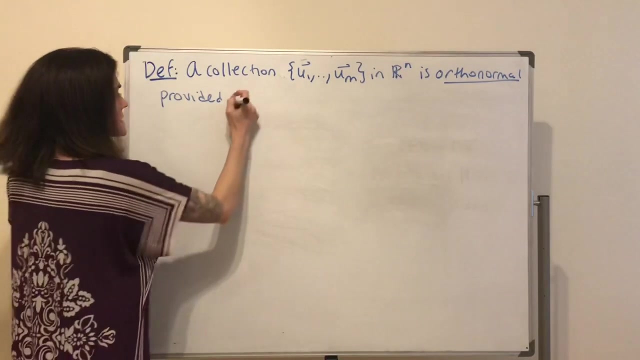 u one to u m n r n is what's referred to as u one to u m n r n What's referred to as orthonormal provided. well, we need two things to be orthonormal. We need that each vector is unit. 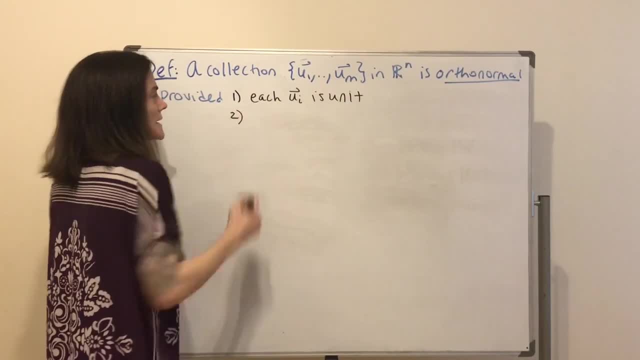 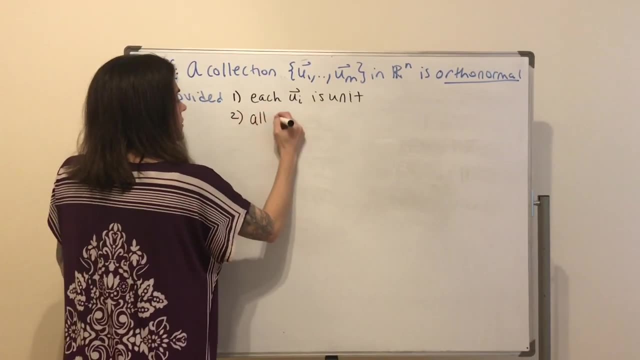 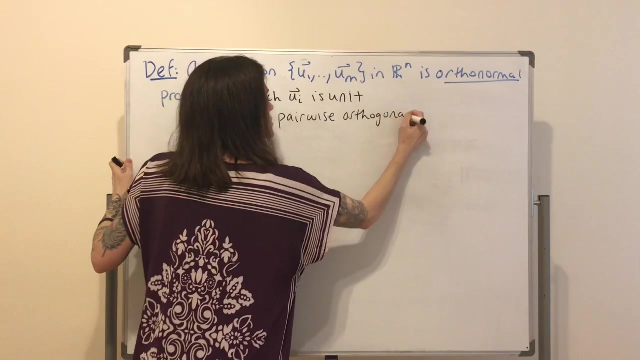 meaning it has length one. and the second thing we need is that they're all, are also orthonormals and that means that they're all orthonormals, so they are all. I'll say pairwise orthogonal, meaning you take any two of 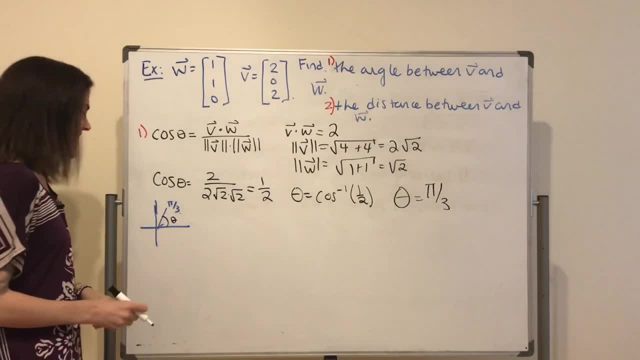 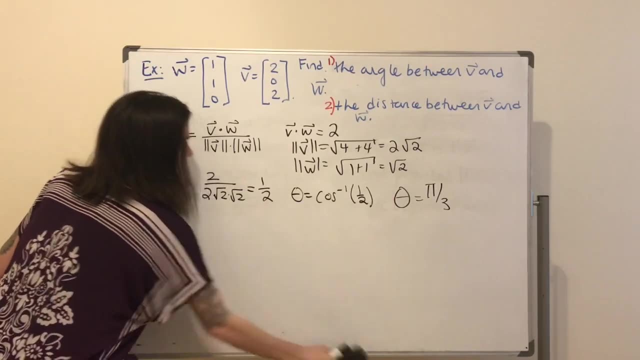 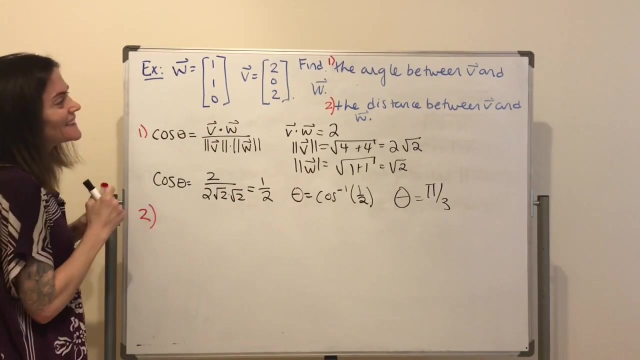 And this is the number one. Okay, now let's move on to number two. Maybe I'll erase my picture that was helping me think about how to figure out theta. Maybe I'll erase my picture that was helping me think about how to figure out theta. 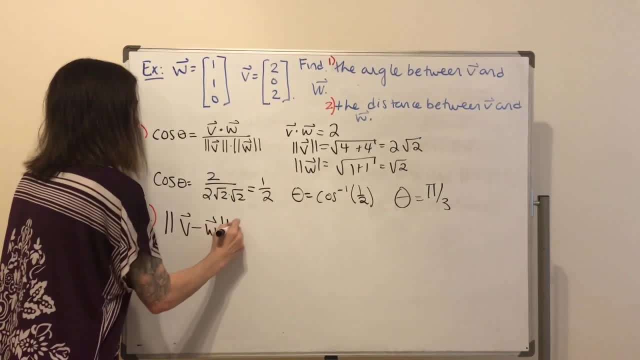 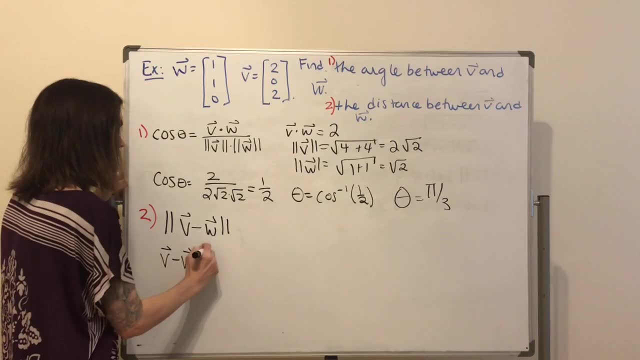 I need this v minus w, And this will just be well. first let's compute v minus w, and then I will compute the length. This gives us the distance between the two vectors. This is minus one, one minus two. 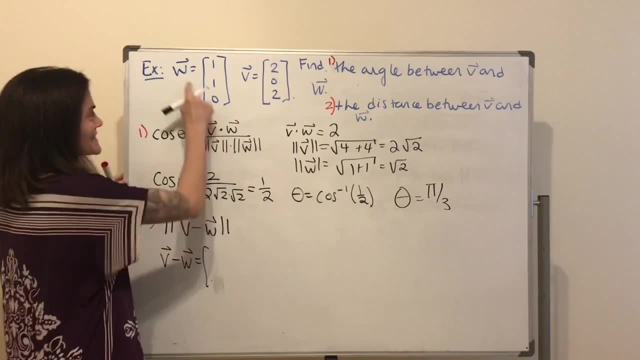 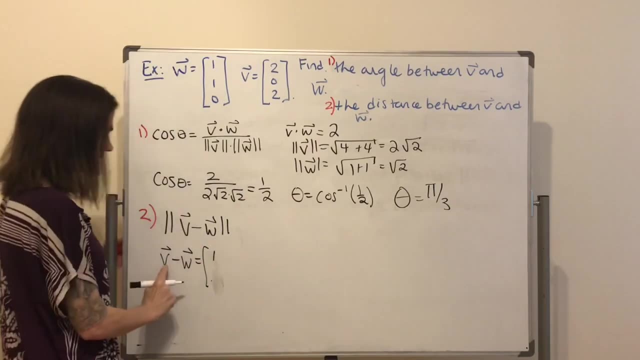 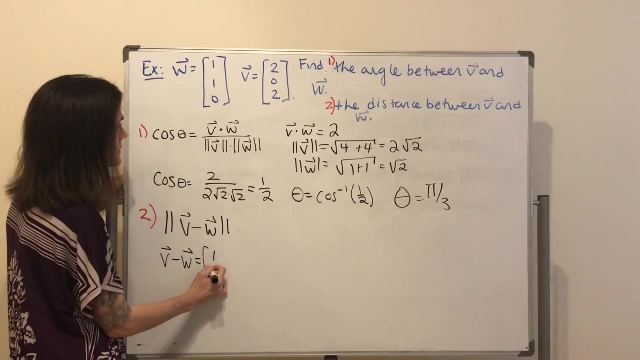 Oh, I did w minus v. Well, I was looking here: V minus w. Pardon me, Reality is I would get the same Length. but since I wrote v minus w, let's actually do v minus w. One minus one minus two. 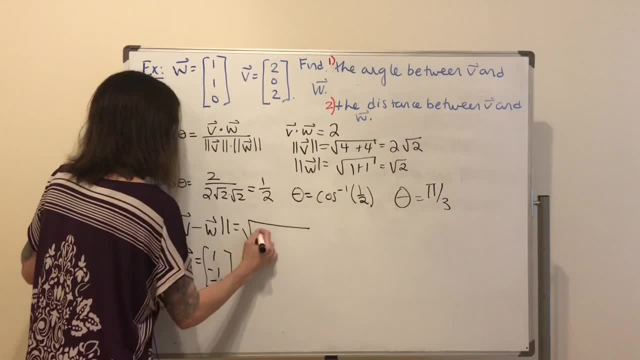 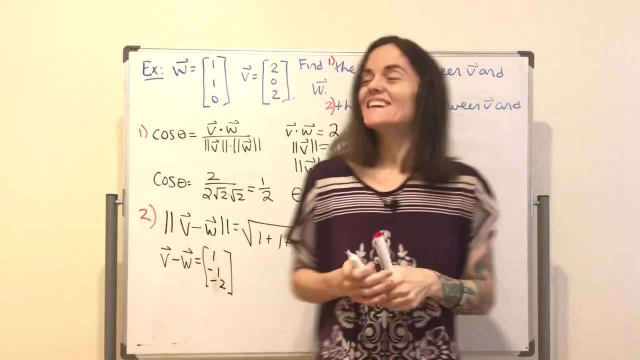 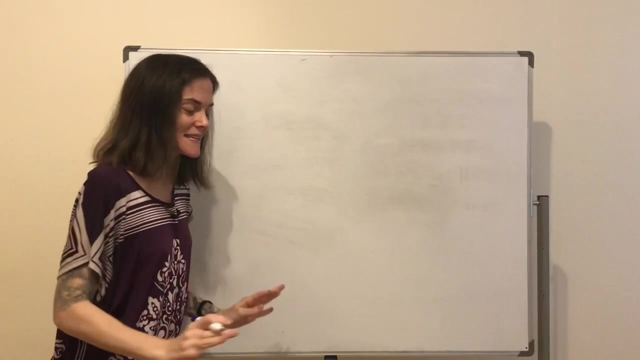 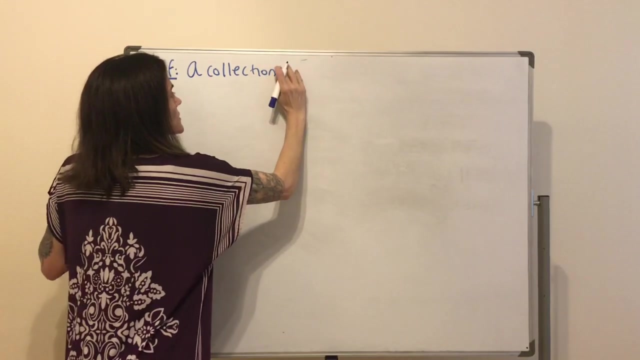 Okay, and then this is the square root. It's one plus one plus four, It's the square root of six. So this is the distance between these two vectors. Now we'll move into the orthonormal bases, The definition, a collection of vectors. 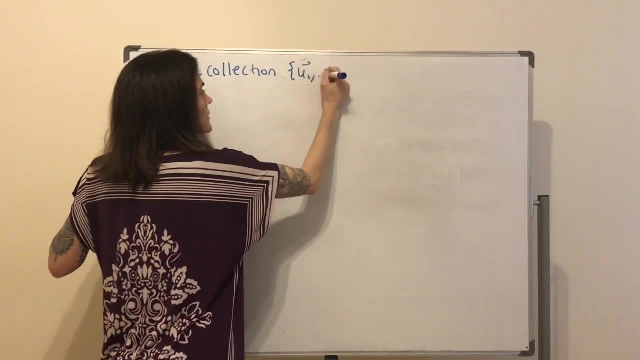 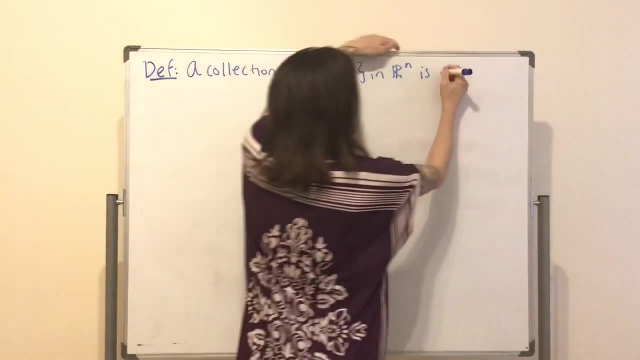 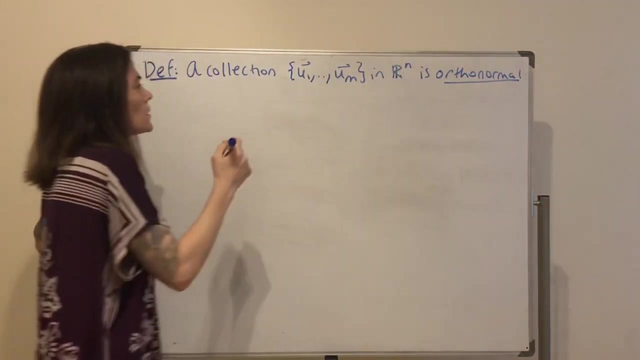 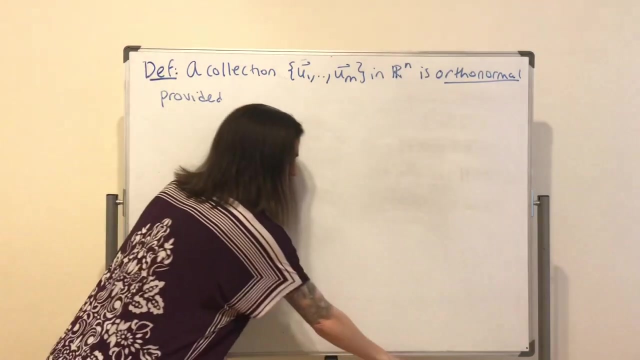 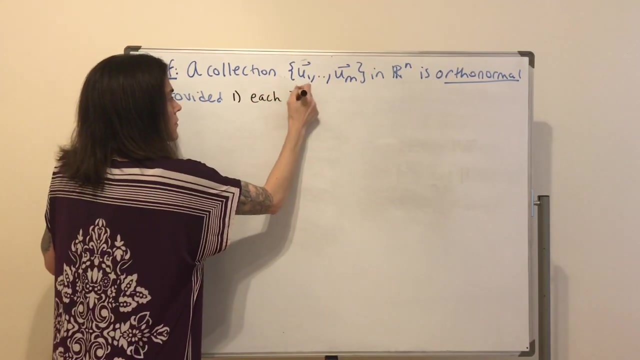 Let's say I call them u1 to umnrn. is what's referred to as orthonormal, Orthonormal Provided? Well, we need two things To be orthonormal. we need that each vector is unit, Meaning it has length one. 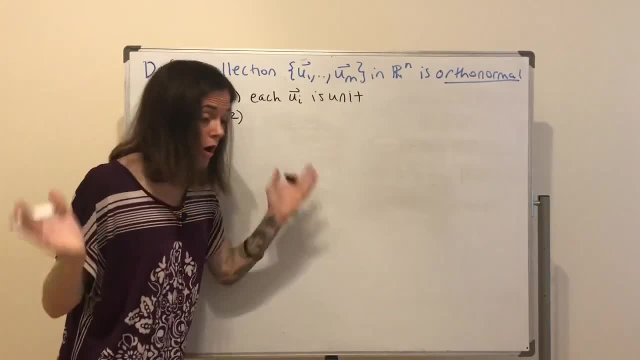 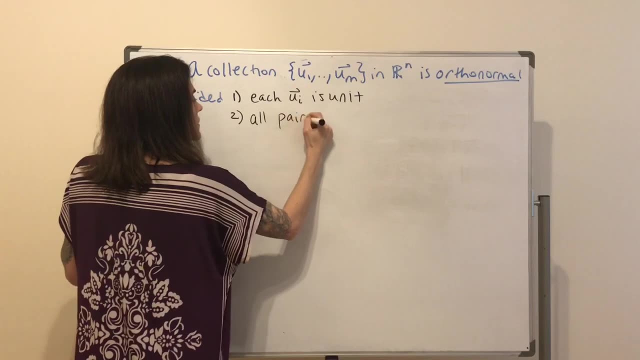 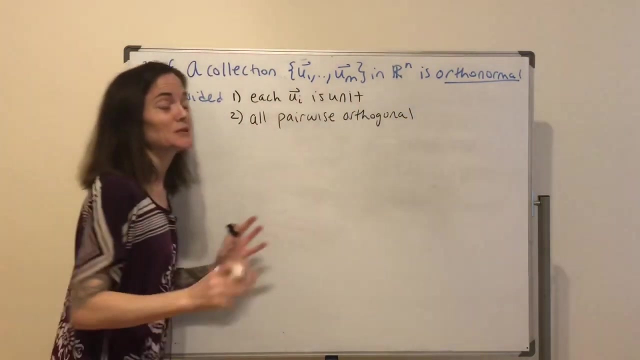 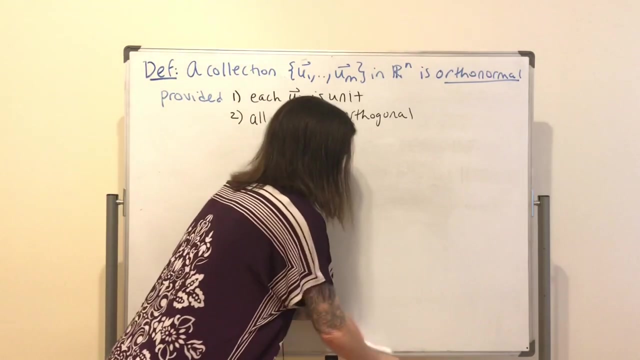 And the second thing we need is that they're all orthogonal. So they are all I'll say. pairwise orthogonal Meaning you take any two of them, any two different ones, you take their dot product and you get zero. So another way we could write this is entirely of the dot product. 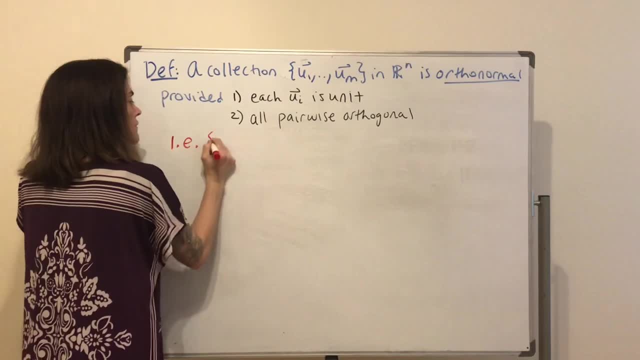 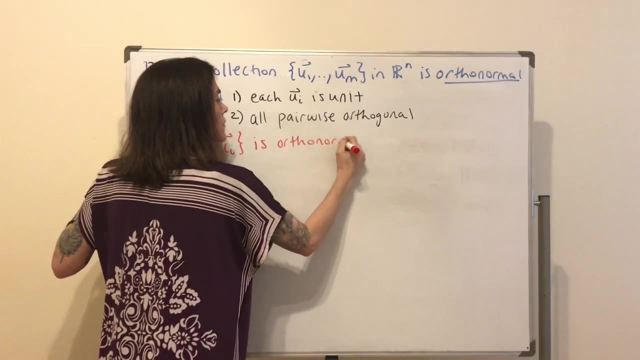 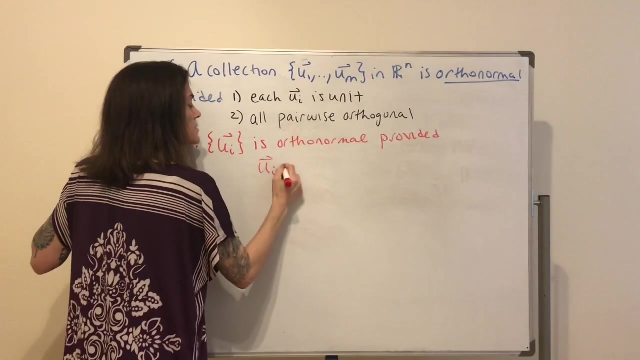 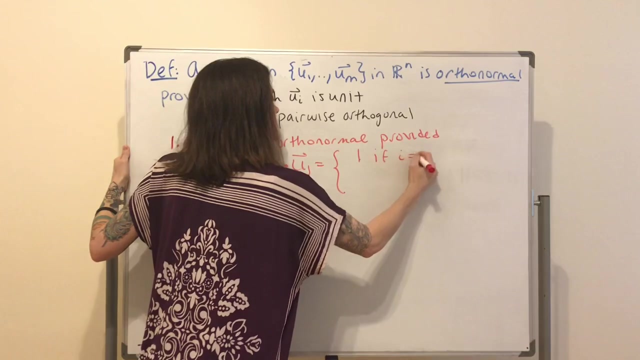 So, in other words, this collection collection is orthonormal, Orthonormal Provided. if I take ui dotted with uj, I get one of two things. I get one. if i is not equal to j, Oh, pardon me. 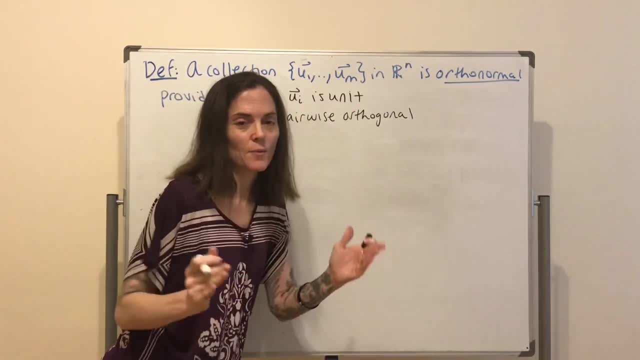 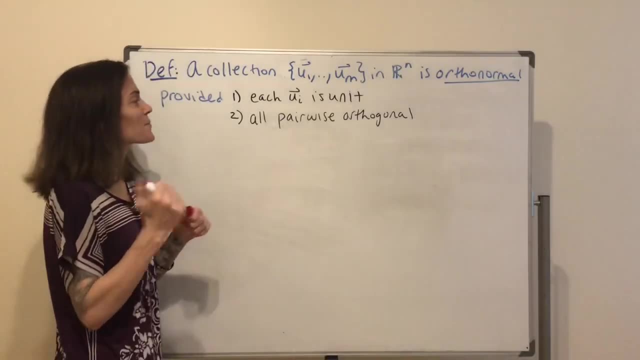 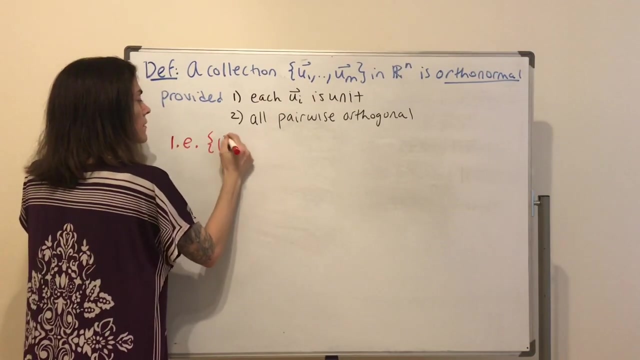 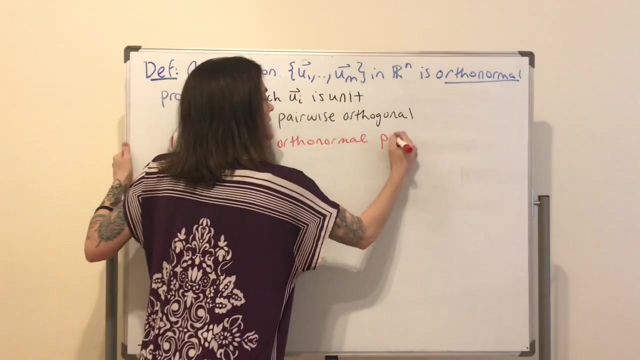 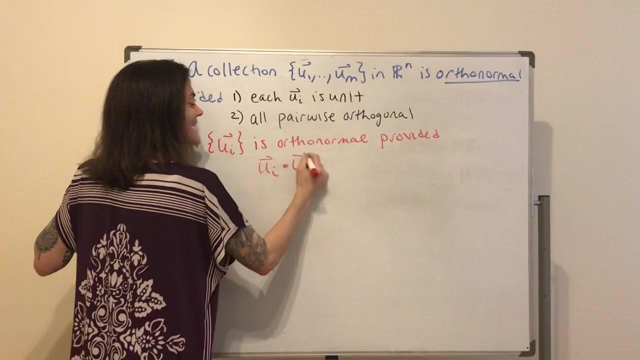 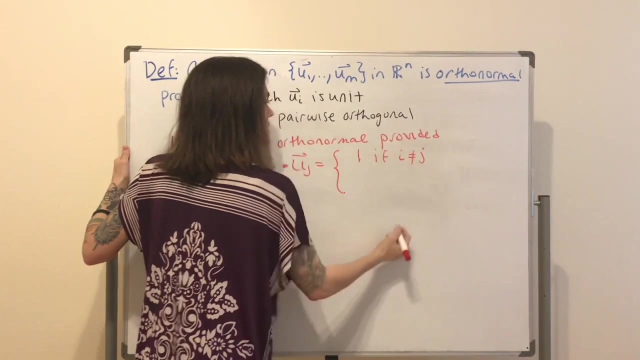 them any two different ones. you take their dot product and you get zero. so another way we could write this is entirely of the dot product. so in other words, this collection collection is orthonormal. provided if I take U I dotted with U, J, I get one of two things. I get one if I is not equal to J. oh, 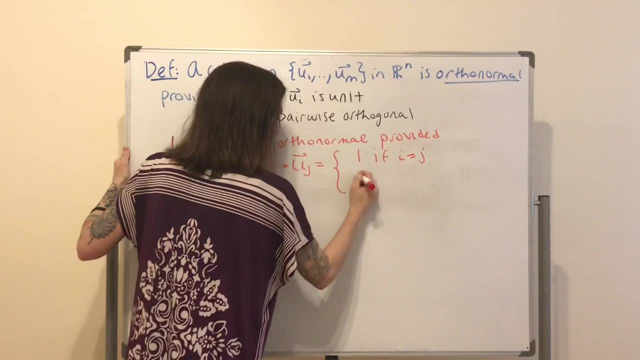 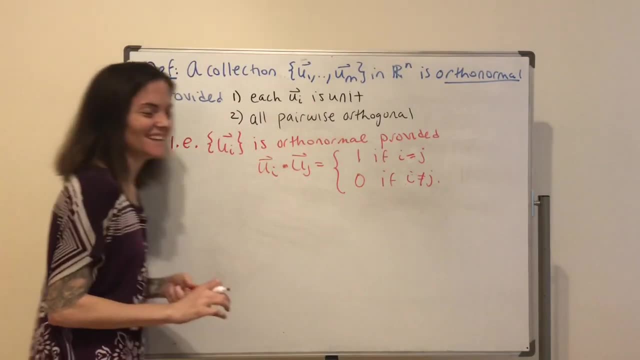 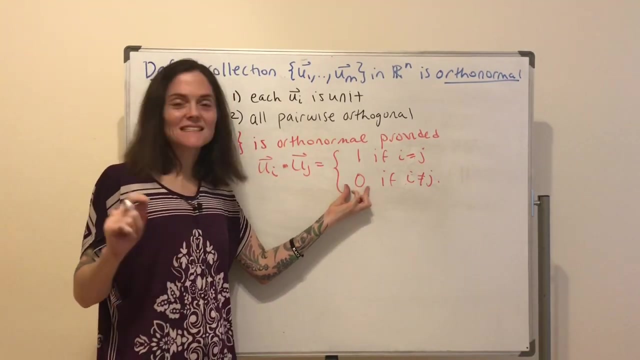 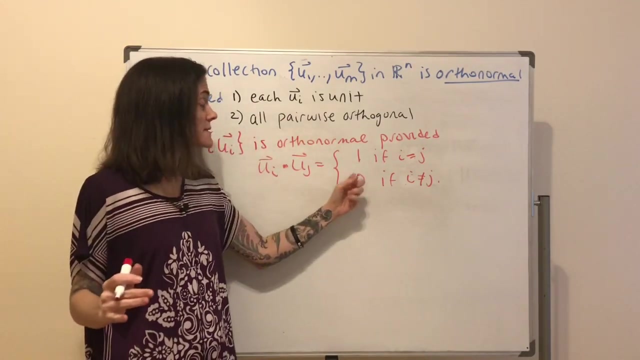 pardon me this way if I is not equal to J. okay, then let me tell you what each one means, since I started to write it wrong here. this is saying that you take any two different ones. they are orthogonal. right there, dot product is zero and this one, if you have. 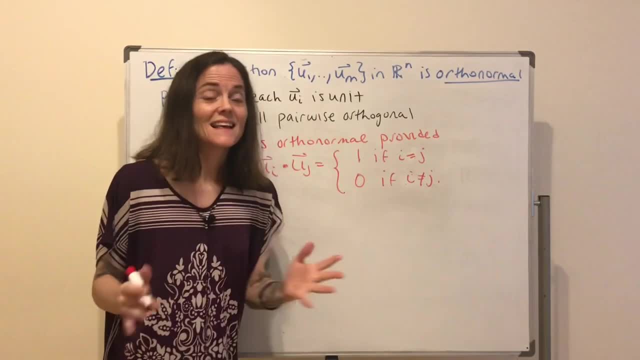 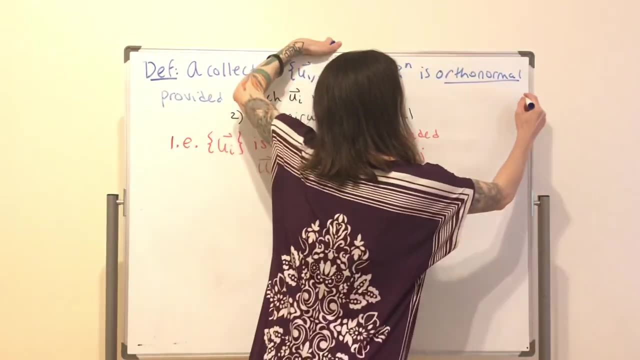 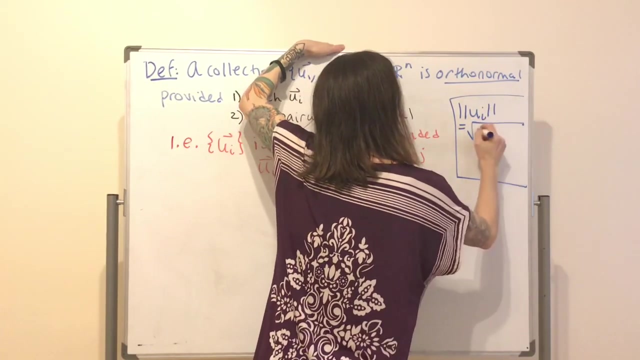 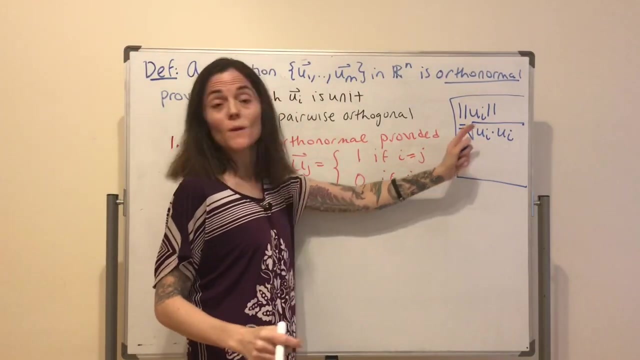 a vector dotted with itself and you get one. this means it's unit, right? because the definition of the length- this is maybe a comment I'll put in a box- the definition of this is: it's the square root of U I dot U I, and so if U I dot U I is one, then so is the square. 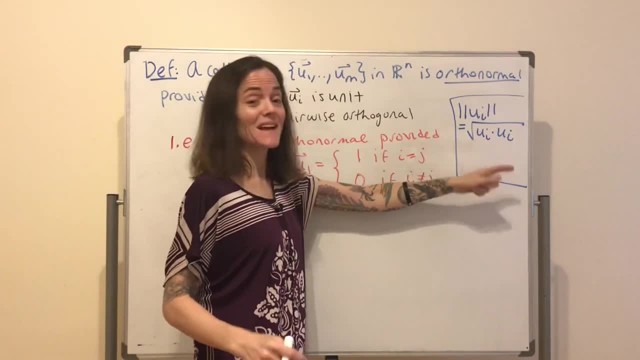 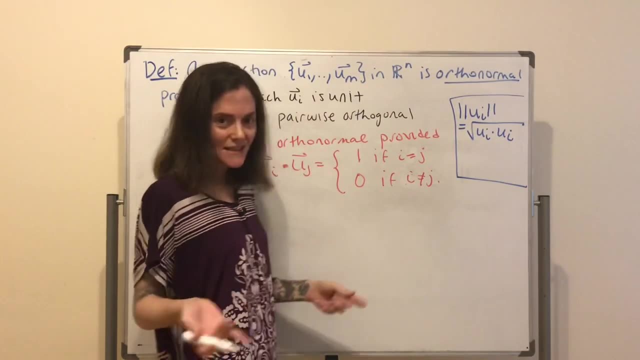 root and similarly, if the square root of U I dot U I is one, then so is U I dot U I. so saying that you take a vector, dot it with itself and you get one, it's equivalent to saying it's unit: okay, that's the only time you have linked one. 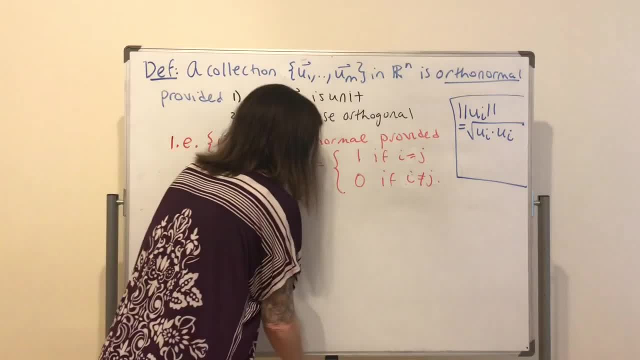 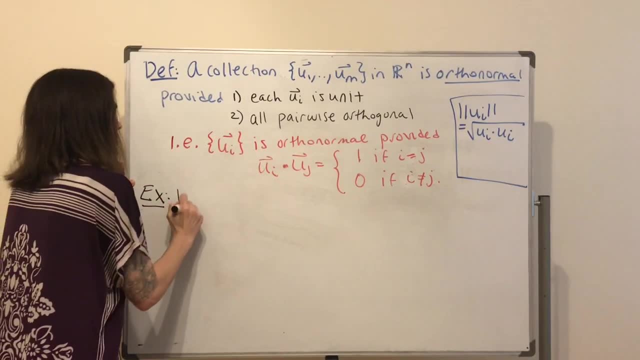 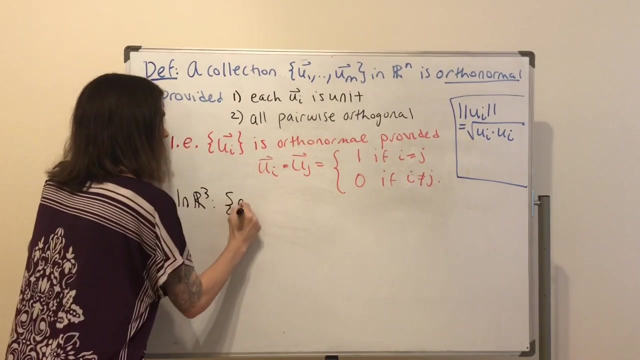 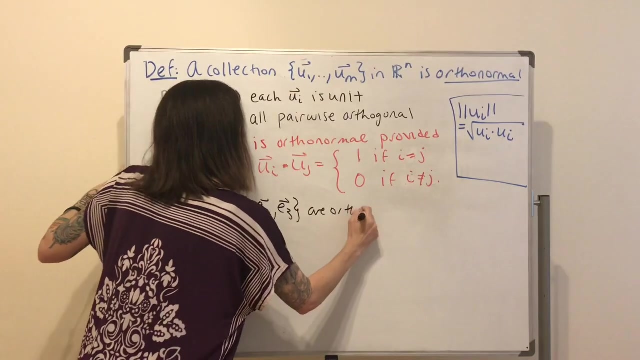 okay, so this is what characterizes orthonormal collection of vectors. so well, what are some examples? let's speak about R3 for the moment, this E1, E2 and E3- these are orthonormal. these were our standard or so normal. these are our. 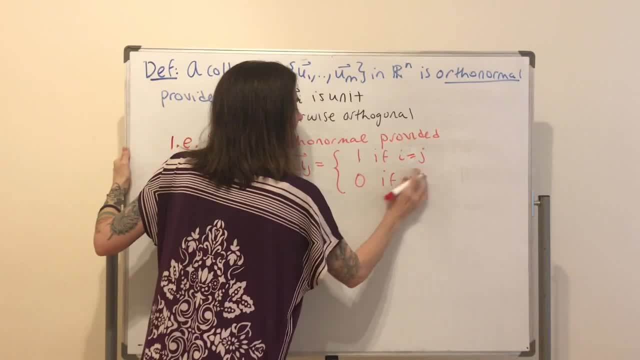 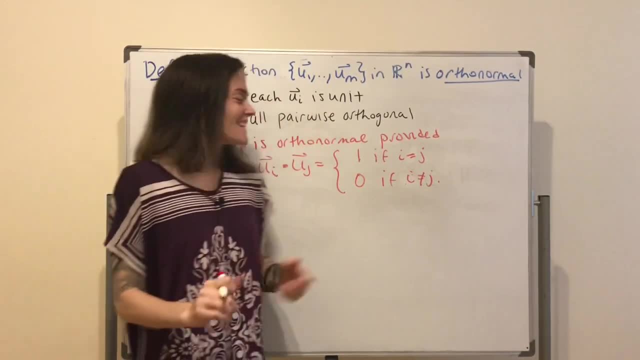 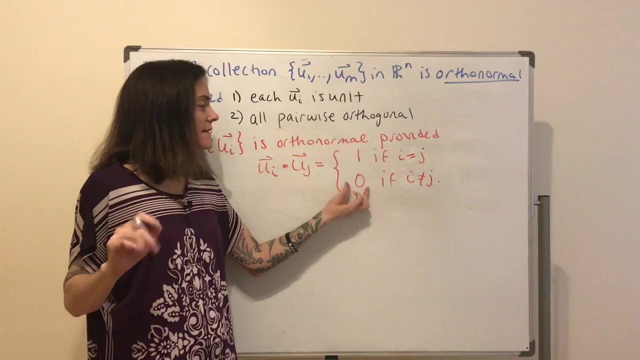 This way zero if i is not equal to j. Okay, And let me tell you what each one means, since I started to write it wrong Here. This is saying that you take any two different ones, They are orthogonal, right? They're dot product to zero. 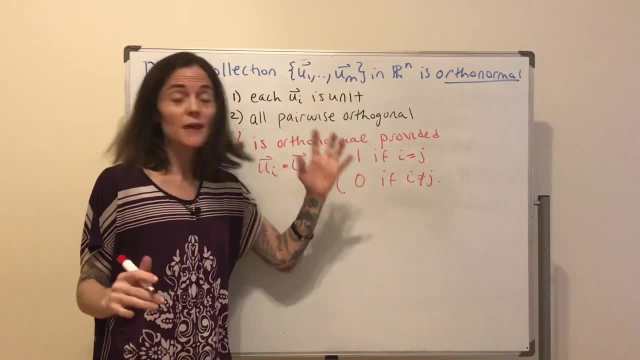 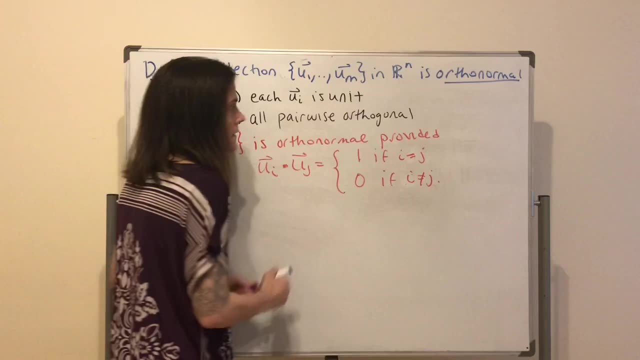 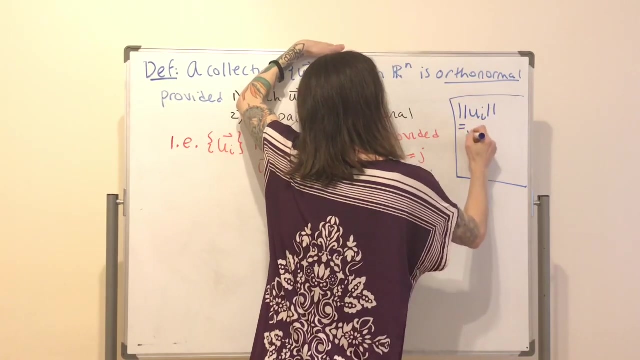 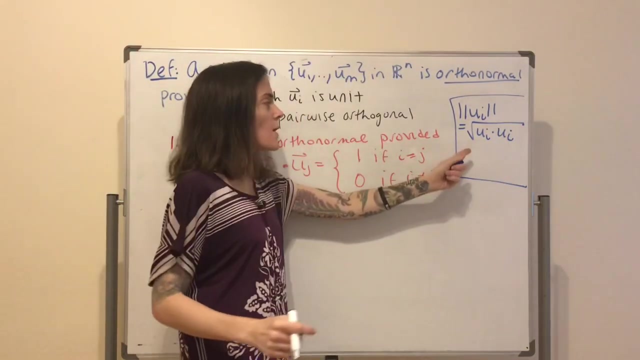 And this one: if you have a vector dotted with itself and you get one, this means it's unit, right? Because the definition of the length- This is maybe a comment I'll put in a box- The definition of this Is: it's the square root of ui, dot ui, and so if ui, dot ui is one, then so is the square root. and similarly, if the square root of ui, dot ui is one, then so is ui, dot ui. 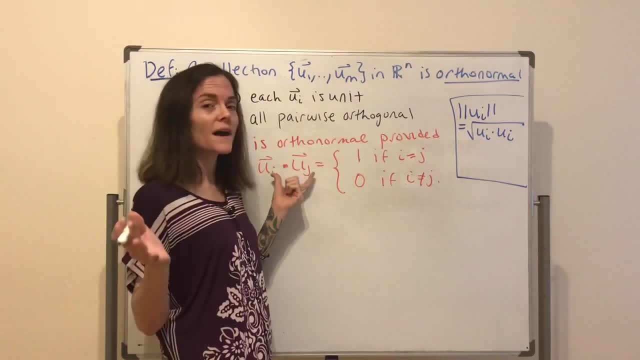 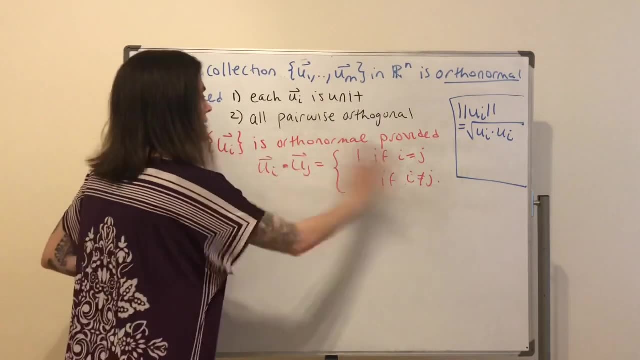 So saying that you take a vector dotted with itself and you get one, it's equivalent to saying: it's unit, Okay, That's the only time you have linked one. Okay, so this is what characterizes orthonormal collection of vectors. 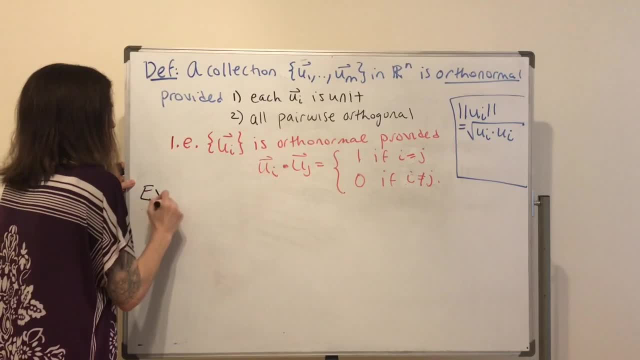 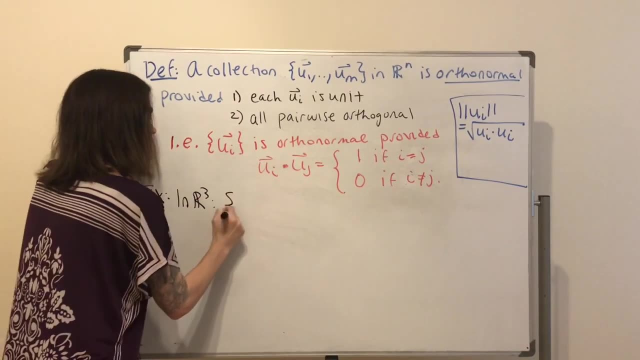 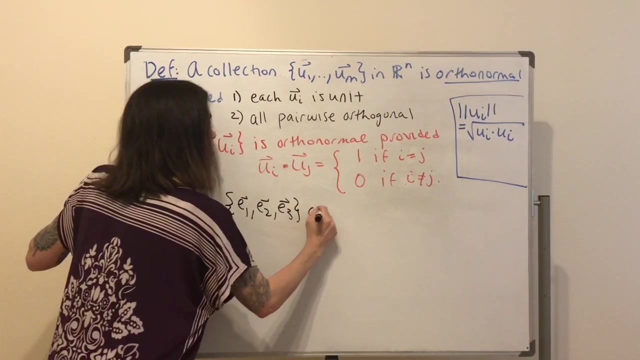 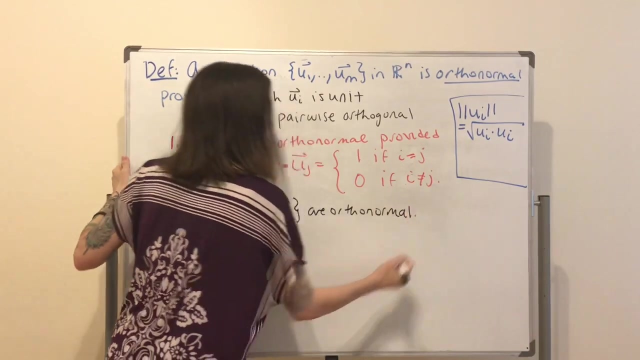 So well. what are some examples? Let's speak about R3 for the moment, This E1,, E2, and E3, these are orthonormal, These were our standard orthonormal, These are our standard vectors. and R3, where you have a one and one component, zero everywhere else. 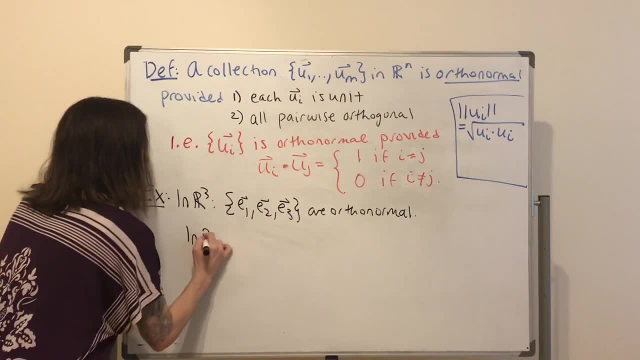 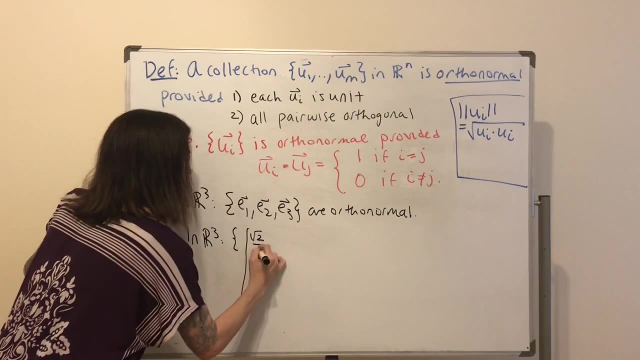 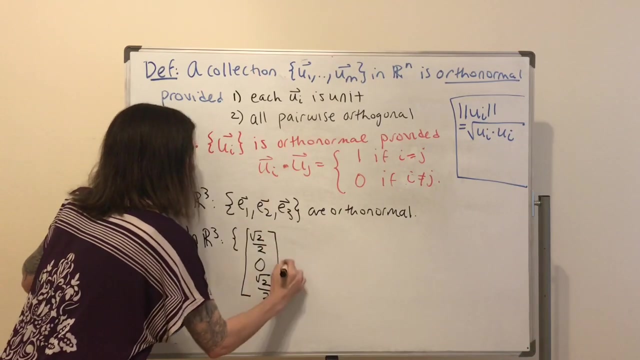 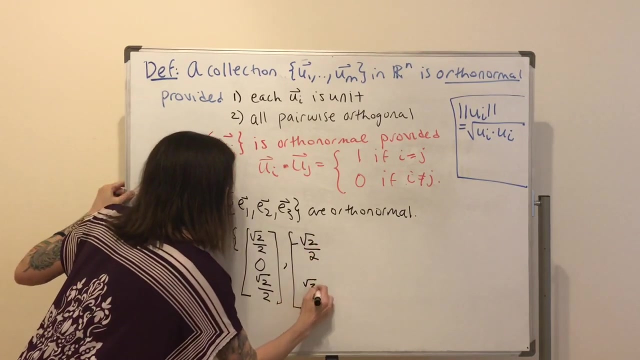 Okay, what else? These are not the only orthonormal collections. Maybe I'll just do two if I took. Okay, and that's one vector. And then how about I do Okay, Okay, Okay, Okay, Okay Okay. 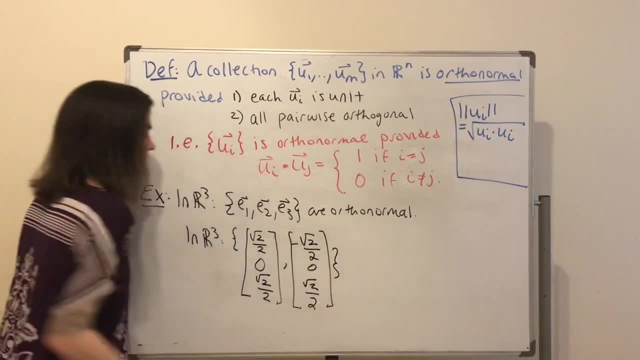 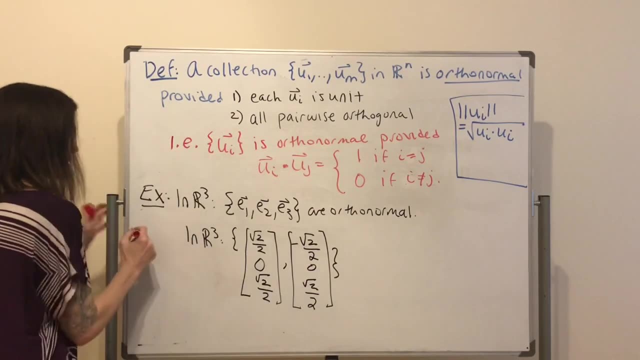 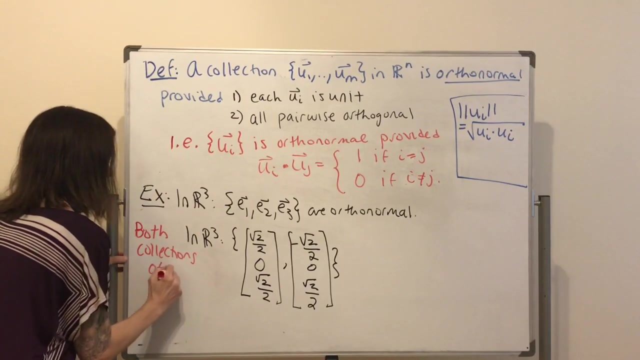 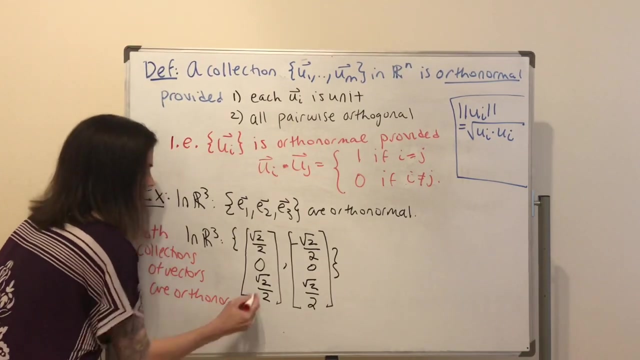 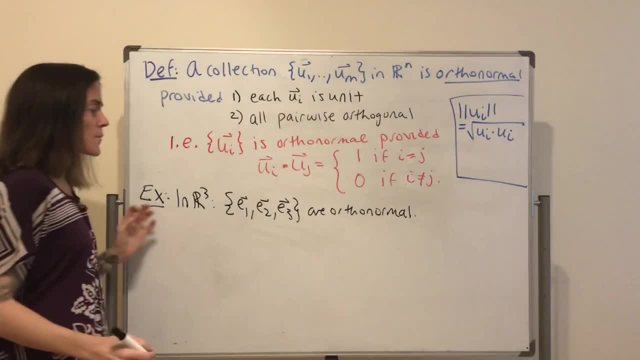 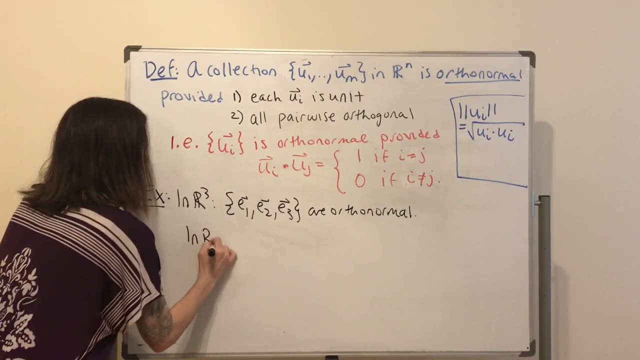 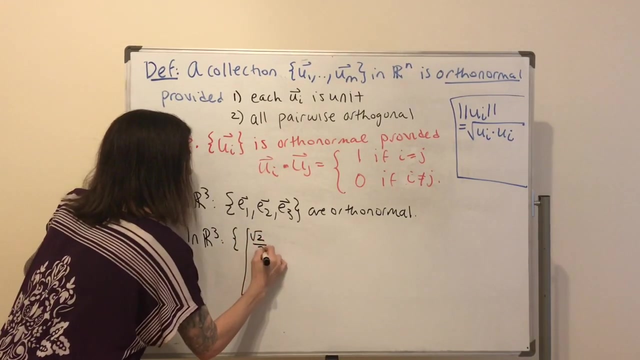 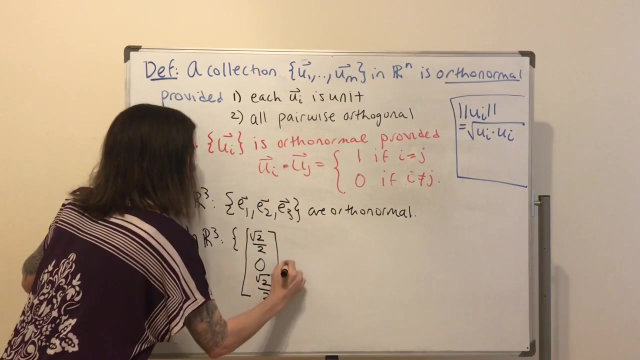 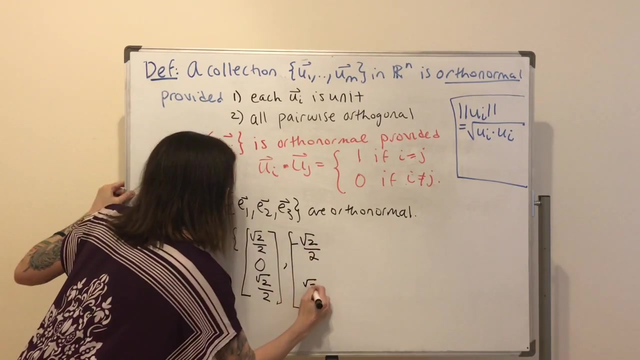 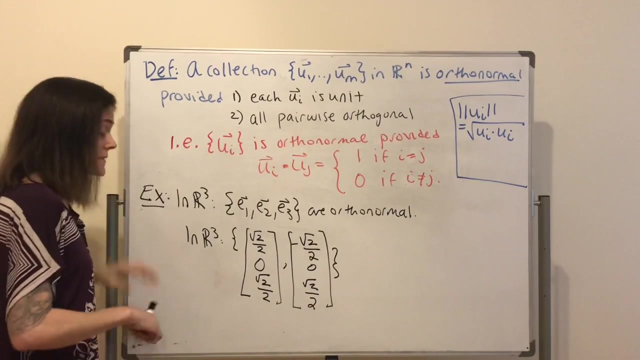 these are our standard vectors and our three, where you have a one and one component, zero everywhere else. okay, what else? these are not the only orthonormal collections. maybe I'll just do two, if I took okay, and that's one vector, and then how about I do? both of these are orthonormal collections, maybe. 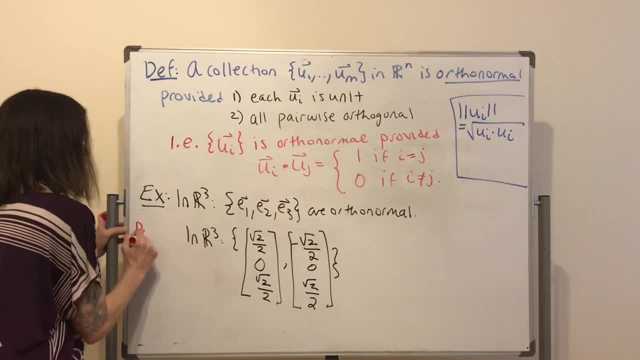 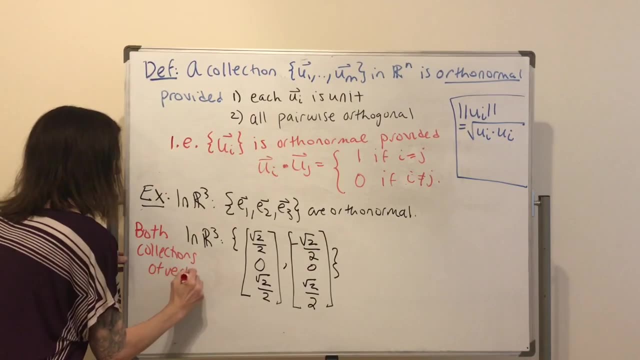 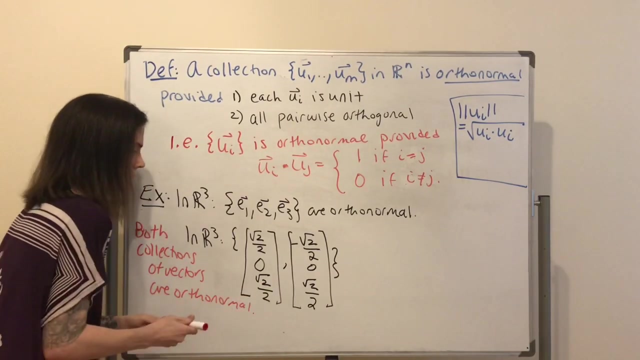 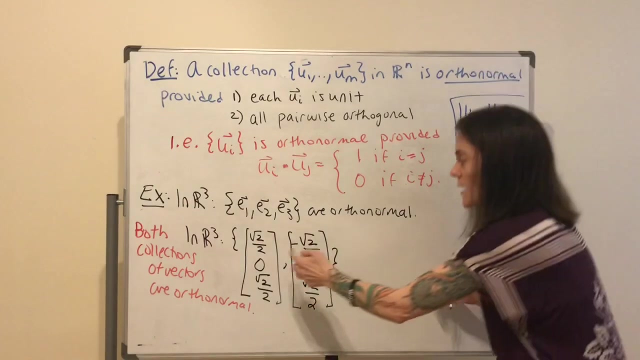 I should write that both of these collections of vectors are orthonormal. this one if this one, might be the easiest to think about. if you don't aren't sure about the second collection, well, what is the length of one of these, or what is the dot product of one with itself? if you take the square root of 2, 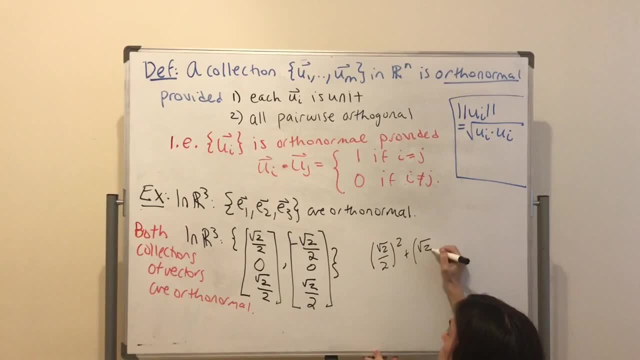 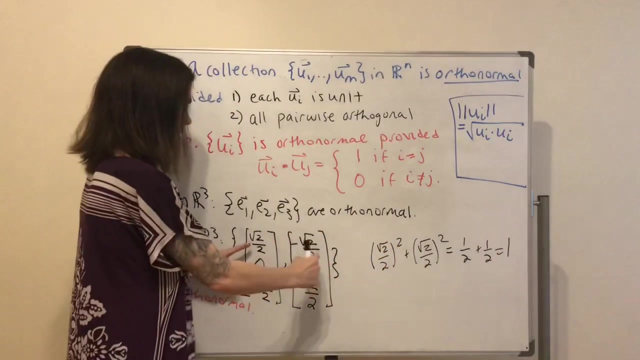 over 2 squared, plus the square root, 2 over 2 squared, which is, even though this is a minus, this would be what you'd calculate for both you. this is: this is a half plus a half, which is one right that would. so this says that both of these are our unit. and then you can also see: here you get negative. 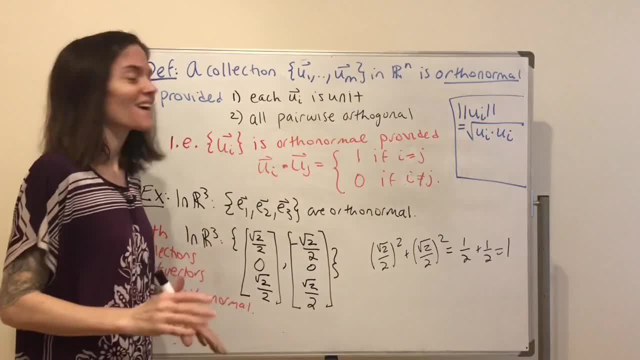 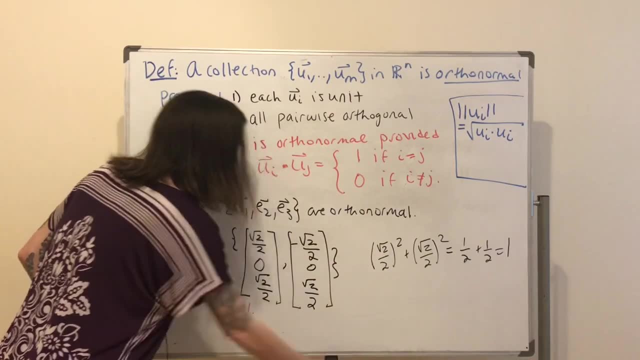 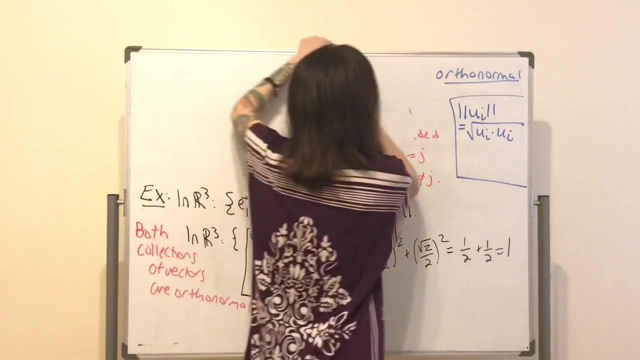 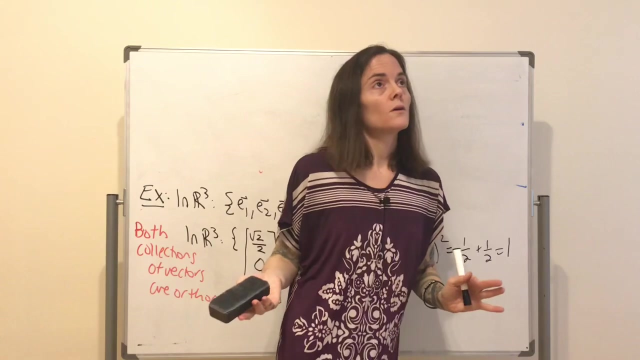 and positive of the same thing, so they are also orthogonal. so here are two collections of orthonormal vectors in our three. now the next thing that I want to say- or we will actually prove, is that if you have a collection of orthonormal, oh yeah. 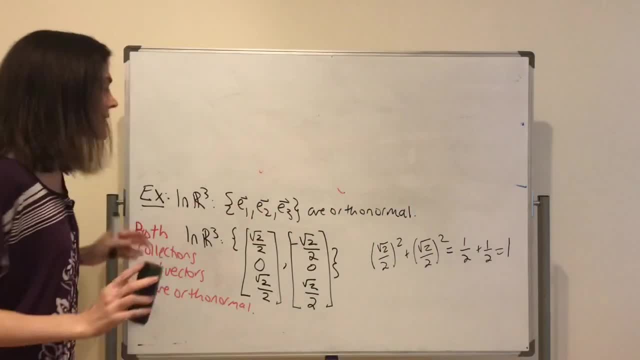 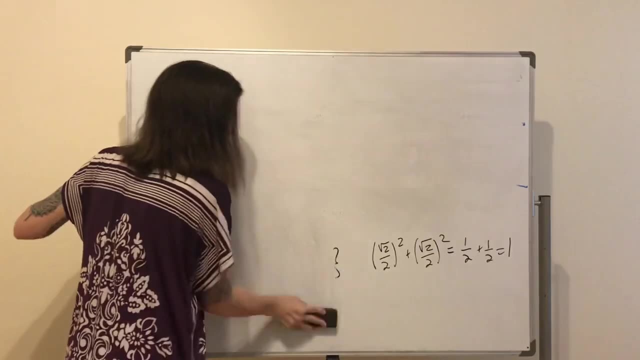 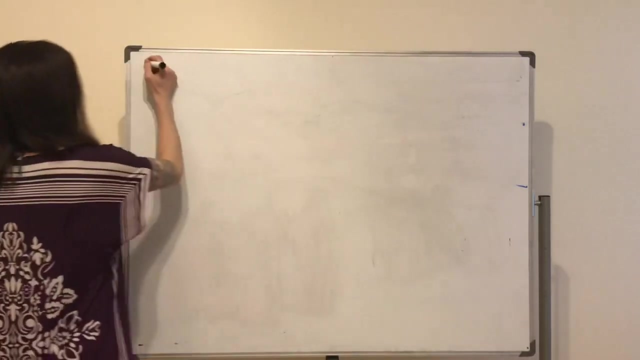 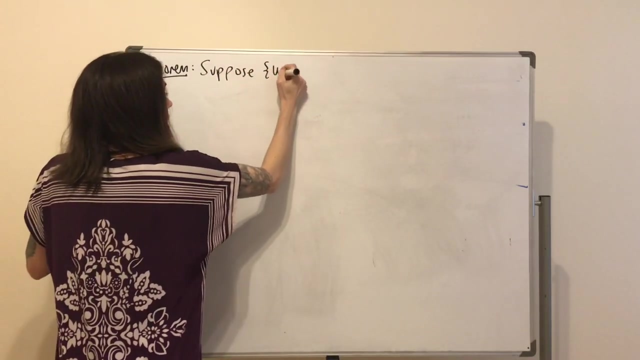 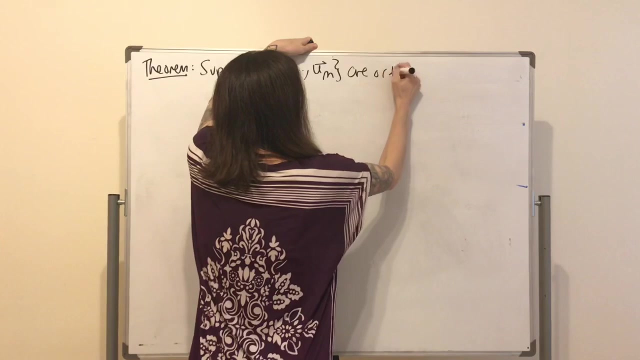 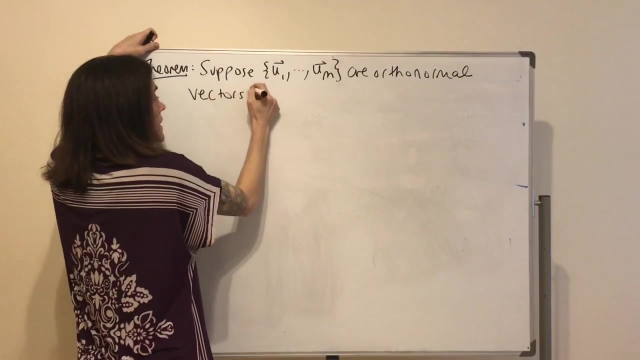 I'll say it this way: orthonormal vectors in our n, then the collection is literally independent, and this is what will lead us to make a definition of orthonormal basis. okay, so theorem simplification: suppose we have u1 to bump us to u, m and these are orthonormal vectors in're. 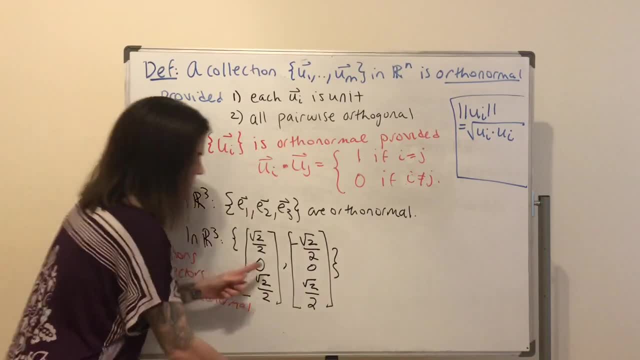 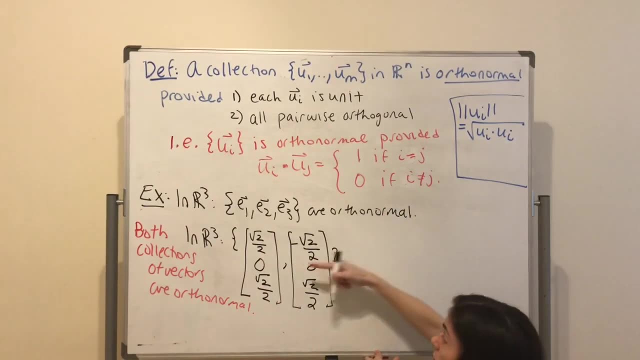 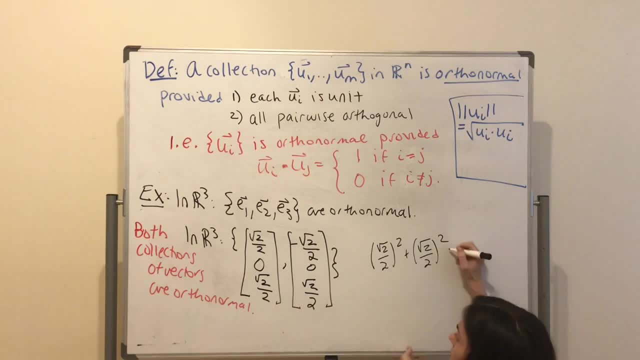 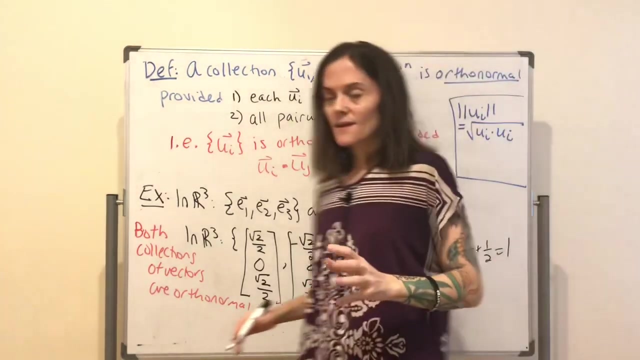 is, even though this is a minus, this would be what you'd calculate for both. this is: this is a half plus a half, which is one right that would. so this says that both of these are our unit. and then you can also see: here you get negative. 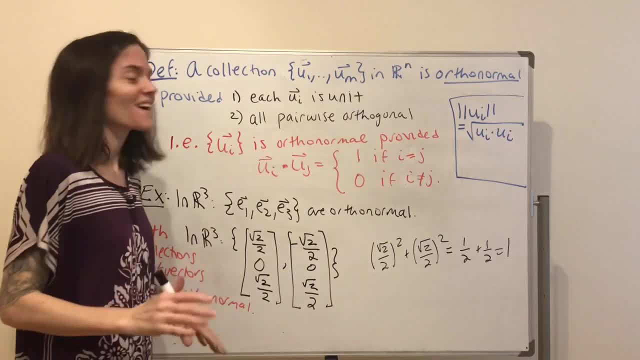 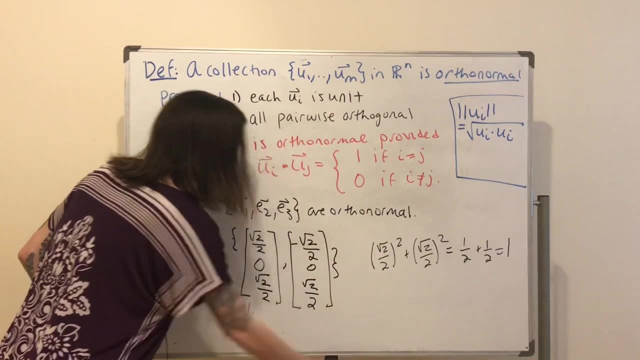 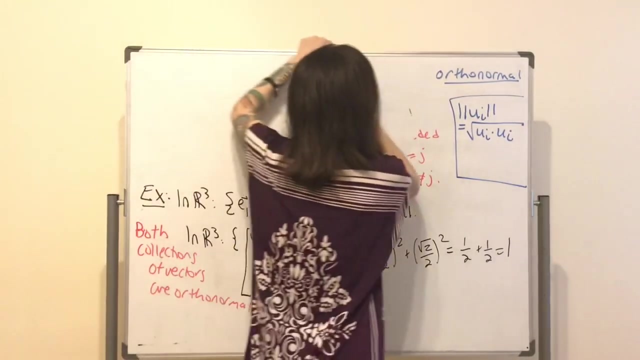 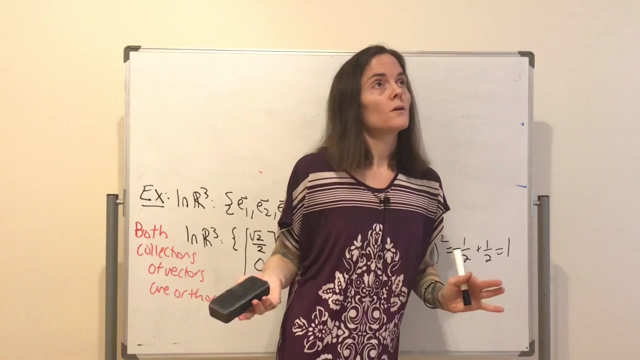 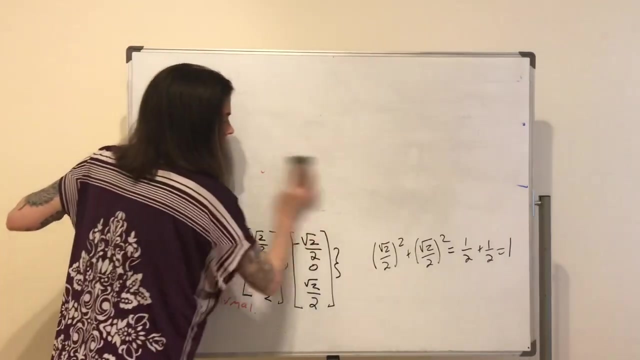 and positive of the same thing, so they are also orthogonal. so here are two collections of orthonormal vectors in our three. now the next thing that I want to say, or we will actually prove, is that if you have a collection of orthonormal- oh yeah, I'll say it this way- orthonormal- vectors in our n, then the 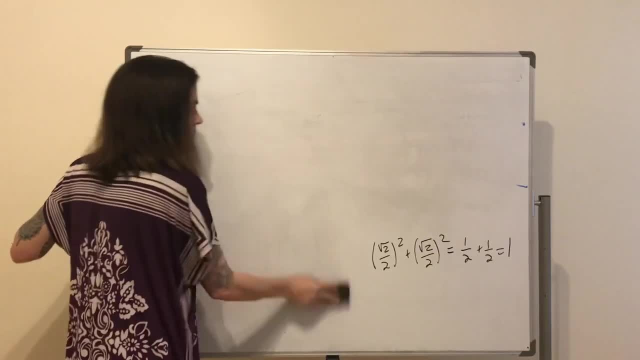 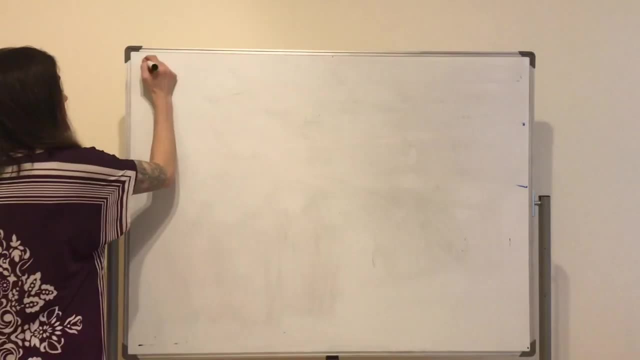 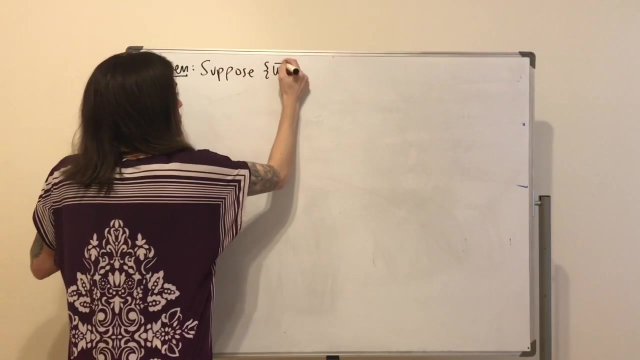 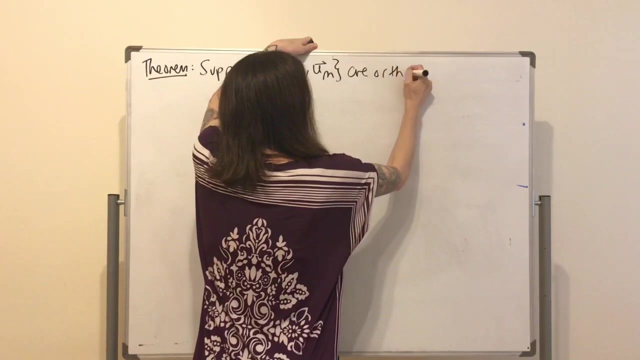 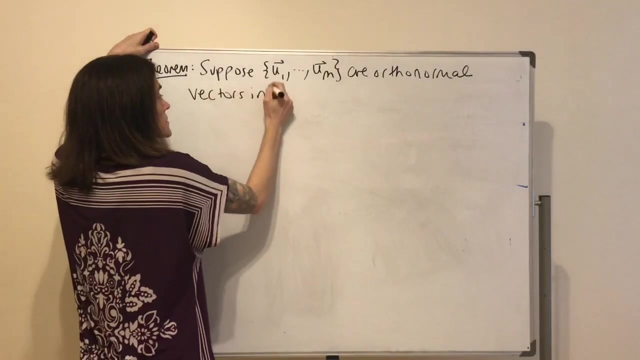 collection is literally independent, and this is what will lead us to make a definition of orthonormal basis. okay, so theorem suppose we have u1 to UM. okay, so theorem suppose we have u1 to UM. okay, so theorem suppose we have u1 to UM. and these are orthonormal vectors in our 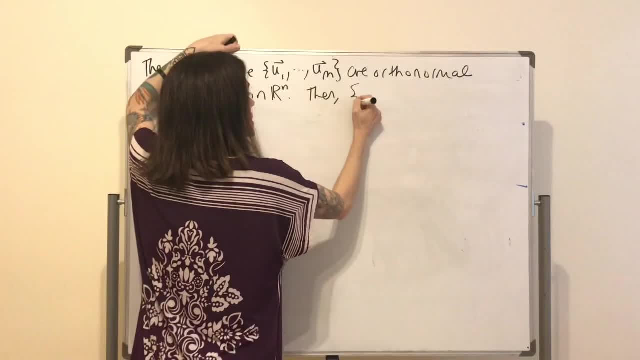 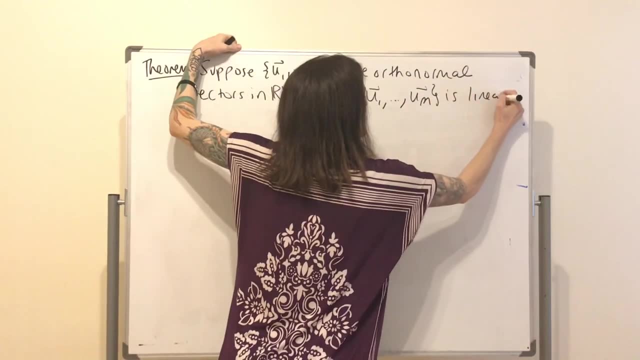 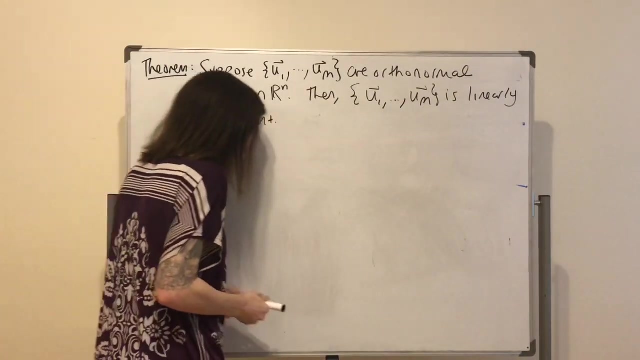 and these are orthonormal vectors in our and these are orthonormal vectors in our: n then this collection is linearly n. then this collection is linearly n. then this collection is linearly independent, and this I will prove okay, independent, and this I will prove okay. 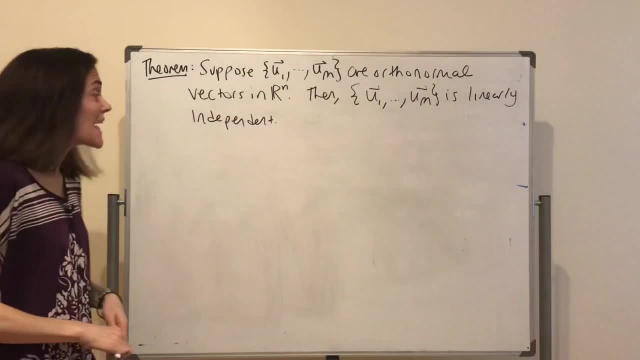 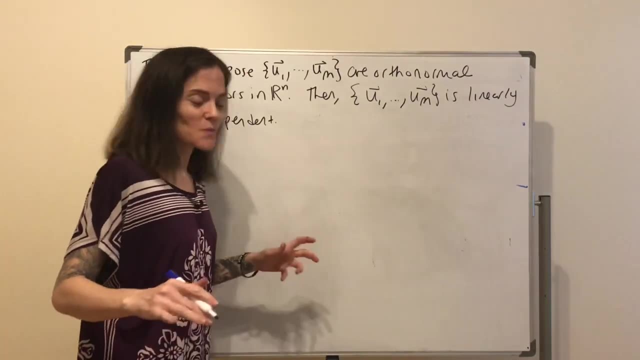 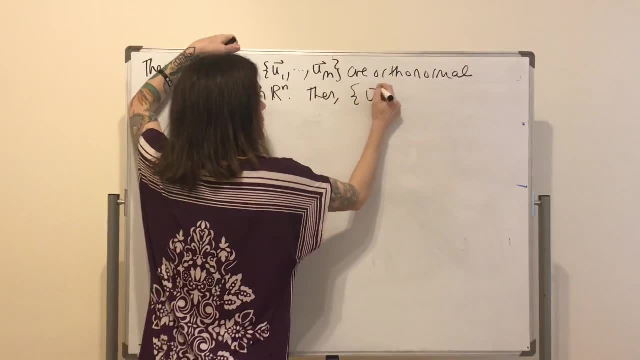 then this collection, this collection Exc parfait, is linear theta square root r, that's R times 0.75 talked about. if you have a value of one first, then dot thor işte, abus additions. enter the sub Bye, because this is mayonnaise, suppose if you have a whole starts from a U by. this is like an odd class. 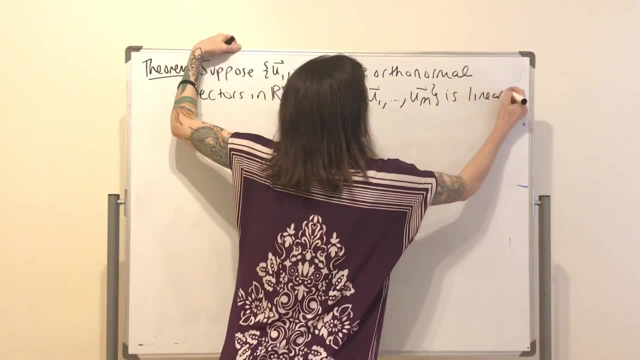 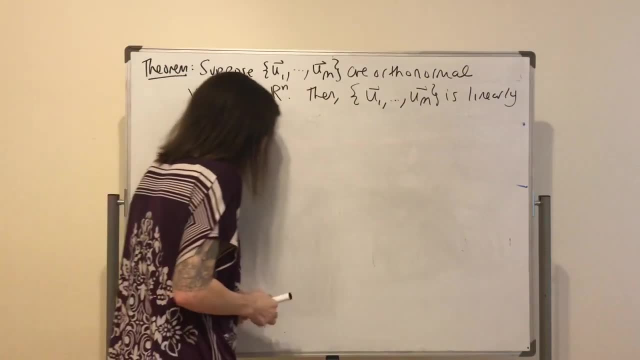 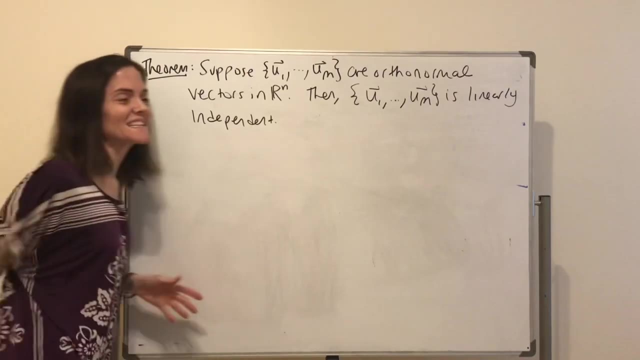 but even if you are right, if x is better- because x might help you find out how you really care about the better vet- is linearly independent, and this I will prove okay. well, how do you prove this? or what is one way, and I mentioned when we first started talking about linear: 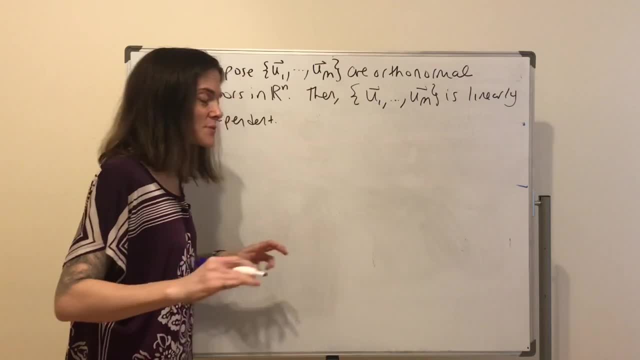 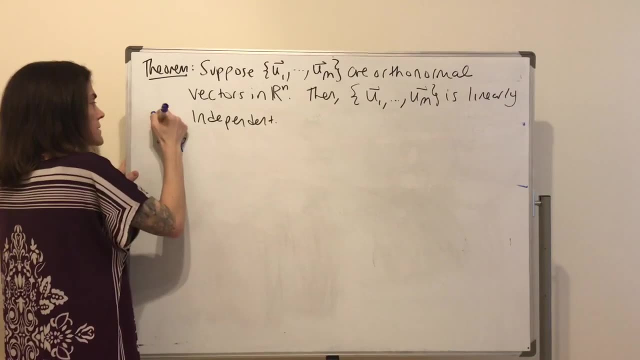 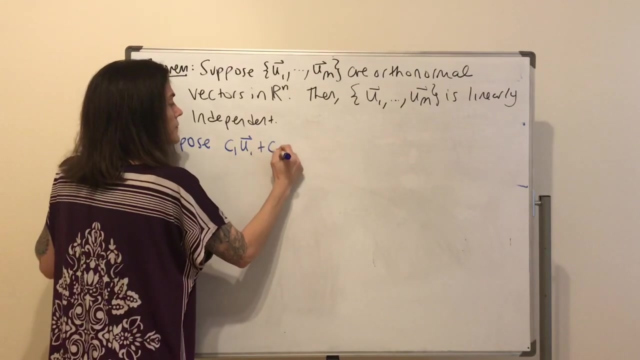 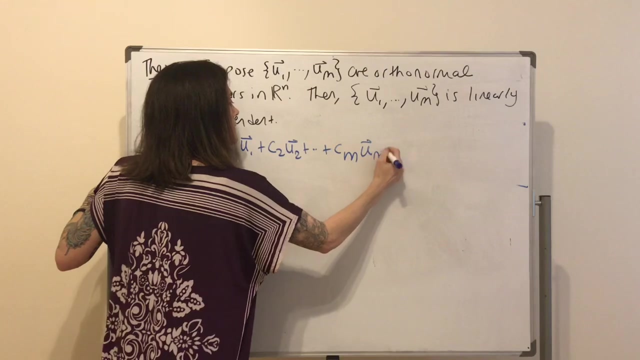 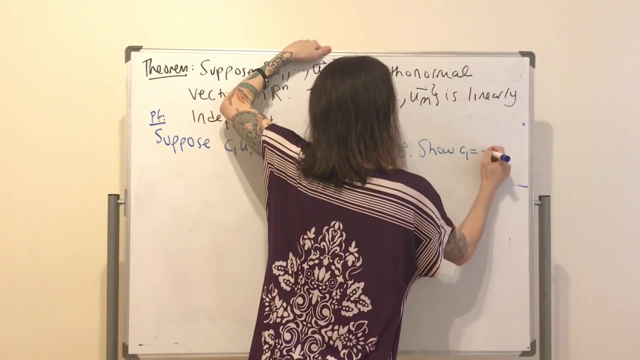 independence, that this is one way that's very natural to prove, because one of the criteria was if, then, and so this is how I will prove this. so suppose I have some linear relation among these vectors and then I just need to show that all the C eyes are zero, see zero. 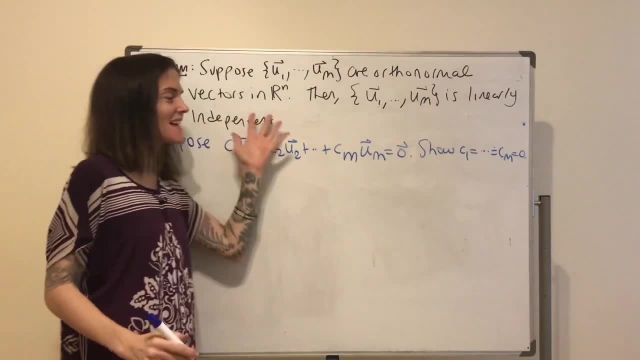 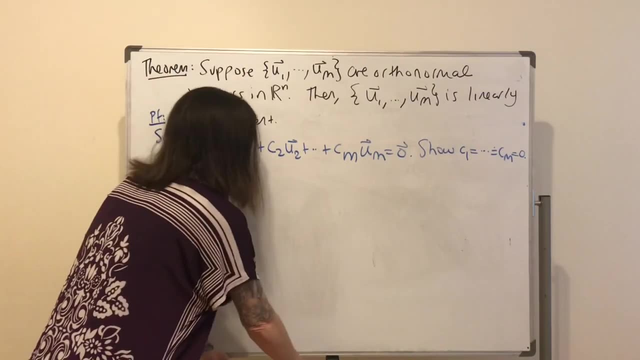 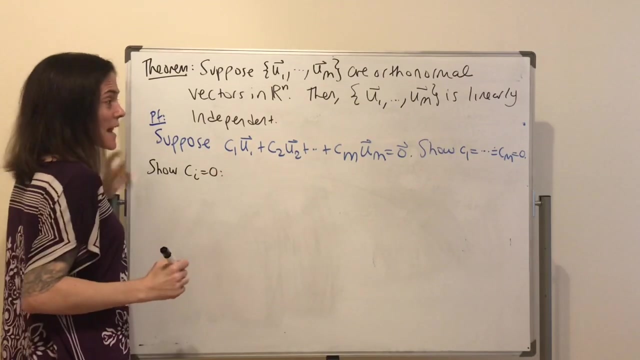 and this will prove that this collection is linearly independent. How do we do this? Well, here's what I'm gonna do. So let's show C, i is zero And I'm working generally. let i be some number between one to m. 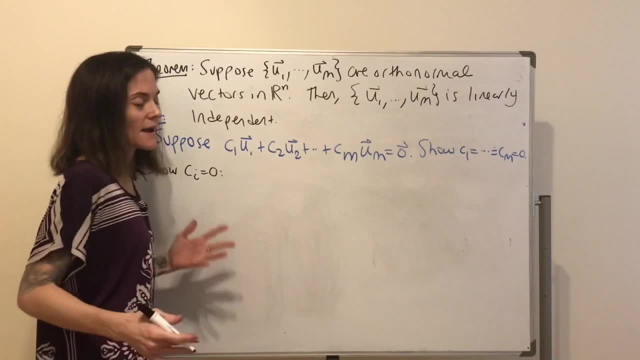 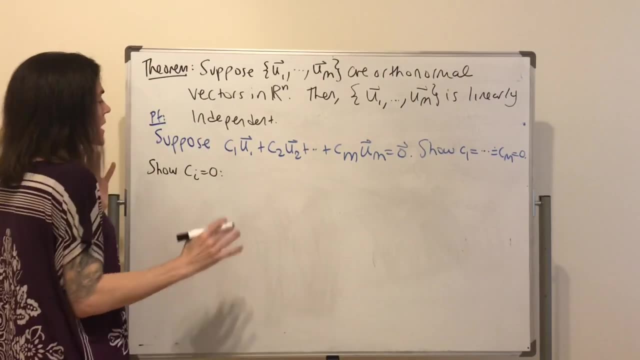 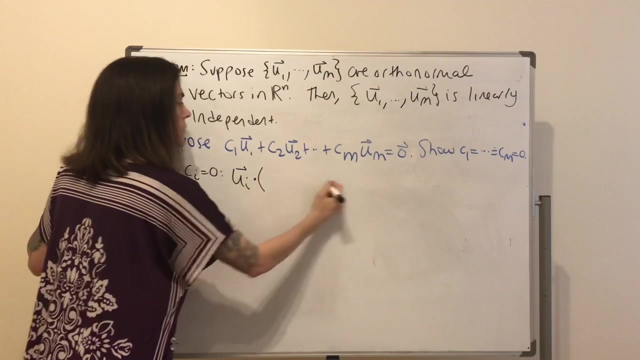 And I will show C, i is zero. in effect, then I have showed that all of this C, one to m, is all zero. Okay, so I'm gonna take this equation and just dot product U, i on each side. So if I take U, i dot this whole thing. 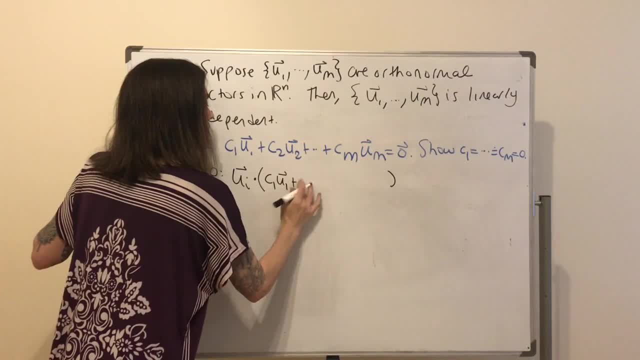 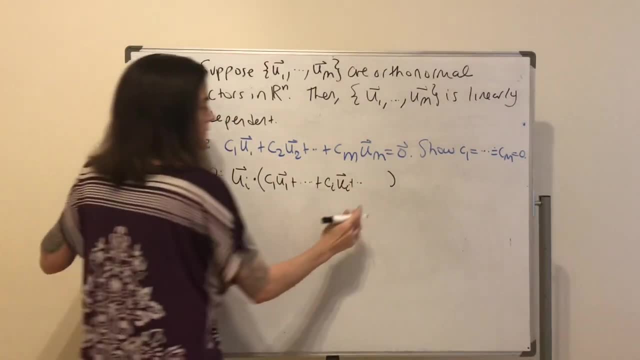 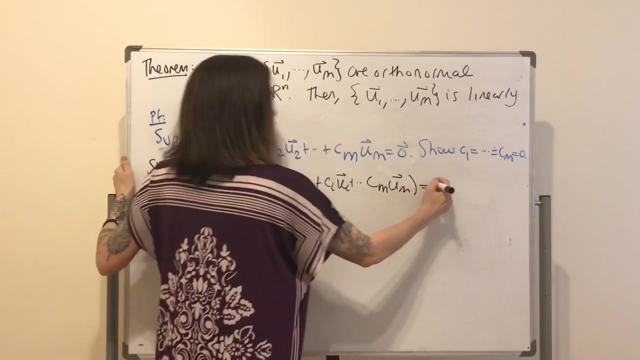 C one U one. Okay, this one I'm gonna include. there's some little C i, U, i in here, whatever that happens to be. And then the very last one is C m, U m, And this will be equal to well. I just take the dot product on this side. 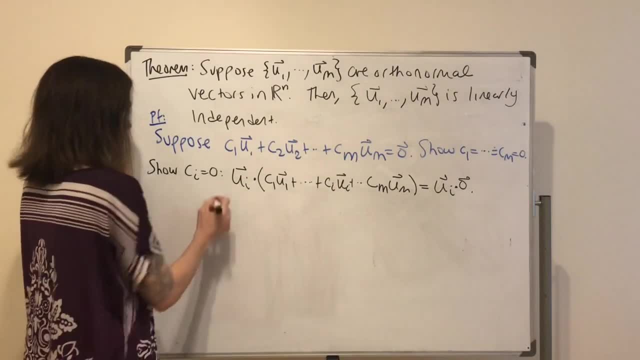 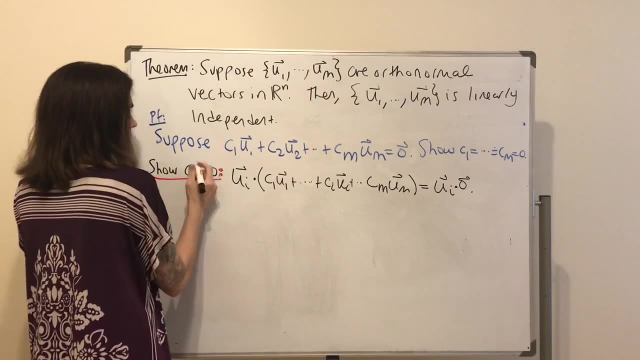 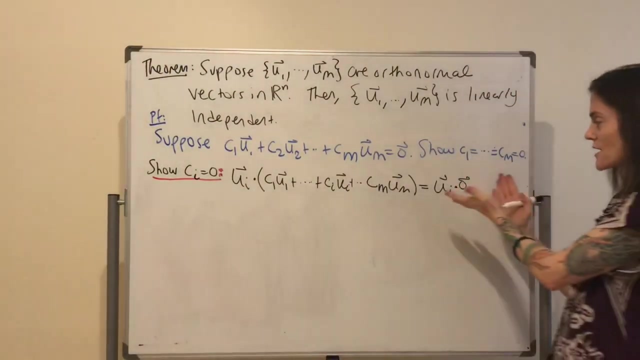 Okay, now we have to think that this is what maybe I will. this is not part of my equation. This is what I'm doing. Showing C: i is zero. Okay, very nice. First, let's start with the more straightforward side. 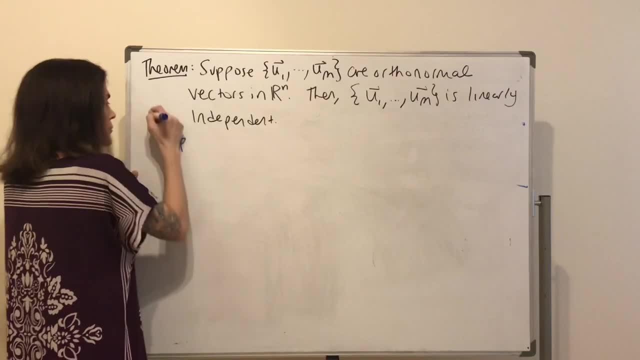 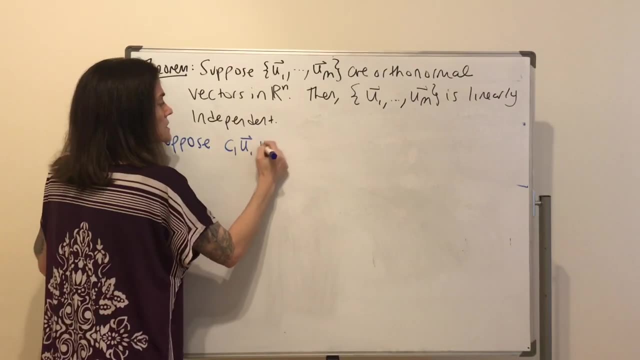 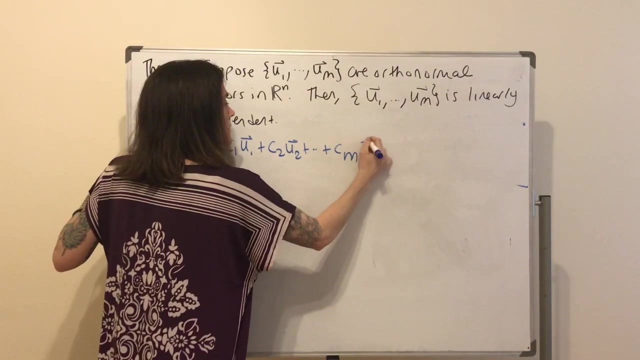 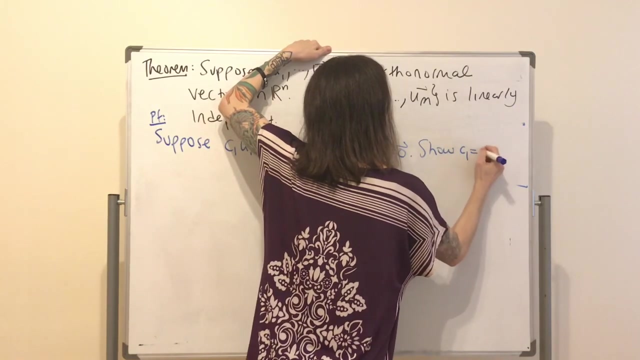 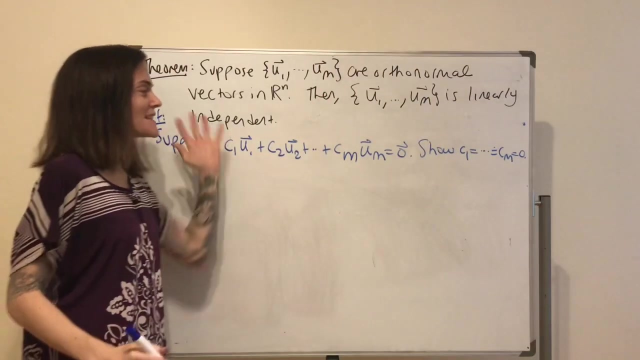 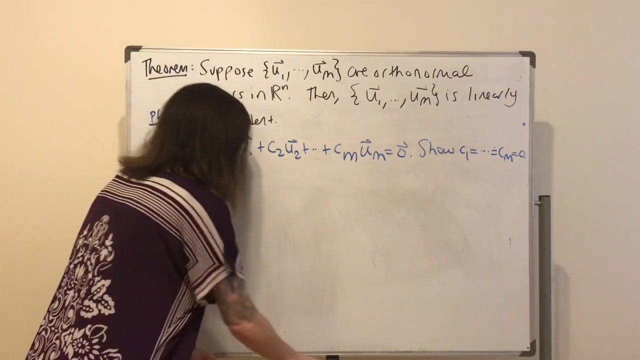 was if, then? and so this is how I will prove this. so suppose I have some linear relation among these vectors, and then I just need to show that all the CI's are zero- see zero- and this will prove that this collection is linearly independent. how do we do this? well, here's what I'm gonna do, so. 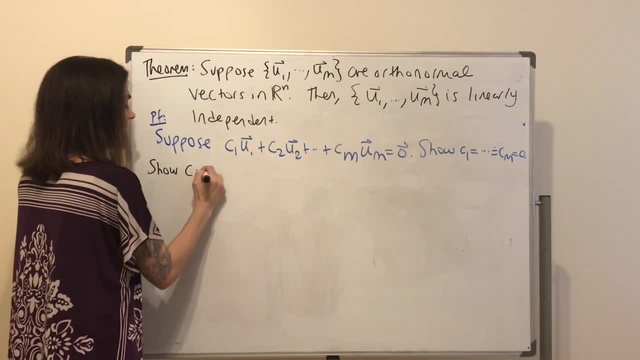 let's show you how to do this. so let's show you how to do this. so let's show you how to do this. so let's show: CI is zero and I'm working generally. let I be some number between 1 to M and I will show. 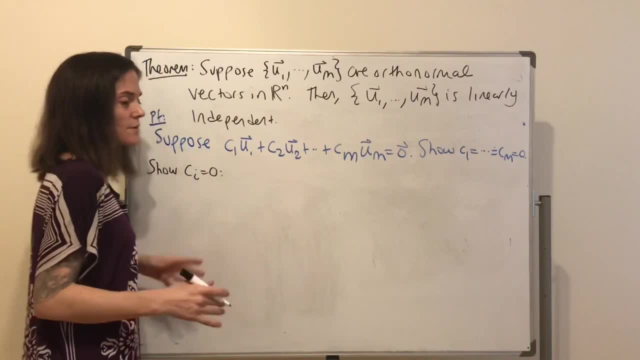 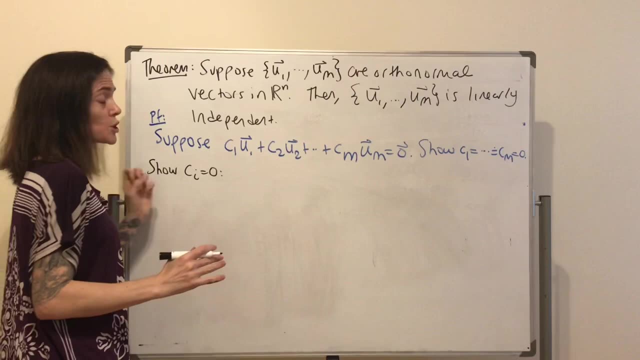 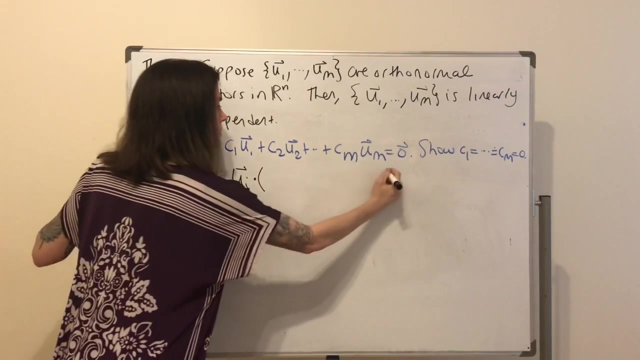 CI is 0 in effect then. then I have showed that all of this- see 1 to M- is all 0. okay, so I'm going to take this equation and just dot product UI on each side. so if I take UI, dot this whole thing: C 1 u 1. 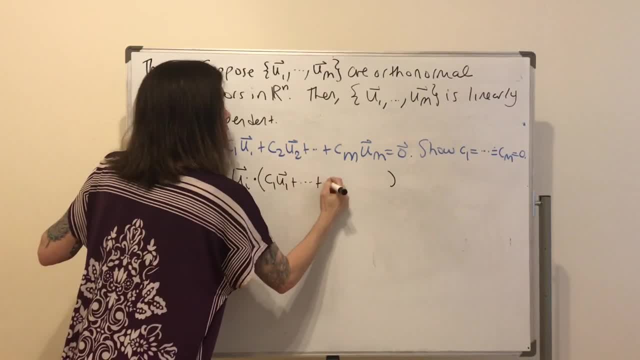 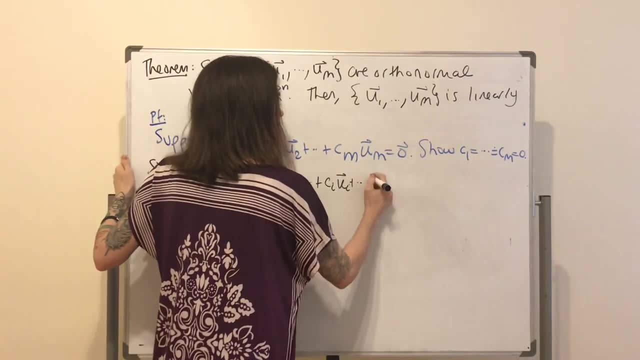 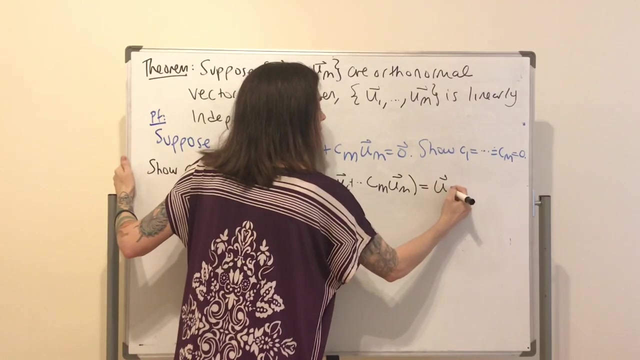 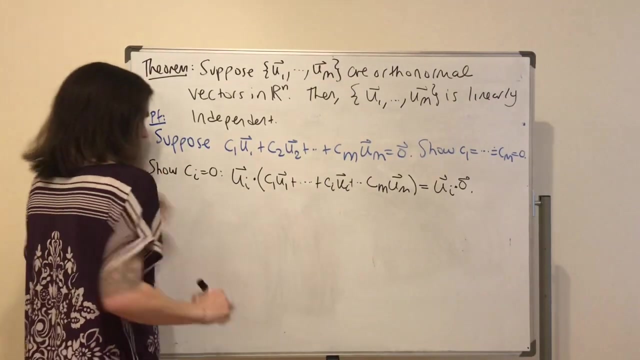 this one I'm going to include. there's some little CI UI in here, whatever that happens to be. and then the very last one is CM, UM, and this will be equal to well. I just take the dot product on this side. okay, now we have to think that this is what maybe I will. this is not part of my equation. this is. 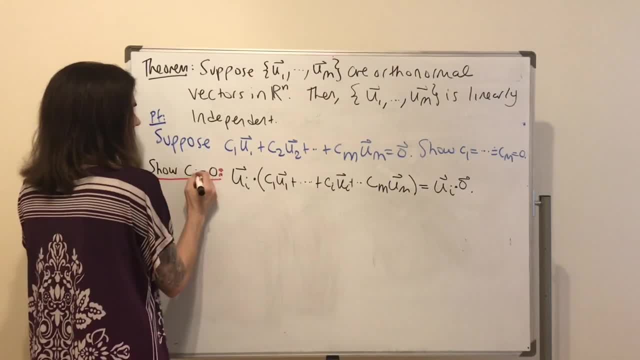 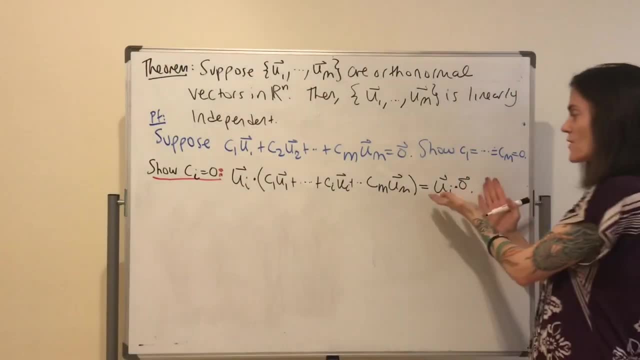 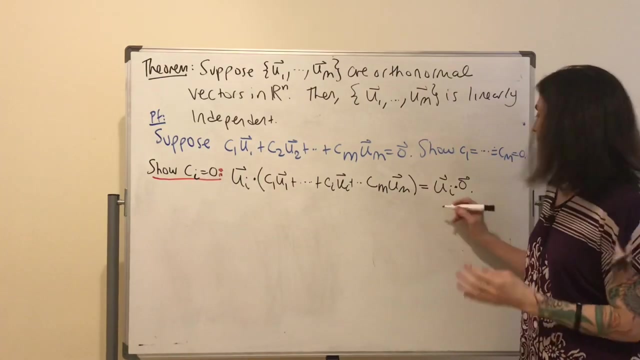 what I'm doing, showing, see I'm doing, is this? okay, let's see. and this is what I'm doing showing, see I'm? i is zero. okay, very nice. first, let's start with the more straightforward side, which is this side: you take any vector, you dot it with the zero vector, you get zero. okay, so this is zero. 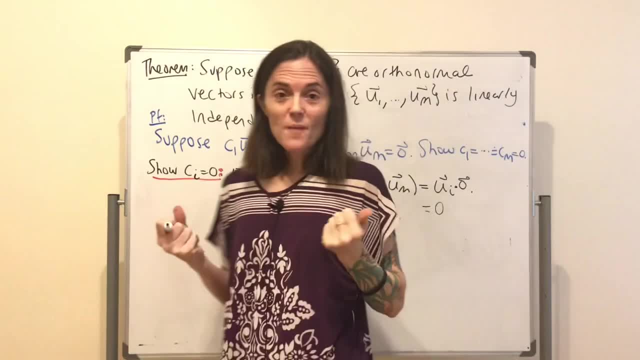 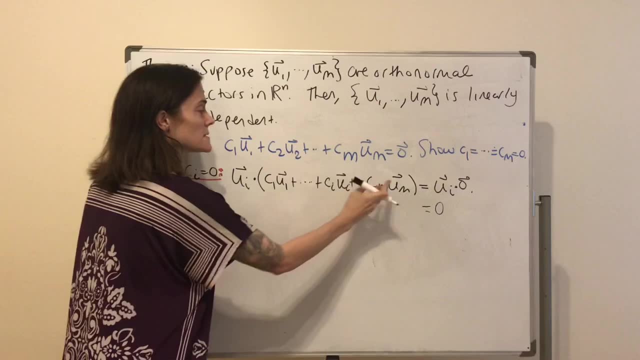 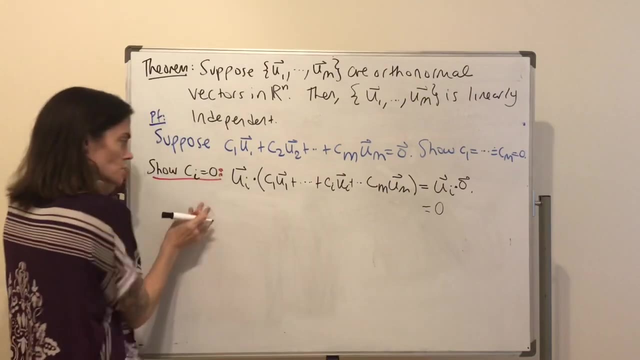 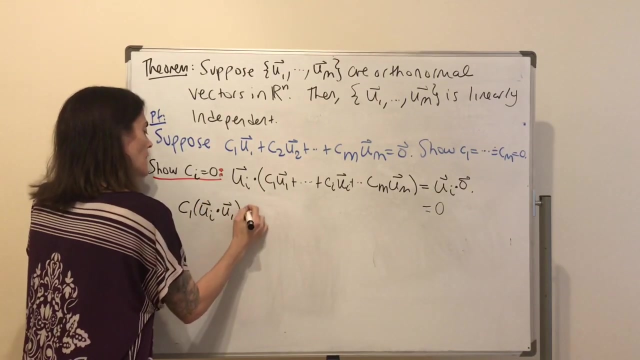 now let's do this side. one thing that we have is properties of dot product, which means i can distribute this across the sum and these constants i could pull in front of the dot, the dot product of the two vectors. so this first term will be c one u i dot u one, and then we have c one- two. 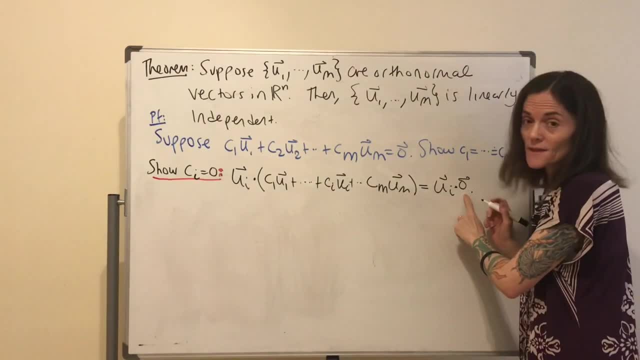 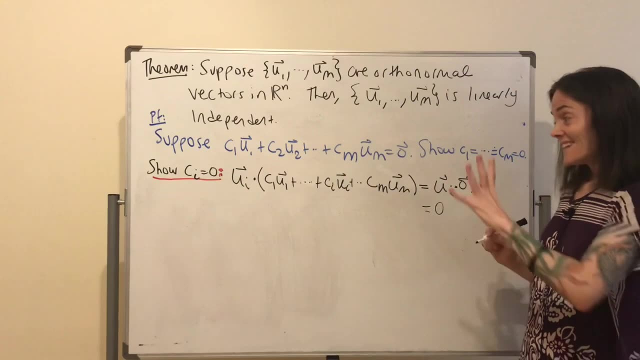 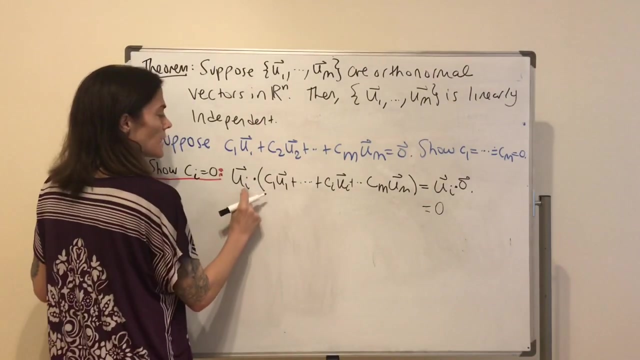 which is this side. You take any vector, you dot it with the zero vector, you get zero. Okay, So this is zero. Now let's do this side. One thing that we have is properties of dot product, which means I can distribute this across the sum. 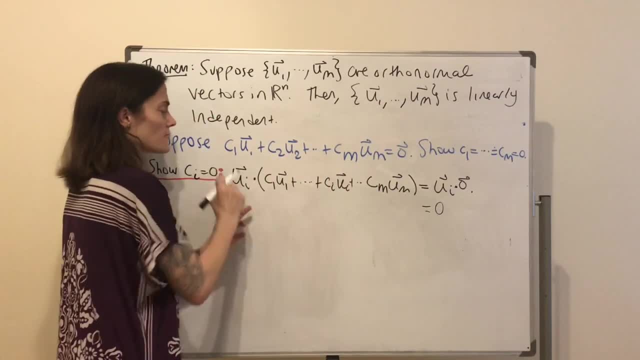 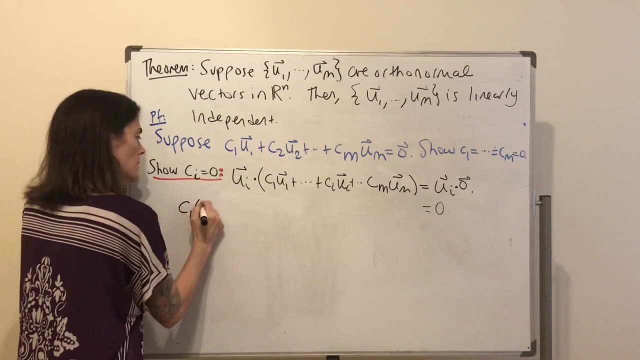 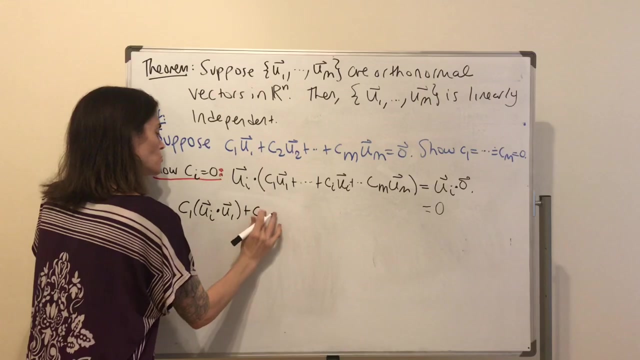 and these constants I could pull in front of the dot product of the two vectors. So this first term will be C one, U, i dot U one. And then we have C one, two, three, four, five, six, seven. 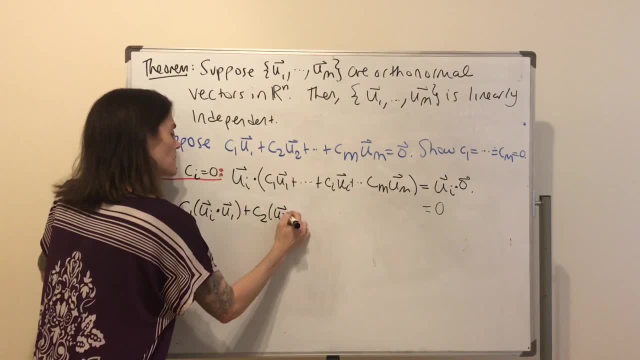 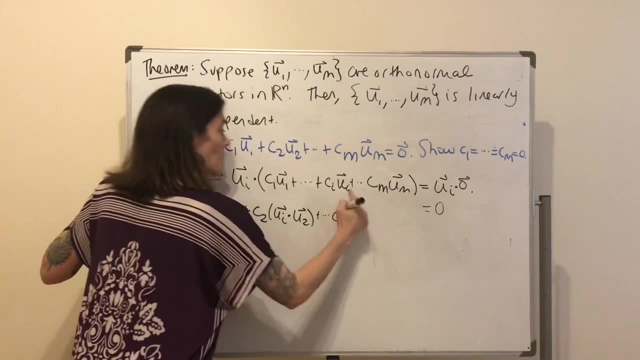 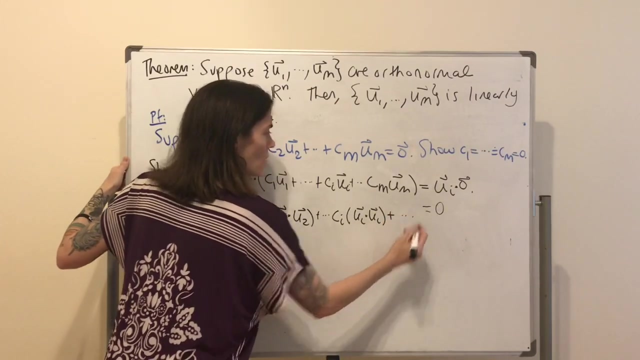 we have dot car e i dot u one U i dot u two would be the next one. Somewhere in here we have a C i u i dot u i, And then the very last one. uh, oh, I got to move my zero. 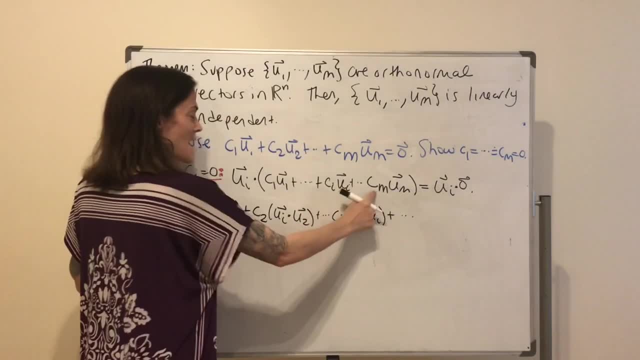 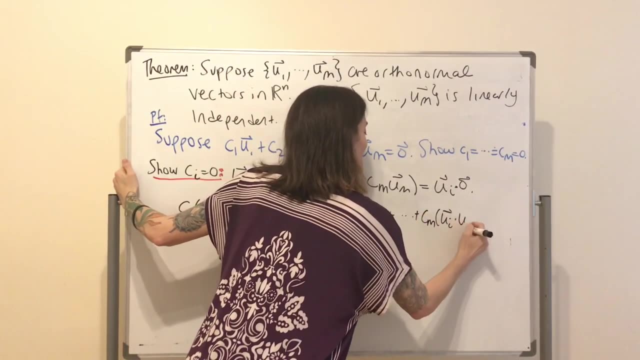 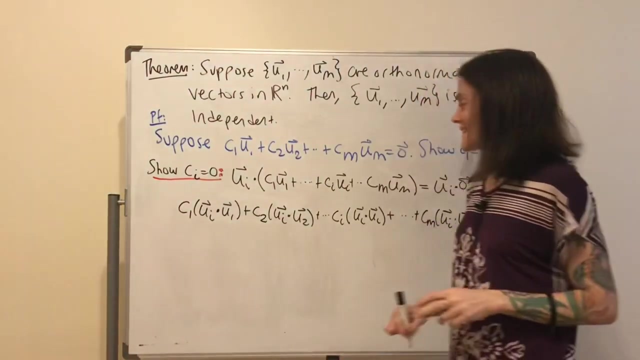 Let's put the last term. It's C m? u i dot u m. It doesn't C m? u i dot u m. This is just C m? u i dot u m, um, and this was zero. okay, maybe it looks complicated, except we're in really great shape because 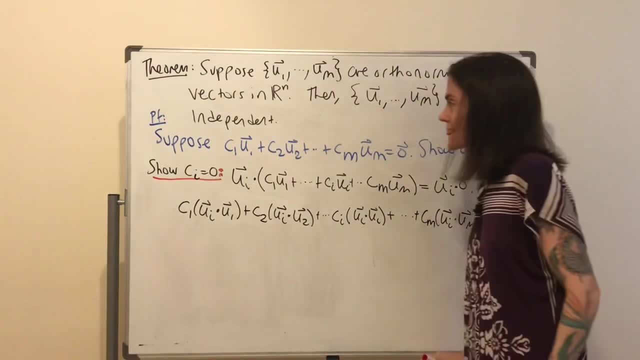 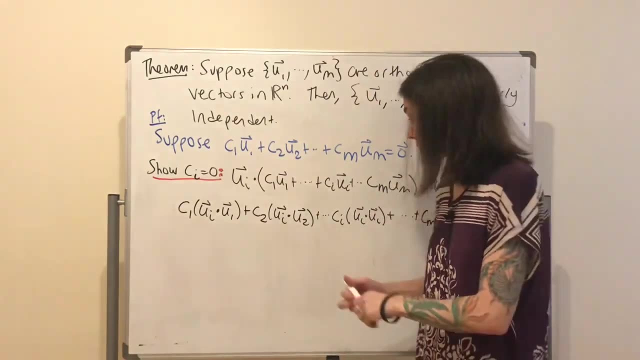 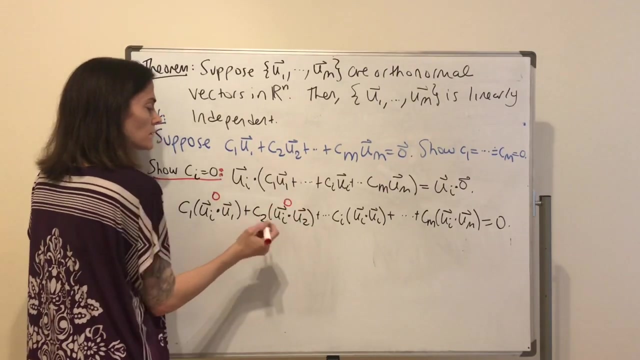 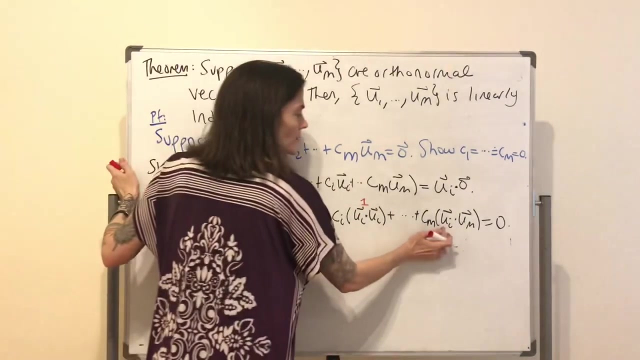 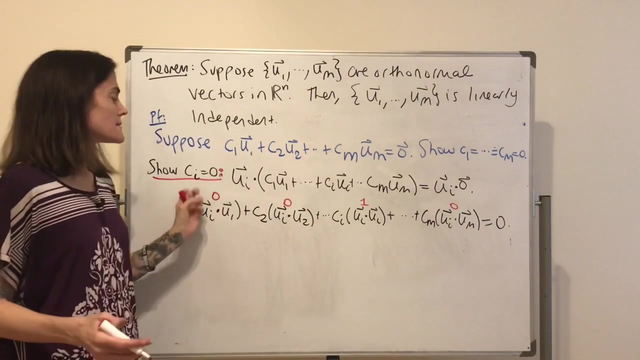 we are assuming that u1 to um or orthonormal, which means well, it means ui dot u1 is zero, this is zero. ui dot u2 is zero, okay. and then here this one: ui dot ui is one, okay. all the way out to ui dot um- zero. so you see, these are orthonormal, which means whatever i is when i dot ui with any. 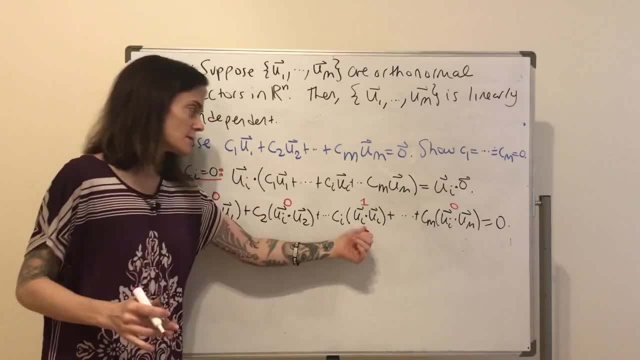 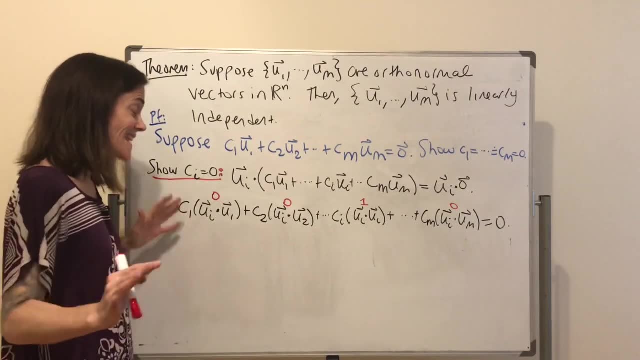 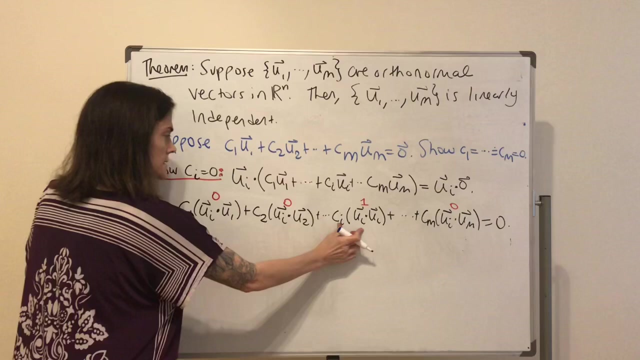 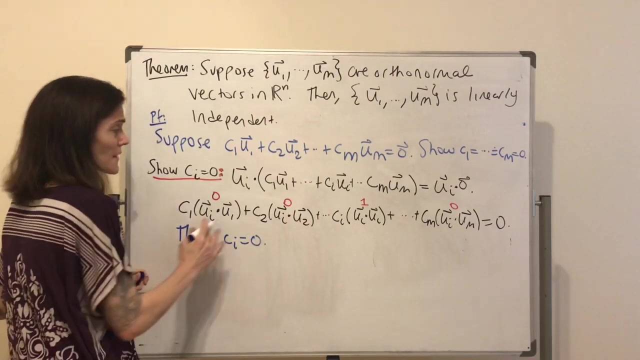 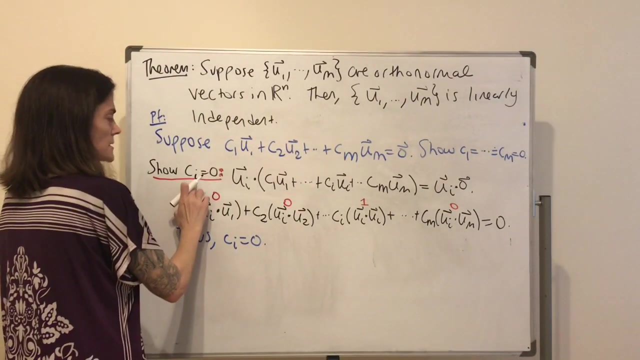 other of these vectors besides ui, this one, i get zero. okay, so what does this equation sort of actually say? every single term is zero, except this one, and this says: CI is zero. that's, CI is zero. that's what this equation says, and so we can conclude. I did this for one, but it's general, so we 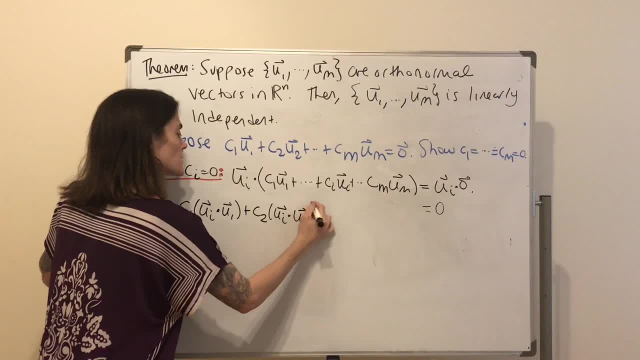 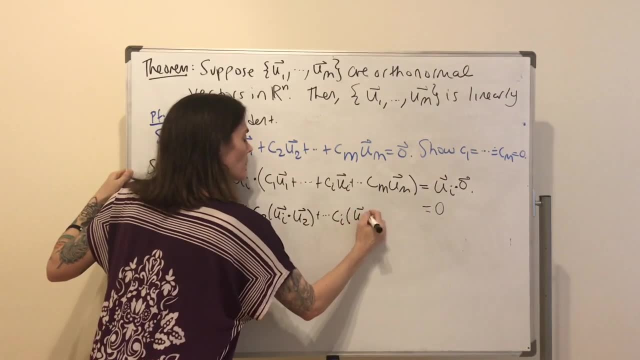 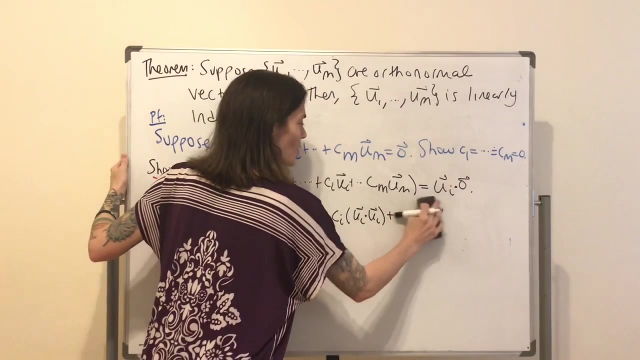 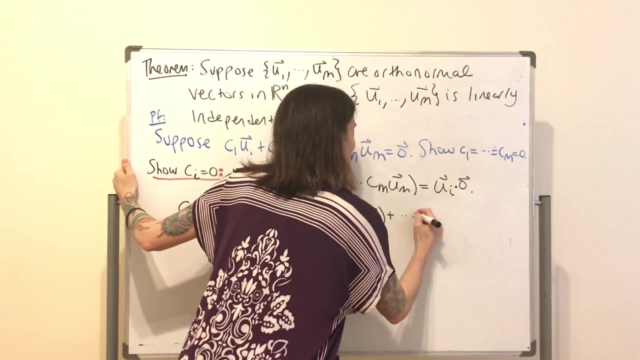 u i dot u two would be the next one. somewhere in here we have a c? i? u i dot u i. and then the very last one. uh, oh, i gotta move my zero. let's put the last term. it's c m? u i dot dot u m. so this is c m? u i dot u m, and this was zero. 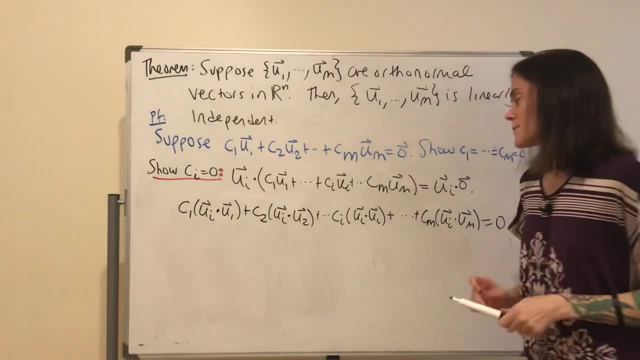 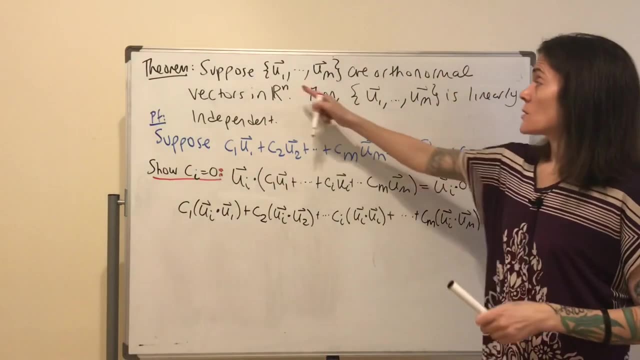 okay, maybe it looks complicated, except we're in really great shape, because if u1 is considered normal in case that internals is included within the movie, that means u1 dot, u1 is zero and this is zero. okay. so then we're going to go think about what. 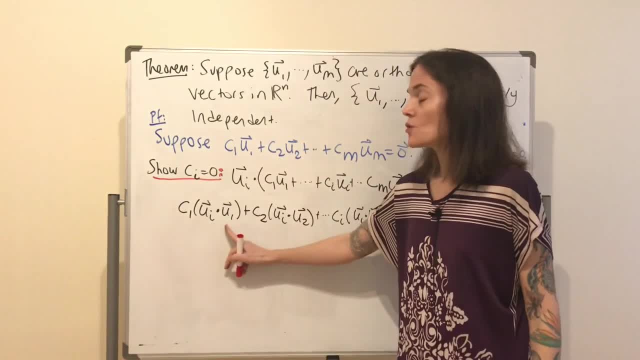 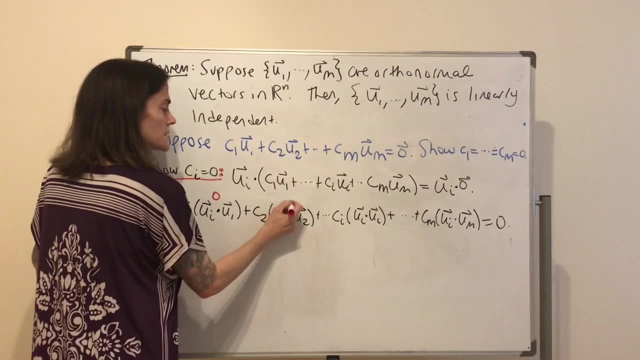 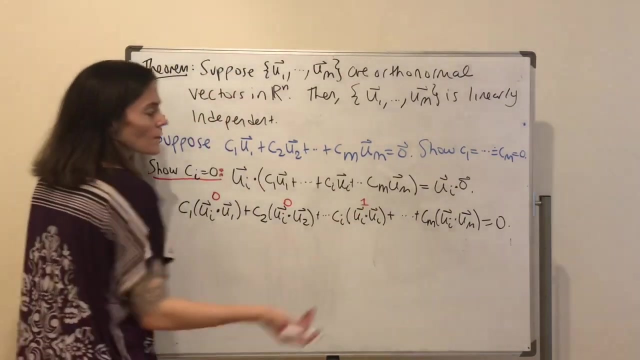 that means okay, because we are assuming that u1 to um orthanormal, which means well, it means ui dot u1 is zero, this is zero. ui dot u2 is zero, okay. and then here this one ui dot ui is one, okay, all the way out to when we are figuring the uium, because that means ui dot u1 is 1, because it is empty zero. so after this value, n will answer as uium is zero. 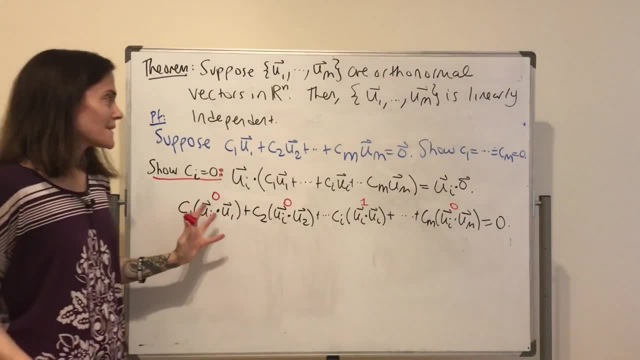 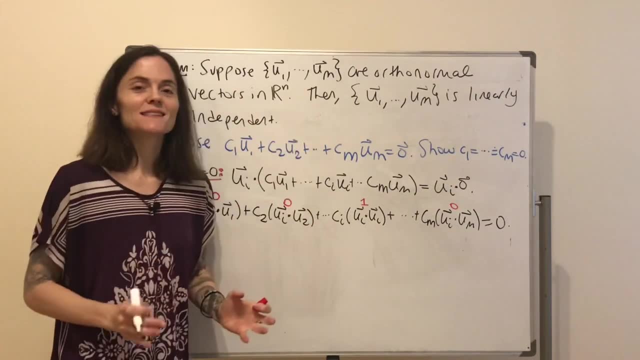 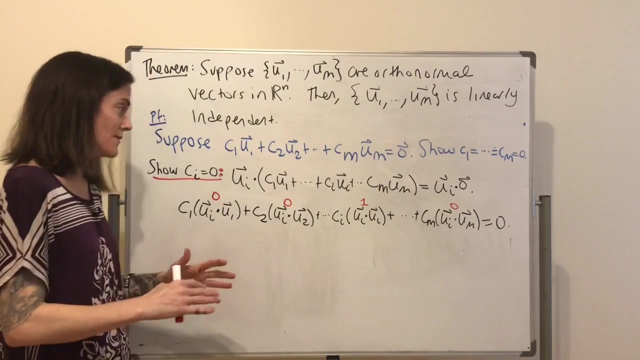 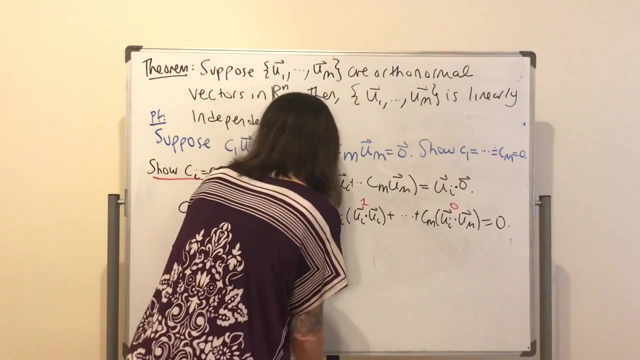 m zero. so you see, these are orthonormal, which means, whatever i is, when i dot u i with any other of these vectors besides u i this one, i get zero. okay, so what does this equation sort of actually say? every single term is zero, except this one, and this says: 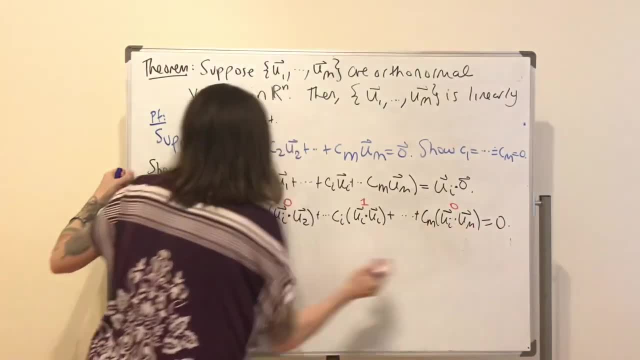 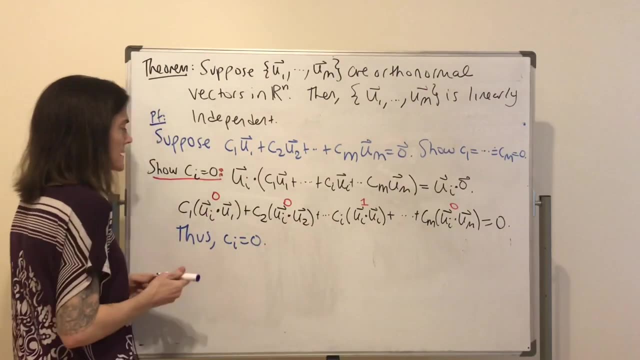 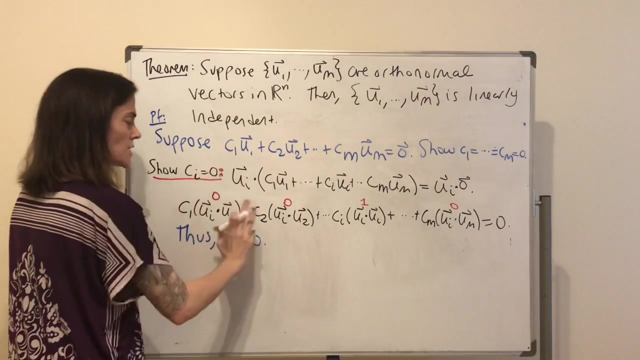 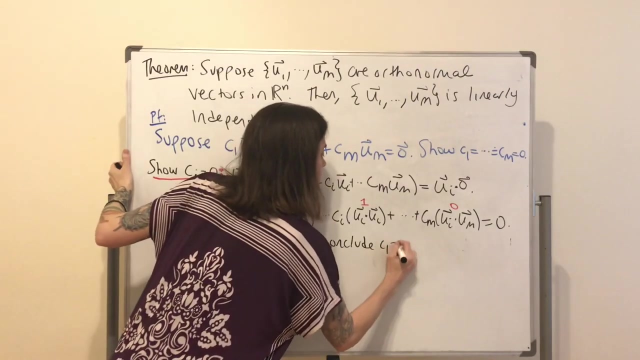 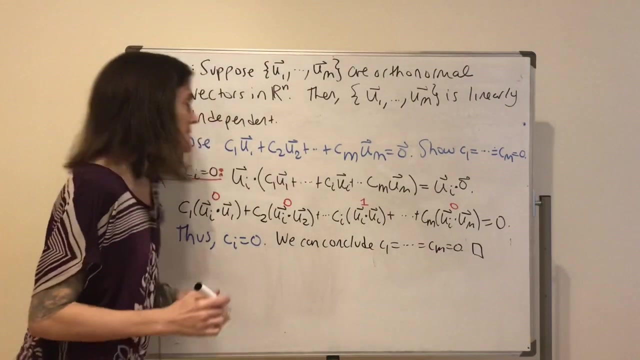 c i is zero. that's: c i is zero. that's what this equation says, and so we can conclude. i did this for one, but it's general, so we can conclude that all of them are from the similar argument and this shows the vectors are are literally independent. now i'll make one comment and then we will. i will define or the. 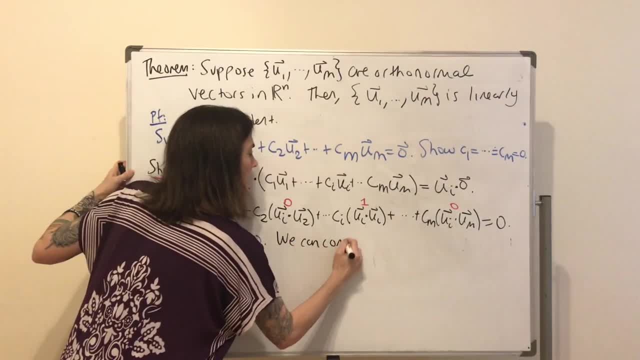 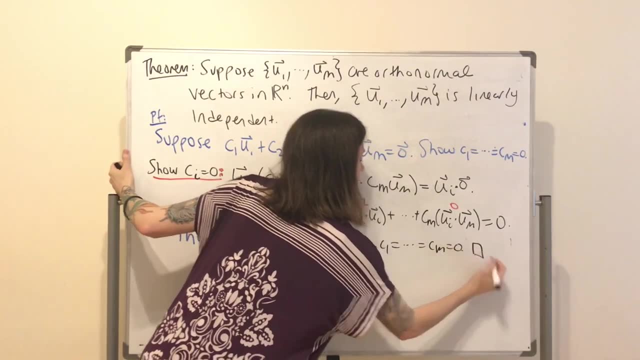 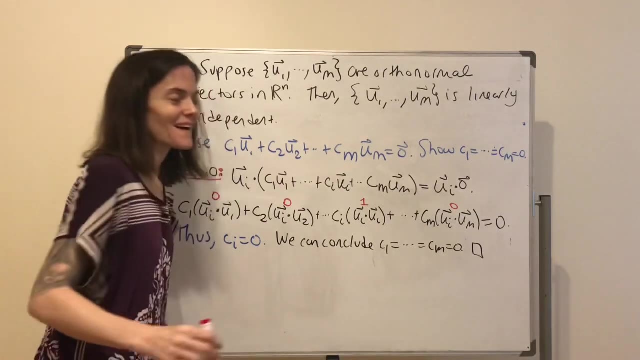 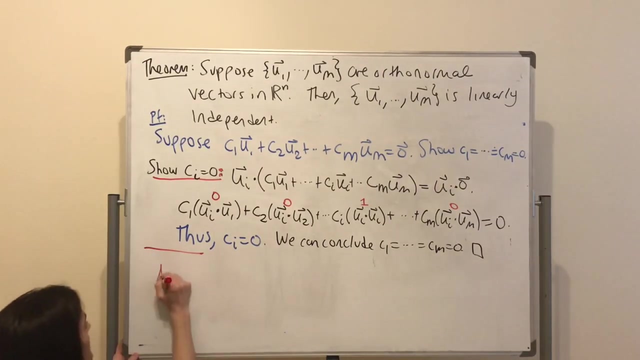 can conclude, but all of them are from a similar argument and this shows the vectors are literally independent. now I'll make one comment and then we will. I will define or the normal basis and this is the. so I'm done without proof. okay, my other comment is that I only really needed here. 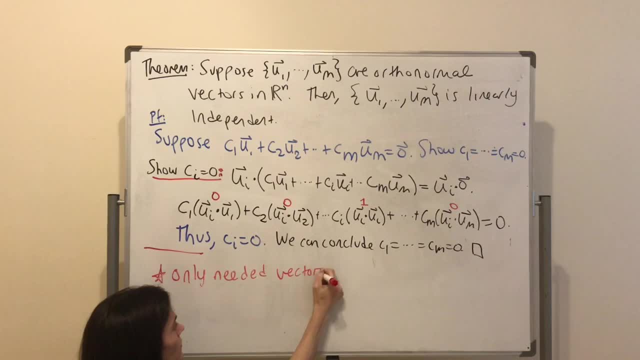 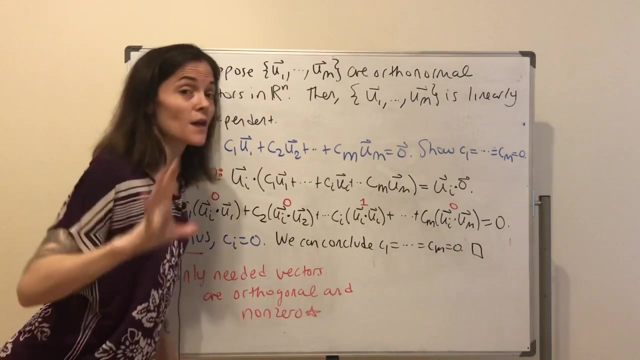 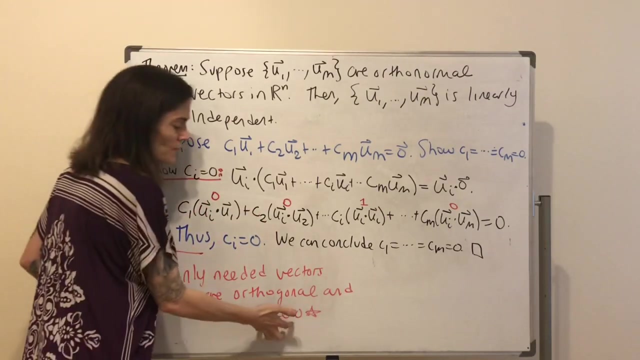 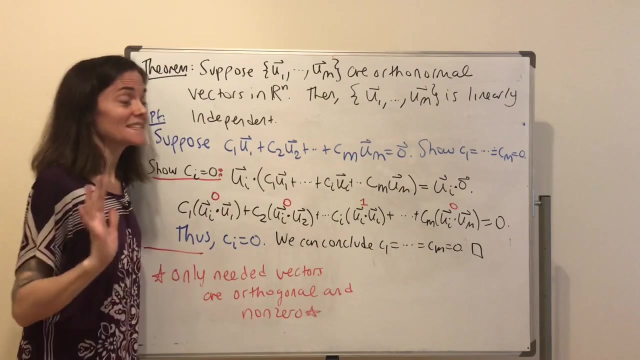 that the vent were orthogonal and nonzero. so if you have a collection of vectors that are all orthogonal so you can remove the unit part just orthogonal, then they'll be linearly independent, provided you don't have the zero vector and the set zero is orthogonal to every vector but zero is never a part of any linearly. 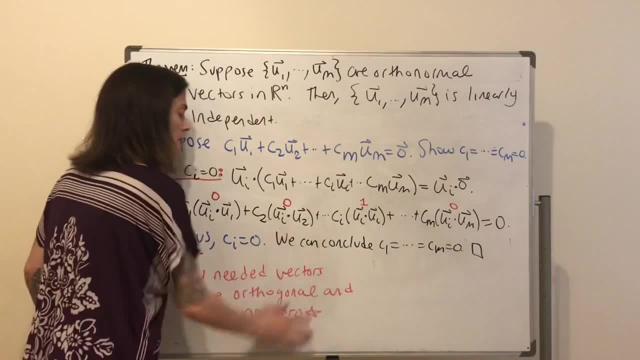 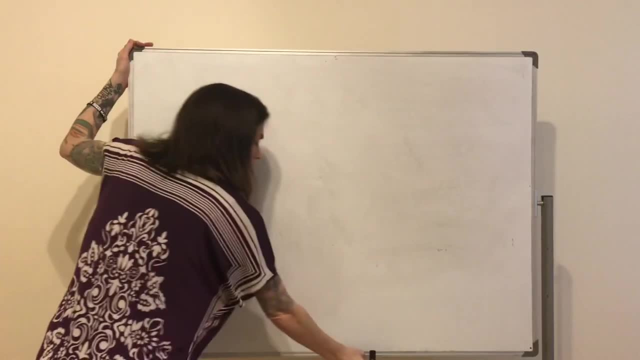 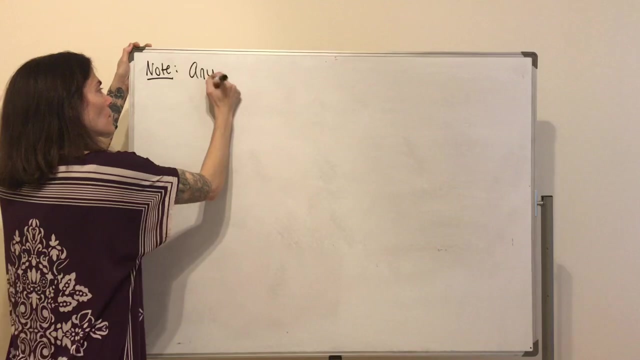 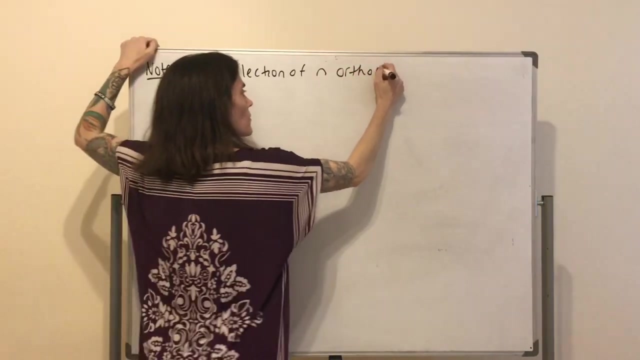 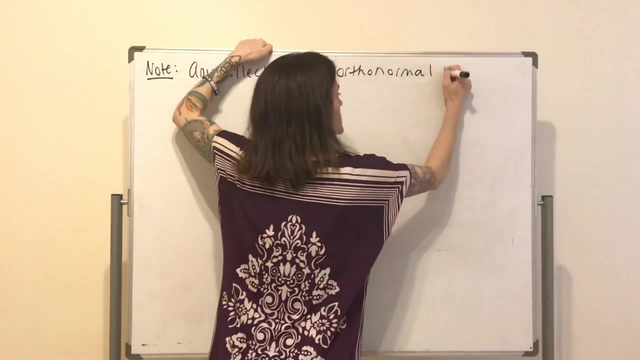 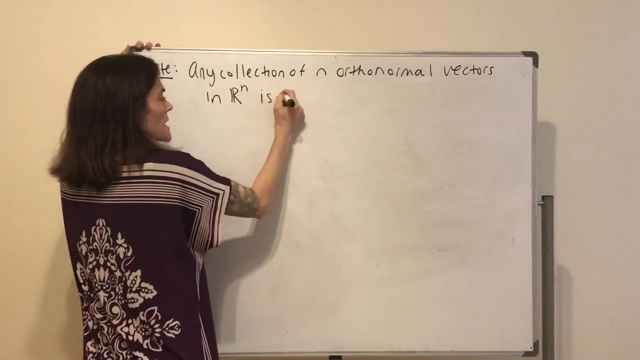 independent collection of vectors. okay, this is really just a comment, because what we're really interested in is orthonormal collections of vectors. one thing that we get from this is is any collection of an orthonormal vector vectors in Rn is a basis for Rn. 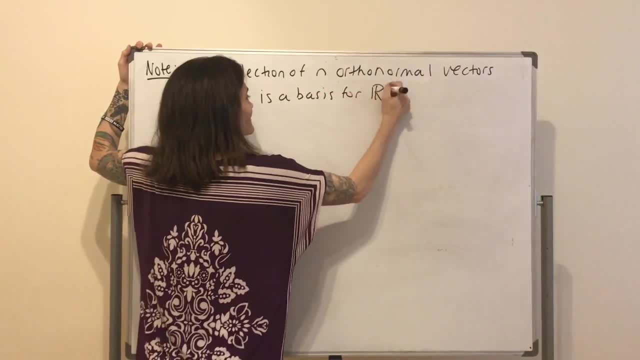 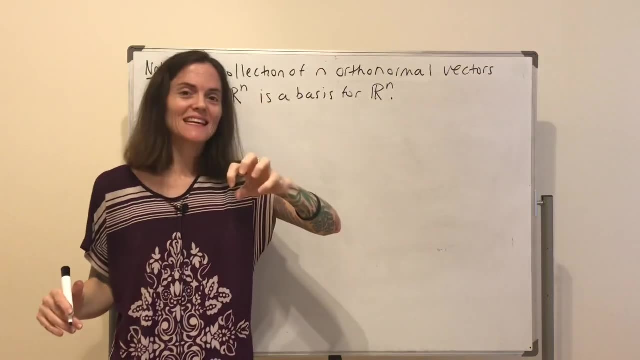 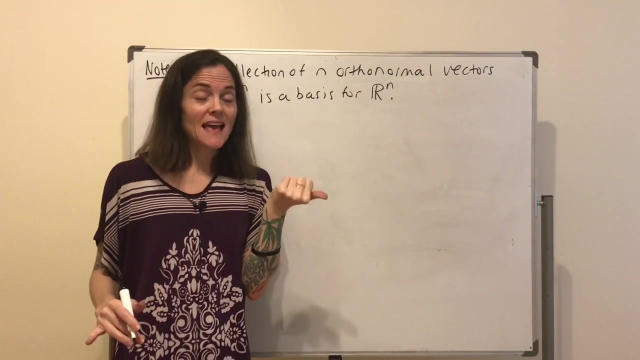 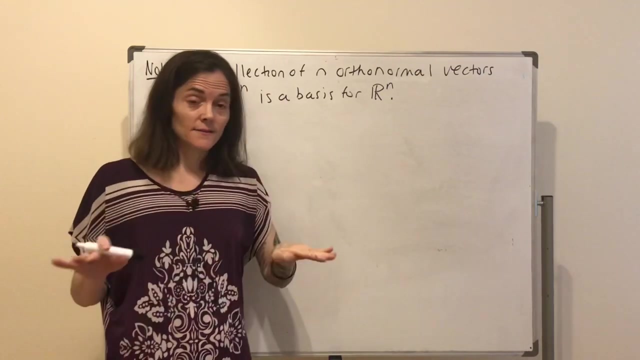 because we have N vectors. that's how many we need in a basis for Rn and what we just proved is which is just life, Because they're orthonormal. this collection must be linearly independent. So anytime you have a collection of n orthonormal vectors- n or n- you have a basis. 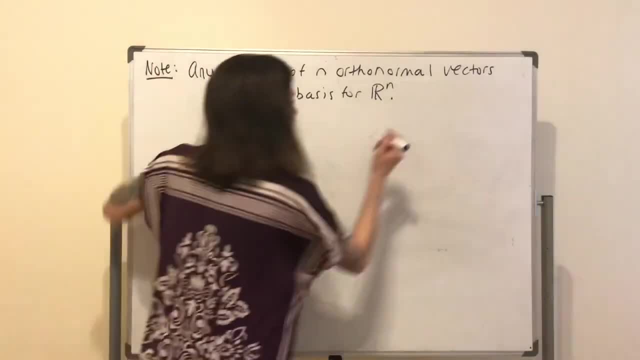 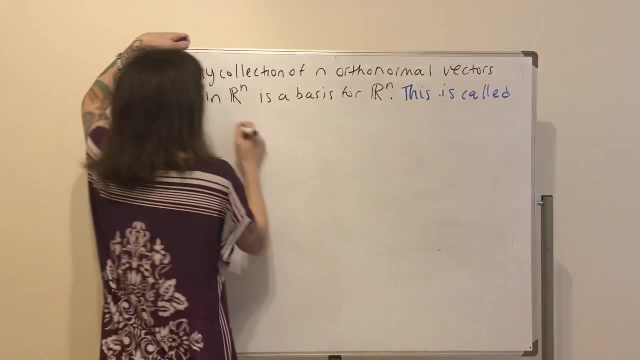 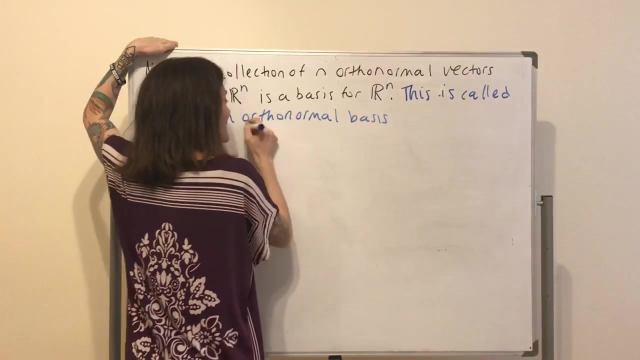 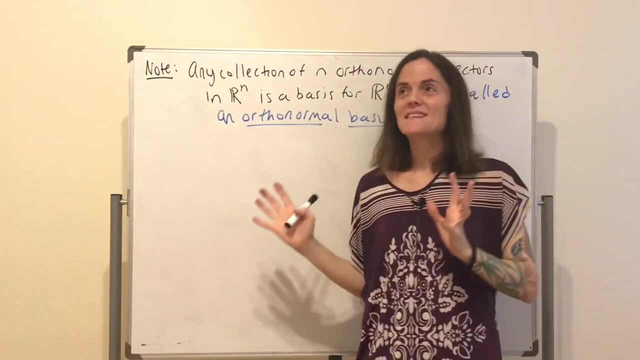 And it has a name And this is called an orthonormal basis. Maybe this part shouldn't be a surprise to you. Okay now, these are very nice orthonormal bases. We are going to be working with orthonormal- that concept in the next couple of sections. 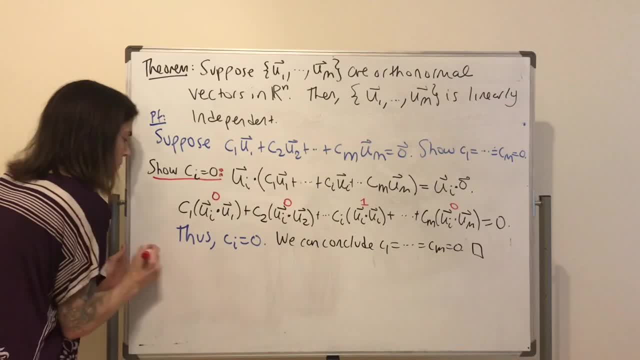 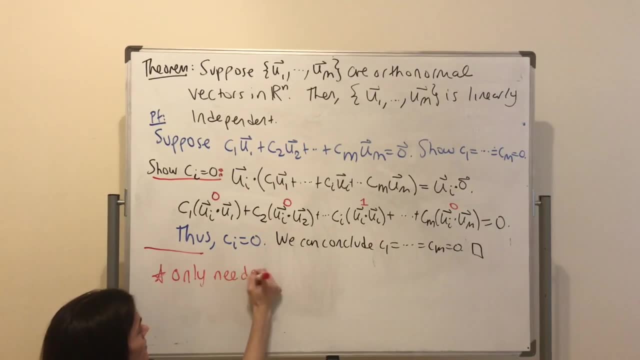 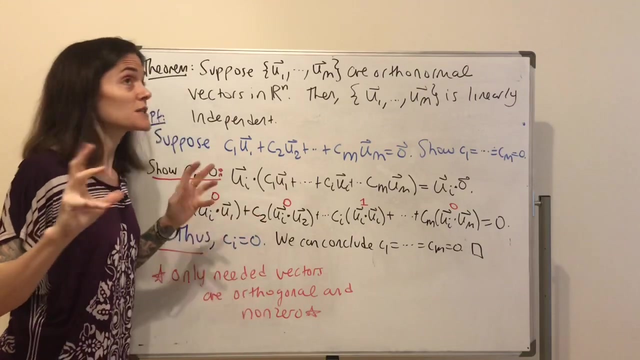 normal basis and this is the. so i'm done with that proof. okay, my other comment is that i only really needed here that the vectors were orthogonal and non-zero. so if you have a collection of vectors that are all orthogonal, so you can remove the unit part, just orthogonal. 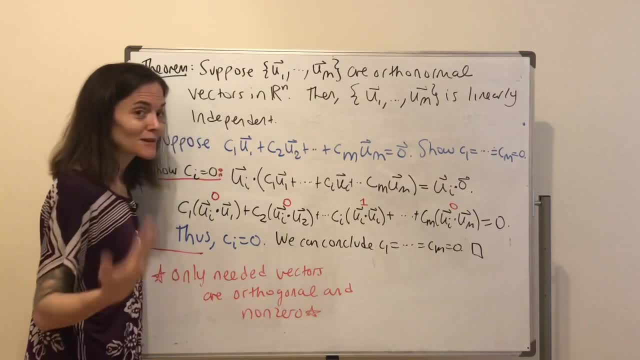 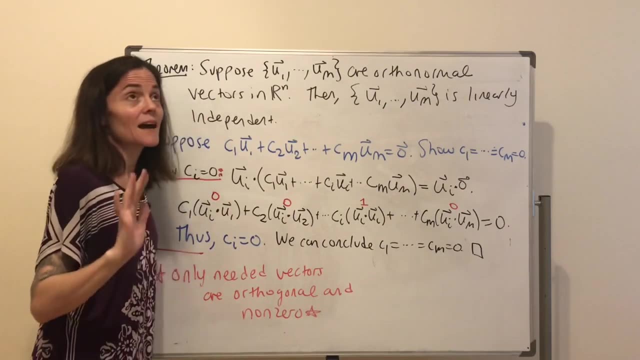 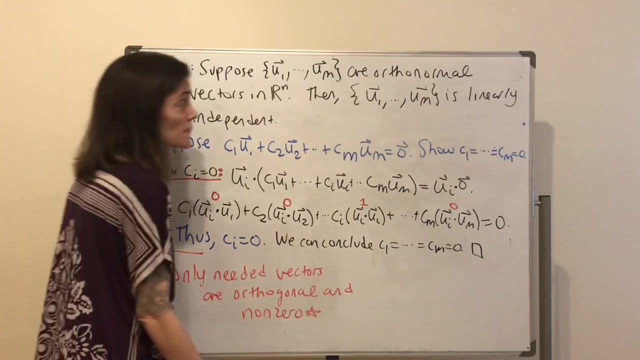 then they'll be linearly independent, provided you don't have the zero vector and the set zero is orthogonal to every vector, but zero is never a part of any linearly independent collection of vectors. okay, this is really just a comment, because what we're really interested in is orthonormal. 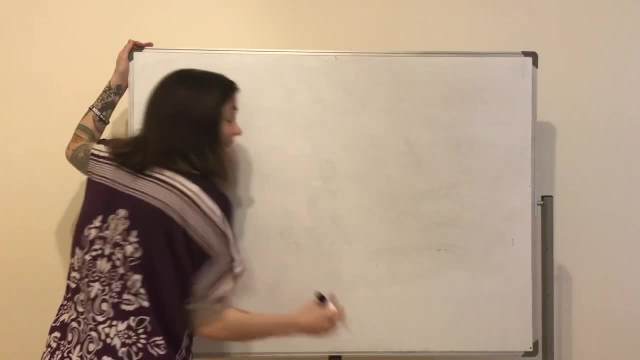 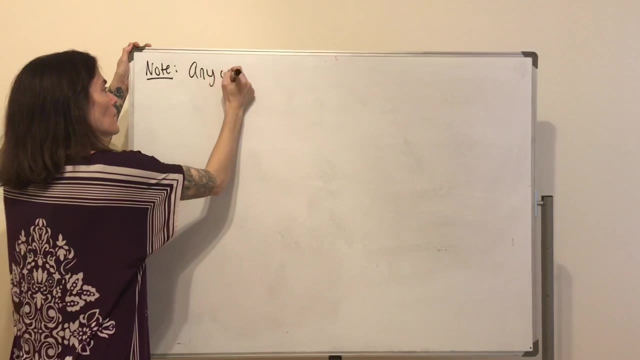 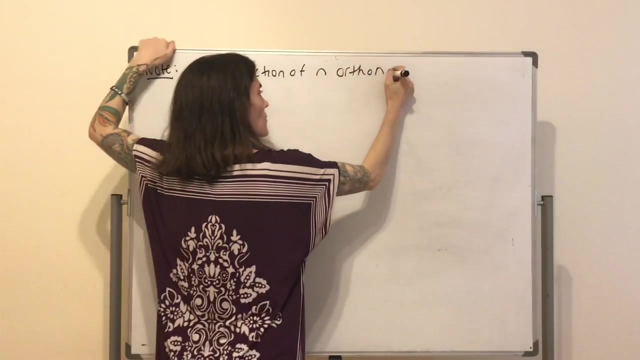 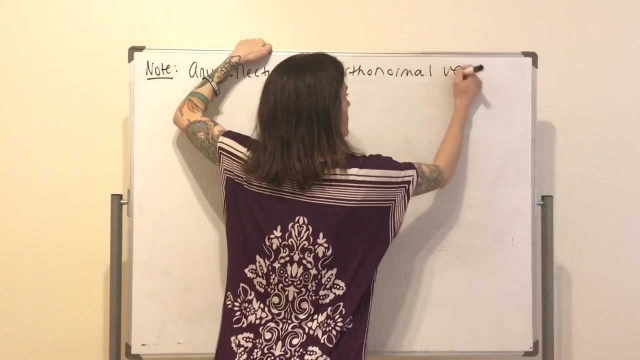 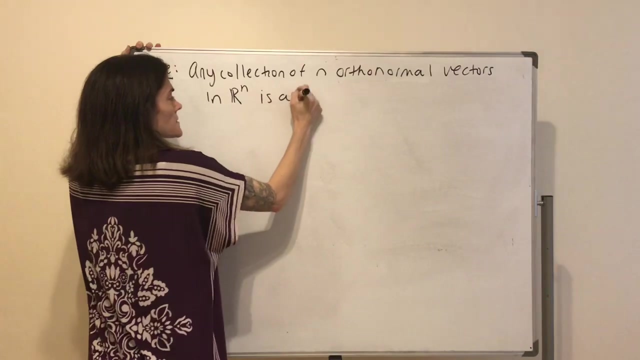 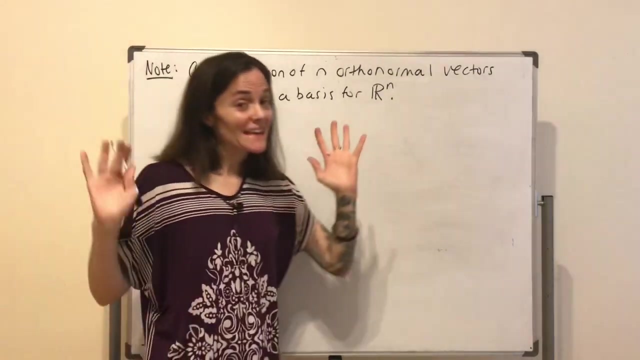 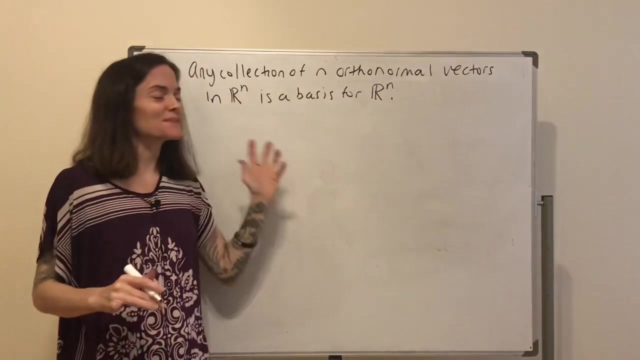 collections of vectors. one thing that we get from this is: is any collection of n orthonormal oh vectors in rn is a basis for rn, because we have n vectors. that's how many we need in a basis for rn and what we just proved is because they're orthonormal, this collection must be linearly independent. so anytime you have a 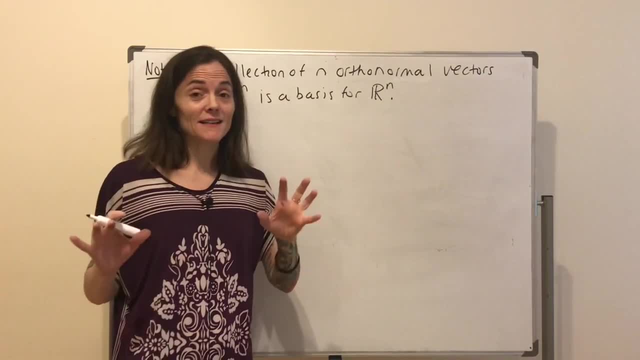 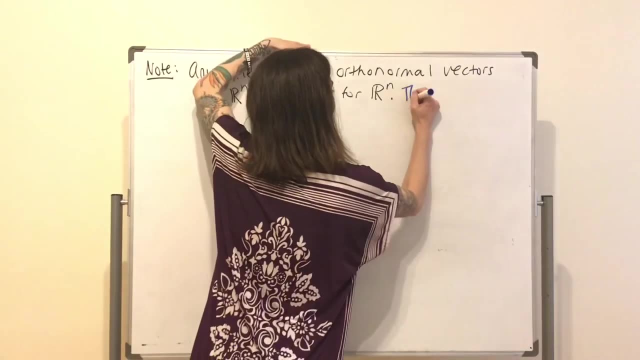 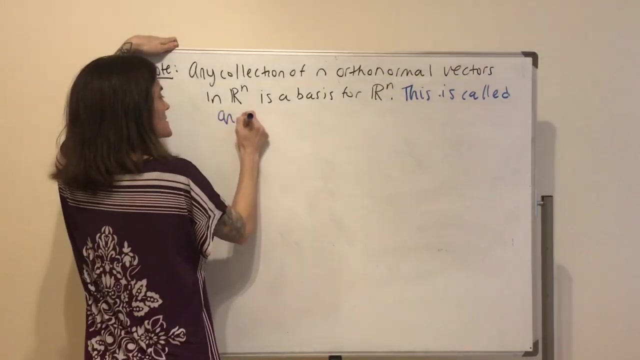 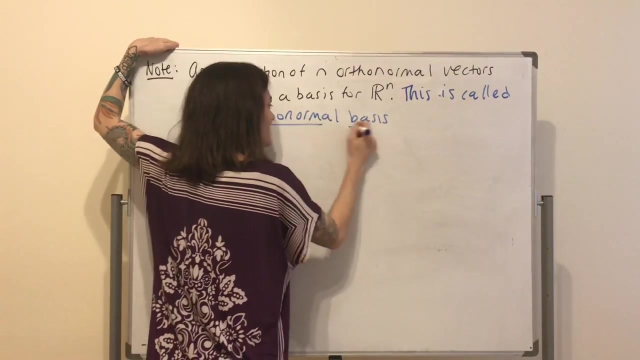 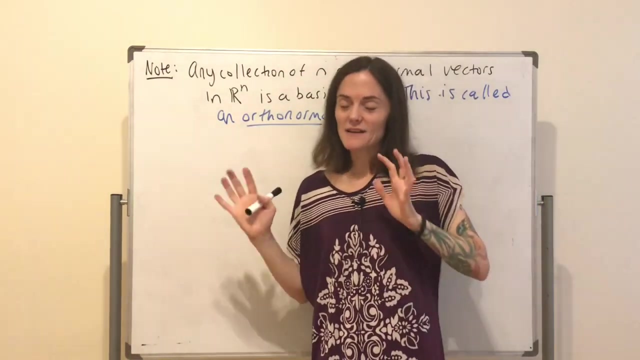 collection of n orthonormal vectors in rn. you have a basis and it has a name and this is called an orthonormal basis. maybe this part shouldn't be a surprise to you. okay now, these are very nice orthonormal bases. we are going to be working with orthonormal that. 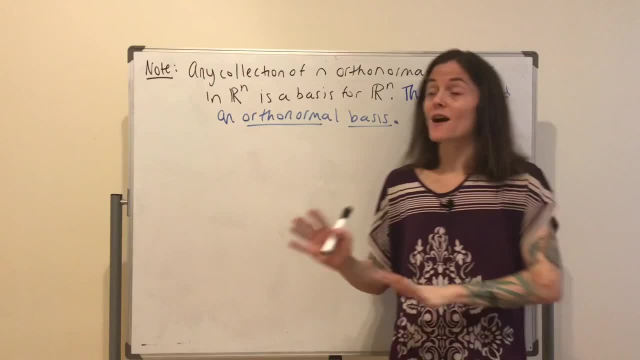 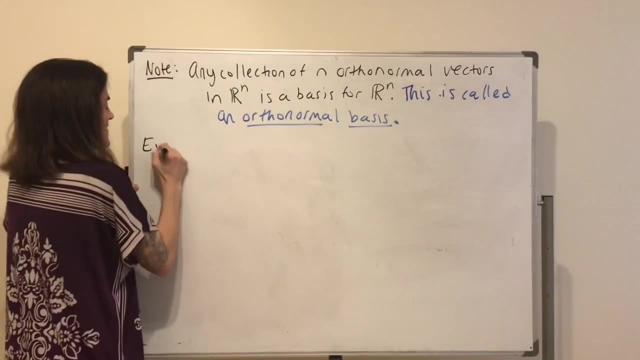 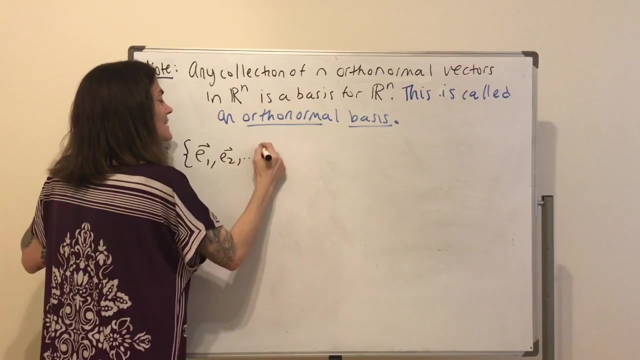 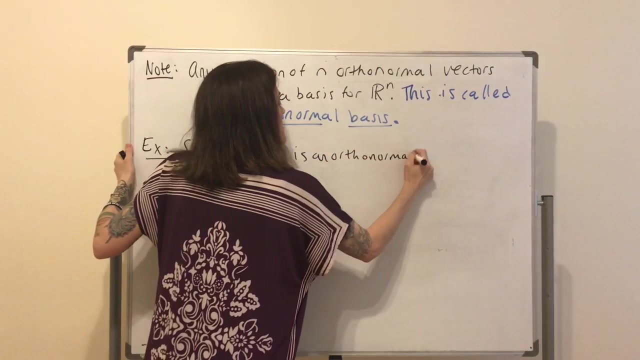 concept. in the next couple of sections, orthonormal bases are actually going to come to be more paced. are the nice bases that we like? well, for instance ah, e1. so, for example, building on what I discussed earlier, this e1, e2 to e? n, this is an orthonormal basis for. 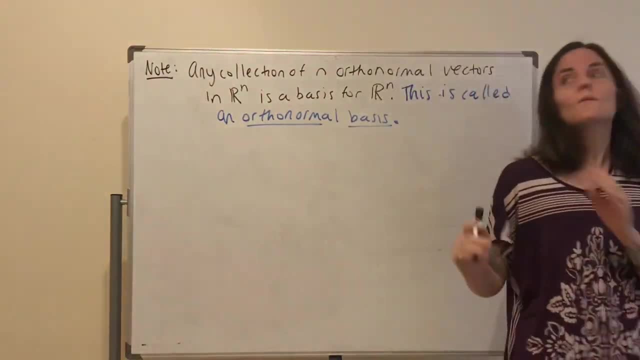 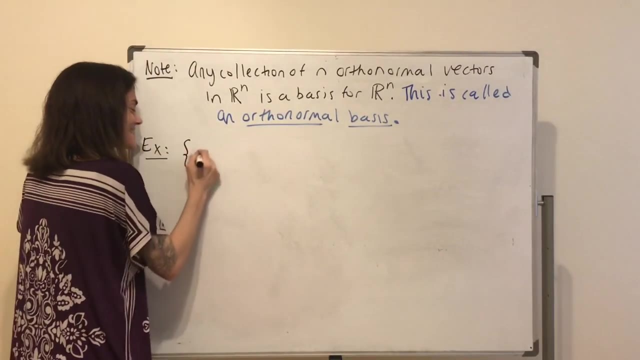 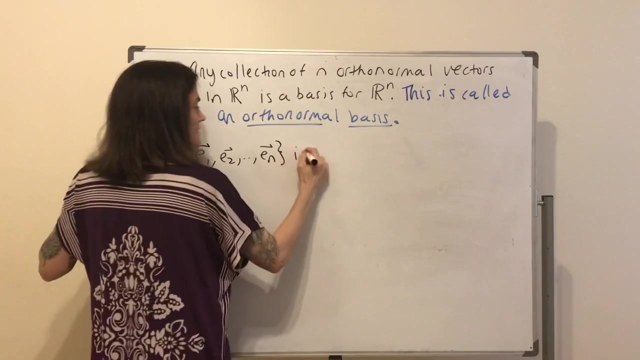 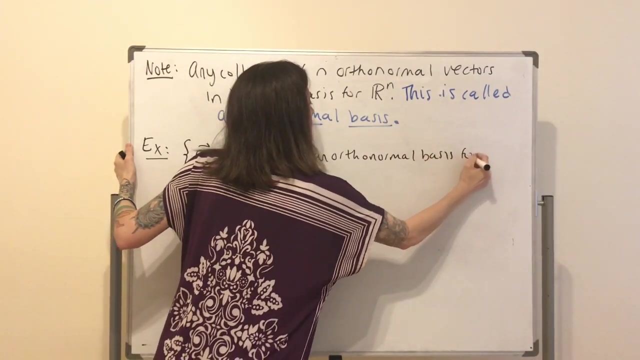 Orthonormal bases are the nice bases that we like Well, for instance, E1.. So, for example, building on what I discussed earlier, this E1, E2, to En, this is an orthonormal basis for Rn. 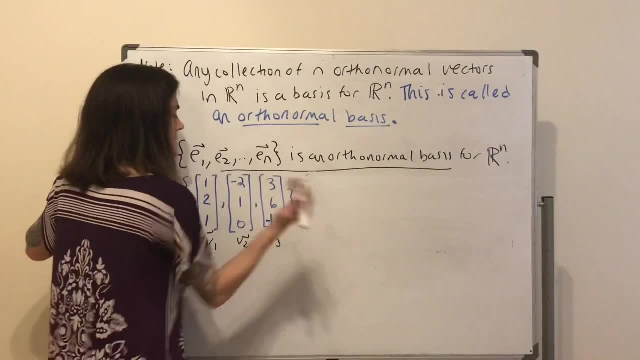 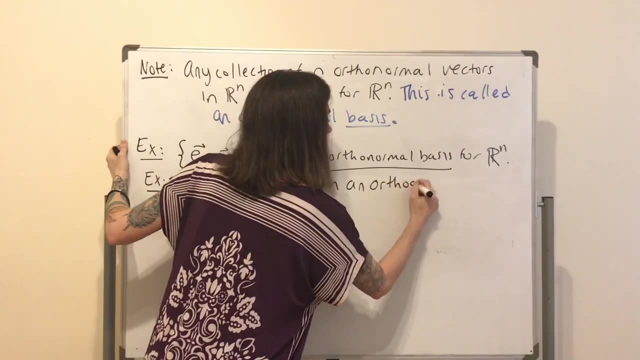 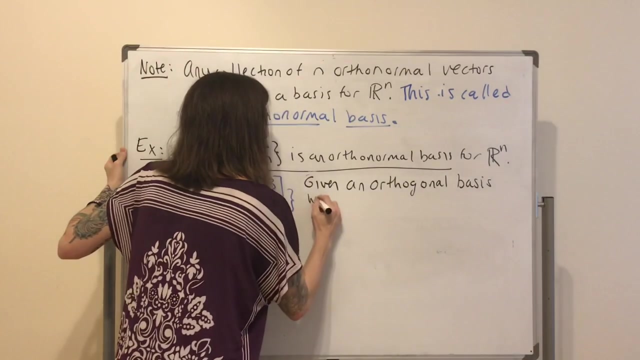 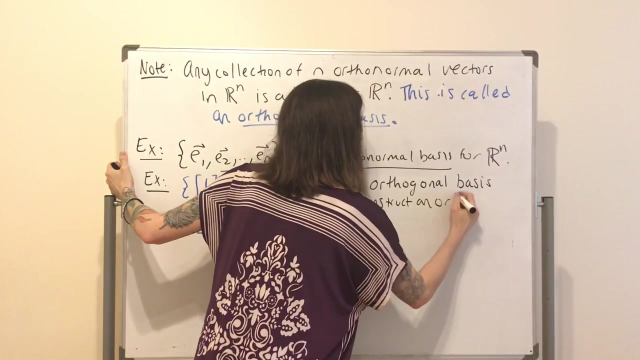 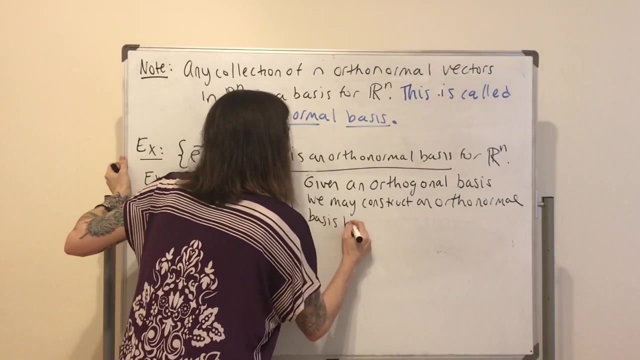 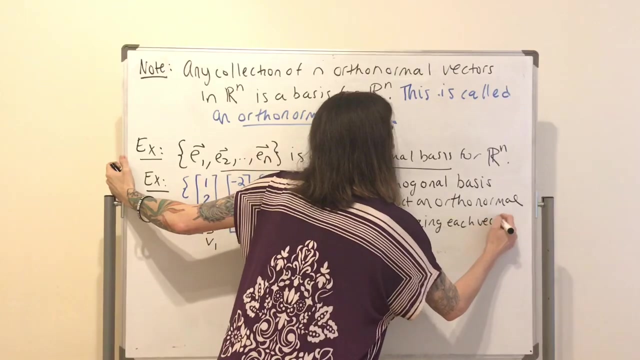 Now let's do another example. So what is this example going to be about? Given a or an- I should say- orthogonal basis, we may construct an orthonormal basis by normalizing each vector. Now, what does this mean? 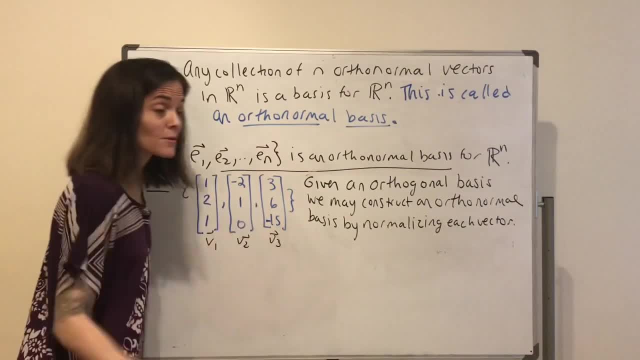 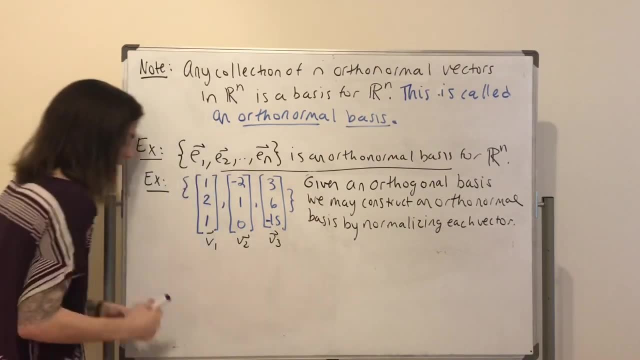 Well, here I have V1, V2, V3, they're in R3, I have the right number. None of them are zero, If I can show, Oh, that if I dot product, then let's check, Let's check. 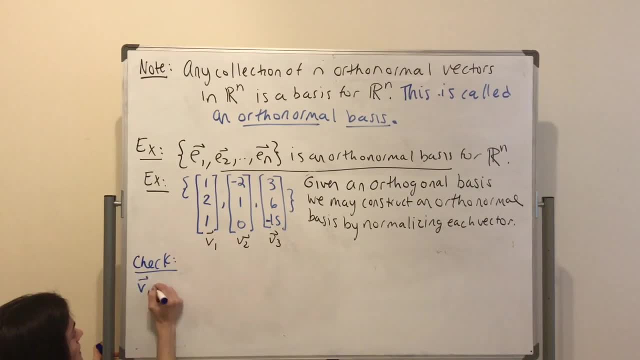 What I need to check here is that V1.V2 is zero. V1.. Uh-oh, I'll check it, but it should be zero. V1.V3 should be zero and then V2.V3 should be zero. 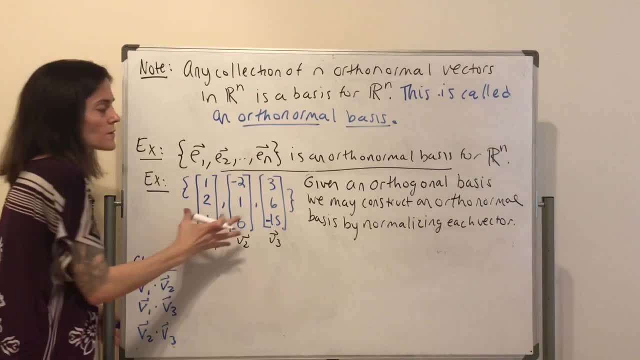 And if I have all of these zero, then I know that these are orthonormal, So I can just write this down. So I can write this down. So if I have all of these zero, then I know that these are orthonormal. 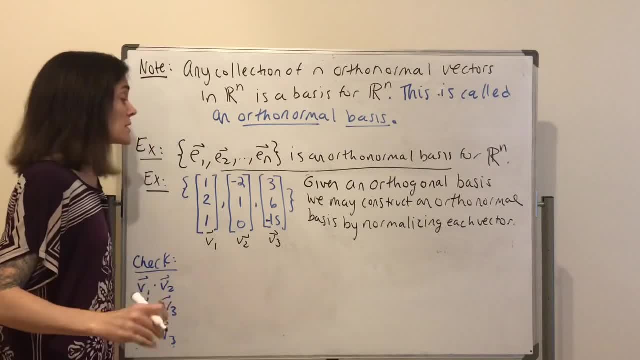 And if I have all of these zero, then I know that these are orthogonal And none of them are zero. They're in all three. They are a basis, But you can tell even by looking at V1 that these are not unit vectors. 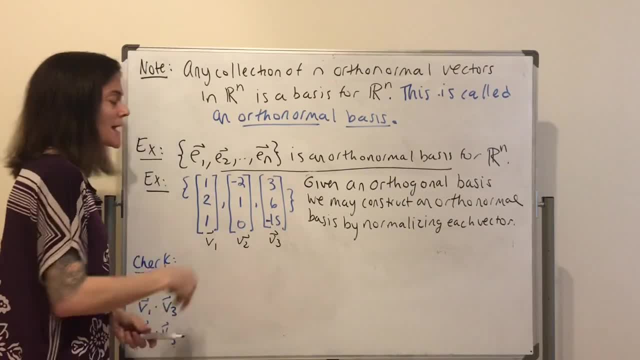 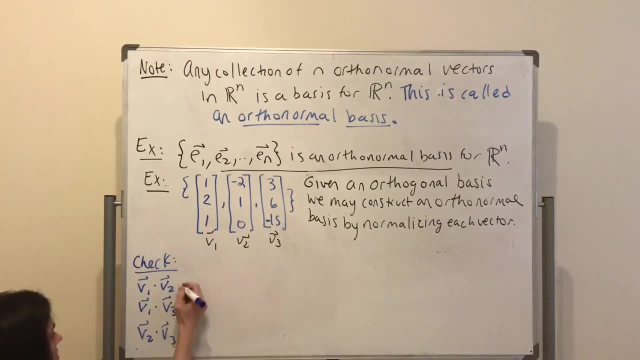 We can make an orthonormal basis by just taking each one and dividing by its length. Okay, that's what we'll do. So let's just check, just to make sure we have orthogonal vectors. V1.V2 is minus 2, plus 2.. 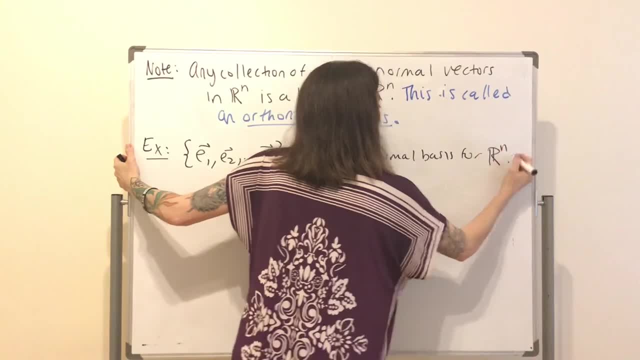 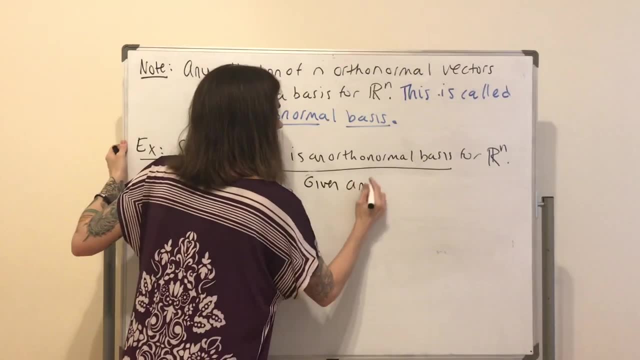 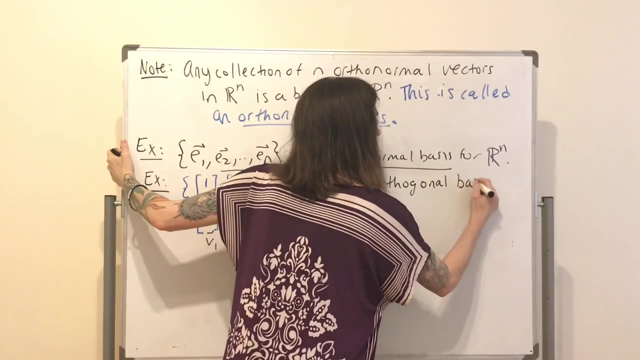 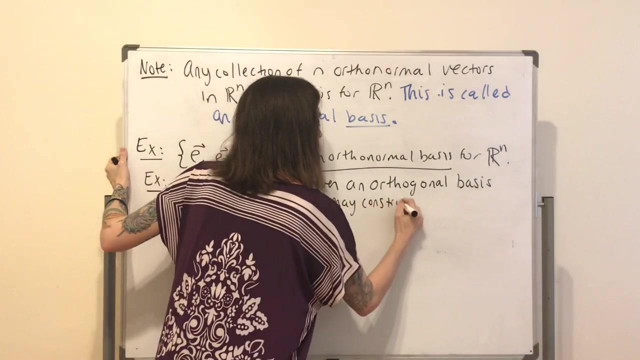 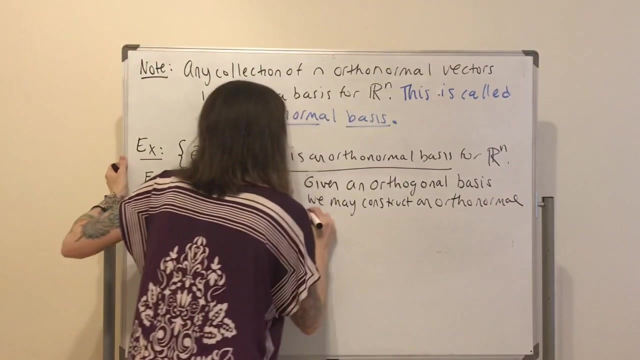 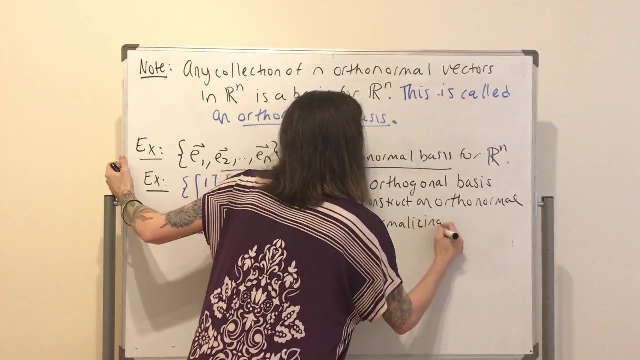 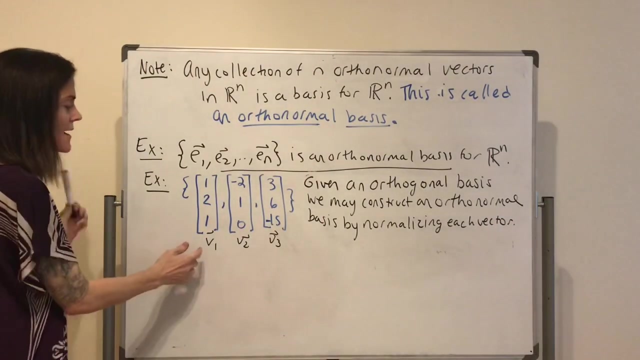 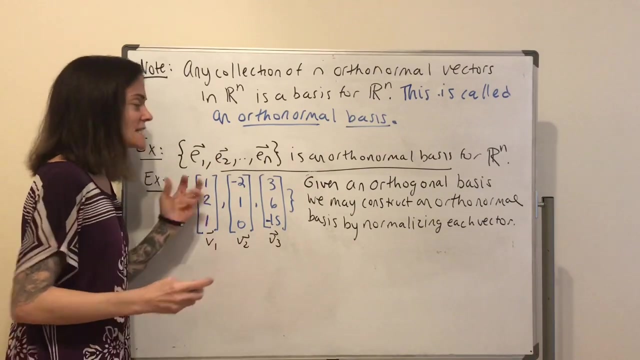 RN. now let's do another example. so what is this example going to be about? given a or an- I should say- orthogonal basis, we may construct an orthonormal basis by normalizing each vector. now, what does this mean? well, here I have be 1, v, 2, v, 3. there, in R 3, I had the right number, number 0. if I can show, then if I 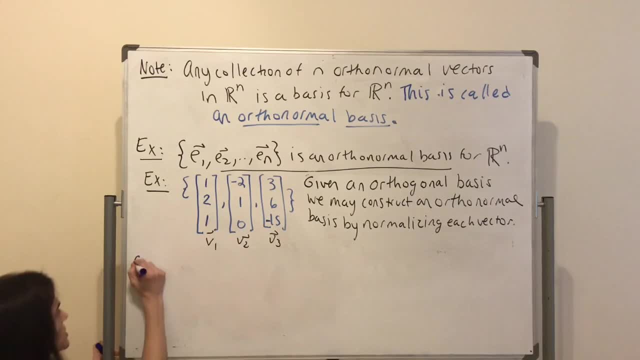 dot product and then let's check. let's check. what I need to check here is that V- V1- dot- V2 is 0.. V1, uh-oh, I'll check it, but it should be 0.. V1- dot- V3 should be 0.. 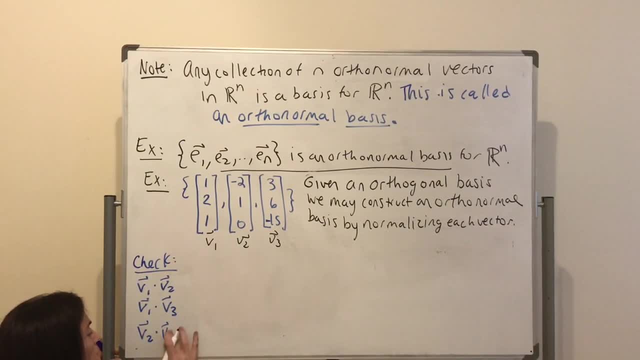 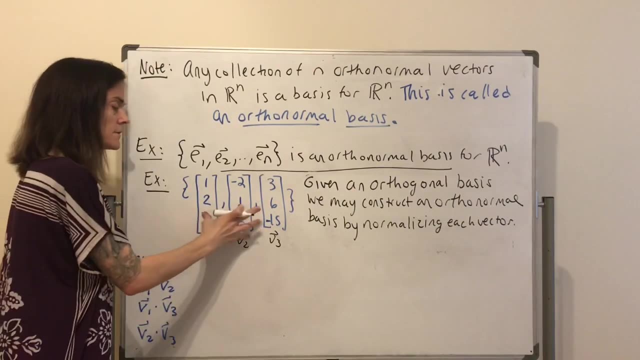 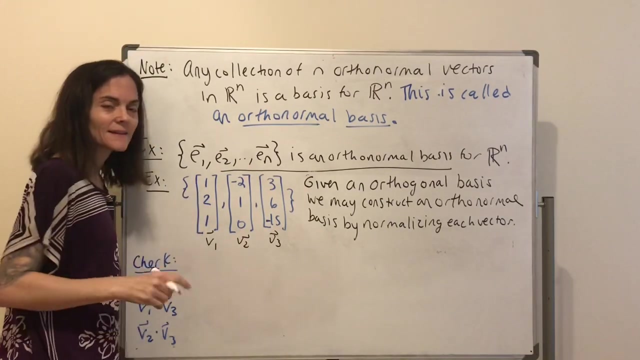 And then V2, dot. V3 should be 0. And if I have all of these 0, then I know that these are orthogonal And none of them are 0. They're in all three. They are a basis, But you can tell even by looking at V1 that these are not unit vectors. 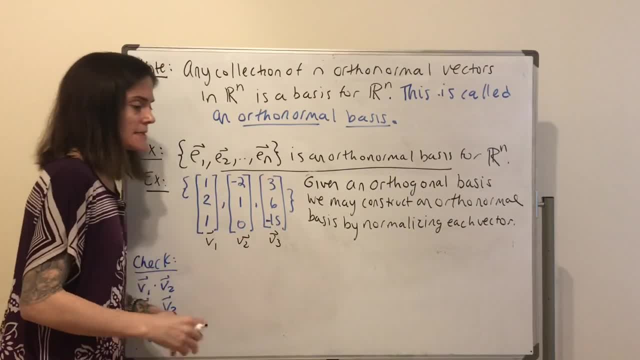 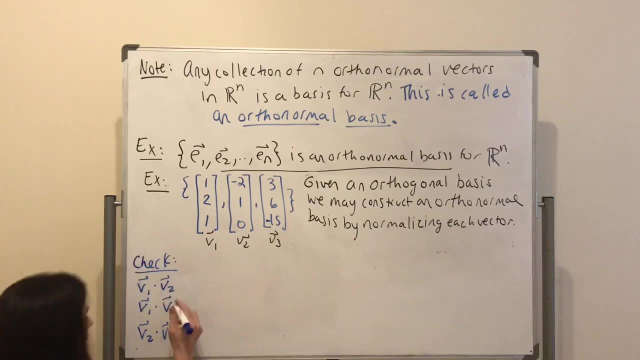 We can make an orthonormal basis by just taking each one and dividing by its length. Okay, that's what we'll do. So let's just check, just to make sure we have orthogonal vectors. V1 dot. V2 is minus 2 plus 2.. 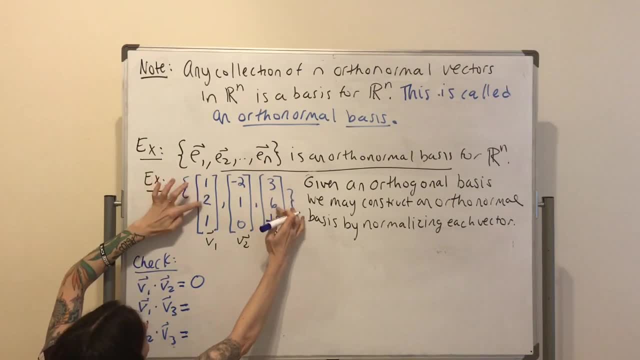 V1 dot V3 is 3, 12.. 3 and 12, 15. Minus 15.. And then V2 dot V3, minus 6 plus 6.. Okay, so in fact these are orthogonal. 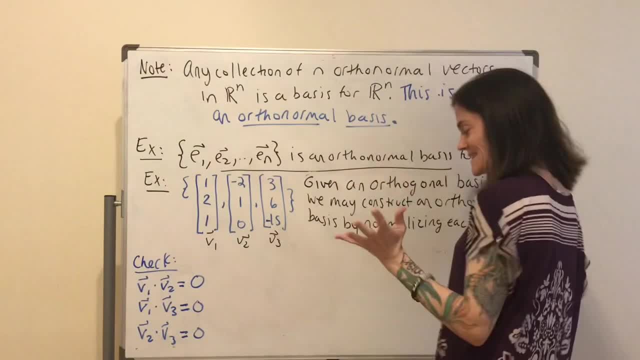 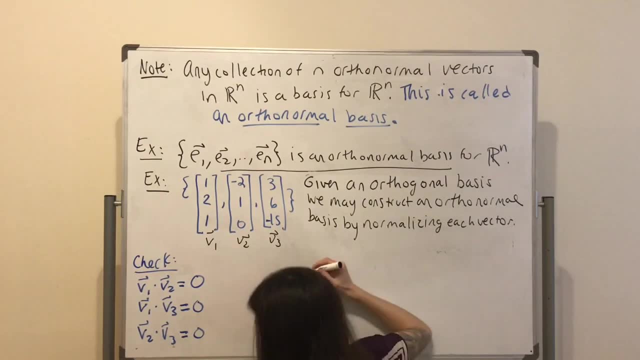 And then I can construct. Well, just as I said. Okay, so what we need to do is- maybe I'll move a little bit this way- The length of V1.. This is going to be the square root of 1, plus 4, plus 1.. 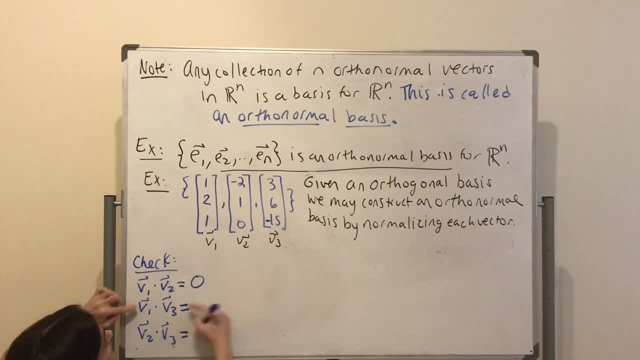 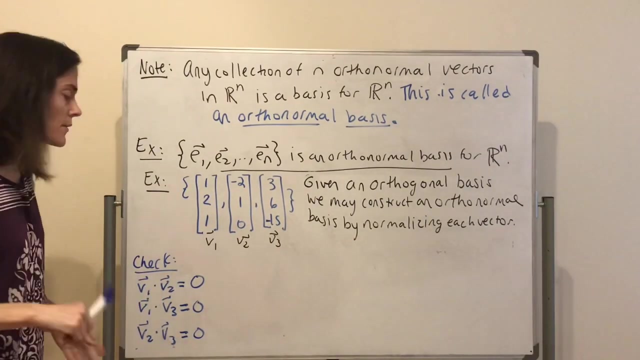 minus 2 plus 2, v1 dot v3 is 3, 12,, or 3 and 12,, 15, minus 15,, and then v2 dot v3 minus 6 plus 6.. Okay, so in fact these are orthogonal, And then I can construct. Well, just as I said, 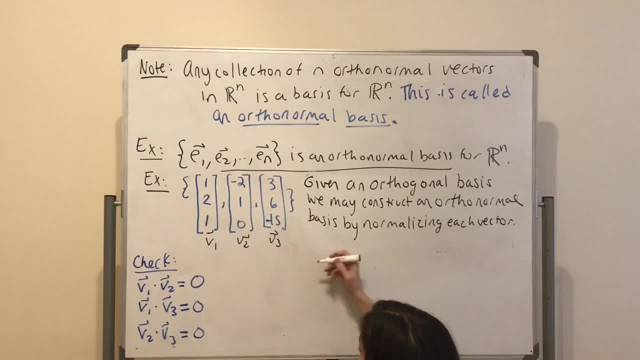 Okay, so what we need to do is- maybe I'll move a little bit this way- The length of v1, this is going to be the square root of 1 plus 4 plus 1.. This is the square root of 6.. The length of v2 is the square root of 4 plus 1.. 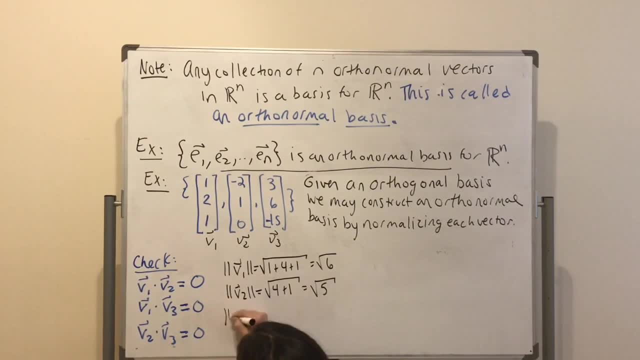 This is the square root of 5.. And the length of v3,. this is the square root of 9 plus 36,. uh-oh, 15 squared, Let's see We would have 15 times 10 is 150,. 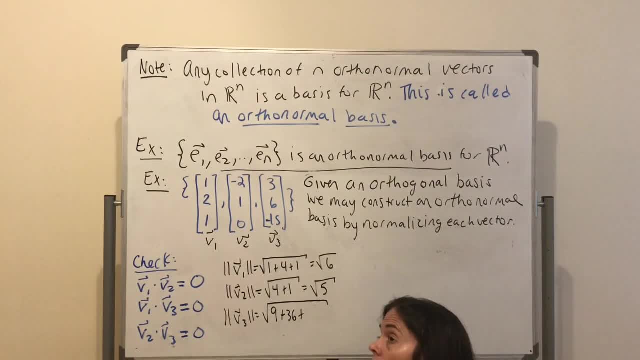 and then 15 times 5 is another 75. So this is 225, and when we add these to 70.. Okay, and this is the same as 9 times. oh, so it's going to be 3 square root of 30.. 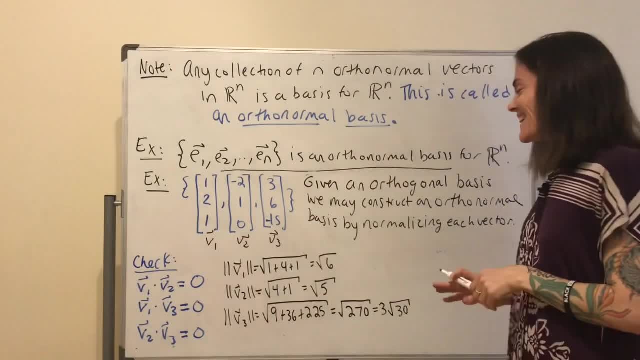 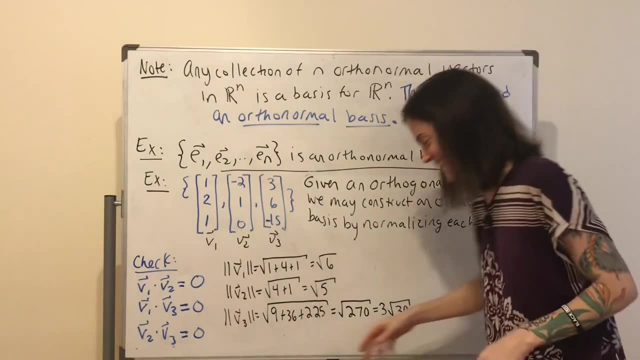 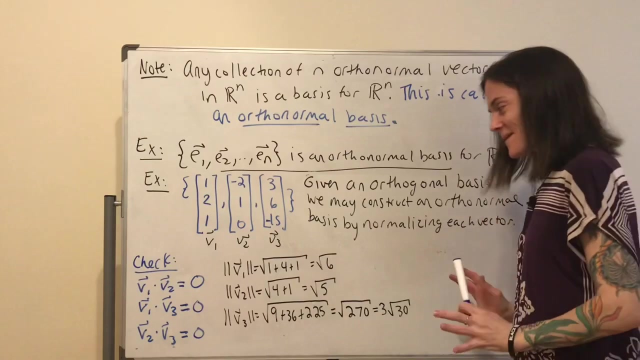 Okay, Okay. I don't really multiply numbers so well in my head. Okay, that was challenging for me. I should be up here with a calculator if I'm going to put numbers like that in a problem. I think we're okay now. 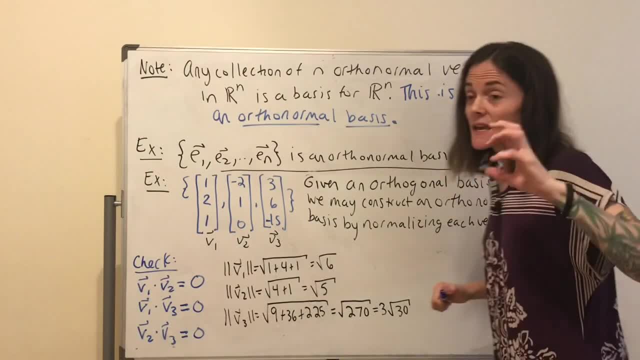 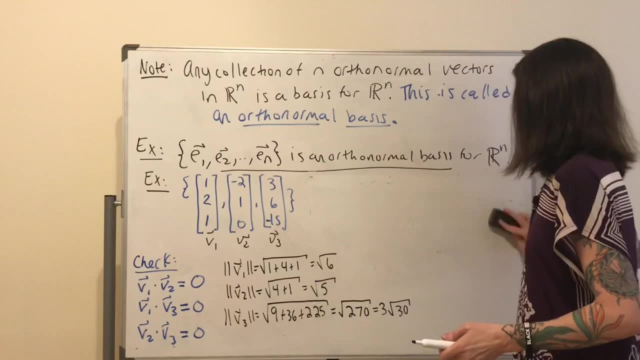 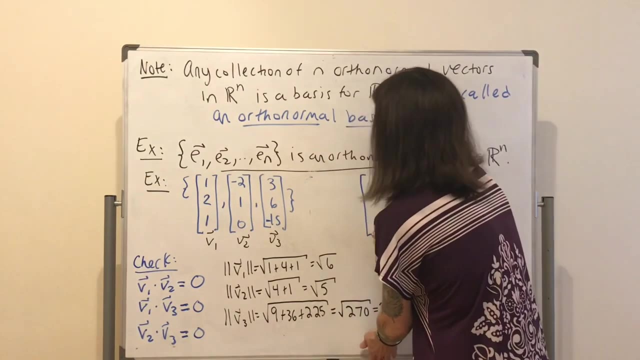 Hopefully I didn't make a mistake. So now you see to get the orthonormal basis. Maybe at this point I will erase this. I've discussed what we are doing. It gives me space to write our orthonormal basis. My orthonormal basis is as follows. 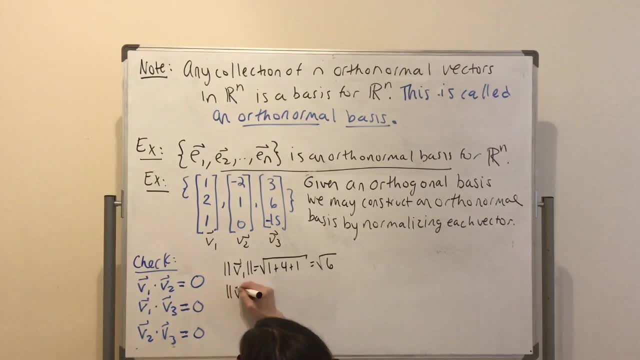 This is the square root of 6.. The length of V2 is the square root of 4 plus 1.. This is the square root of 5. And the length of V3.. This is the square root of 9 plus 36.. 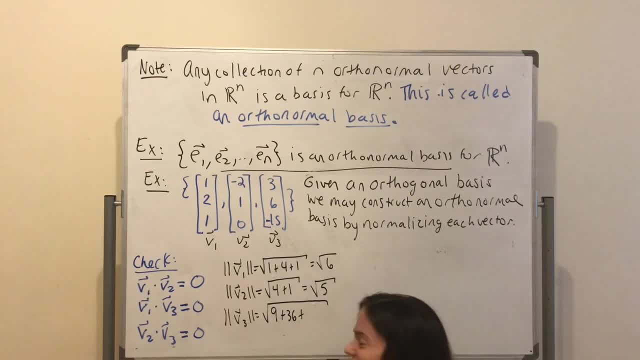 Uh-oh, 15 squared, Let's see We would have: 15 times 10 is 150. And then 15 times 5 is another 75. So this is 225. And when we add these to 70.. 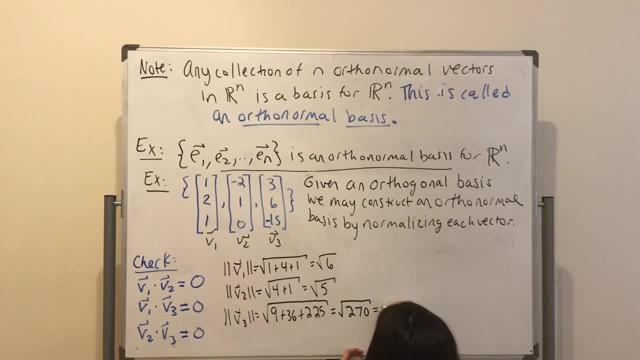 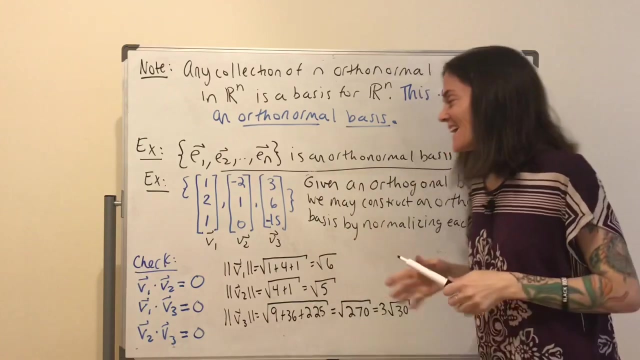 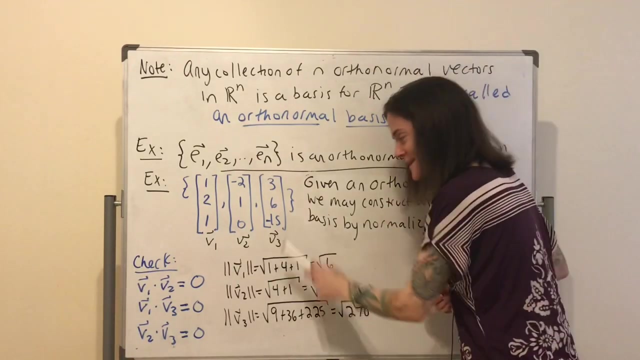 Okay, And this is the same as 9 times Oh, so it's going to be 3 square root of 30.. Okay, I don't really multiply numbers so well in my head. Okay, That was challenging for me. I should be up here with a calculator if I'm going to put numbers like that in a problem. 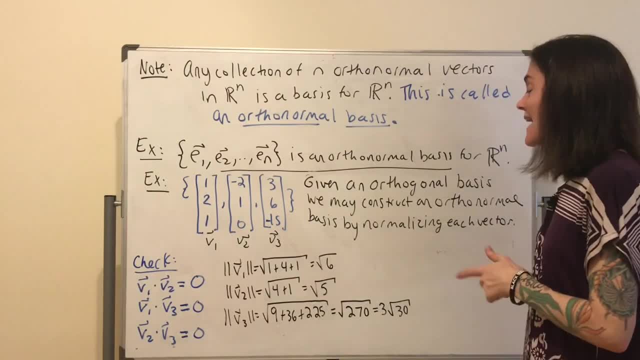 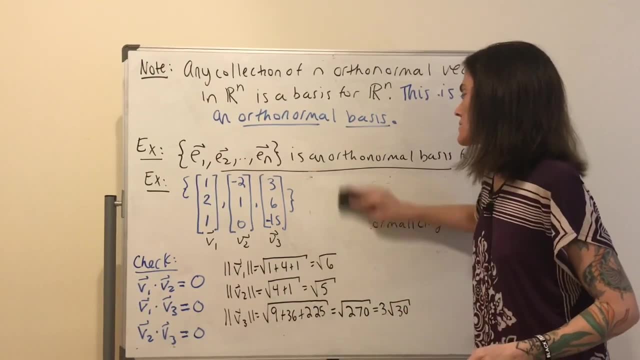 I think we're okay. Okay now, hopefully I didn't make a mistake. So now you see to get the orthonormal basis. Maybe at this point I will erase this. I've discussed what we are doing. It gives me space to write our orthonormal basis. 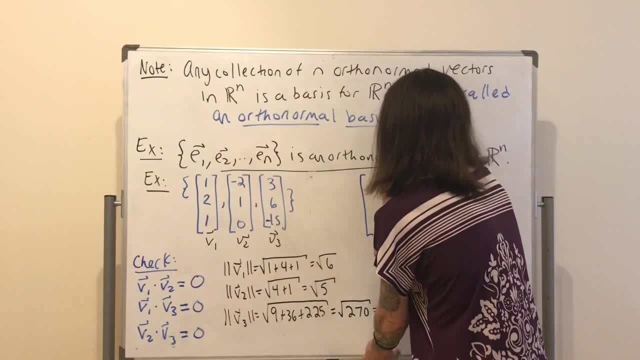 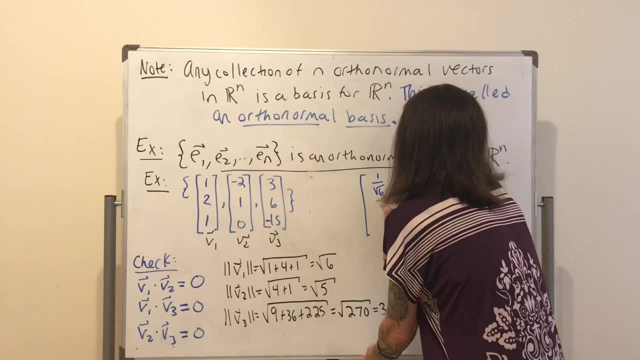 My orthonormal basis is as follows: 1 over the square root of 6.. Uh-oh, Maybe I'll have a little more space. And then we have 2 over the square root of 6.. And then we have: 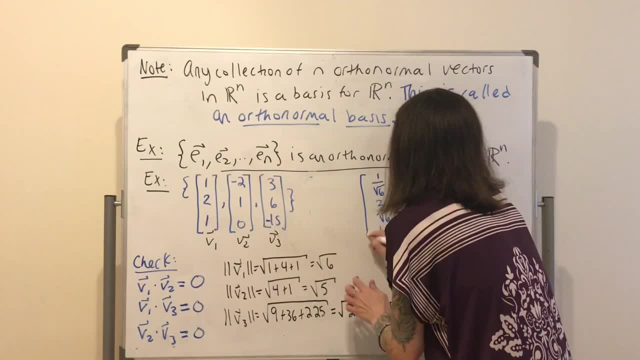 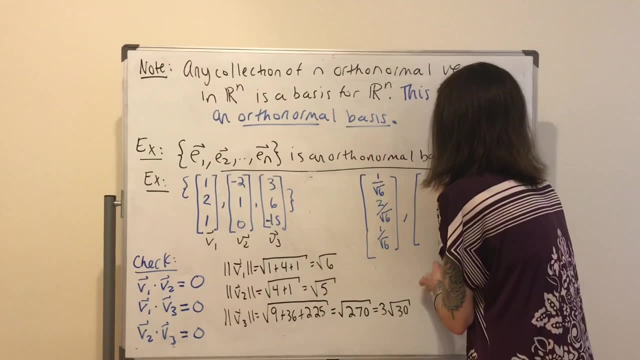 1 over the square root of 6.. This is my first vector. I took v1 divided by its length. My second vector is minus 2 over the square root of 5.. 1 over the square root of 5 and 0.. 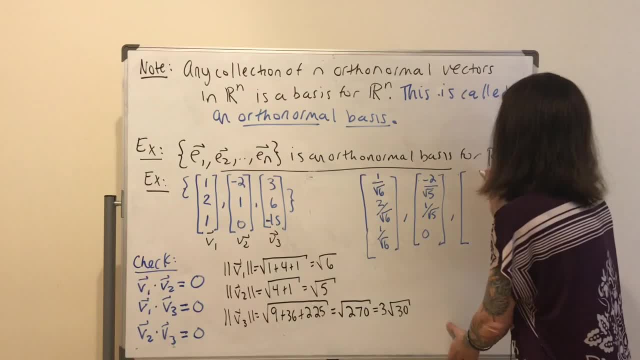 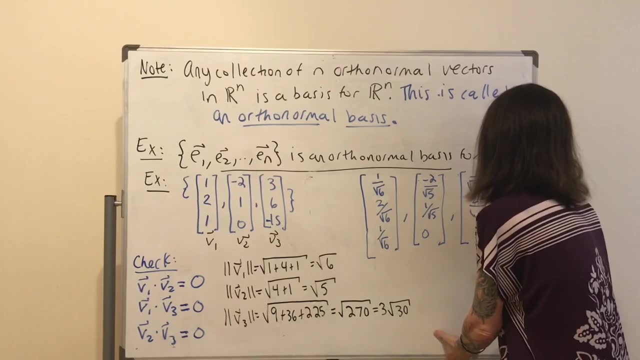 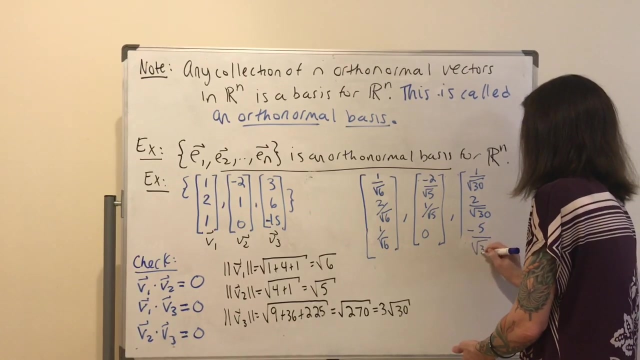 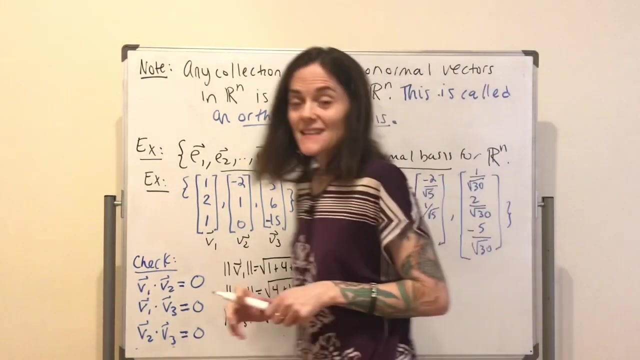 Finally, my third vector, Okay, is 1 over the square root of 30.. And then 2 over the square root of 30. Finally, minus 5 over the square root of 30.. Okay, This collection here is an orthonormal basis for our 3.. 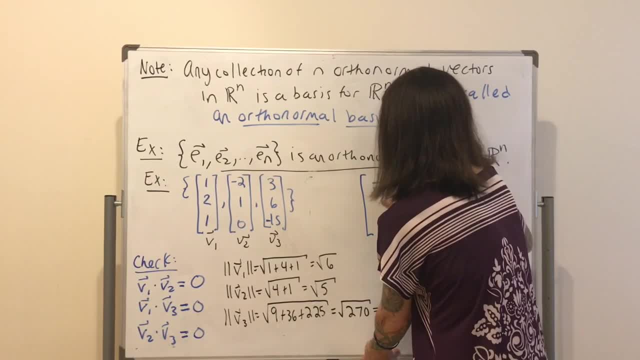 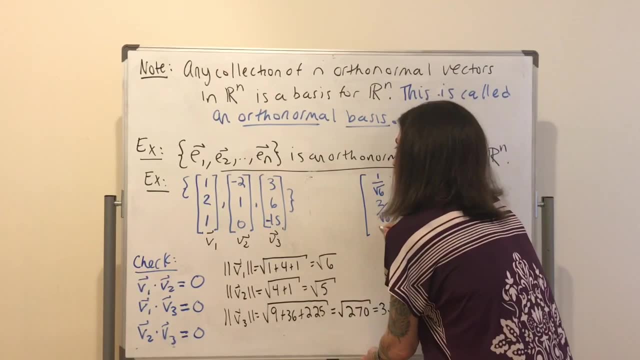 1. 1 over the square root of 6.. Uh-oh, Maybe I'll have a little more space. And then we have 2 over the square root of 6.. And then we have 1 over the square root of 6.. 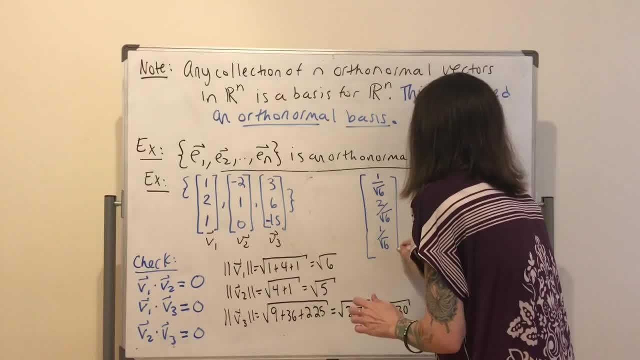 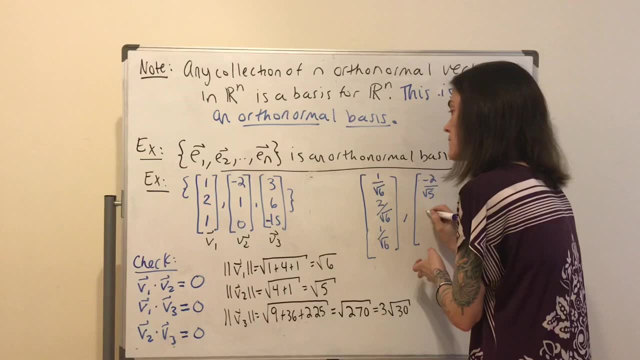 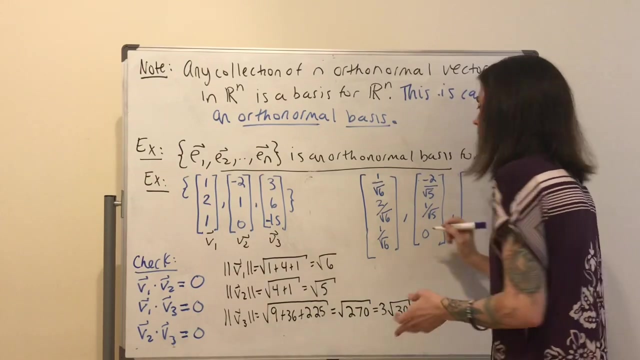 This is my first vector. I took v1 divided by its length. My second vector is minus 2 over the square root of 5.. 1 over the square root of 5 and 0. Okay. Finally, my third vector- okay- is 1 over the square root of 30.. 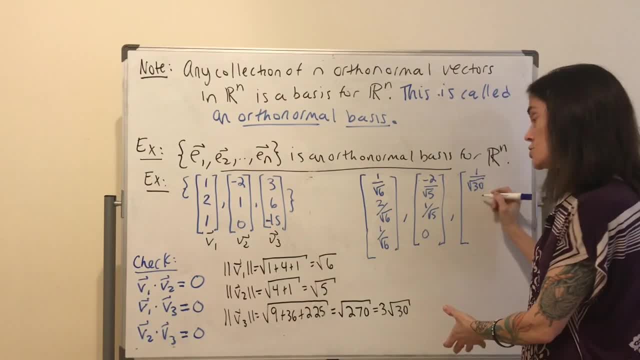 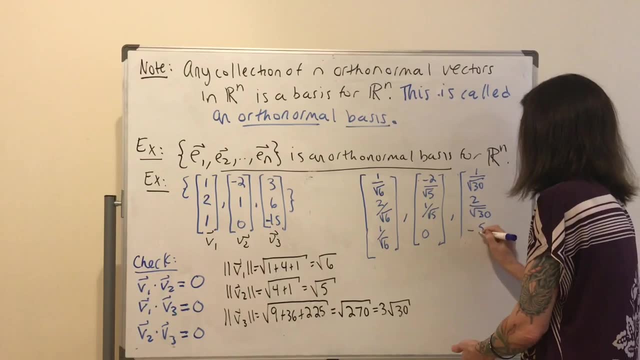 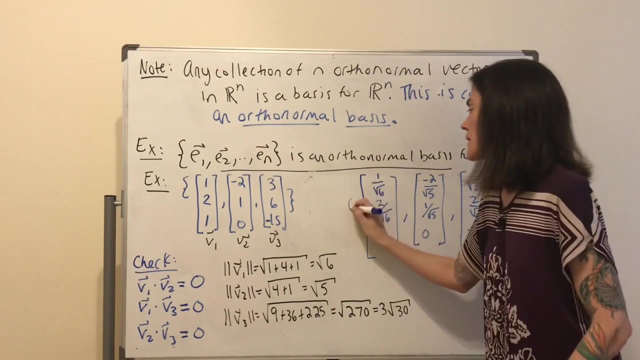 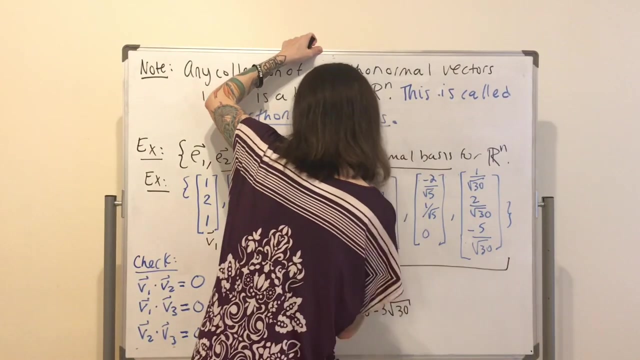 And then 2 over the square root of 30.. Finally, minus 5 over the square root of 30.. Okay, This collection here is an orthonormal basis for our 3.. So here, Maybe I'll write this: Okay. 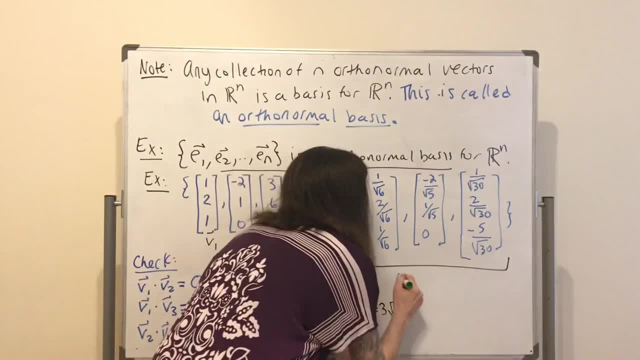 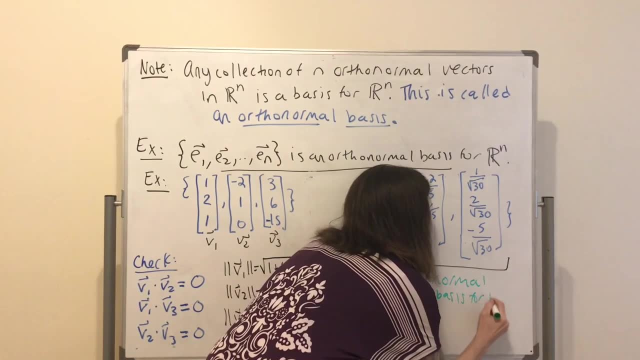 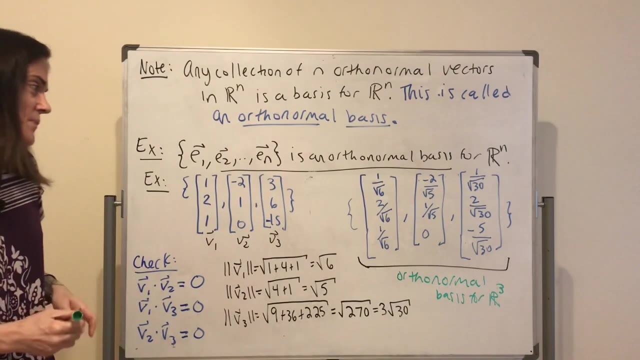 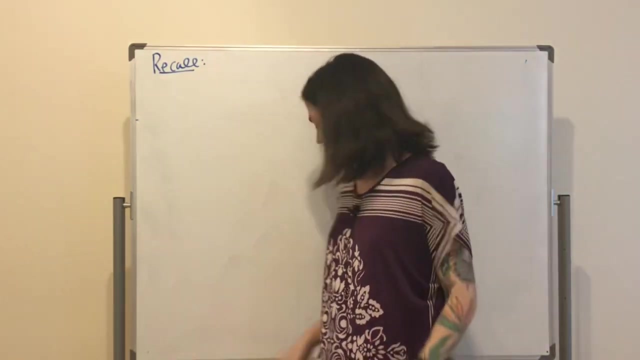 Maybe I'll write what I just said. This is an orthonormal basis for our 3. And I'm going to come back and use these vectors and an example in a little while. Let's move into orthogonal projection. However, we have discussed 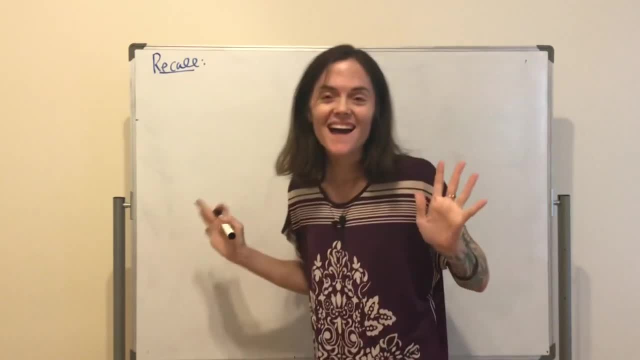 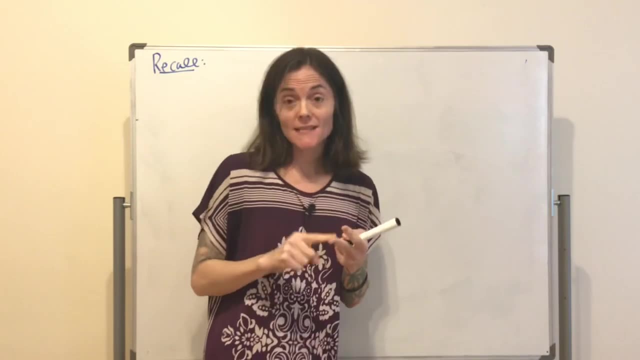 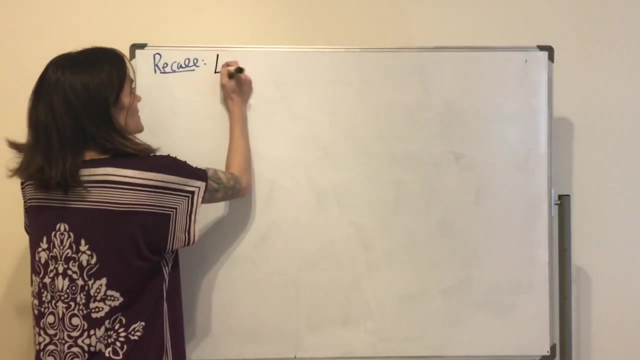 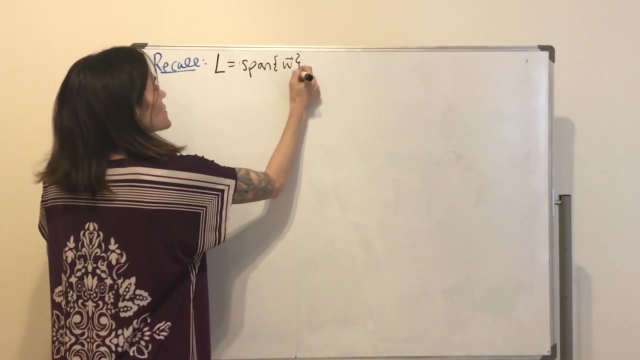 At least to project Uh Um Along a line, And we did this carefully when we were talking about well, rotation, reflection, projection, scaling, Things like this. So What is this? Well, if L is the span of a vector, w for w, not equal to 0 in Rn. 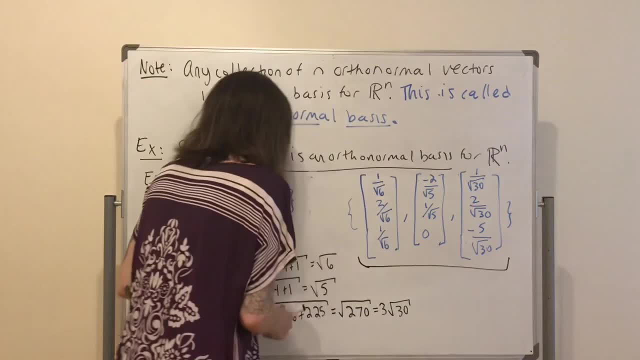 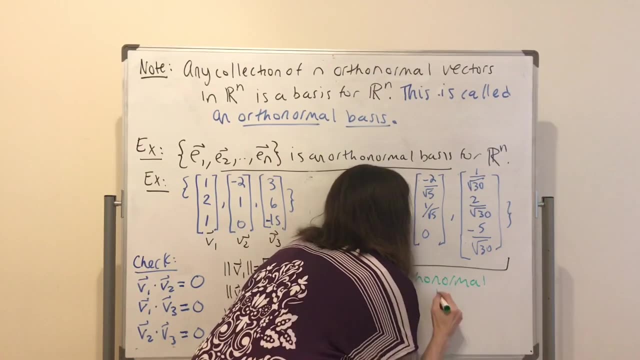 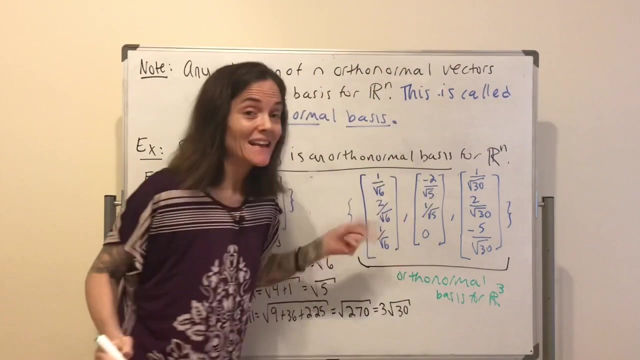 So here, maybe I'll write what I just said. This is an orthonormal basis. This is an orthonormal basis for our 3. And I'm going to come back and use these vectors in an example in a little while. 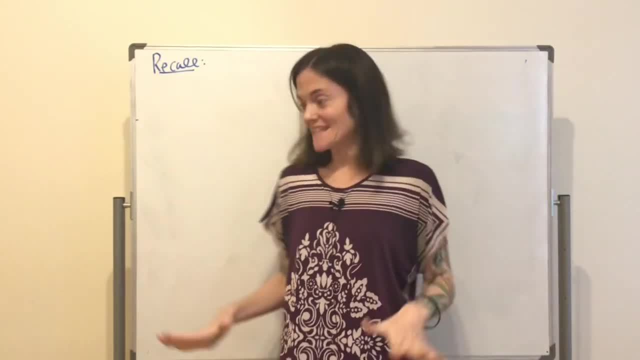 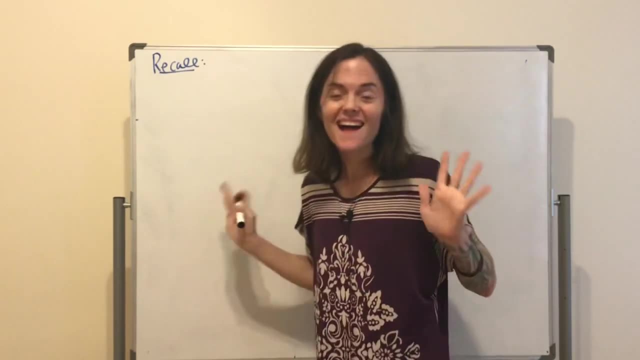 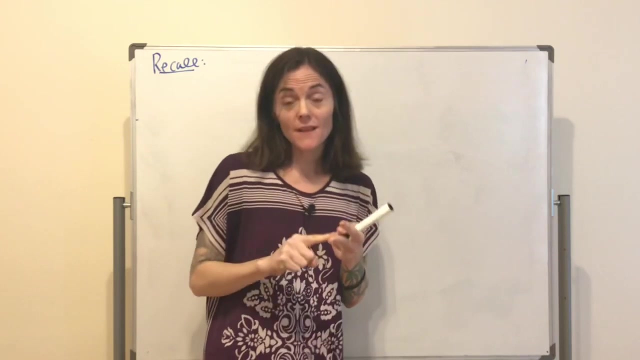 Let's move into orthogonal projection, However. we have discussed at least to project along a line, And we did this carefully when we were talking about well, rotation, reflection, projection, scaling, things like this. So what is this? 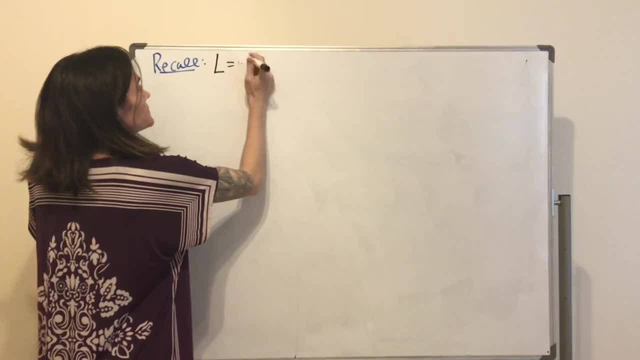 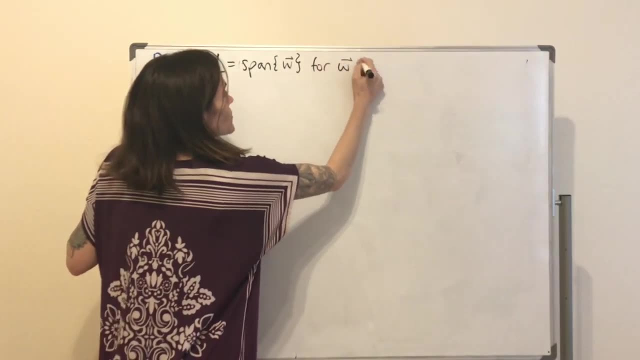 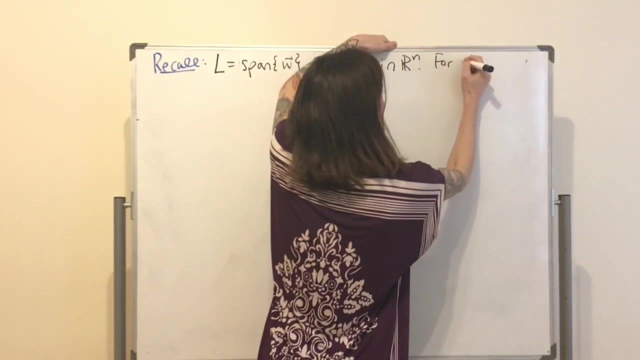 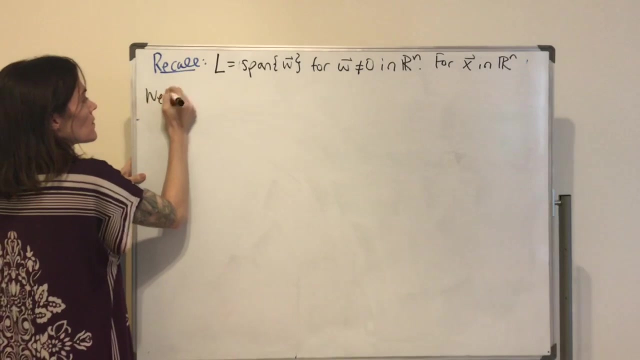 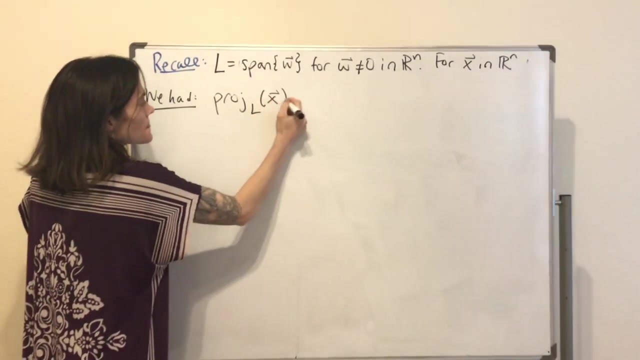 Well, if L is the span of a vector w for w not equal to 0 in Rn, then we take some vector x in Rn, Okay, And we have the following the projection: well, it's along the line. 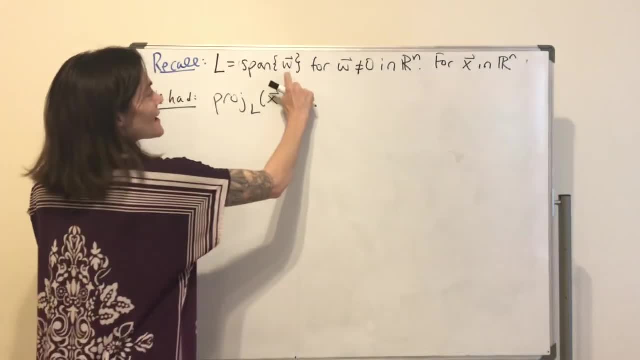 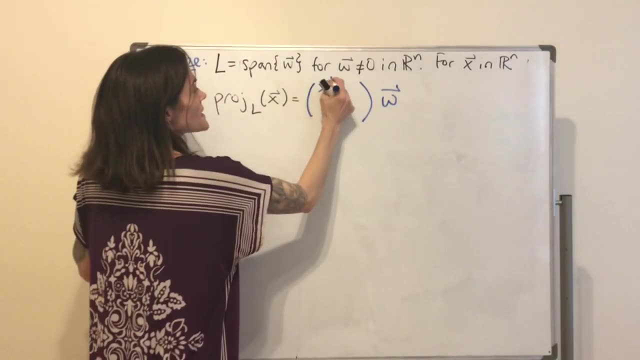 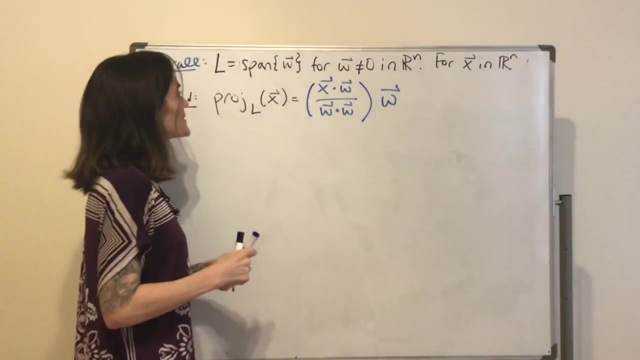 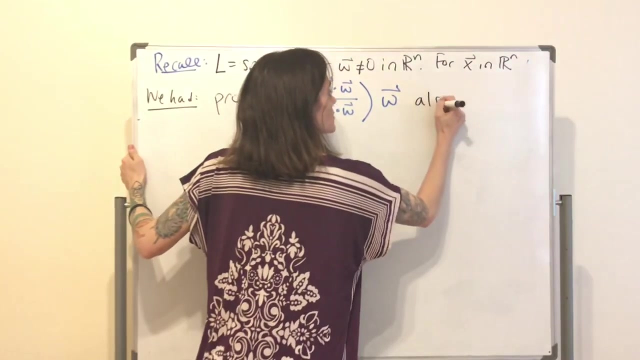 which means the projection will be a multiple of w And the multiple was xw over ww. Okay, And this defines a vector on the line L, And this was also called or also denoted, I should say it was this: 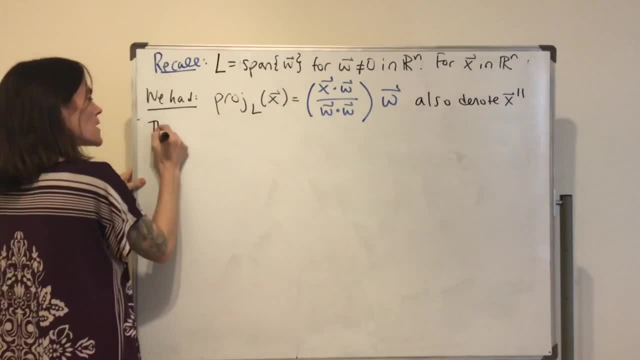 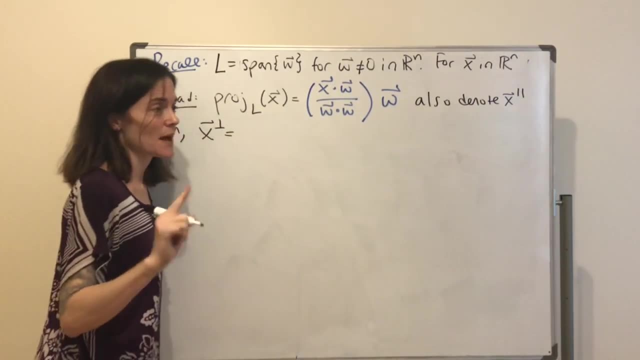 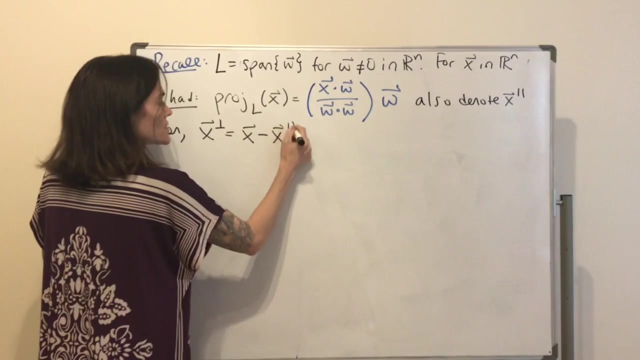 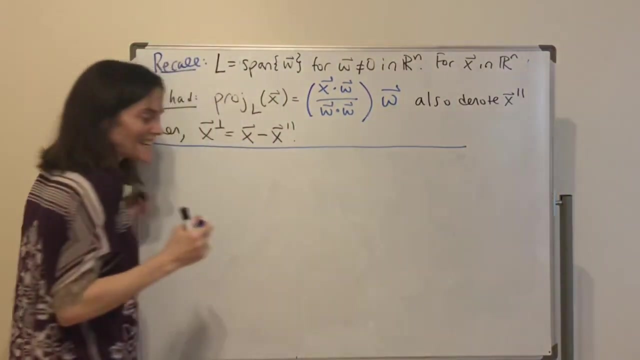 This was the orthogonal projection. And then we also had the following: This was the component of x that was perpendicular to the line or orthogonal to the line. This was x minus. This was the orthogonal projection. Okay, Well, what am I changing now? 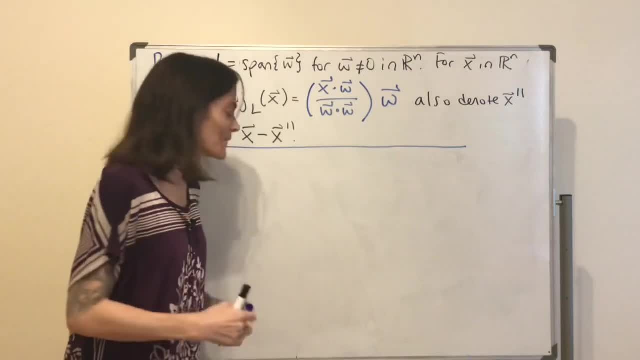 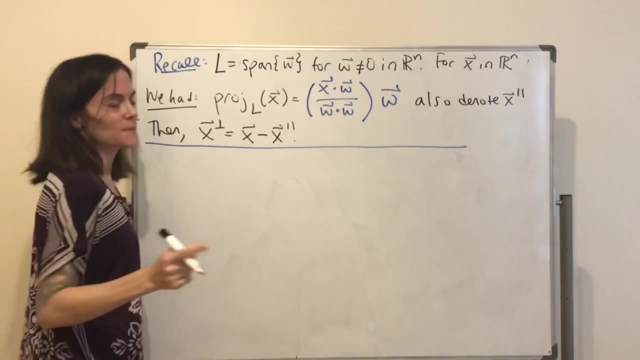 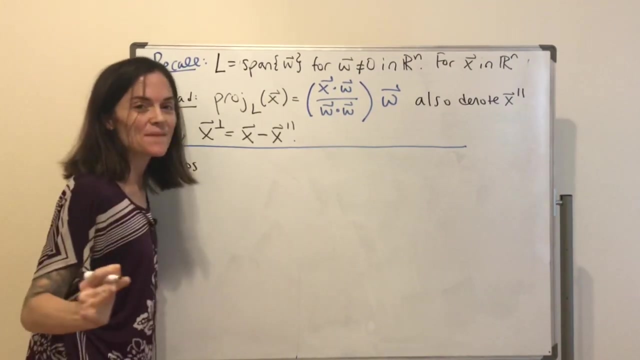 Or what is the orthogonal projection we're talking about now? Well, it's not all that different. in fact, This is a one-dimensional subspace in Rn, And all we're changing is we're taking any subspace of Rn. 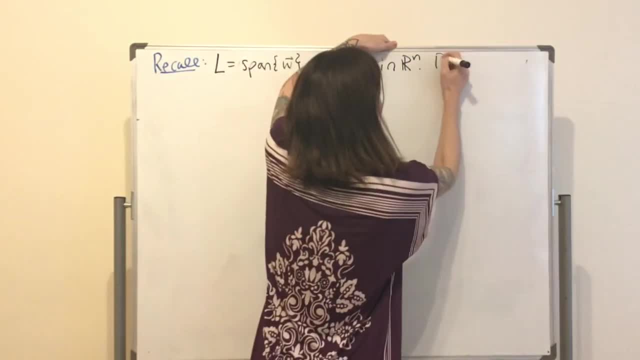 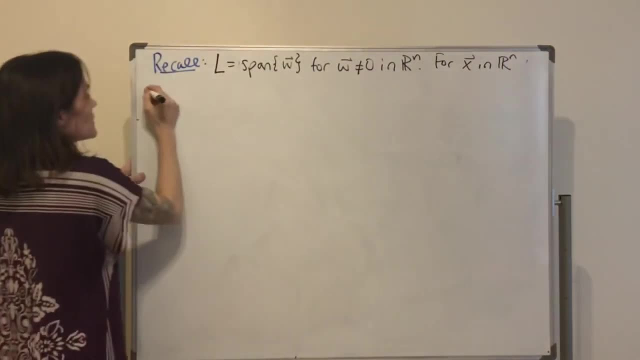 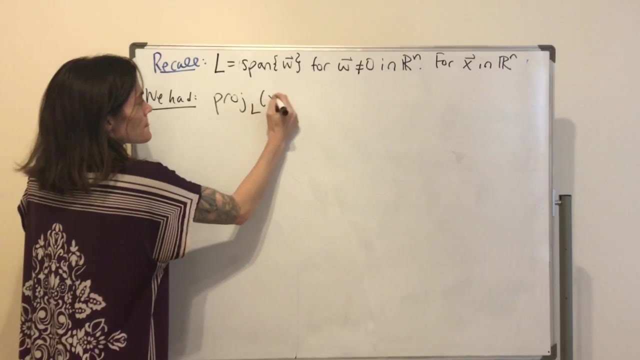 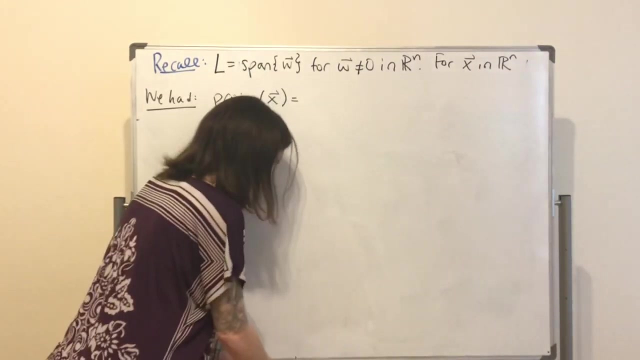 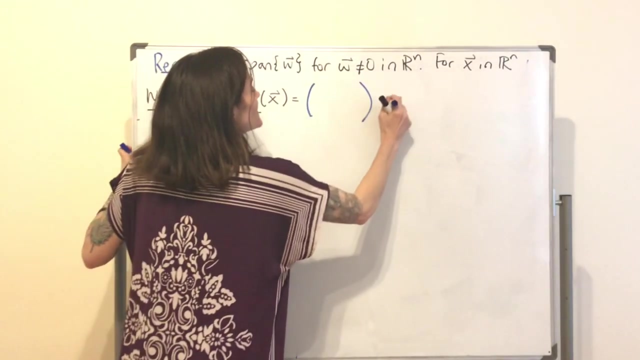 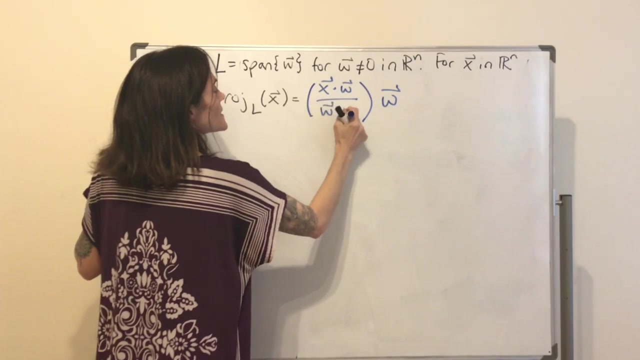 Then we take Some vector x and Rn, We had the following: The projection. Well, it's Along the line, which means the projection will be a multiple of W and the multiple was x dot w over w dot w and this defines a vector on the line l. 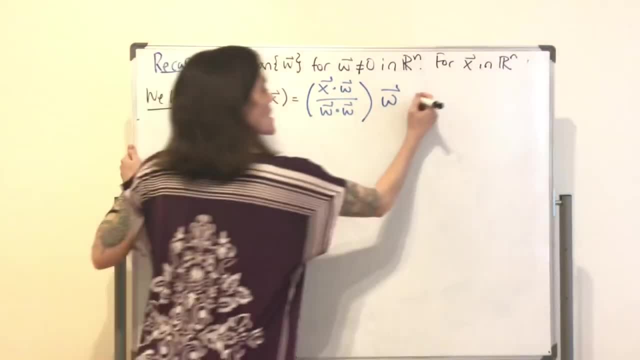 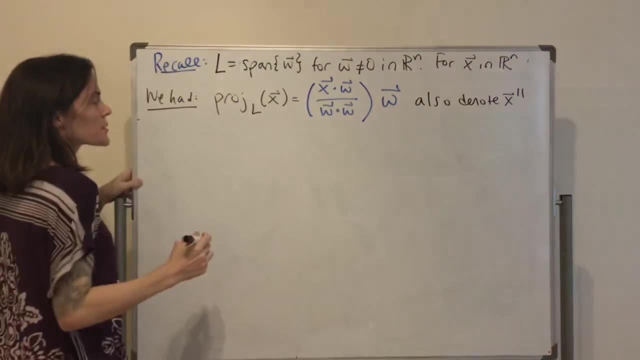 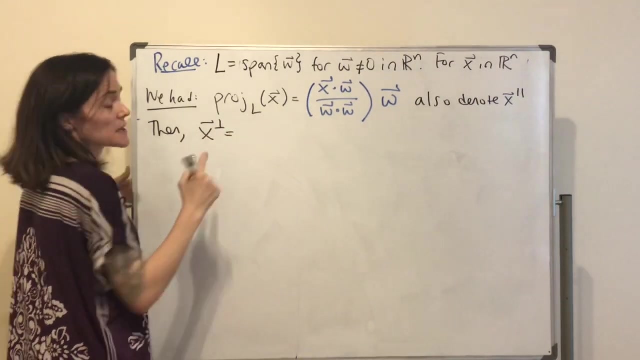 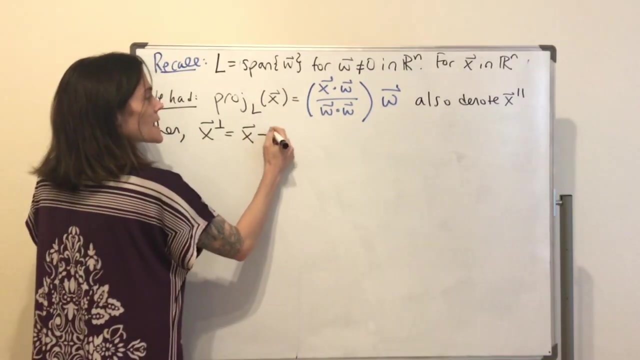 and this. this was also called, or also denoted, I should say it was this: this was the orthogonal projection. and then we also had the following: this was the component of x that was perpendicular to the line or orthogonal to the line. this was x minus the orthogonal projection. 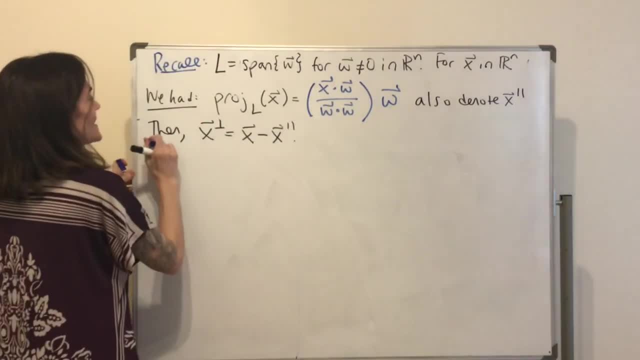 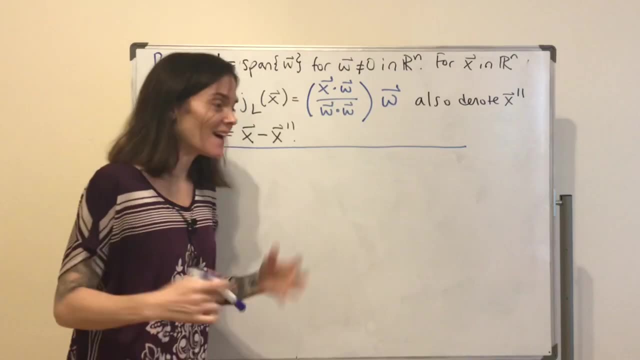 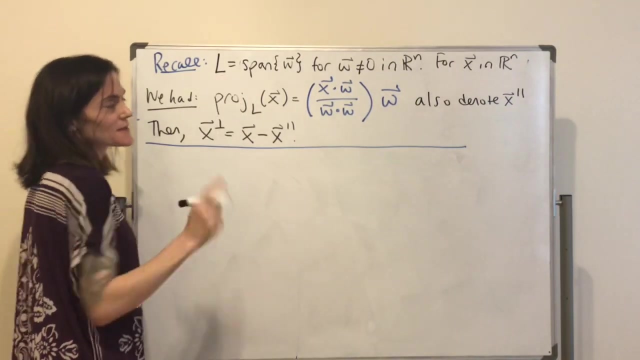 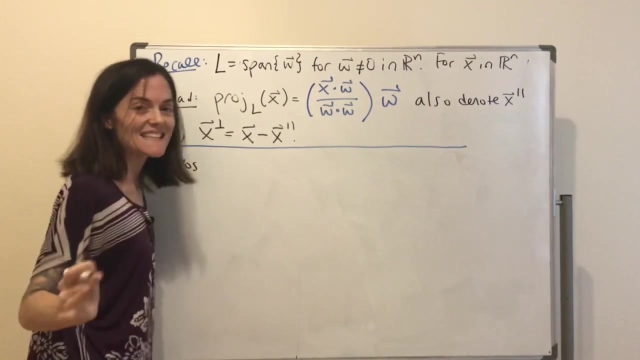 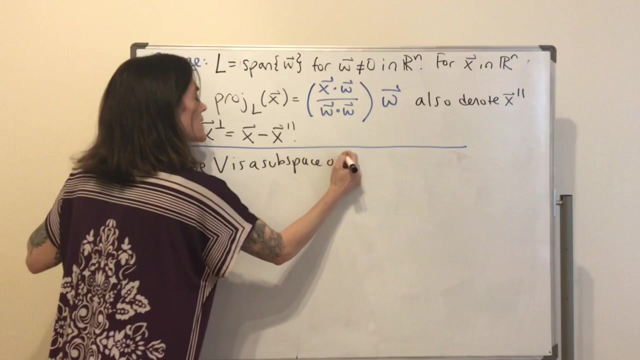 okay. well, what am I changing now? or what is the orthogonal projection we're talking about now? well, it's not all that different. in fact, this is a one-dimensional projection. this is a one-dimensional projection. so suppose we have an orthogonal sub space in our n and all we're changing is 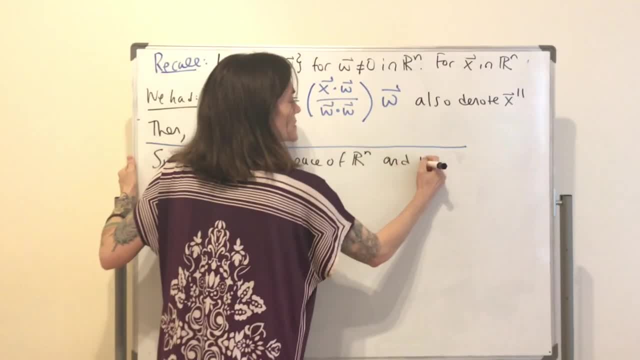 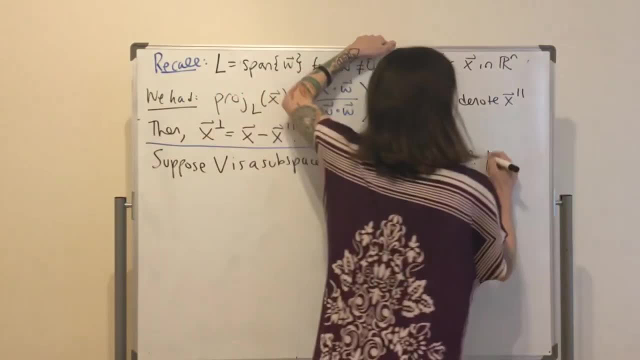 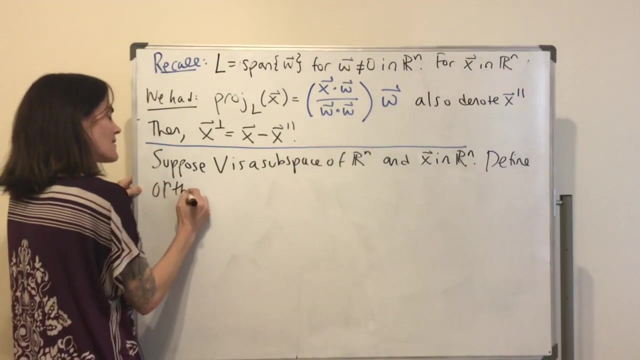 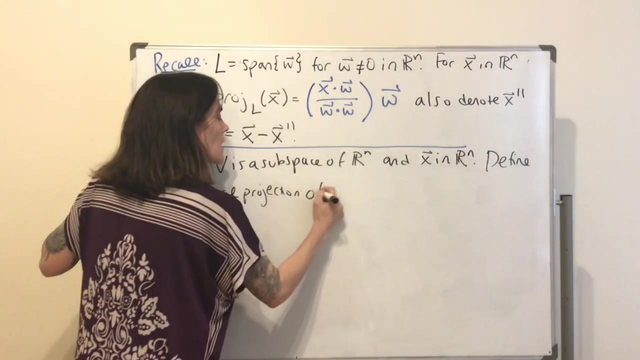 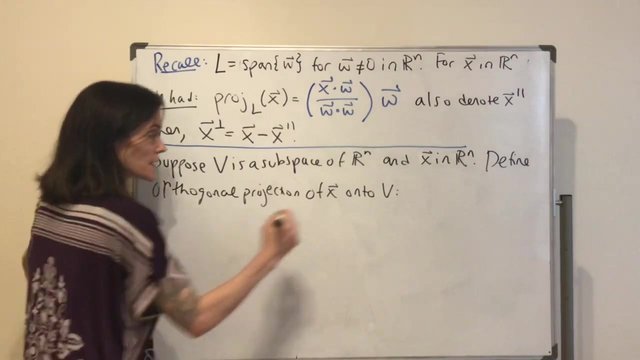 we're taking any subspace of our n. so suppose V is a subspace of our n and we have some vector X in our n, and then we want to define the orthogonal projection of x well on to the subspace v, and this will be denoted. 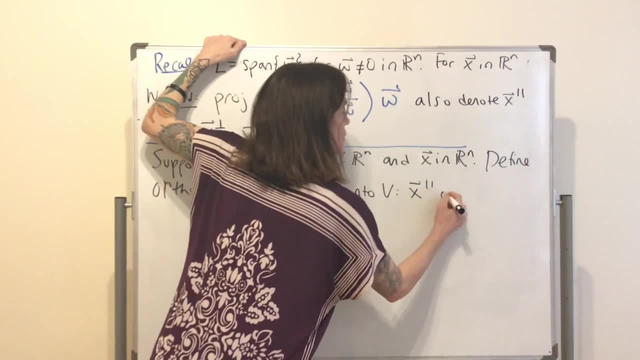 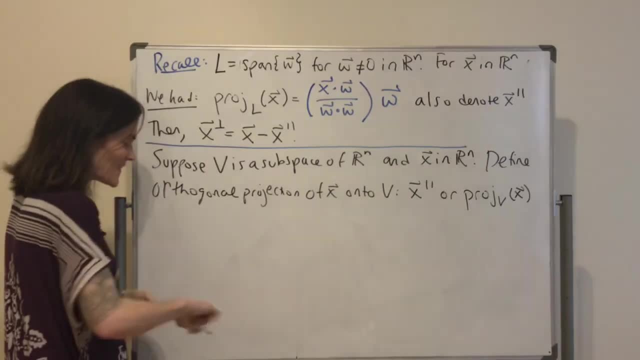 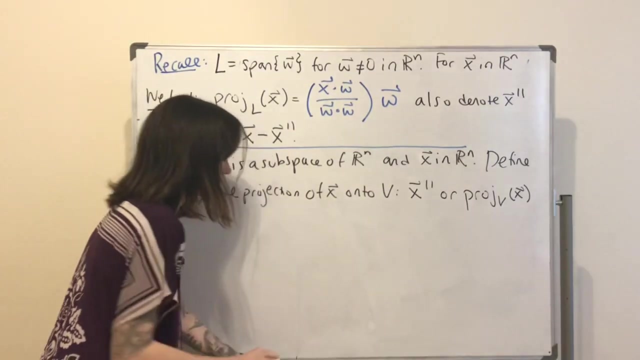 while we still have this notation or this notation, okay, well, what is this? it's going to be a vector and it's going to be a vector in v. okay, that's only thing that would make sense for this here, this well, and it's very much like this, as i 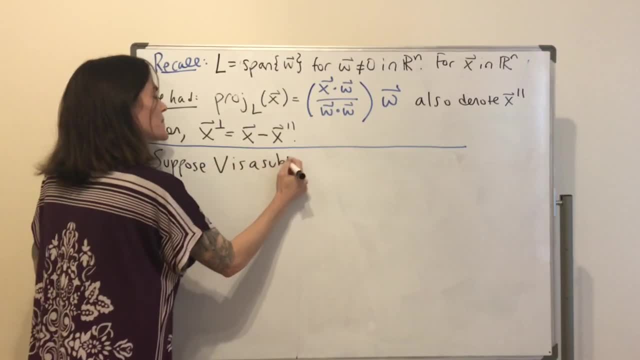 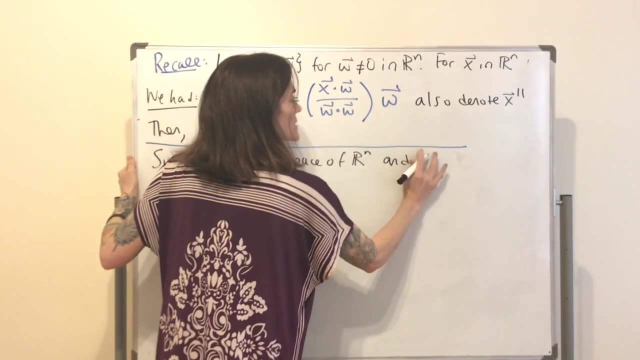 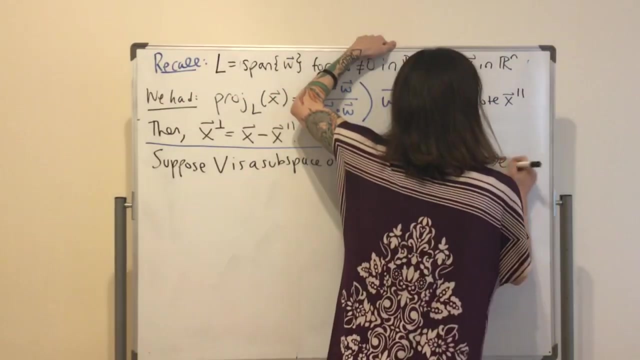 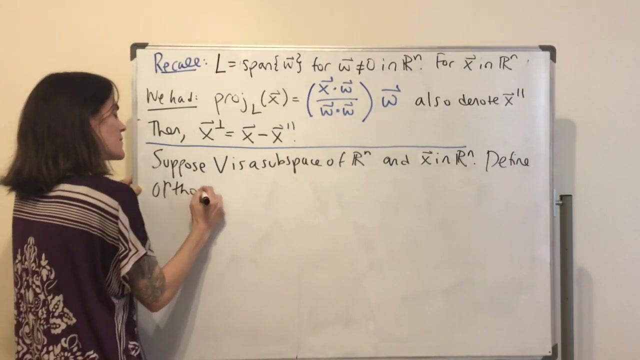 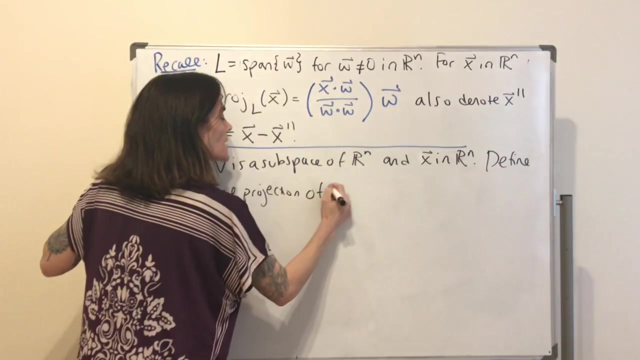 So suppose V is So V is a subspace of Rn, And we have some vector x in Rn, And then we have some vector x in Rn, And then we want to define the orthogonal projection of x Well, on to the subspace V. 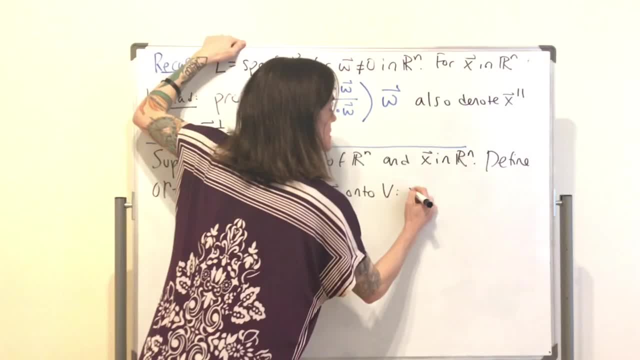 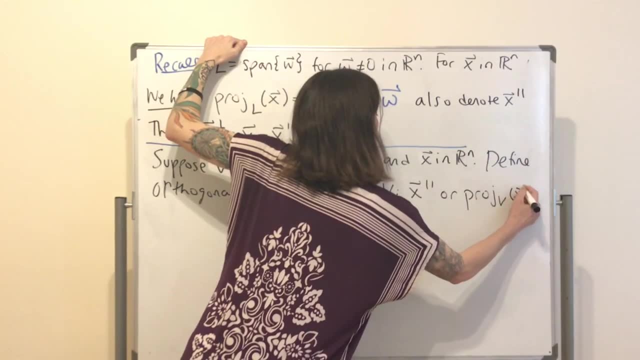 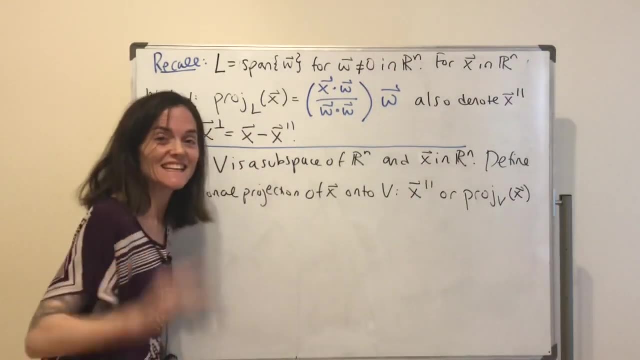 And this will be denoted while we still have this notation or this notation. Okay, well, what is this? It's going to be a vector and it's going to be a vector in V. okay, That's the only thing that would make sense for this here. 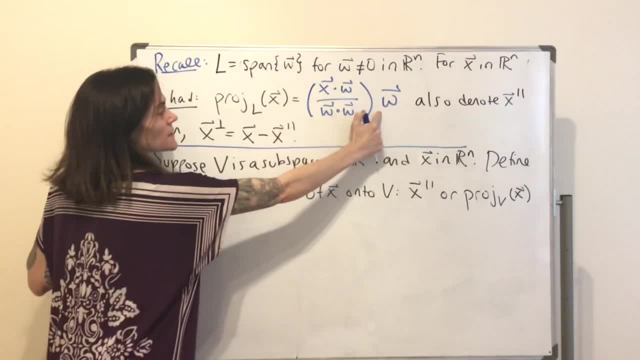 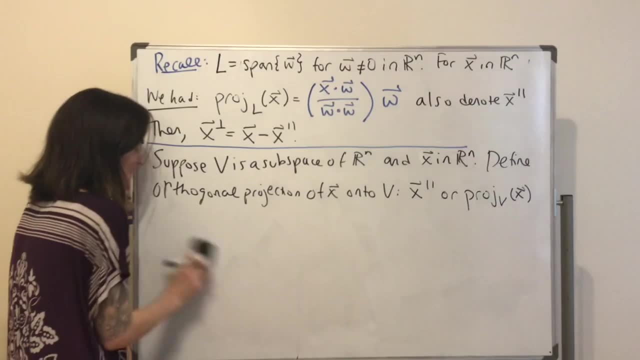 Well, and it's very much like this. as I mentioned, This was a vector in the subspace. once we project it, Uh-oh well, I'm not ready to define it yet. So what I need to define this orthogonal projection is: I need an orthonormal basis for V. 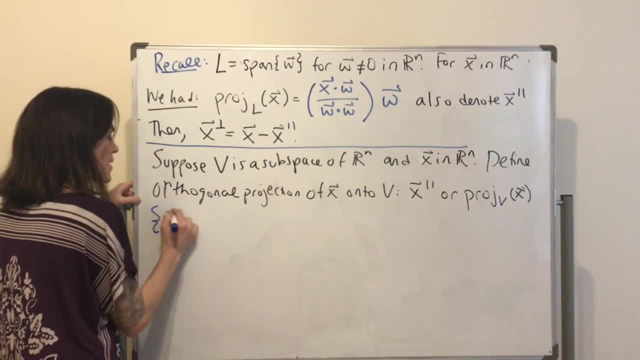 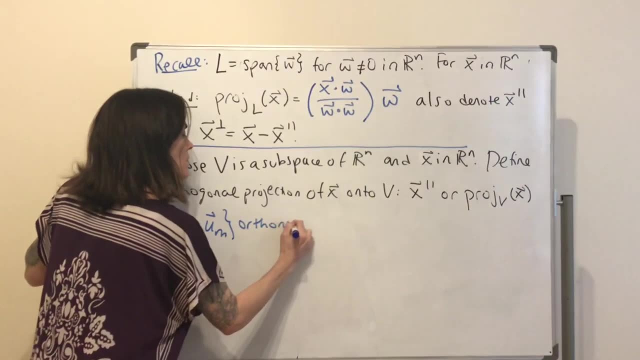 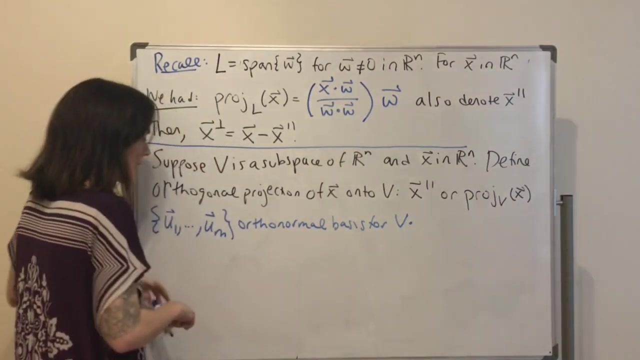 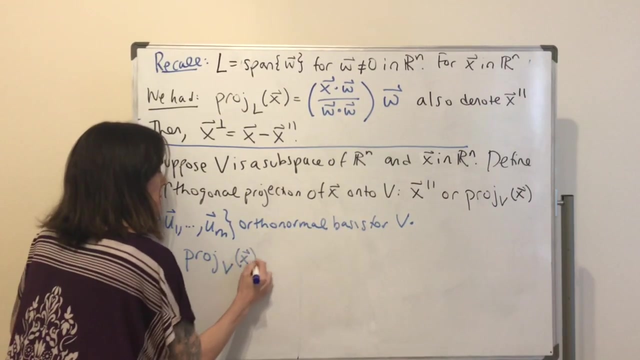 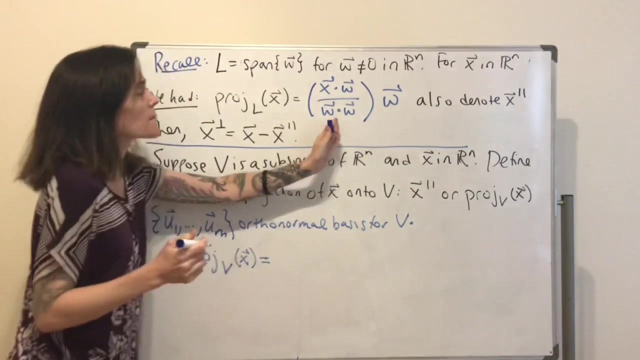 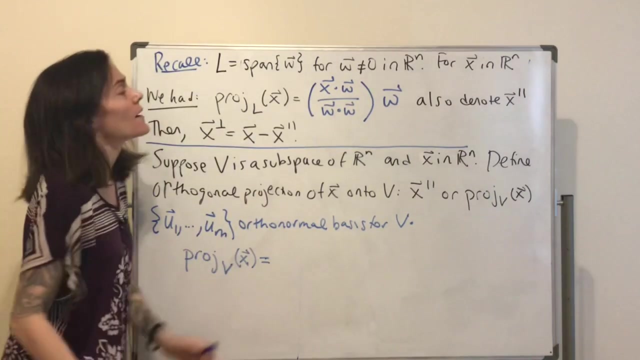 So let's take U1 out to UM orthonormal basis for V, And now I can define this. The projection is equal to: okay, it's going to look just like this. Now, what would this formula- and we even discussed this- if, in fact, W was a unit vector, as all of these are? 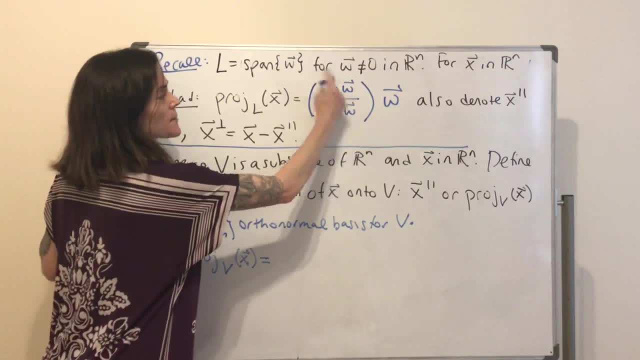 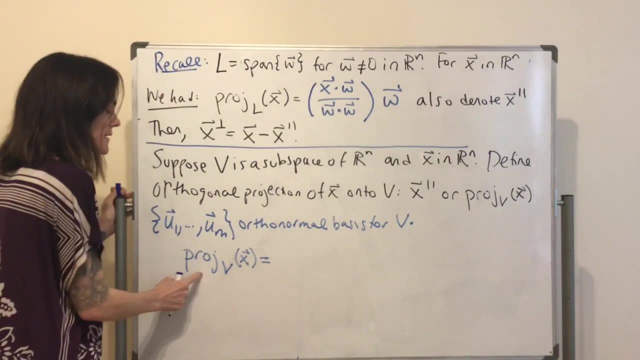 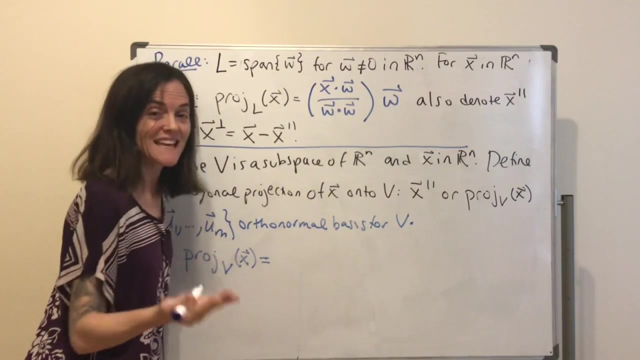 W dot W is 1, and all we would see is X dot W times W. That would be if it was unit. Well, this is what we will see here. So, generally right to get an element of this subspace V, I need a linear combination of these basis vectors. 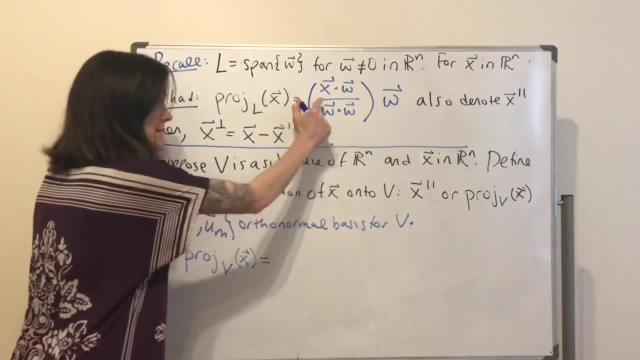 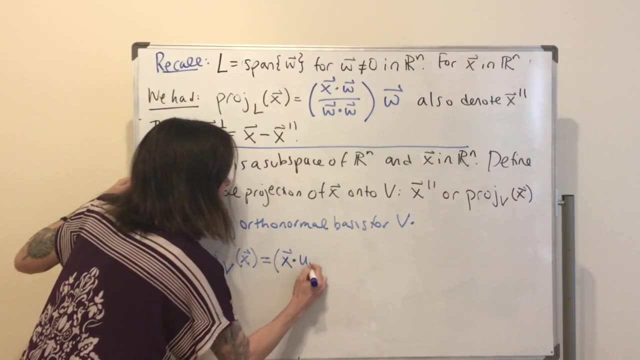 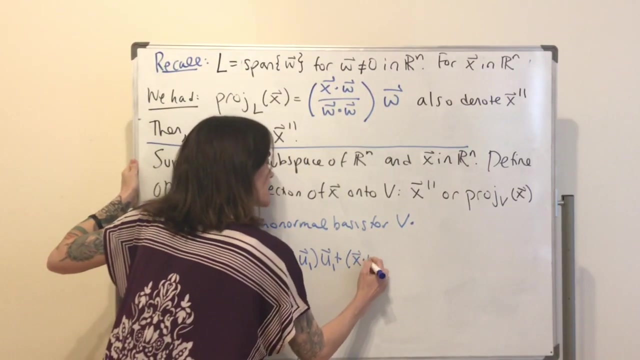 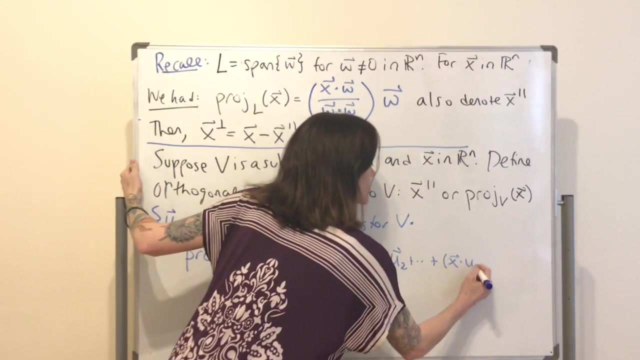 and the coefficient in front of each vector looks like this: except understanding that each UI is unit, So it will be X dot U1.. This is the coefficient times U1 plus X Dot U2,. this is the coefficient times U2, all the way out to X dot UM. 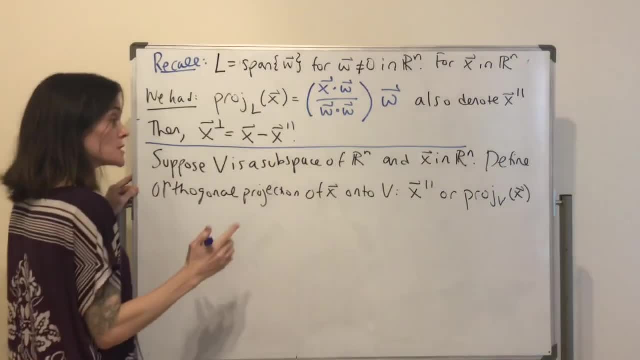 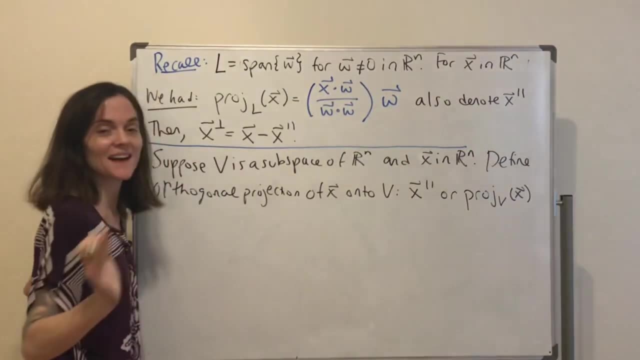 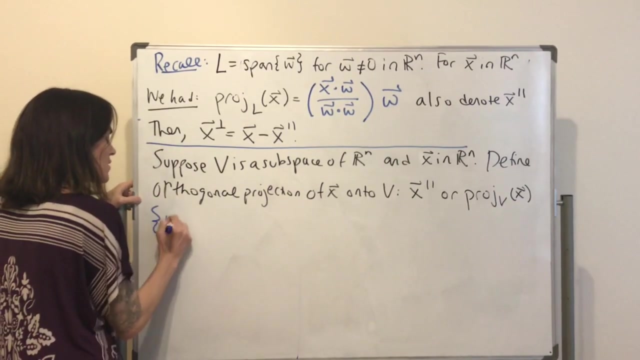 mentioned this was a vector in the subspace. once we project it, uh-oh well, i'm not ready to define it yet. so what i need to define this orthogonal projection is: i need an orthonormal basis for v. so so let's take u1 out to um orthonormal. 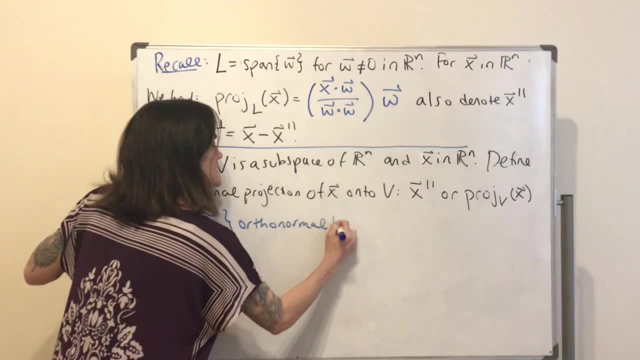 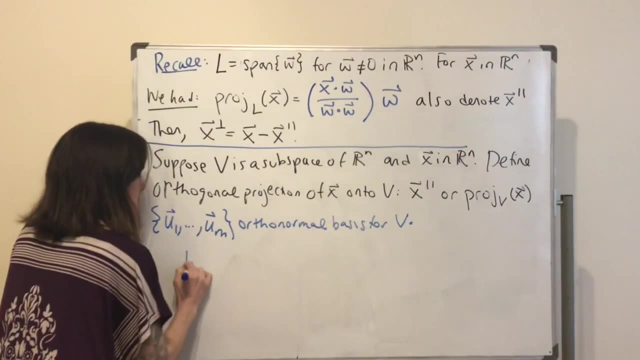 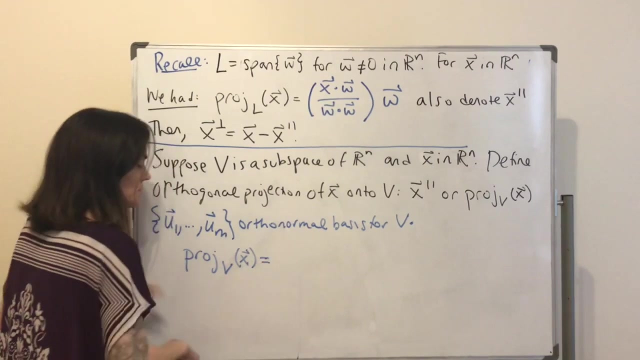 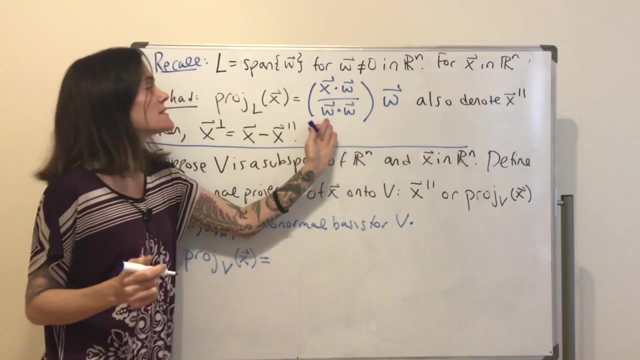 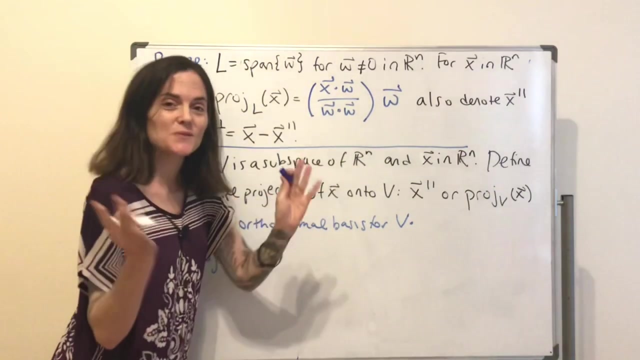 basis for v, and now i can define this. the projection is equal to: okay, it's going to look just like this. now, what would this formula- and we even discuss this- if, in fact, w was a unit vector, as all of these are, ww is one and all we would see. 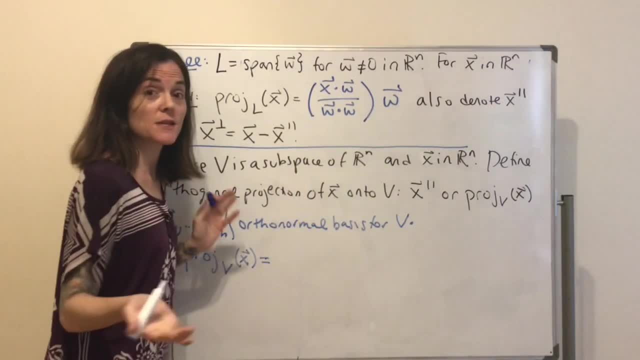 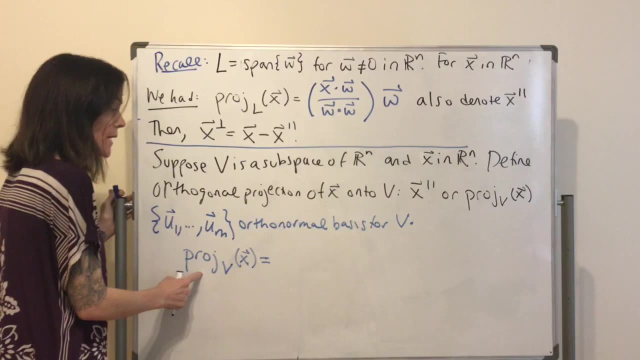 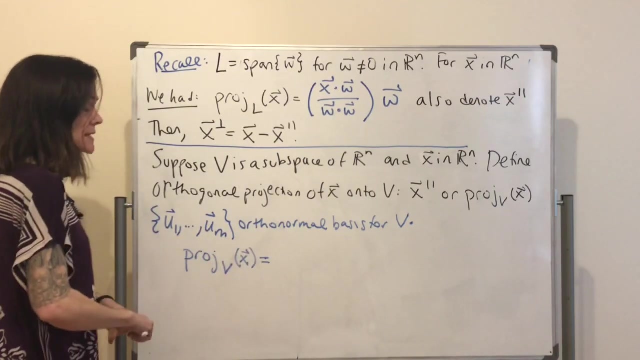 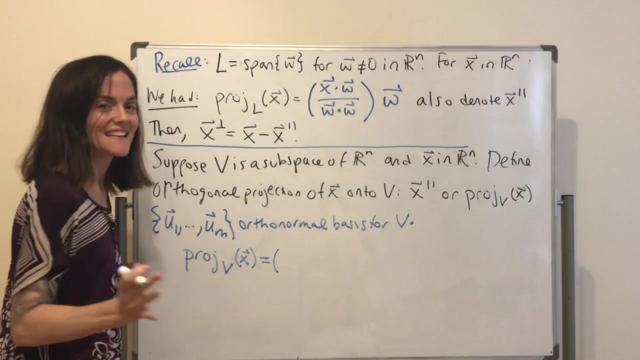 is xw times w. that would be if it was unit. well, this is what we will see here. you So generally right to get an element of this subspace V. I need a linear combination of these basis vectors, and the coefficient in front of each vector looks like this: except understanding that each UI is unit. 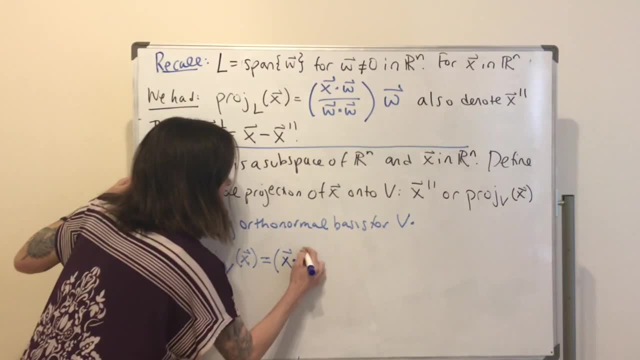 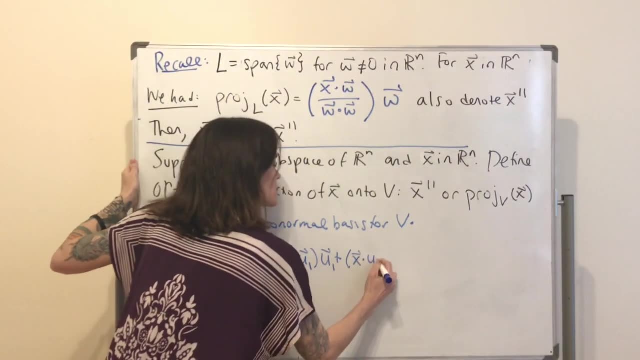 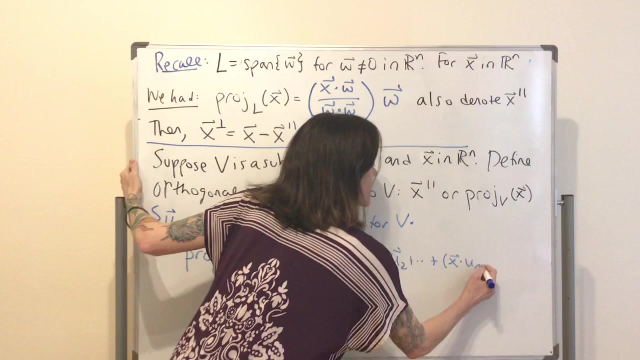 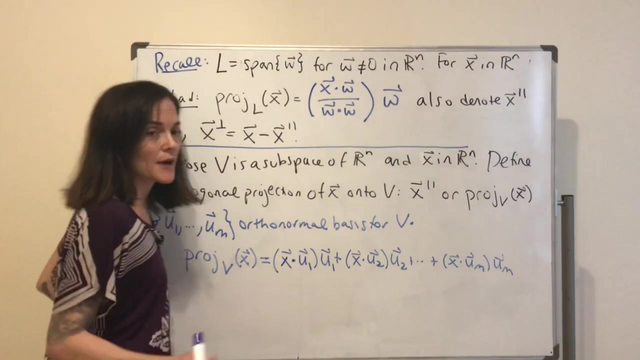 So it will be X dot U1, this is the coefficient times U1, plus X dot U2, this is the coefficient times U2, all the way out to X dot UM. this is the coefficient times UM. And you see, this projection is a linear combination of the basis vectors for V. this linear combination is in V. 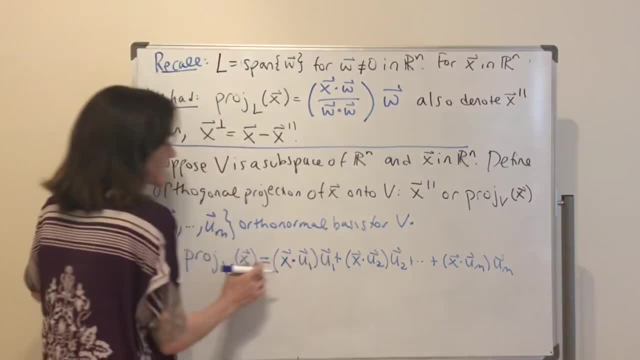 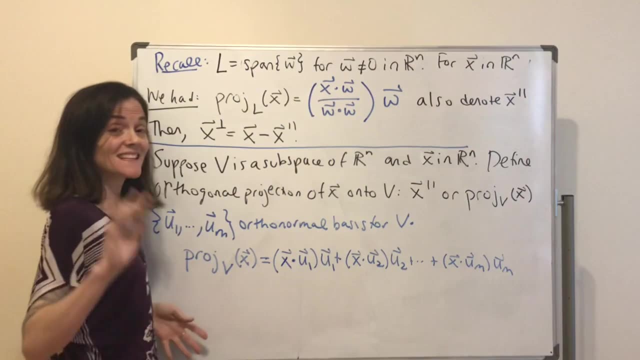 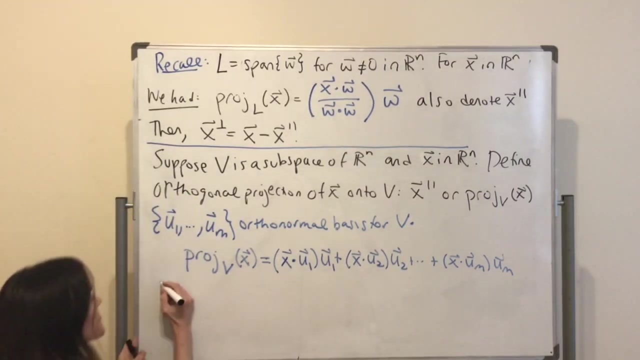 This is the coefficient times UM And you see, this projection is a linear combination of the basis vectors for V. This linear combination is in V And then we also have We also have This. so if this is this notation, okay, which is X minus the orthogonal projection. 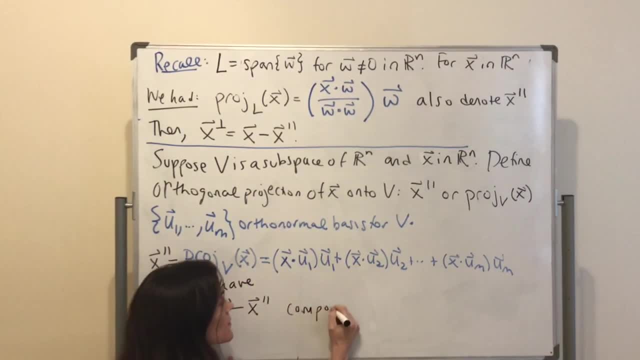 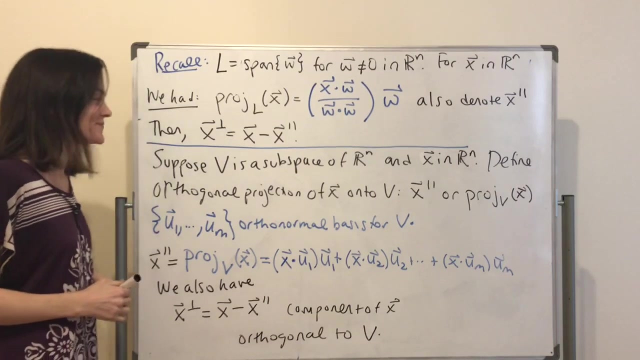 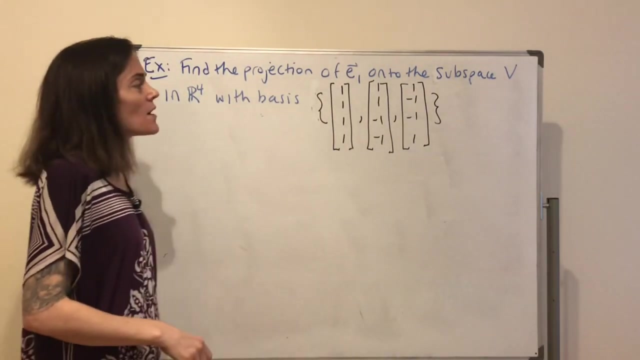 And this will be the component of X, which is orthogonal to the entire subspace. Okay, This is the orthogonal projection. Find the projection of E1 onto the subspace with this basis. Well, we know, this subspace is three-dimensional. 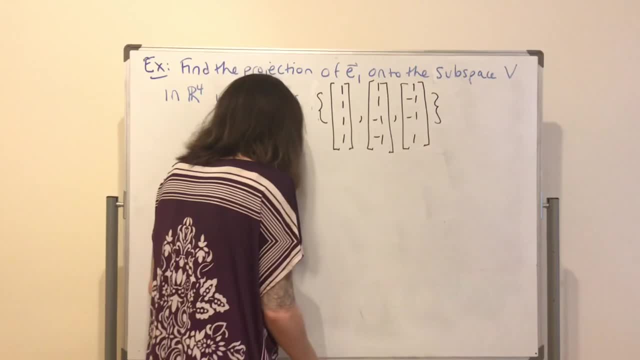 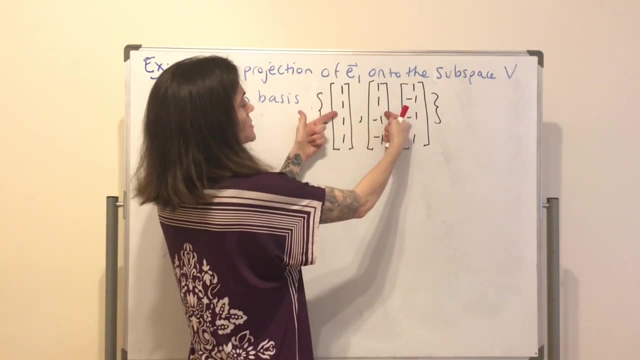 For example, we have three things And you notice just by looking at this that you can quickly take the dot product of these two. you get zero. The dot product of these two, you get zero. And then the dot product of these two, you get zero. 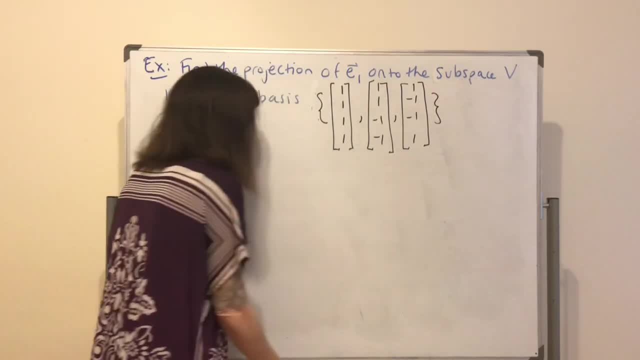 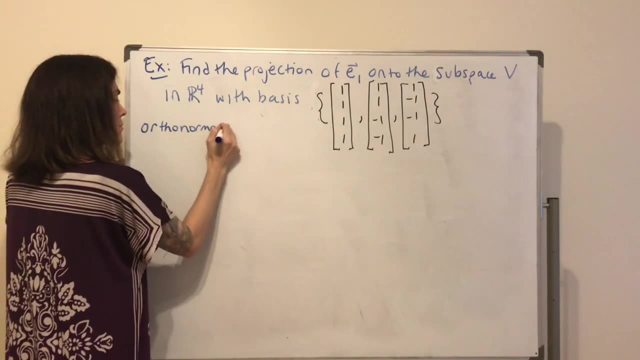 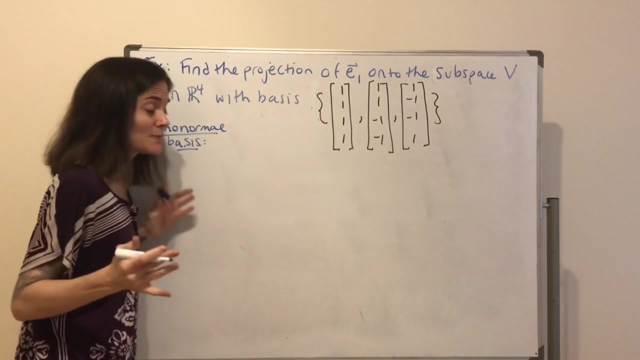 So these are orthogonal. But then to get an orthonormal basis We have to go one more step. This is what we need to start with the orthonormal basis. This is kind of like we did before I defined the orthogonal projection. 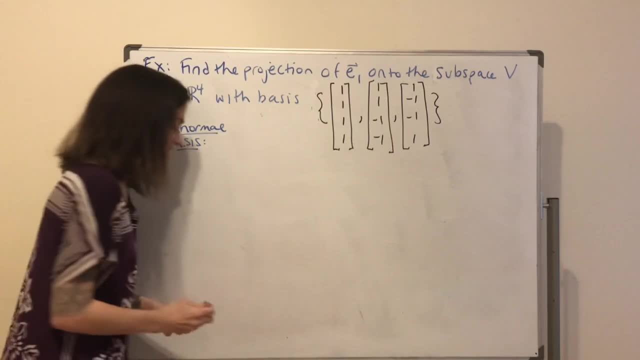 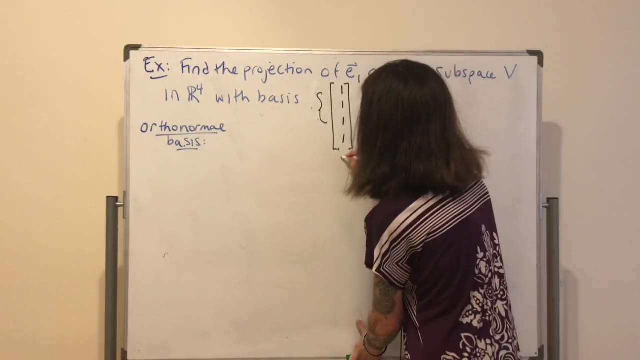 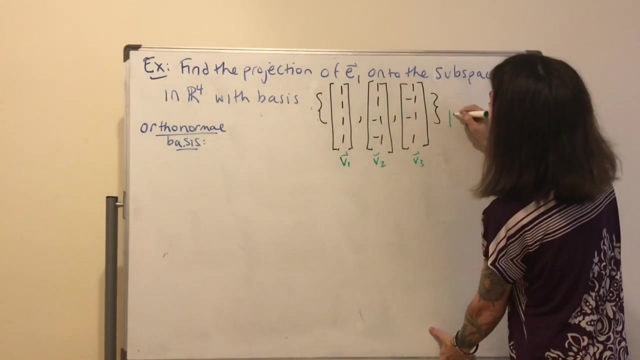 We need to take these three vectors and normalize them. Well, the thing is, they all have the same length. So if I called this, say, V1, V2.. V2, V3. All of these have the same length. 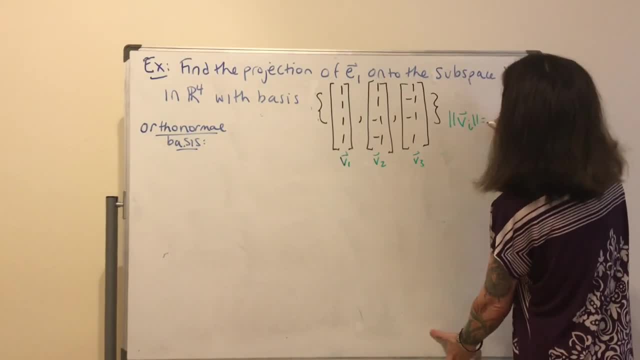 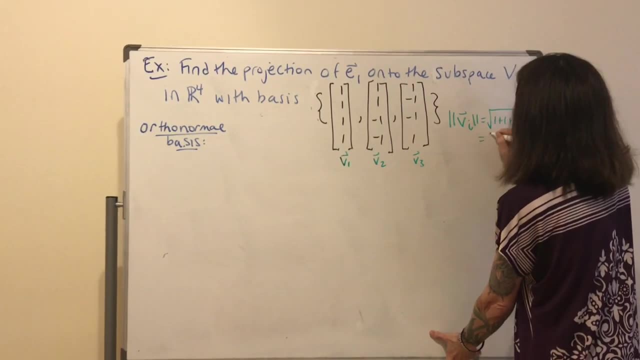 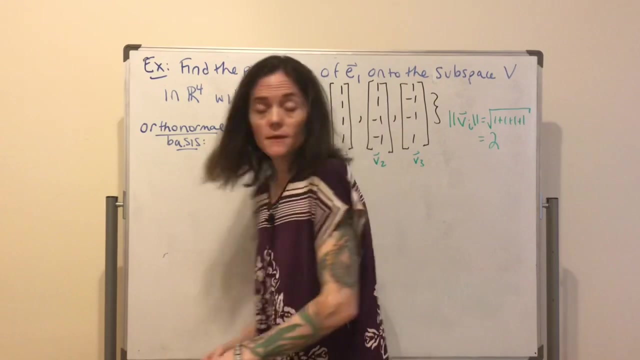 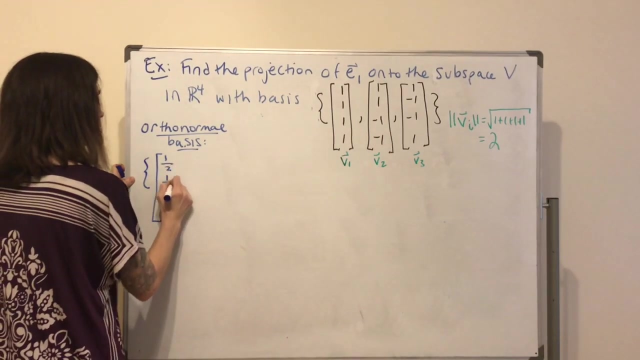 The length of VI is the square root of 1 plus 1 plus 1.. Which is the square root of 4 or 2.. So all I need to do to get an orthonormal basis is Divide every single entry I see by: 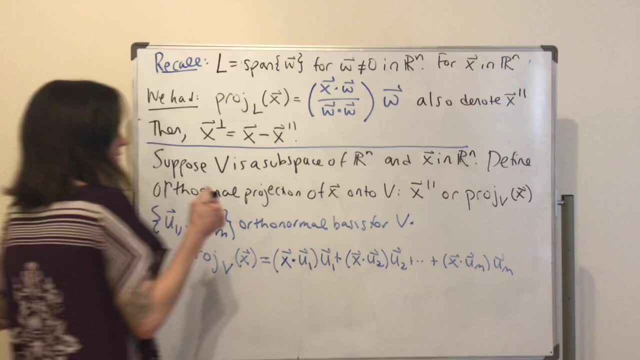 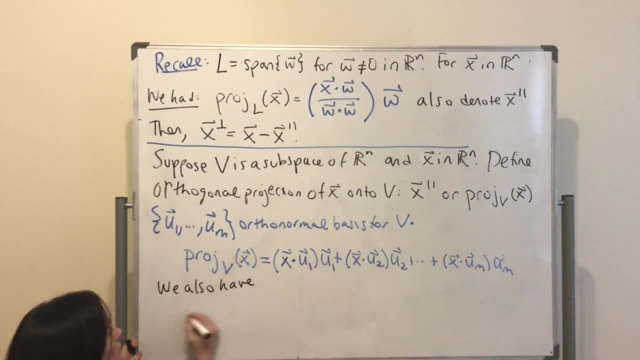 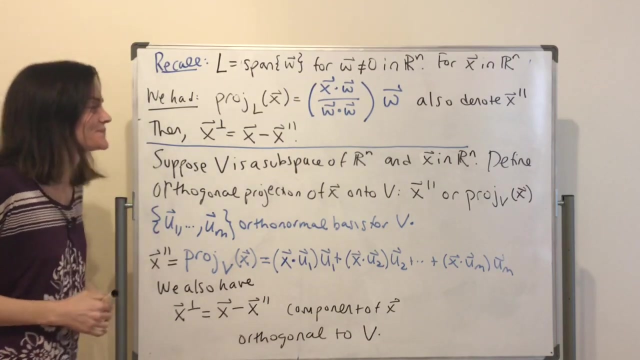 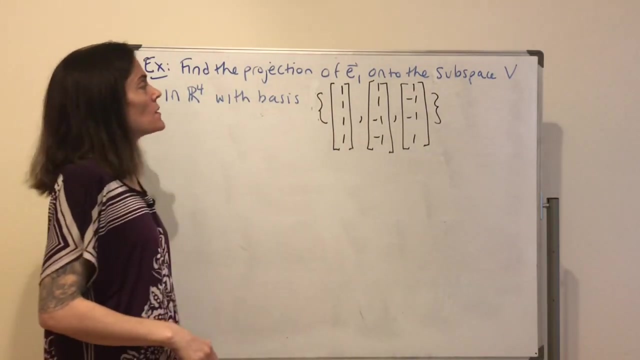 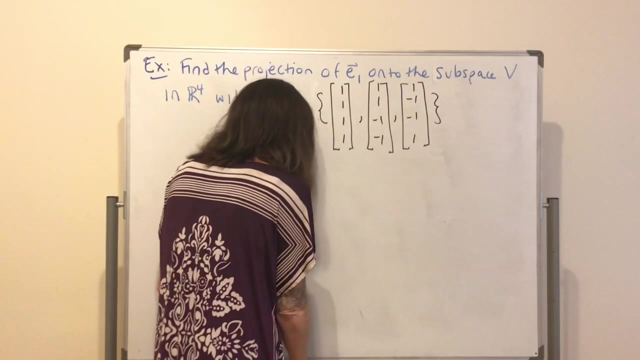 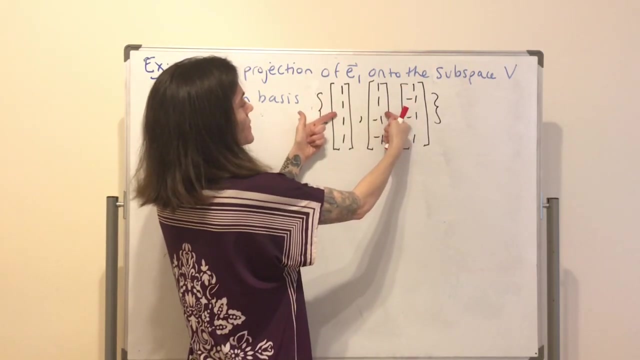 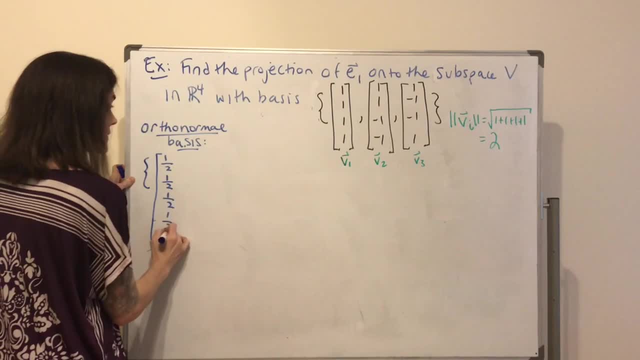 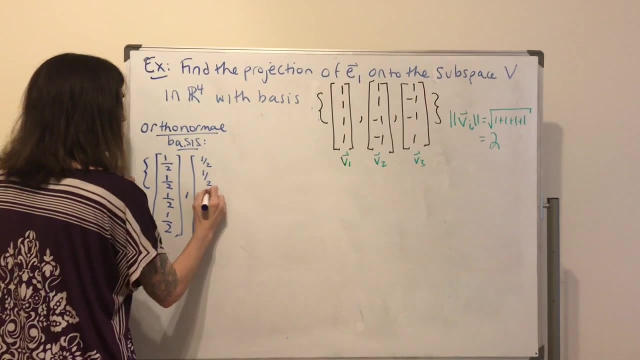 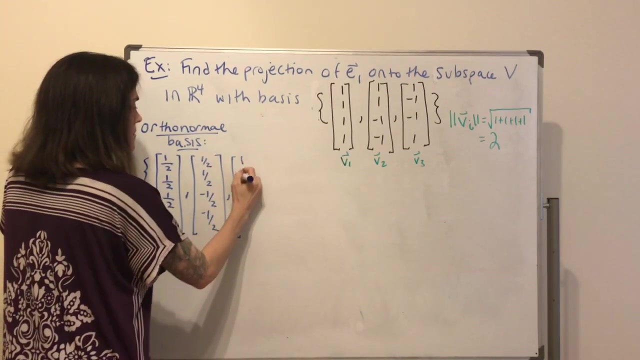 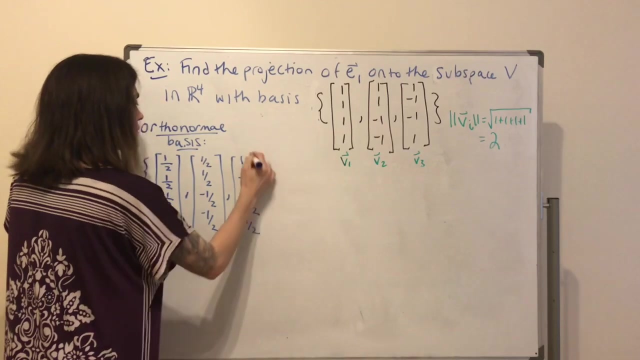 2. Because they all have the same length. So here's the first element of my orthonormal basis, Here's the second And here is the third. Okay, So far, so good. Now let's project E1.. 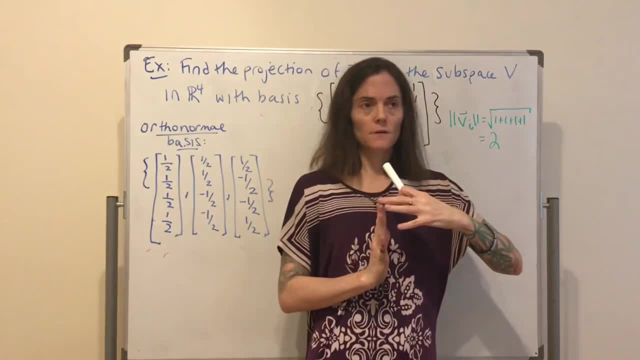 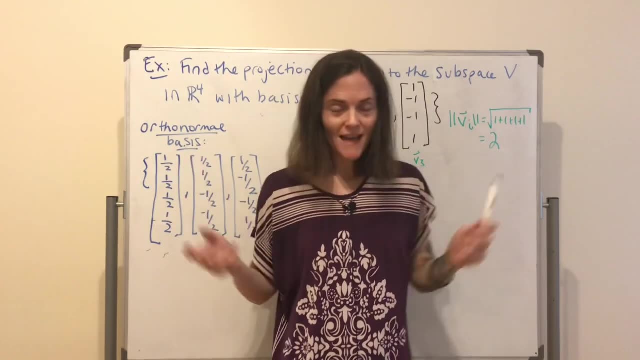 And I will find this other part, which is the component of E1.. That's the orthogonal to the subspace And we'll check, just as a first example. We'll check that in fact it should be orthogonal to the subspace. 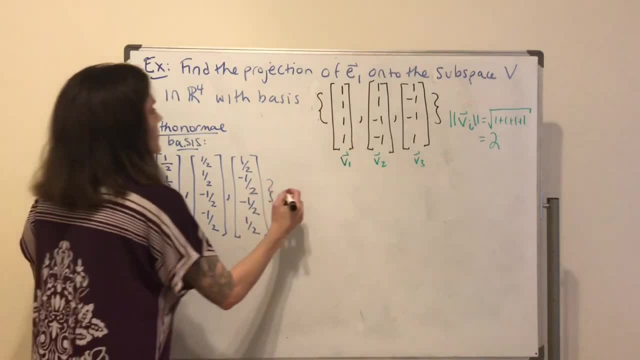 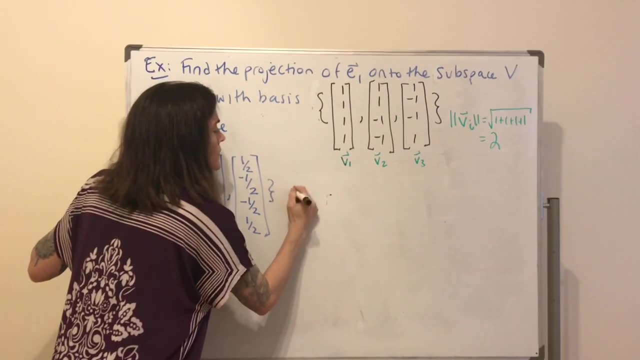 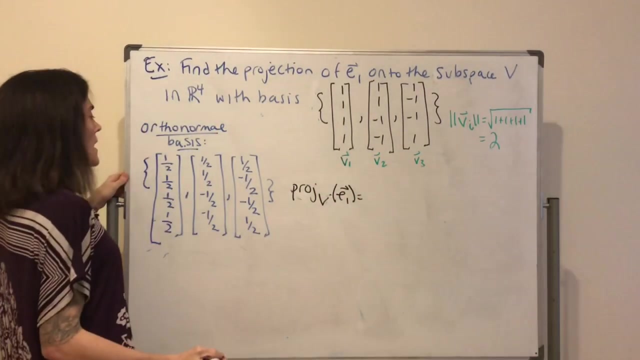 I'll make a comment on that when we get there. Okay, So if we want this, Oh, E1.. I know the vector. I'm doing it to The projection Onto the subspace of E1.. Well, I take E1.. 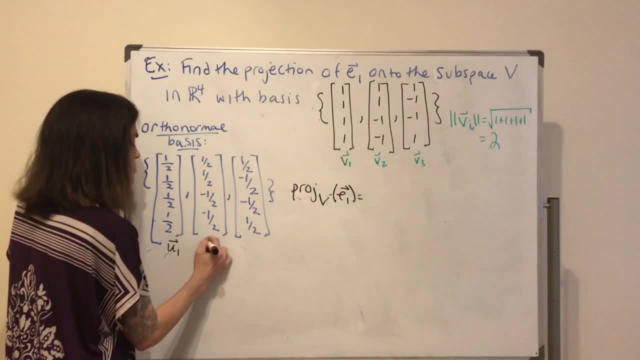 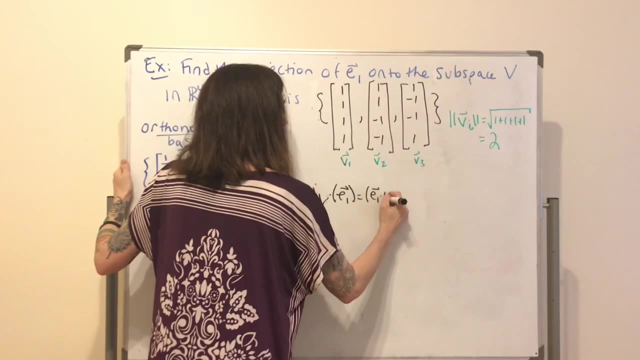 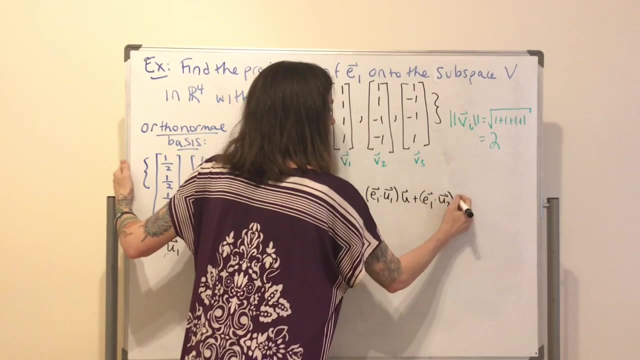 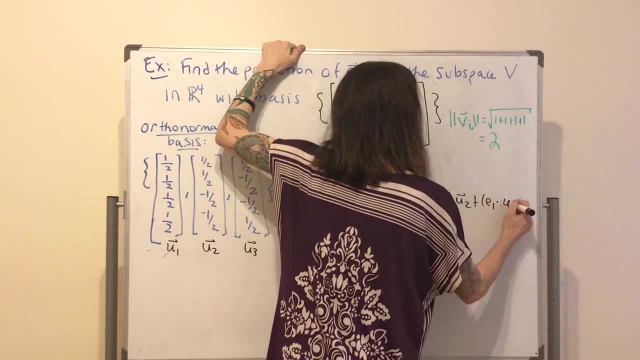 Now this will be my U1. U2. U3. E1.U1. U1. Plus E1.U2. U2. Plus E1.U1. U2.U3. U3.U3. U2.U3. 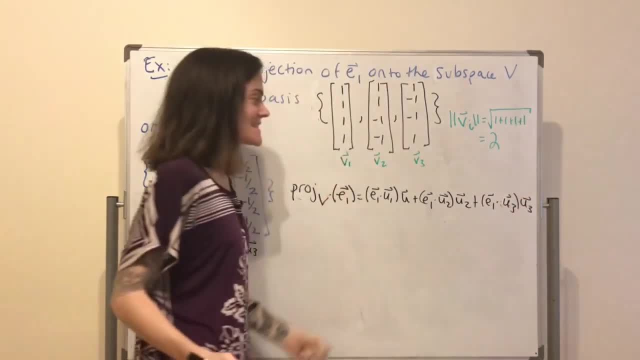 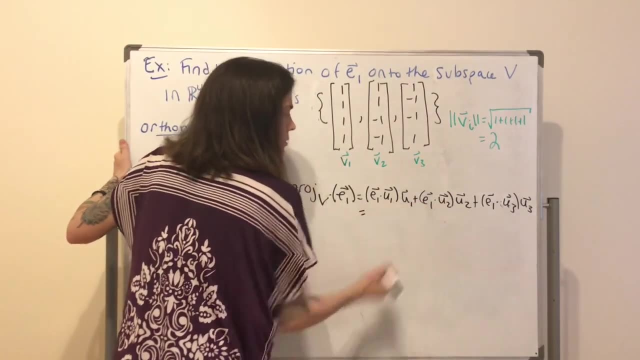 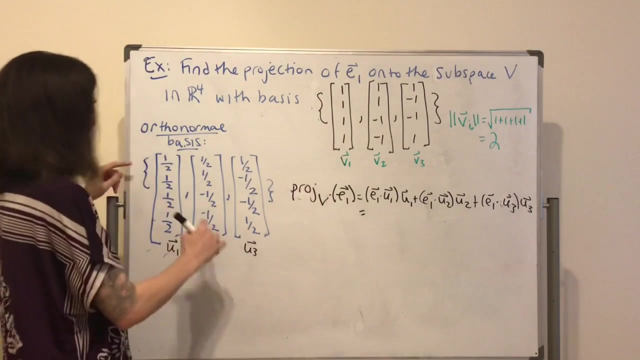 U2.U3.. U2.U3.. U2.U3.. This is orthogonal projection. Okay, And then now we just need to compute some dot products and put, uh, oh, U1.. Put the appropriate vectors there. E1 is the vector with one, with zeros everywhere else. 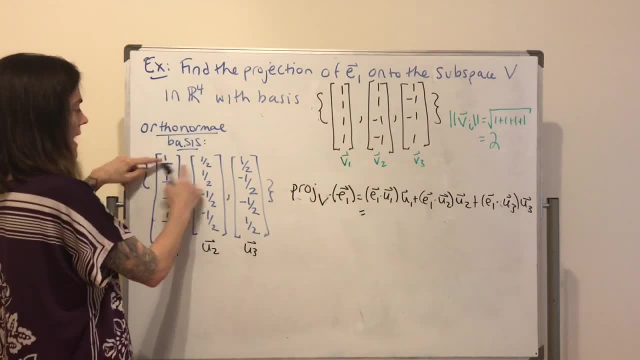 So you dot product with any one of these: E1.this is a half, E1.this is a half And E1.this is a half. So this is going to be a half, And E1.this is a half, So this is going to be a half. 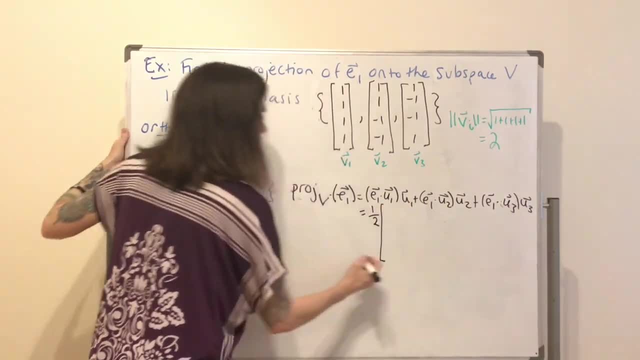 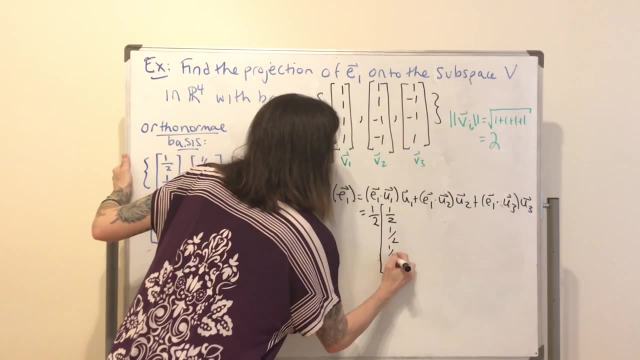 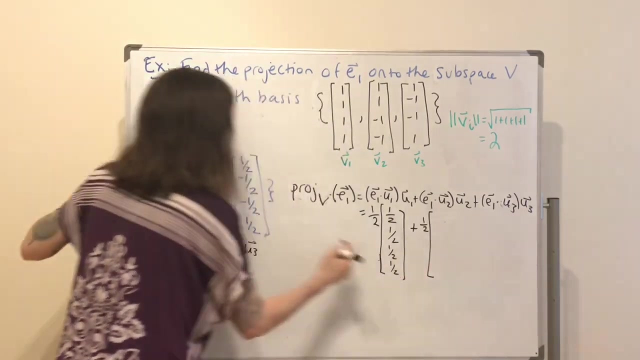 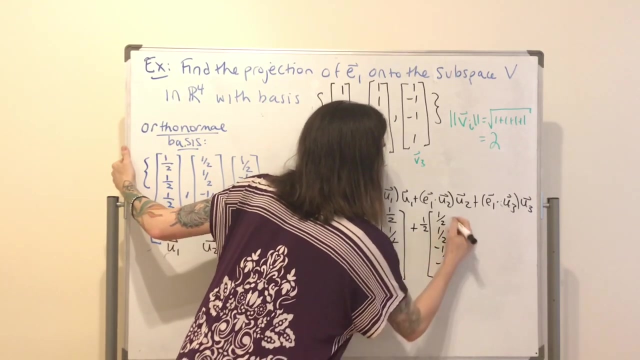 And E1.this is a half, And then I put U1 here, which is all of halves Okay, And then this is another half, E1.U2.. And then one half, one half minus a half, minus a half. 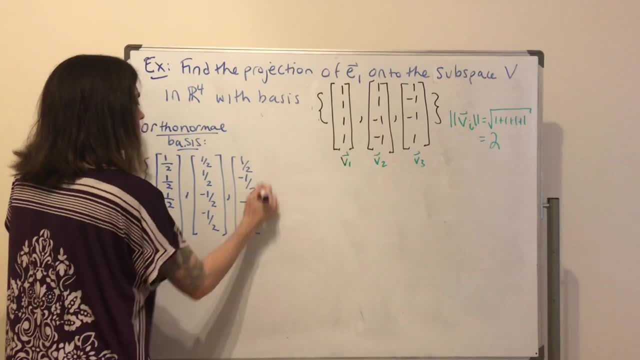 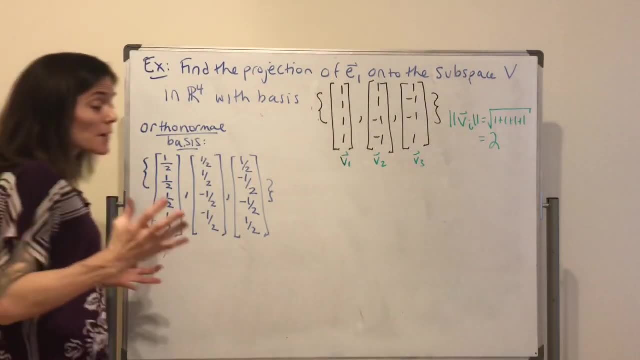 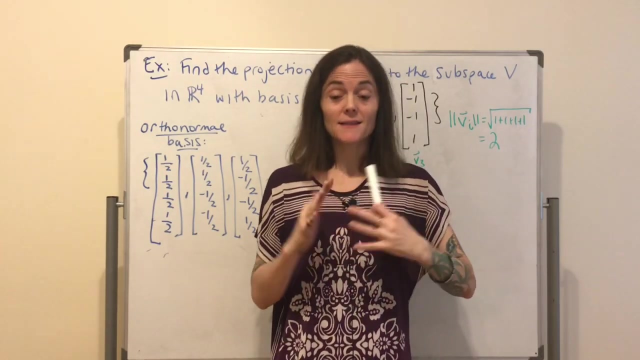 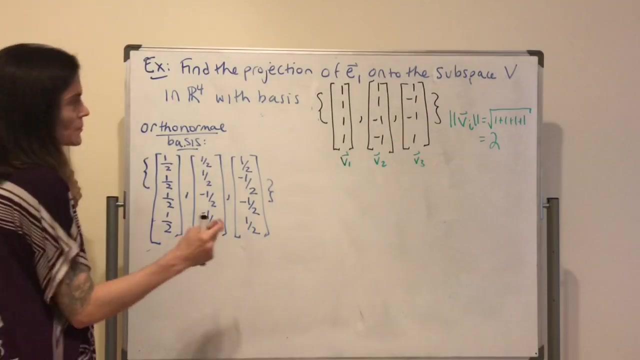 Okay, so far, so good. Now let's project e1. And I will find this other part, which is the component of e1, let's say orthogonal to the subspace, And we'll check. just as a first example, we'll check that in fact it should be orthogonal. 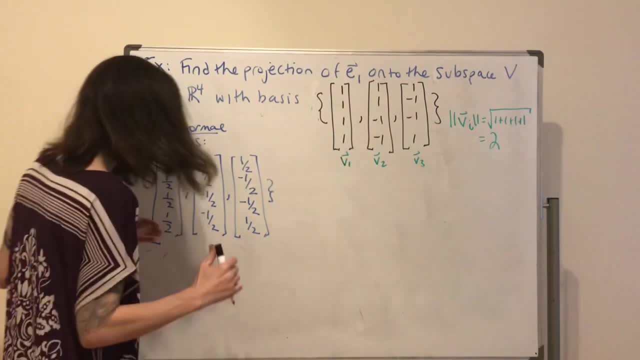 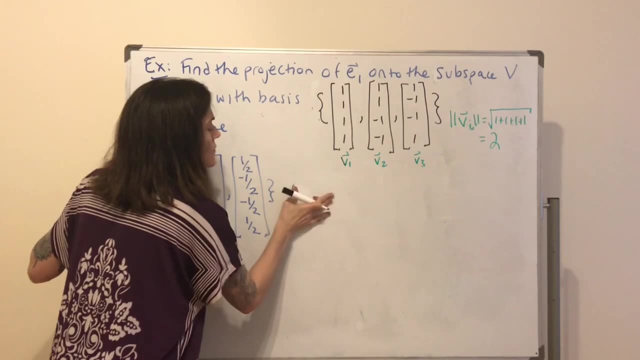 to the subspace. I'll make a comment on that when we get there. Okay, Okay, Okay, Okay. so if we want this, oh, E1.. I know the vector, I'm doing it to The projection onto the subspace of E1.. 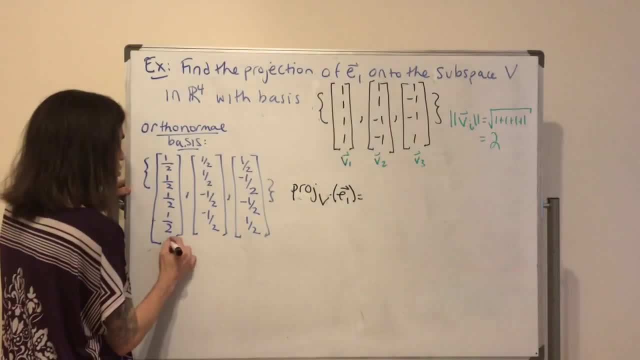 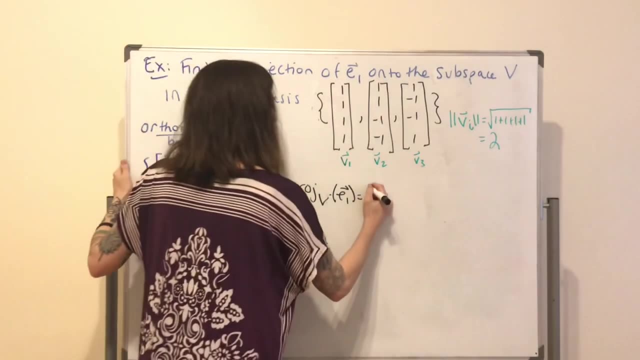 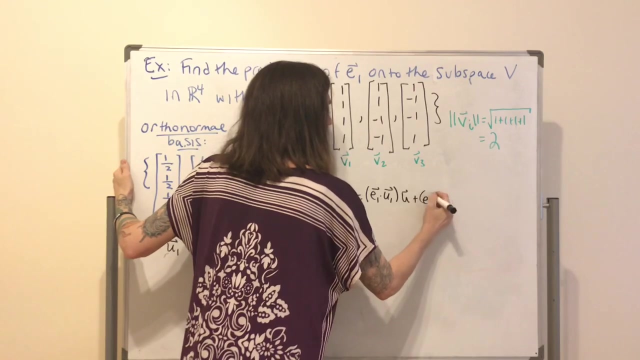 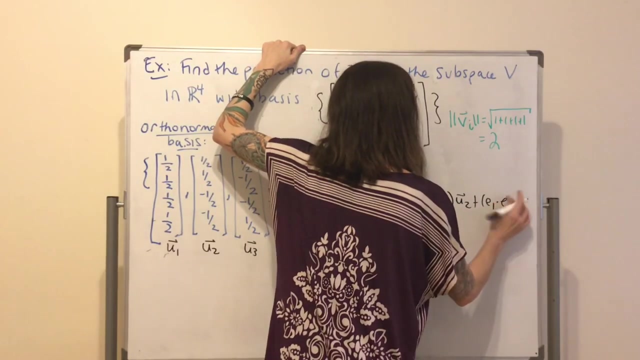 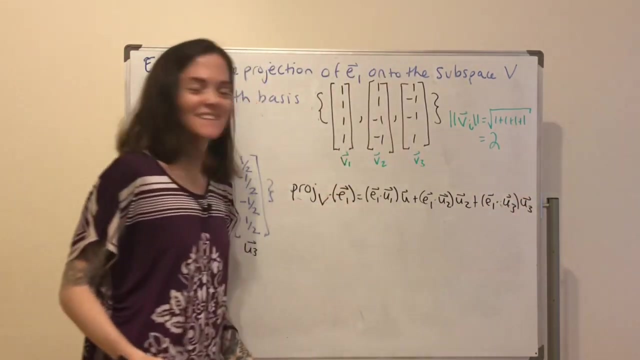 Well, I take E1.. Now this will be my U1, U2, U3, E1.U1, U1, plus E1.U2, U2, plus E1.U3, U3.. This is orthodoxy. 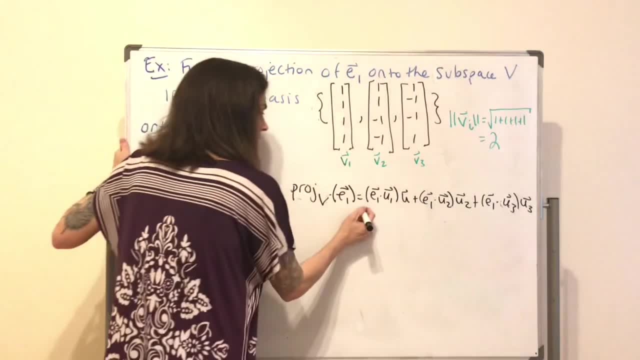 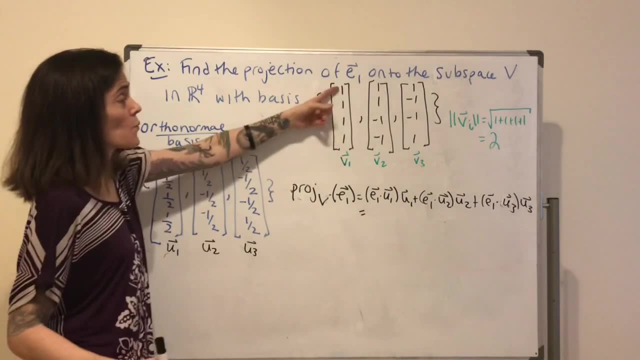 Diagonal projection. okay, And then now we just need to compute some dot products and put uh-oh, U1.. Put the appropriate vectors there. E1 is the vector with one, with zeros everywhere else. So you dot product with any one of these. 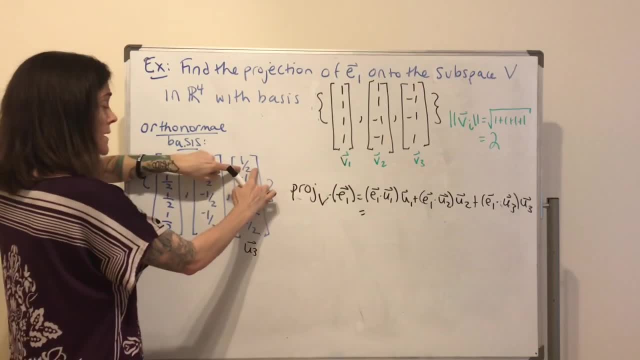 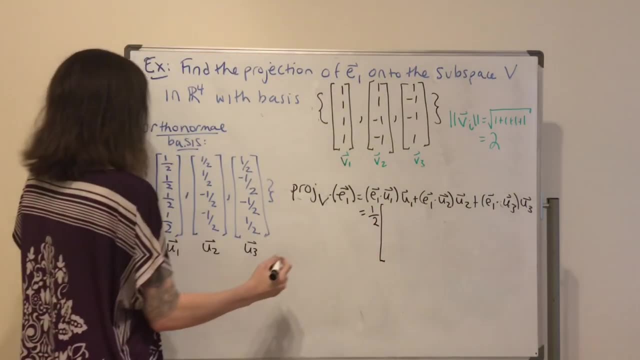 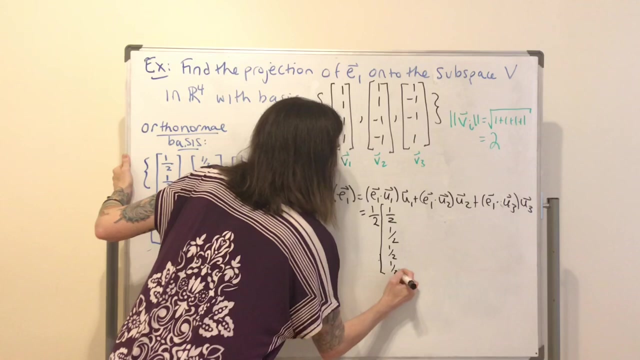 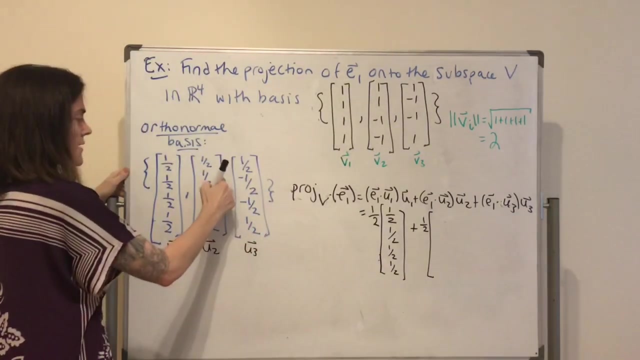 E1 dot- this is a half, E1 dot- this is a half, And E1 dot- this is a half. So this is going to be a half, And then I put U1 here, which is all a halves, Okay, and then this is another half: E1 dot, U2, and then one half, one half, minus a half, minus a half. 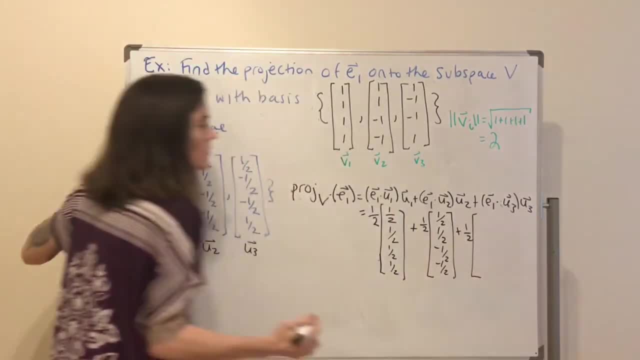 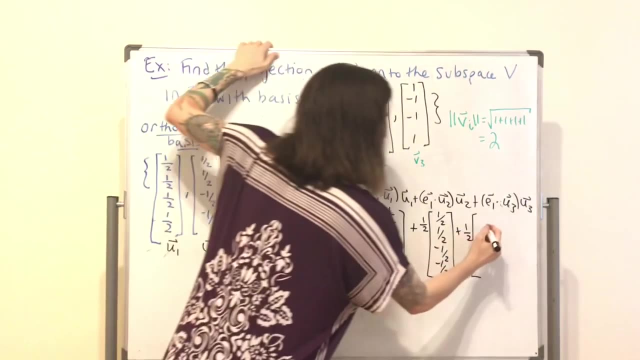 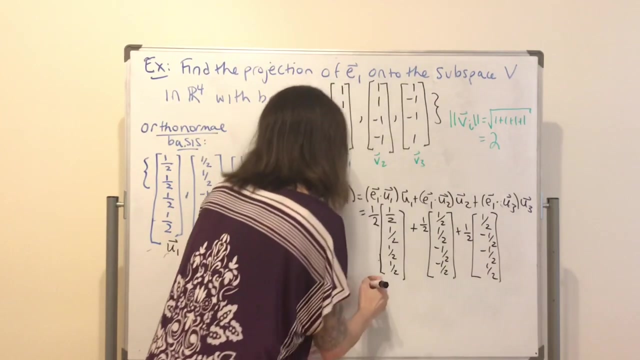 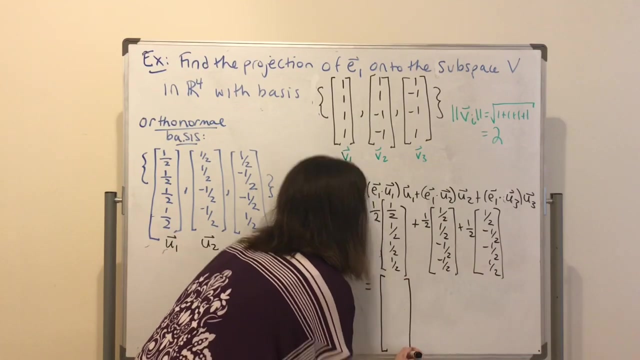 Finally, one half. Here it's going to be one half minus a half minus a half a half. Okay, now what happens when I add all of these together? This would be my final answer here: One, two, three-fourths. 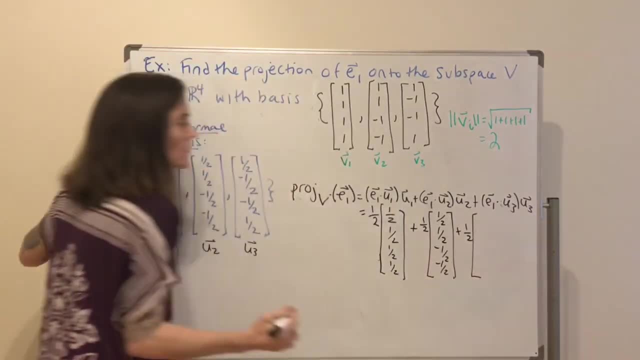 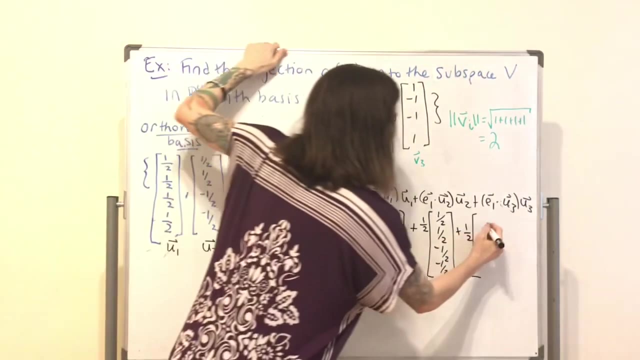 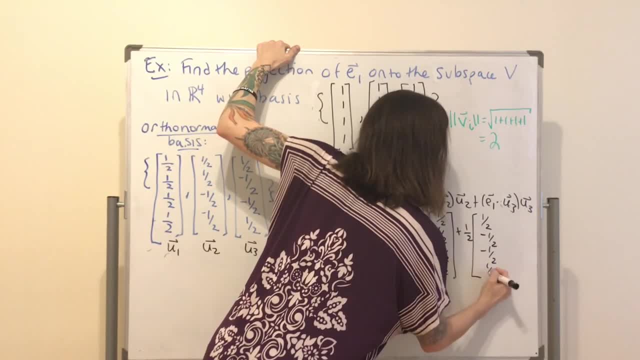 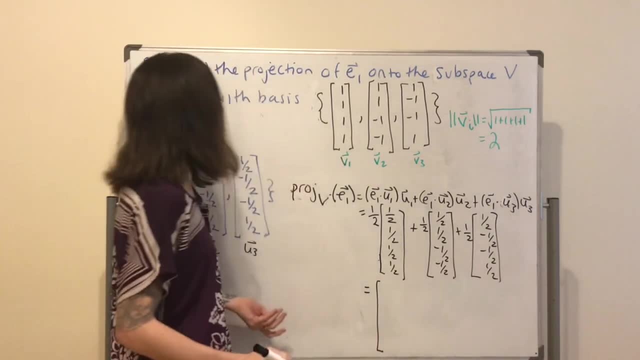 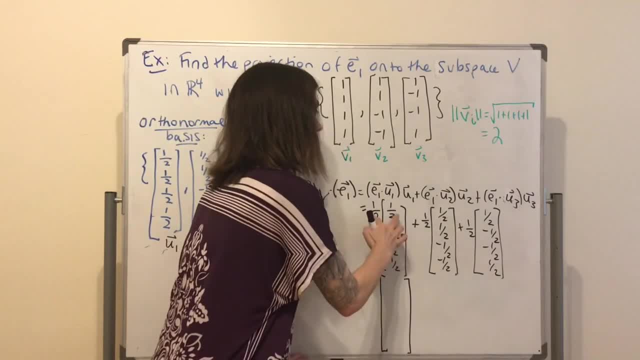 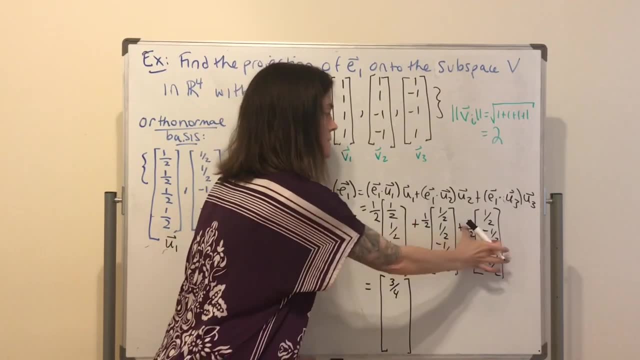 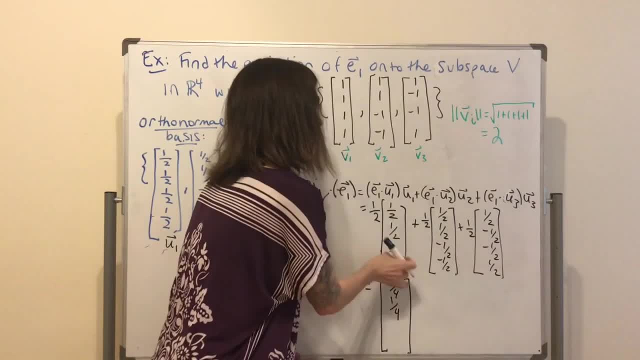 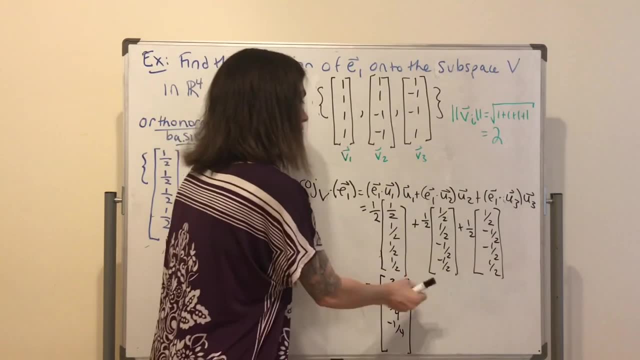 minus 1 4th is 1 4th. 1 4th minus 1 4th. and minus 1 4th is minus 1 4th. Oh, I wrote it out of space. And then 1 4th minus 1 4th plus 1 4th, this is 1 4th. 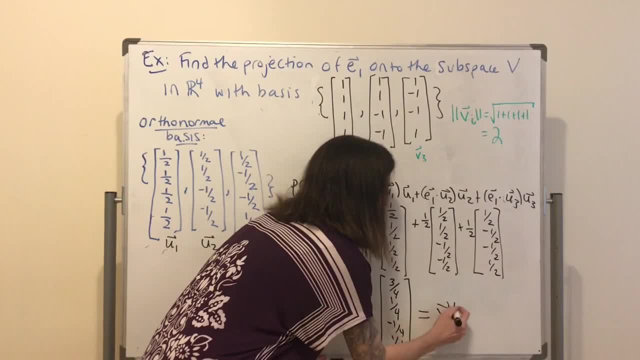 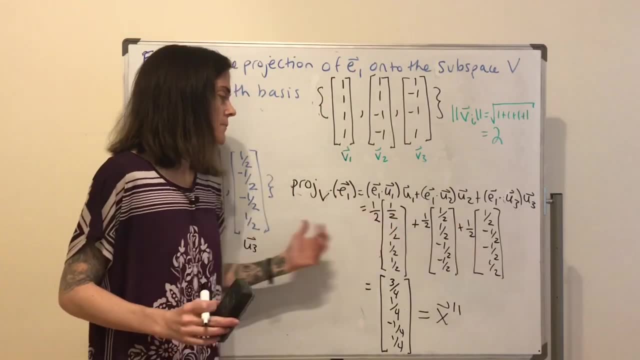 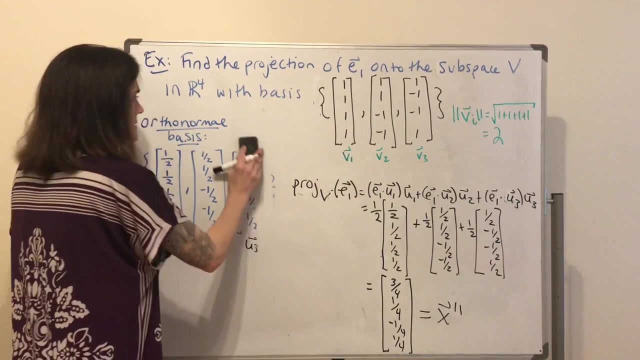 Okay, so this is my vector, like this, which lies in my subspace. Well, of course it does. It's a linear combination of these basis elements. Now, maybe I'll erase my orthonormal basis. I'll leave my original basis. 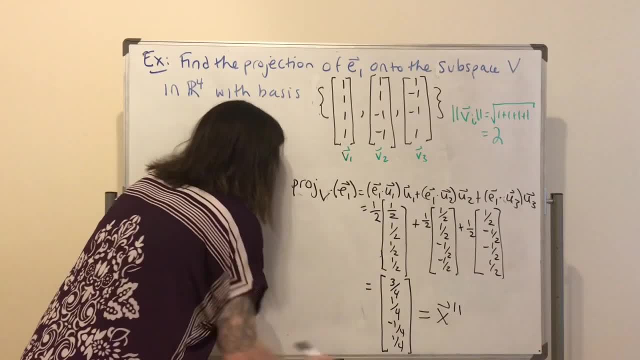 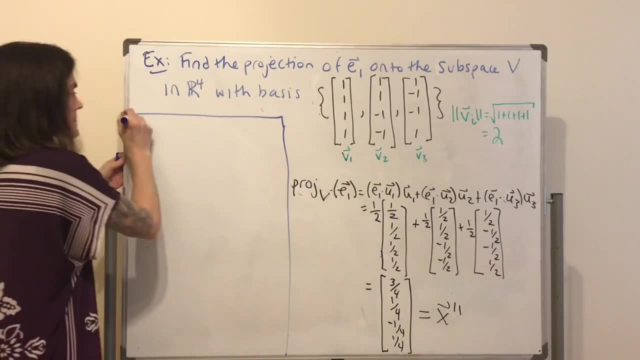 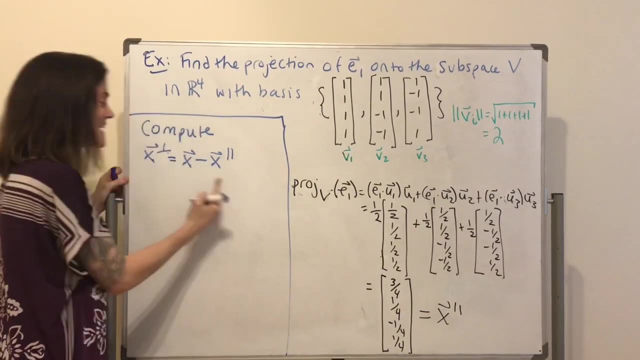 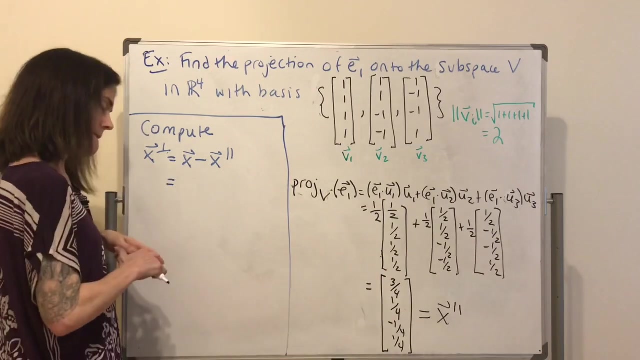 And just for this first example, let's compute, as I mentioned this one, This: You take x minus the orthogonal projection, and it's this, And this should be perpendicular, Orthogonal, Orthogonal to the entire subspace. Well, here we go. 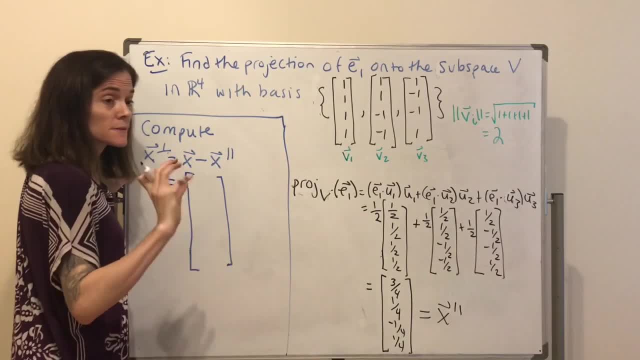 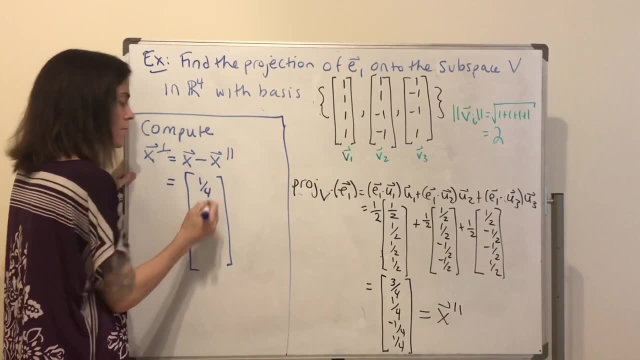 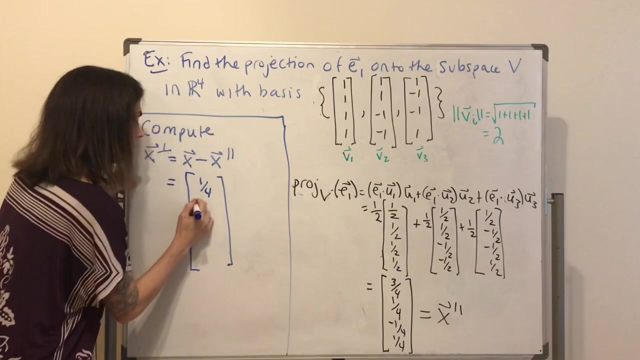 This is a 1 in the first location. 0 is everywhere else. So I take 1 minus 3 4ths, I have 1 4th, But then there's 0s everywhere else. So the other entries of this difference are just negative. what we see here: 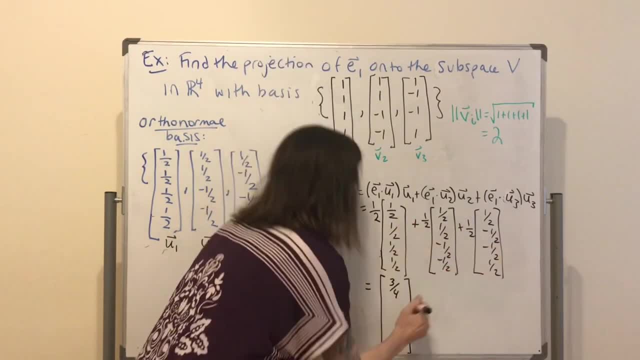 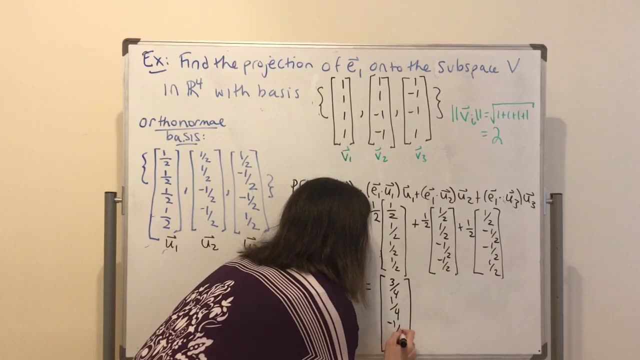 Then I have a fourth. two-fourths minus a fourth is one-fourth. One-fourth minus a fourth, and minus a fourth is minus a fourth. Uh-oh, I run out of space. And then a fourth minus a fourth plus a fourth: this is one-fourth. 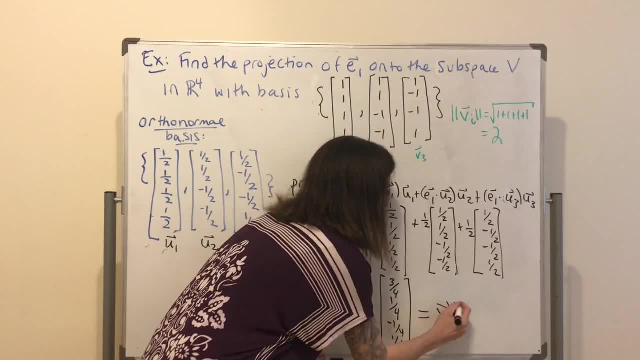 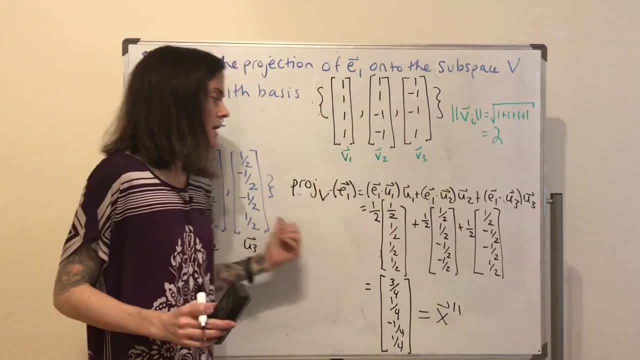 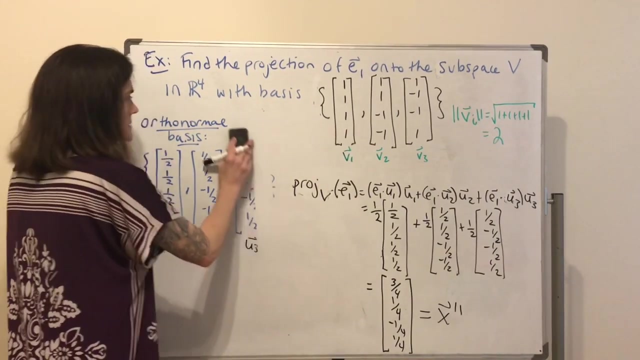 Okay, so this is my vector, like this, which lies in my subspace. Well, of course it does. It's a linear combination of these basis elements. Now, maybe I'll erase my orthonormal basis. I'll leave my original basis. 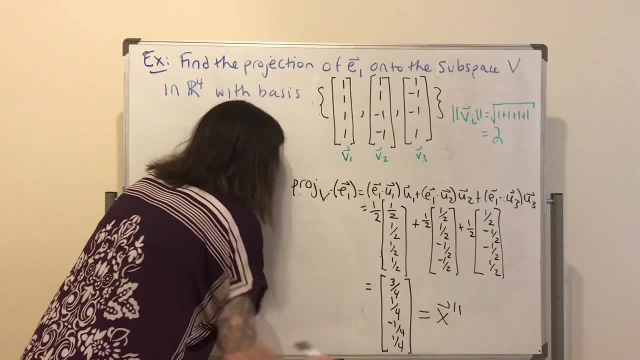 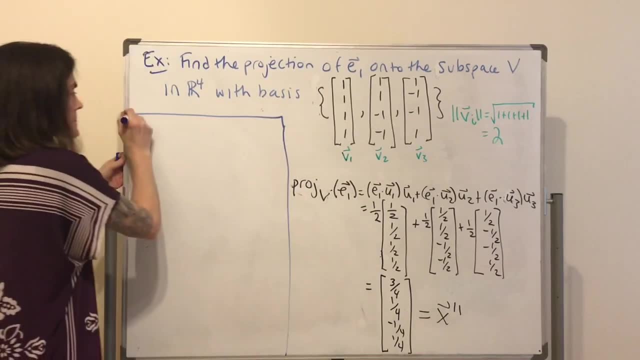 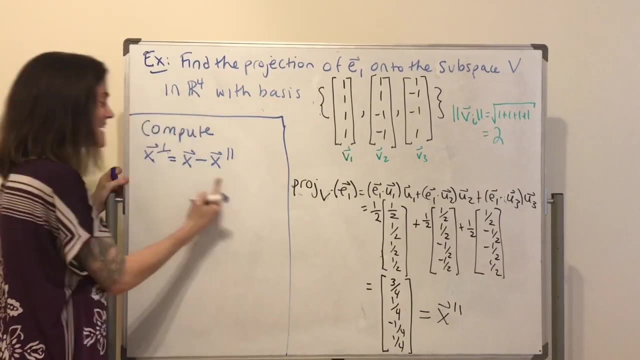 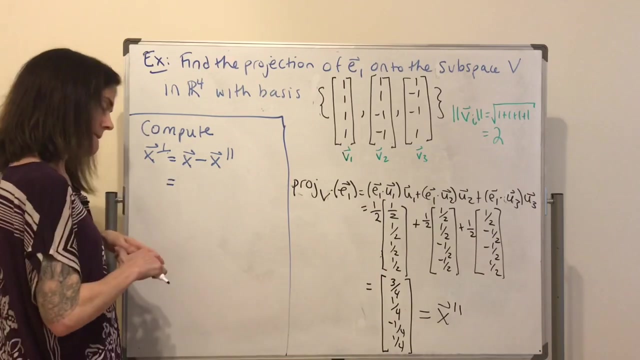 And just for this first example, let's compute, as I mentioned this one, This: You take x minus the orthogonal projection, and it's this: And this should be perpendicular, orthogonal to the entire subspace. Well, here we go. 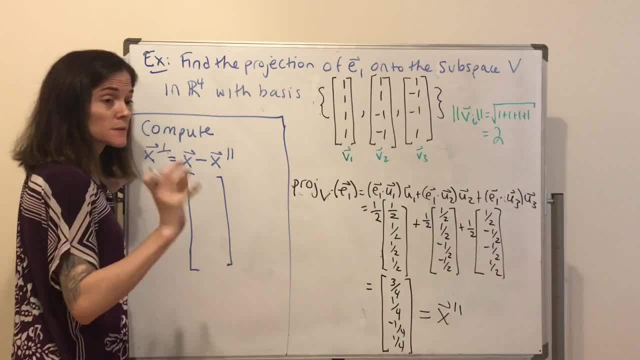 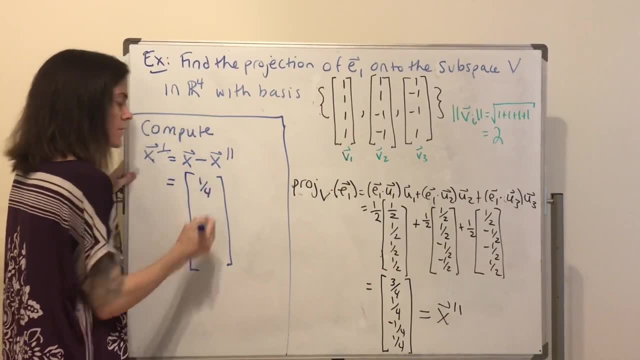 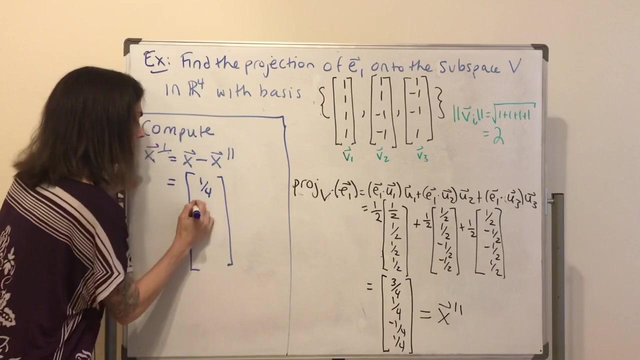 This. It's a one in the first location, zeroes everywhere else. So I take one minus three-fourths. I have one-fourth, But then there's zeroes everywhere else. so the other entries of this difference are just negative. what we see here: 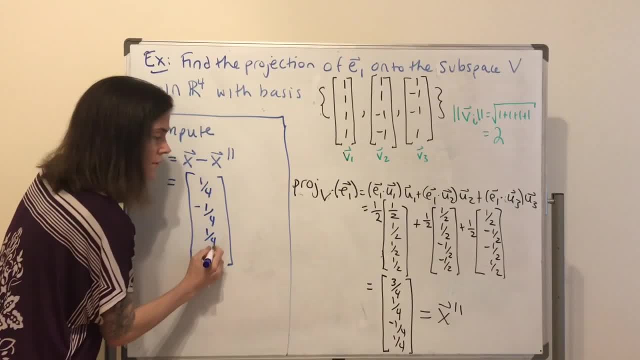 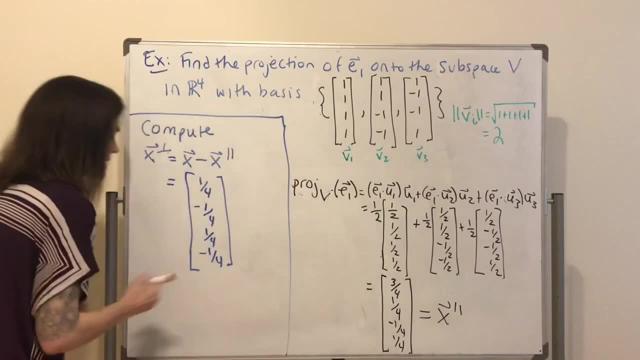 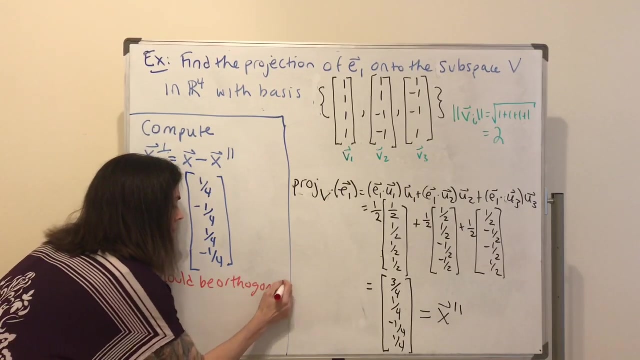 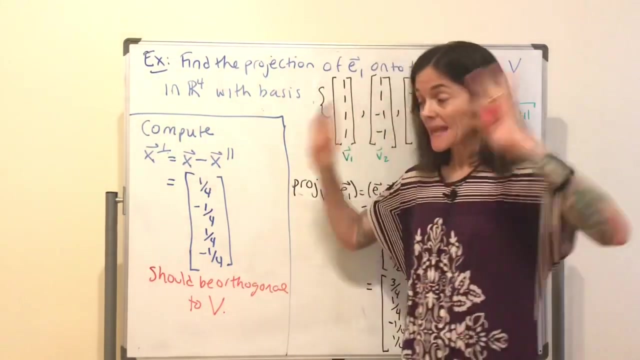 Negative a fourth, positive a fourth and negative a fourth. Okay Now, this is an important observation: This should be orthogonal to v, the whole subspace, which means we take any vector in the subspace v and we dot product with this one and we get zero. 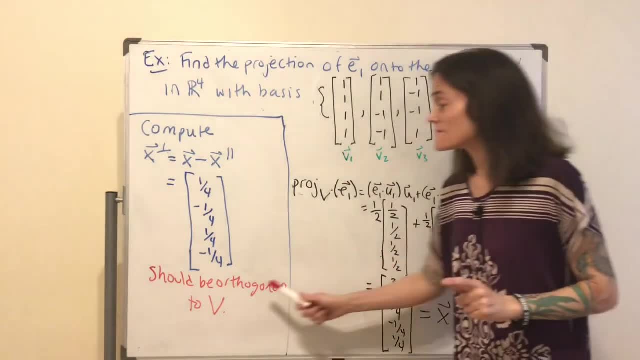 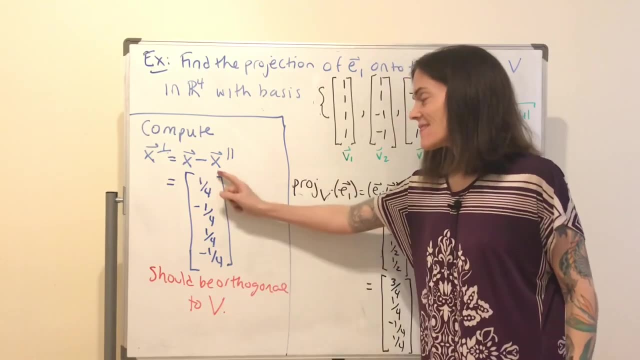 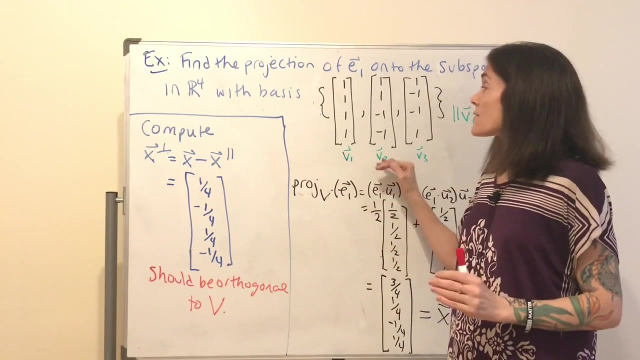 But really to verify this, or justify this or realize this- I should say any of those- we just need that this vector is orthogonal to each vector in a basis for v, Because, well, every vector in v may be written as a linear combination of the basis vectors. 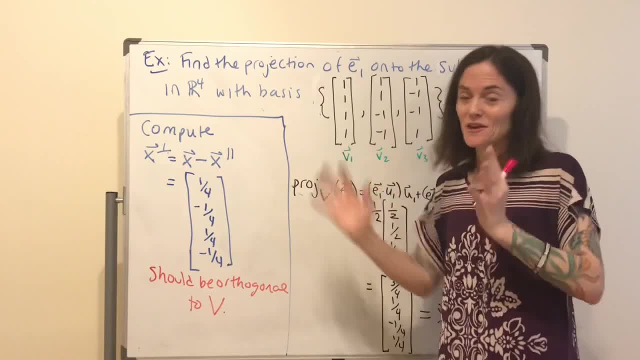 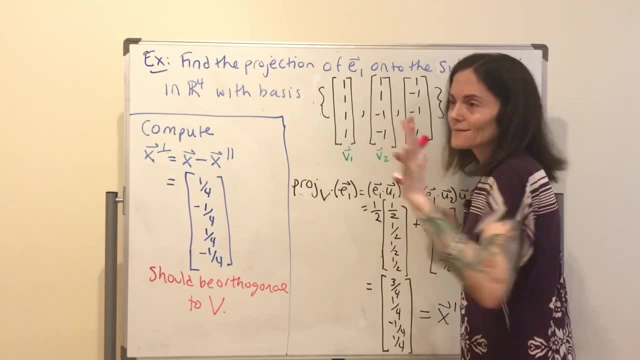 And if you take the dot product with a linear combination, it would be you could write it in terms of dot products with these With, well, some coefficients, But if these all dot to zero, then you would get zero for every single vector in v. 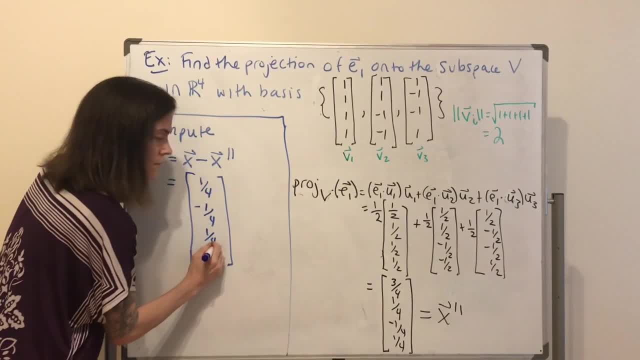 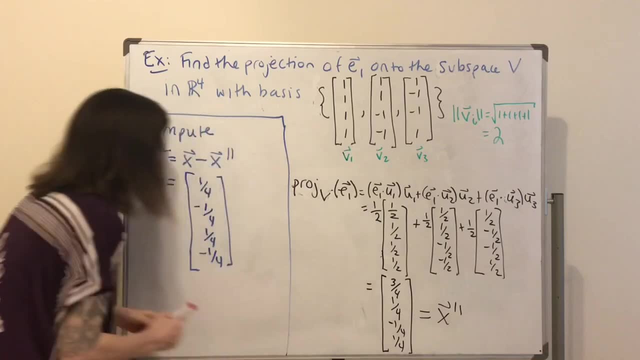 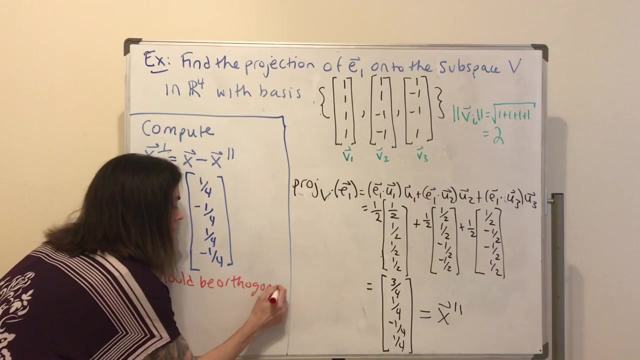 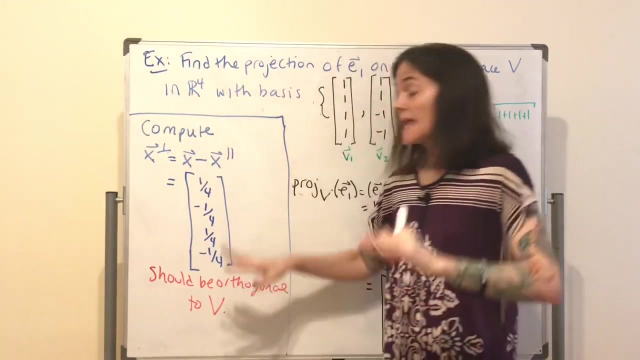 Negative of 4. 4th, positive of 4th and negative of 4th. Okay Now, this is an important observation: This should be orthogonal to V- The whole subspace, Which means we take any vector in the subspace, V. 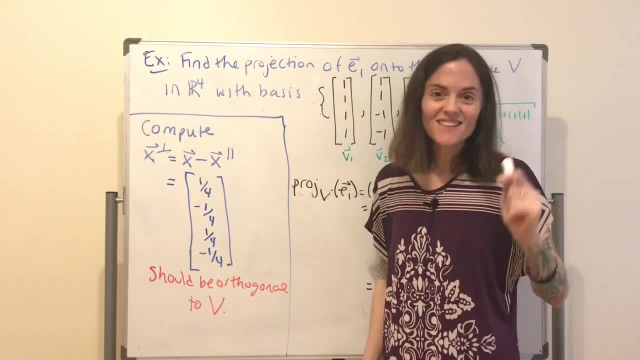 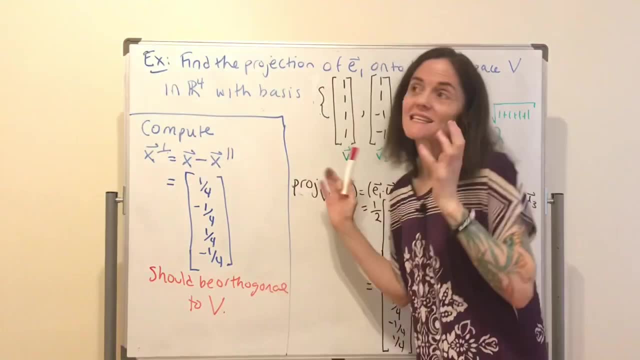 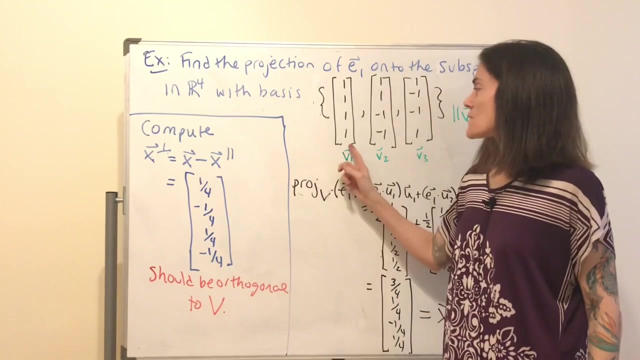 and we dot product with this one And we get 0.. But really to verify this, or justify this or realize this, I should say any of those- we just need that this vector is orthogonal to each vector in a basis for V. 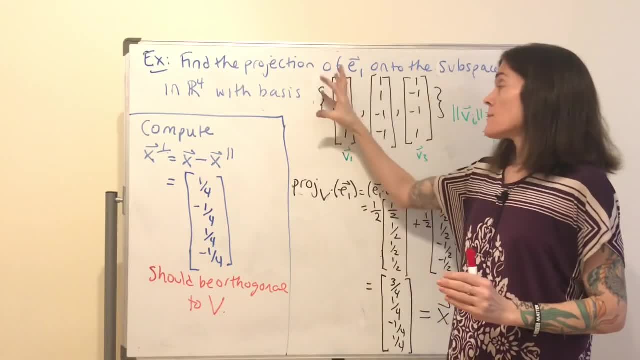 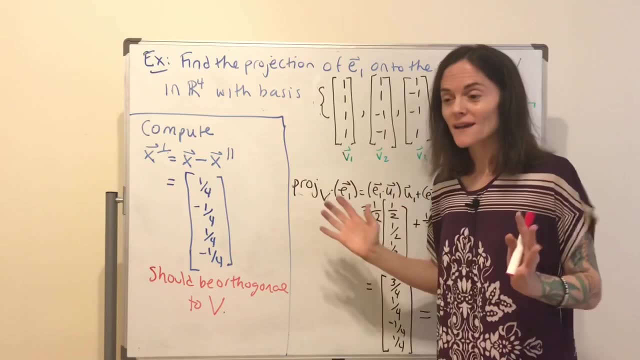 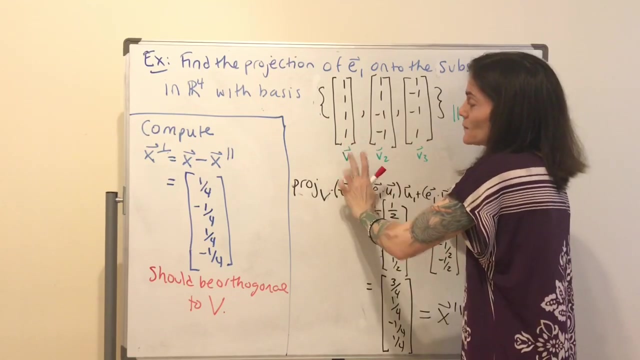 Because, well, every vector in V may be written as a linear combination of the basis vectors And if you take the dot product with a linear combination, it would be you could write it in terms of dot products with these, With, well, some coefficients. 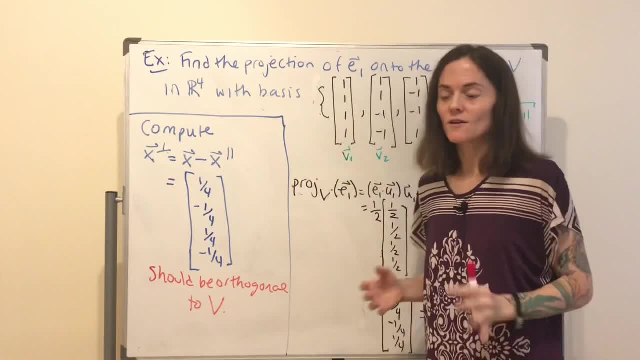 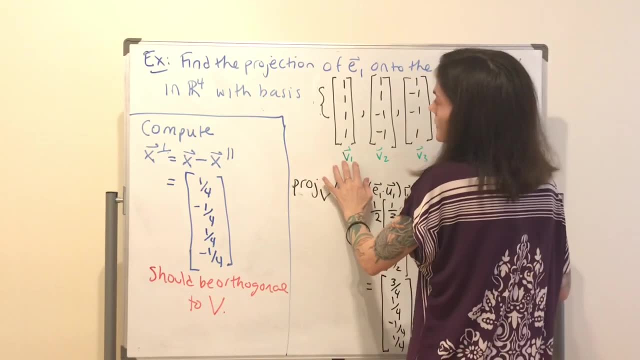 But if these all dot to 0, then you would get 0 for every single vector in V. So let's just think about that here. If you take this and dot with V1, well, a 4th minus a 4th, a 4th minus a 4th- 0. 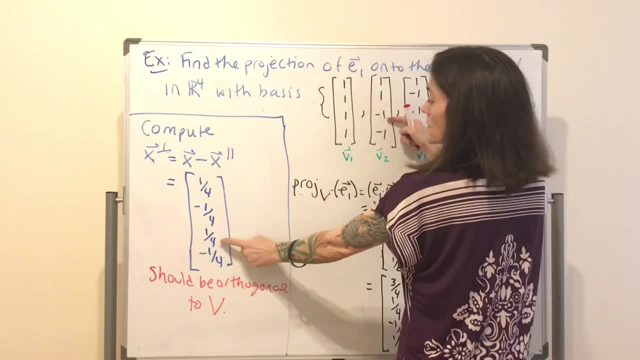 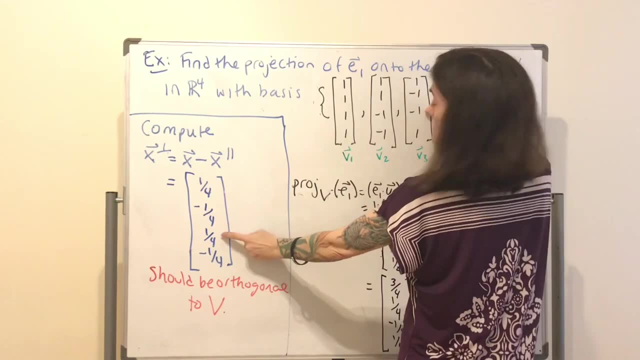 Dot it with V2.. You have a 4th minus a 4th minus a 4th, a 4th 0.. Dot it with V3.. Here we have 2 4ths minus a 4th minus a 4th 0.. 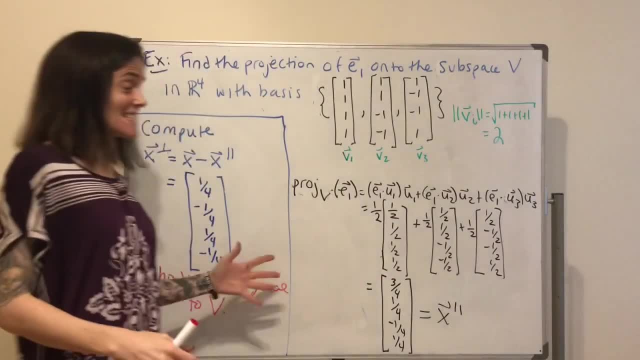 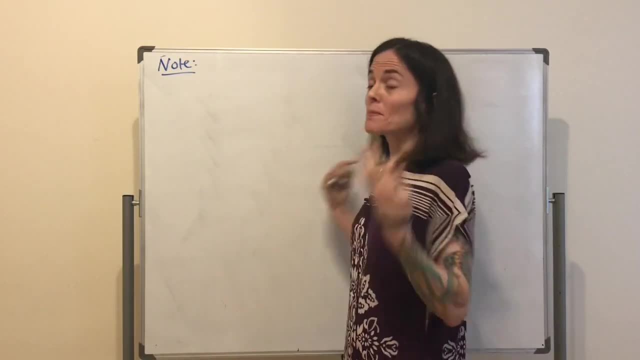 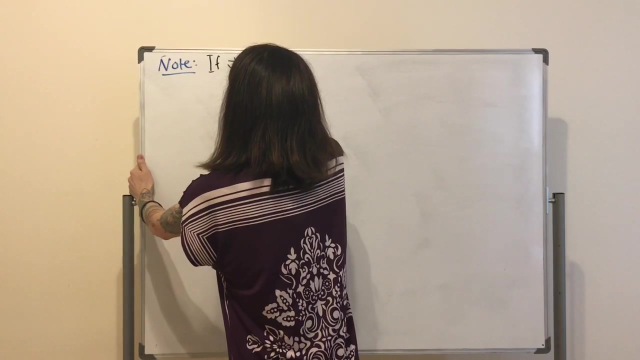 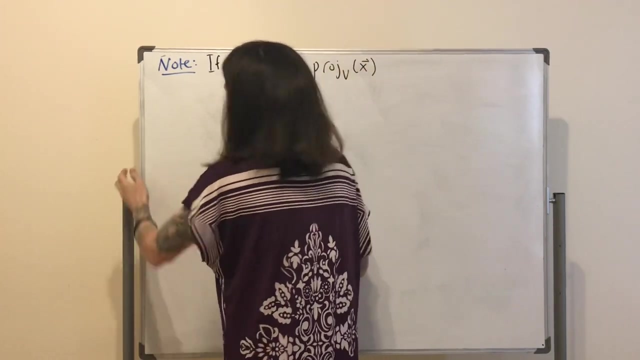 Okay, So in fact this is orthogonal to the subspace V. Let's make well an important observation: If the vector X is already in V, the projection of X, well, into V, what would this possibly be? You are already in the subspace. 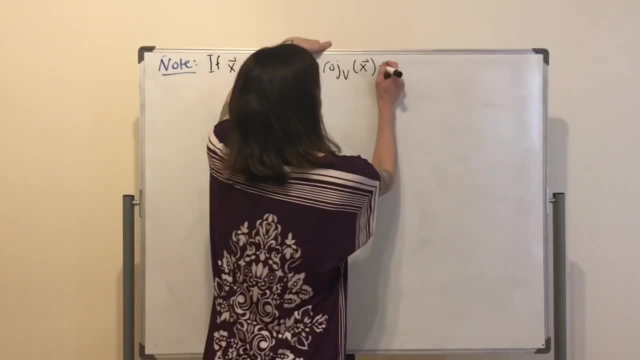 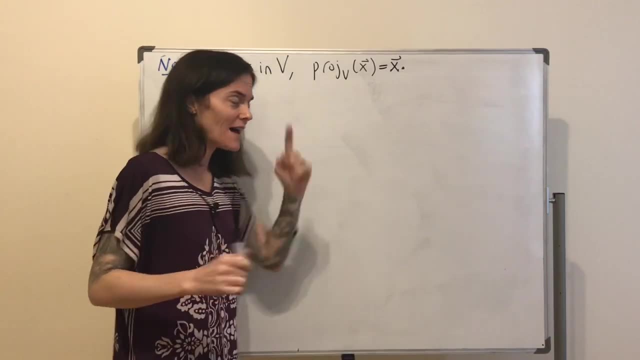 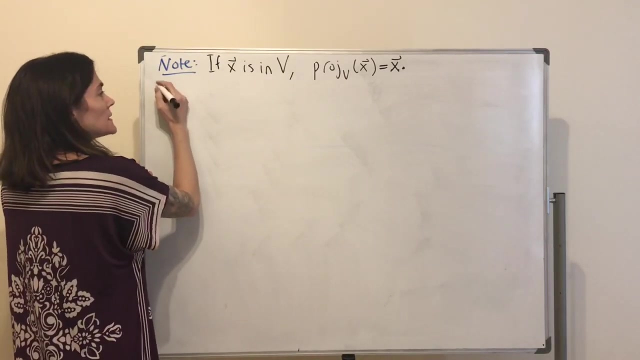 and you project into the subspace. You just get back the vector. okay. Now why is this an important observation? Well, it actually is more important than it seems at the moment. So what is this observation leads to the following: If you have U1,. 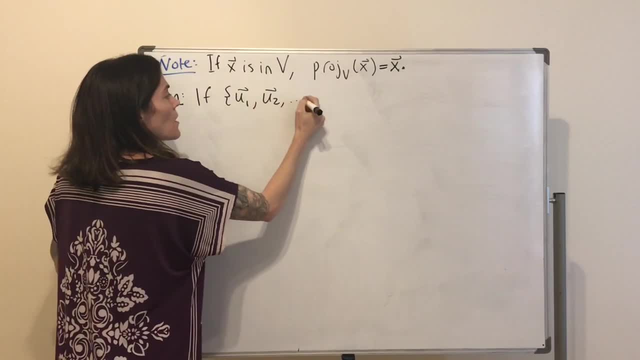 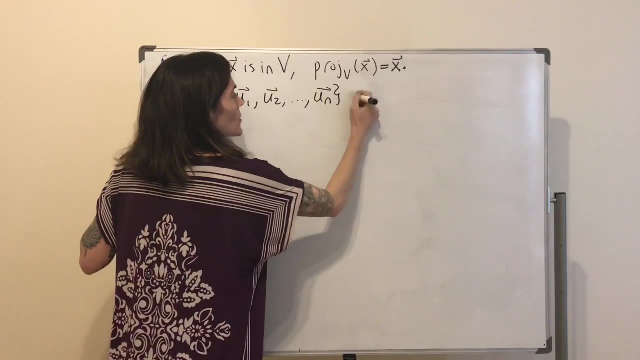 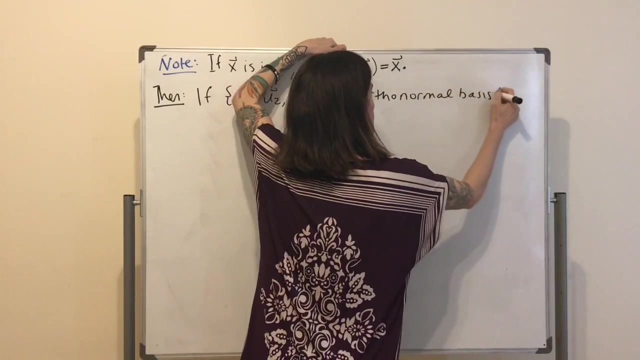 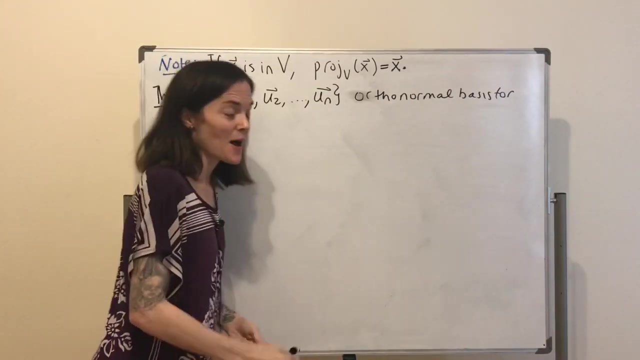 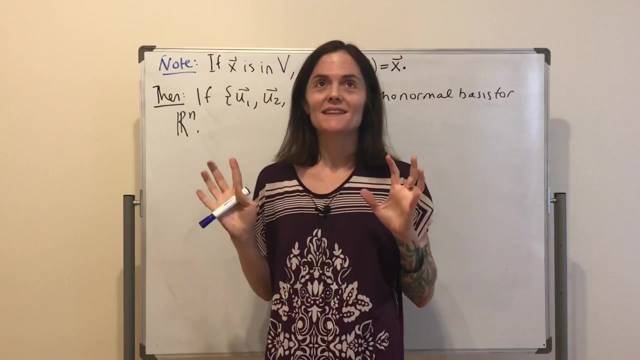 U2, now I'm gonna go all the way out to UN. This is a basis for RN, And I should add orthonormal basis for RN. Okay, well, let me make a comment before I use this. What did we talk about at the very end of our basis video? 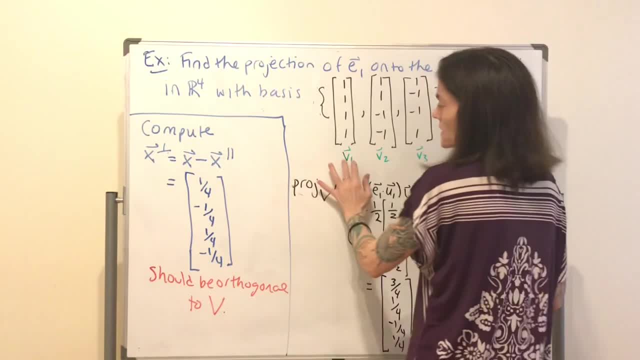 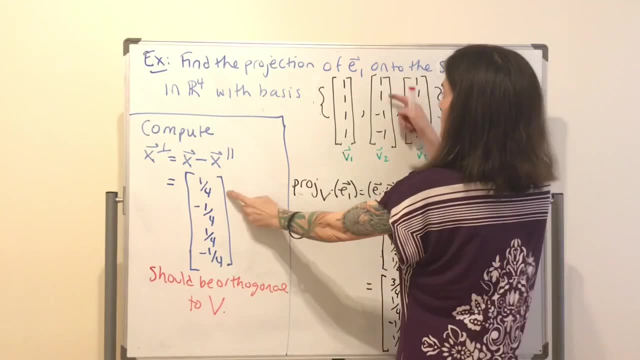 So let's just think about that here. If you take this and dot with v1, well, a fourth minus a fourth, a fourth minus a fourth zero. Dot it with v2.. You have a fourth minus a fourth minus a fourth, a fourth zero. 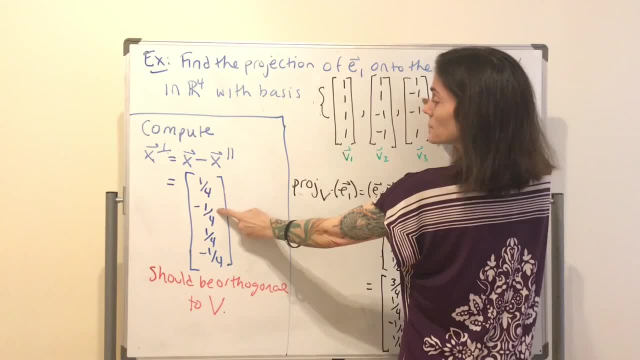 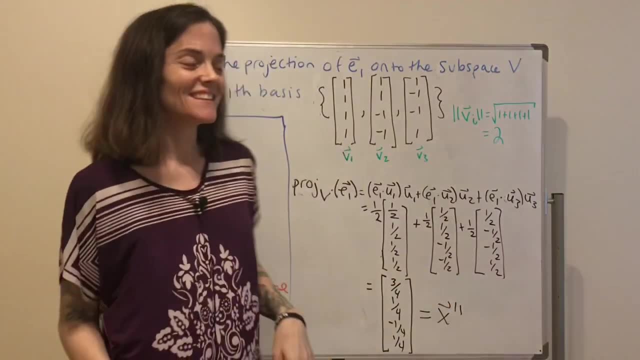 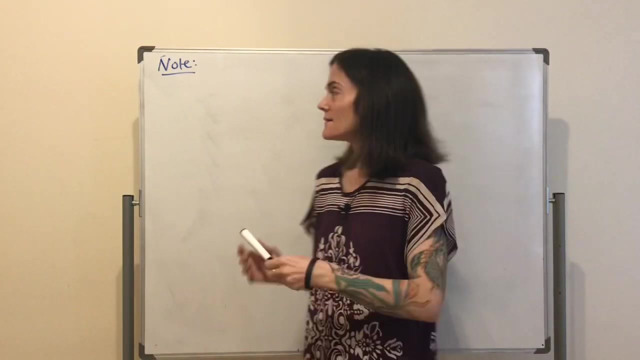 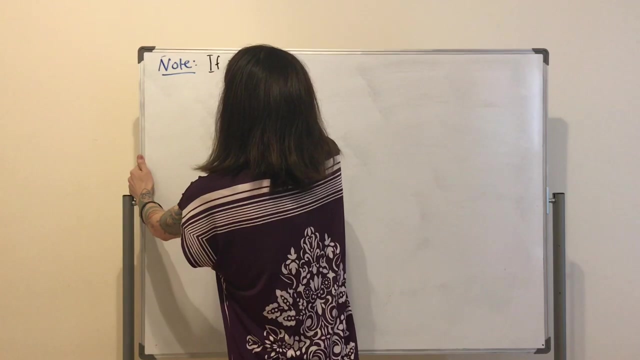 Dot it with v3.. Here we have two fourths minus a fourth minus a fourth zero. Okay, So in fact this is orthogonal to the subspace v. Let's make well an important observation: If the vector x is already in v, 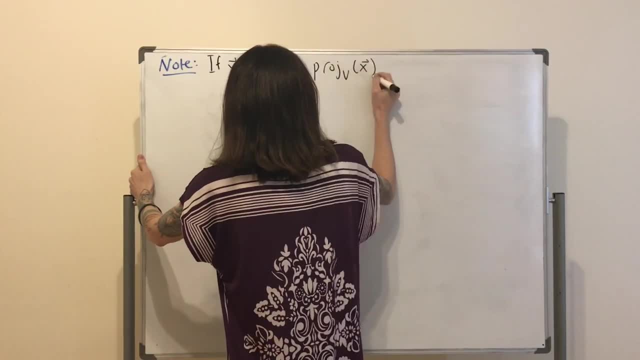 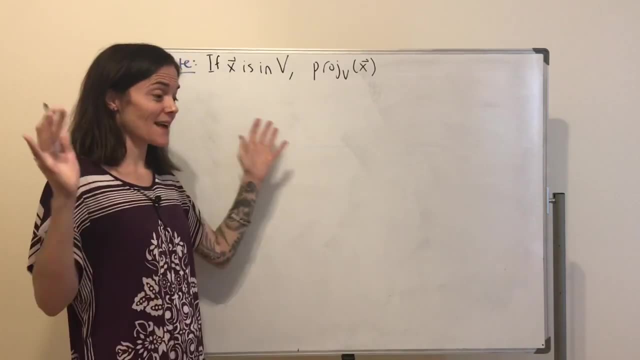 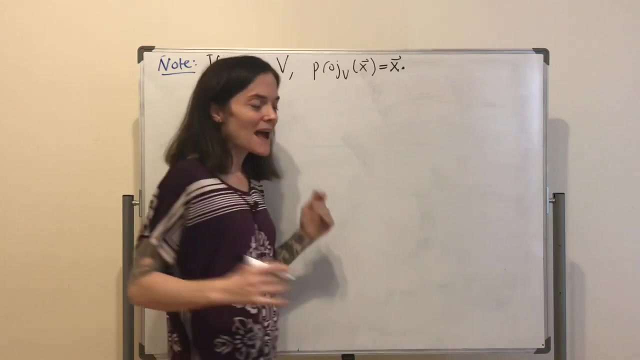 the projection of x, well, into v. what would this possibly be? You are already in the subspace and you project into the subspace. You just get back the vector, okay. Now, why is this an important observation? Well, it actually is more important. 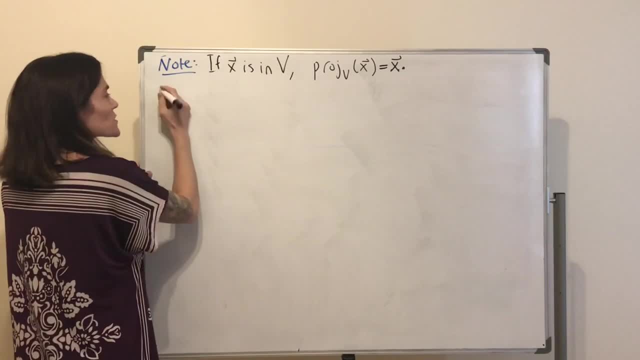 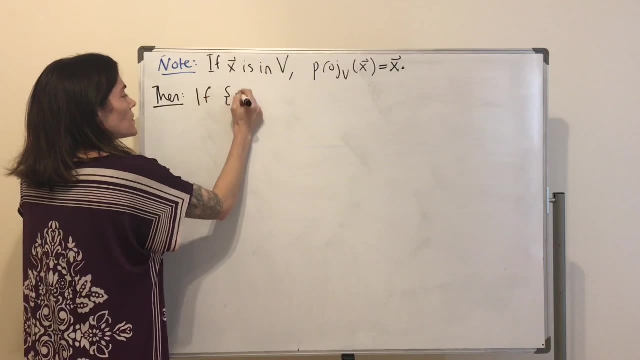 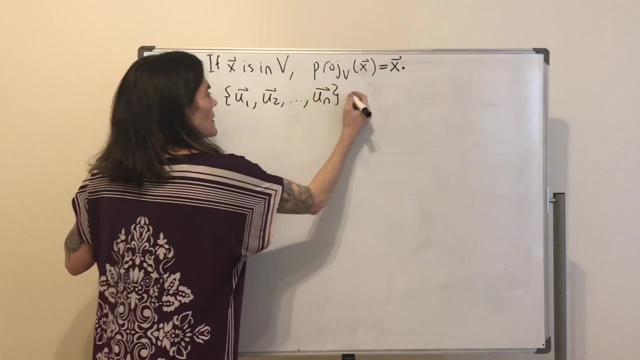 than it seems at the moment. So what is this? observation leads to the following: If you have u1,, u2, now I'm gonna go all the way out to un. This is a basis for our n And I should add, orthonormal. 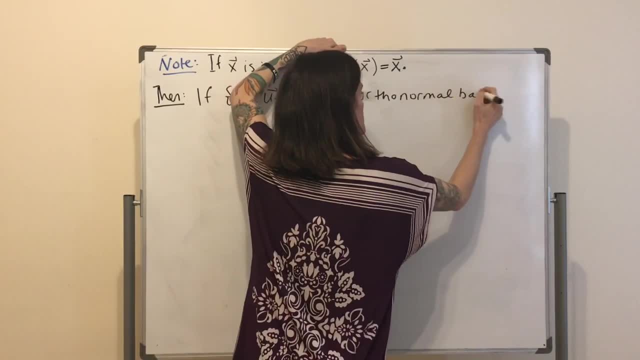 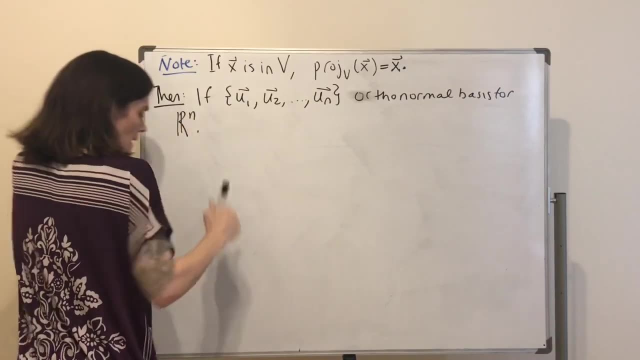 So, if you have u1,, u2,, u3, u4,, u5,, u6,, u7, u8,, u9, u10, this is a basis for our n? Okay, well, let me make a comment before I use this. 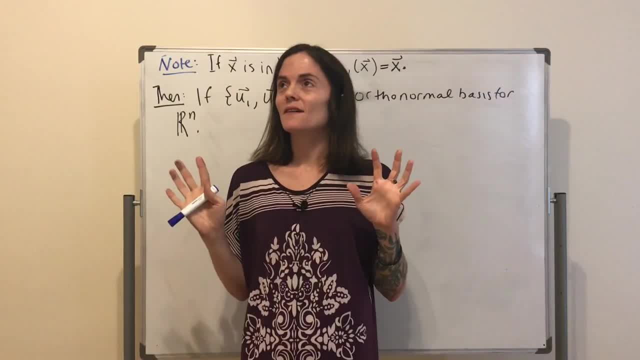 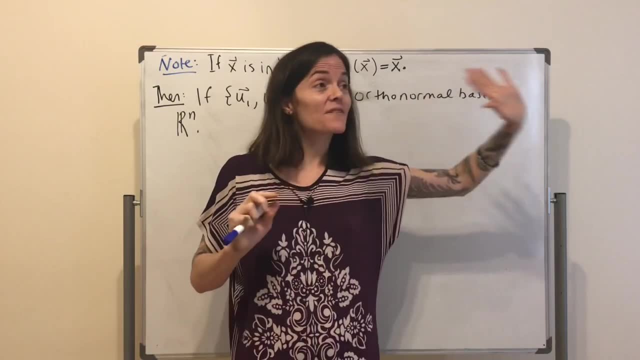 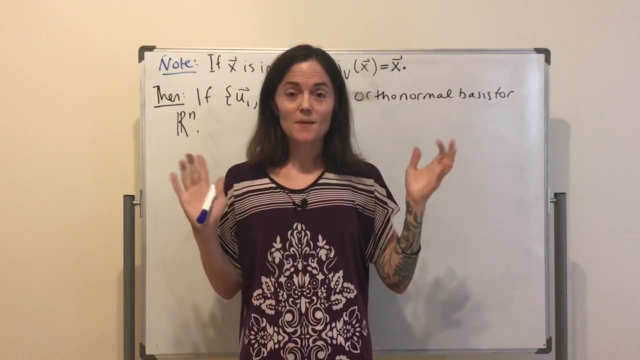 What did we talk about at the very end of our basis video? At least I think it was that video. If you have a basis, then every vector in your vector space can be written uniquely as a linear combination of the basis elements We know. so, given x in our n, 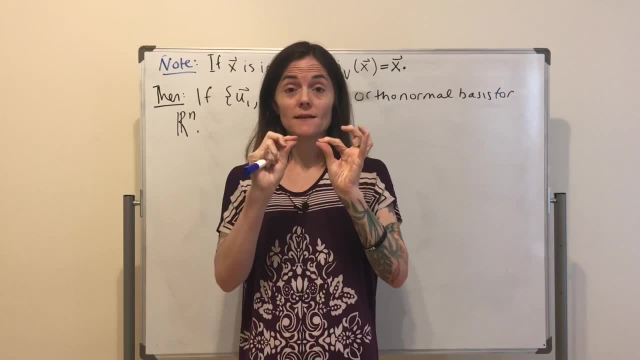 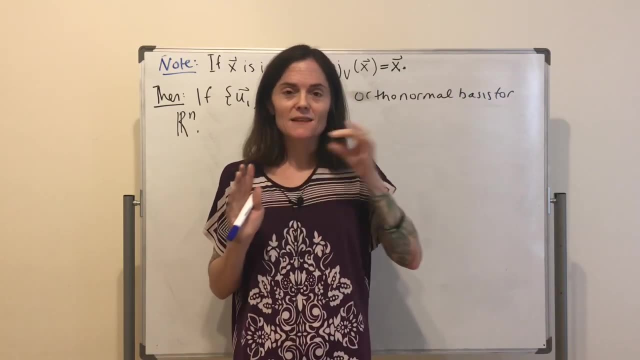 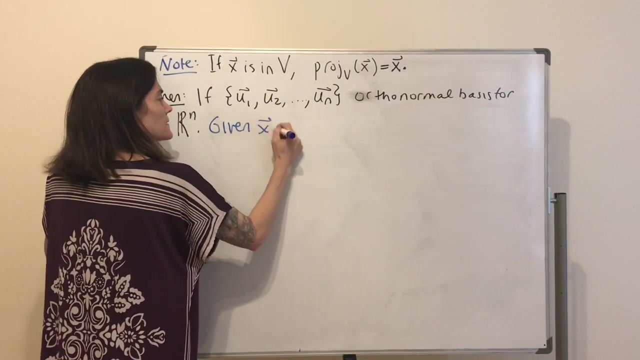 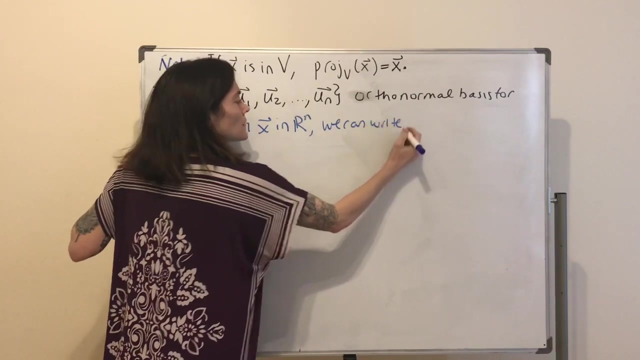 At least I think it was that video- If you have a basis, then every vector in your vector space can be written uniquely as a linear combination of the basis elements. We know so, given X in RN, we know we can write X uniquely as a linear combination of UI. 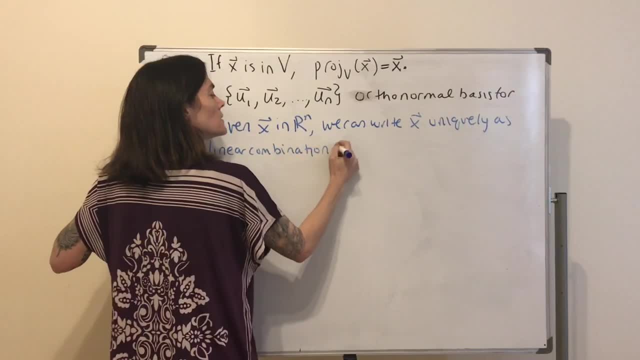 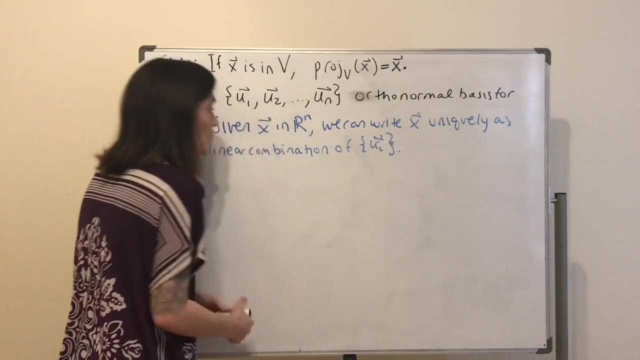 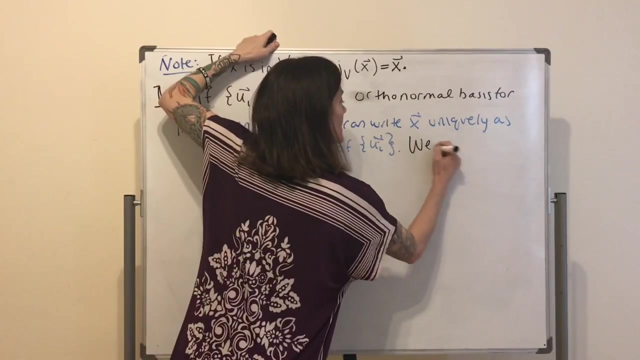 This is combination of this- that's what I just talked about- of this basis. We can find this, so we can find this unique way to write it. We can find, and I'll even tell you what it's called. They're called the coordinates. 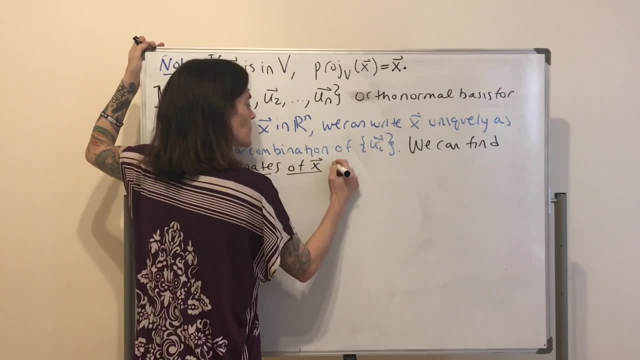 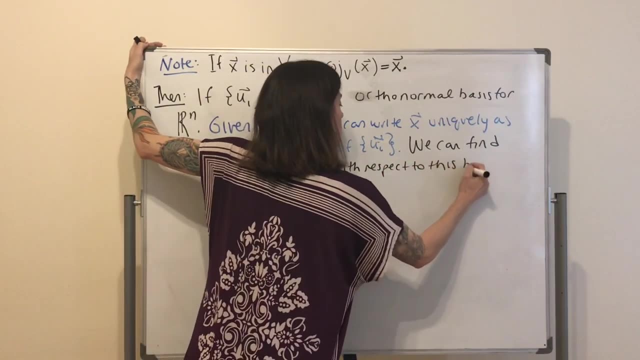 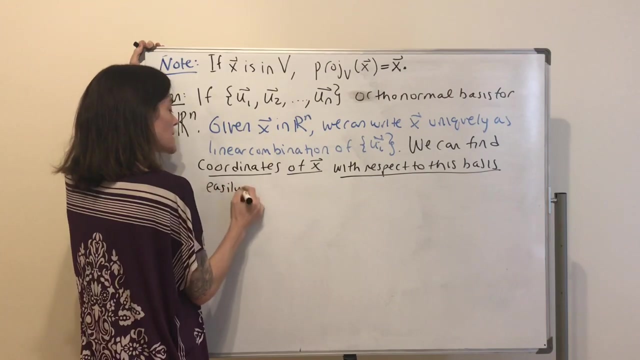 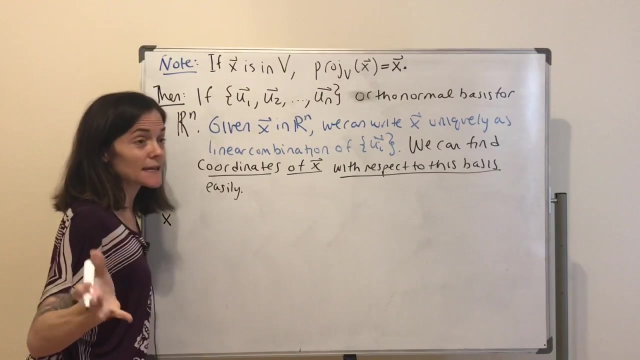 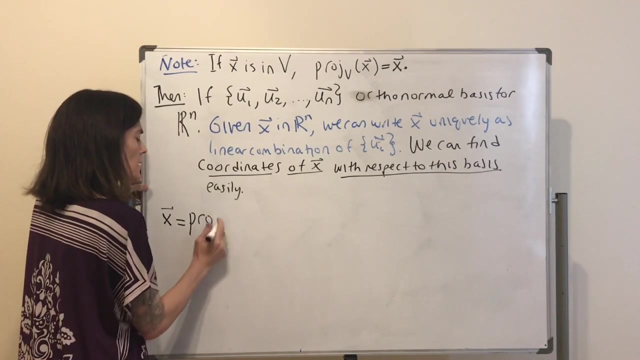 of X with respect to this basis, Easily Using this idea of pretty much of like a vector of projection, because we know that x, x is in our n, therefore it will be equal to the projection. uh, oh, i didn't mean to put that lower the projection here. this is using this observation. 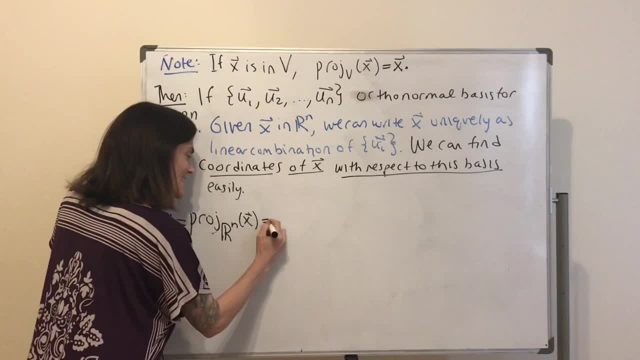 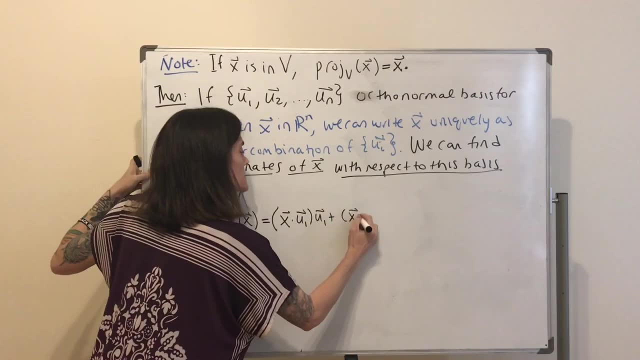 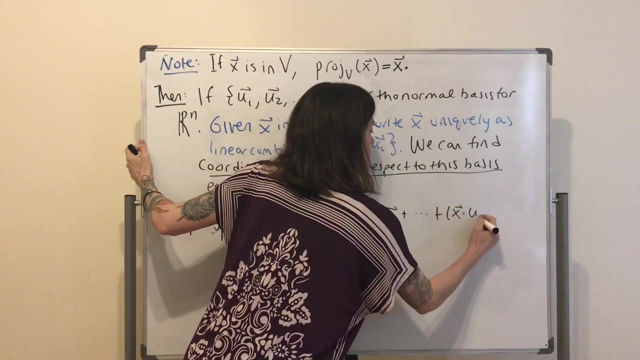 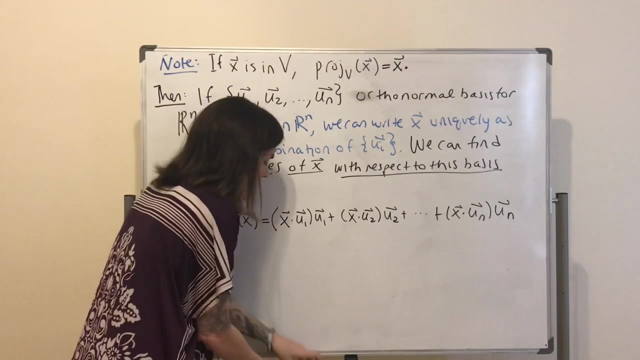 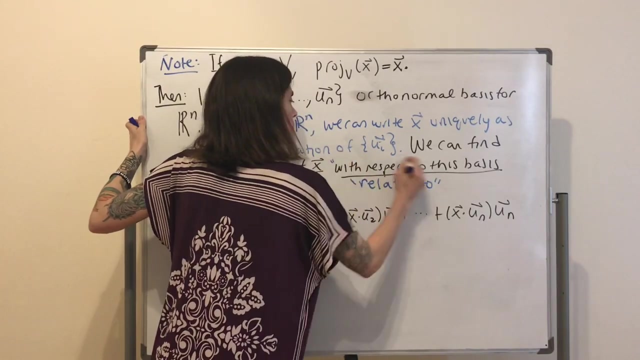 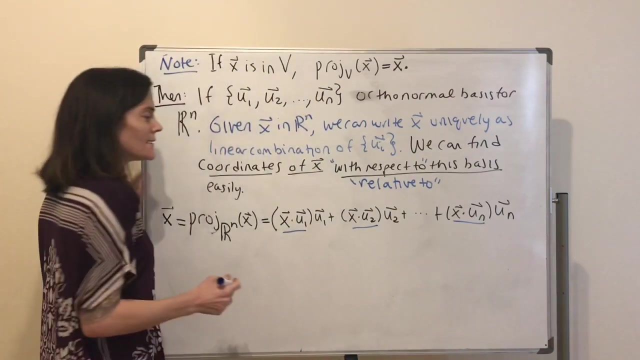 right, and then this equals well, x dot u1- u1 plus x dot u2- u2, out to x dot un- un. and these are what's called the coordinates with respect to, or you might also see, relative to this basis. this is coordinate one, coordinate two, coordinate three. okay, well, excuse me, coordinate n. 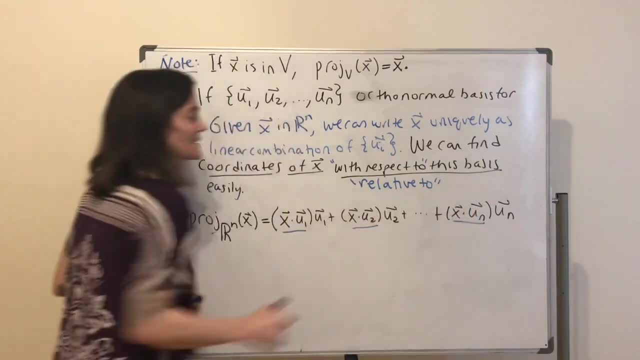 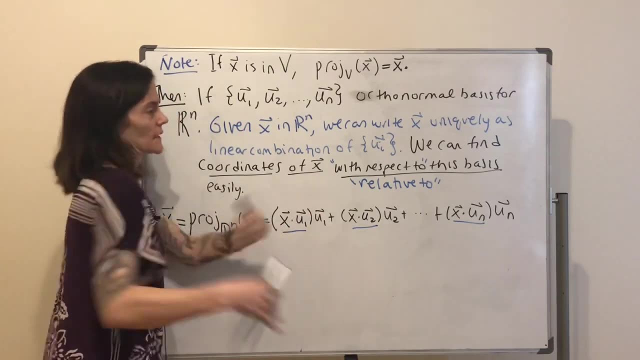 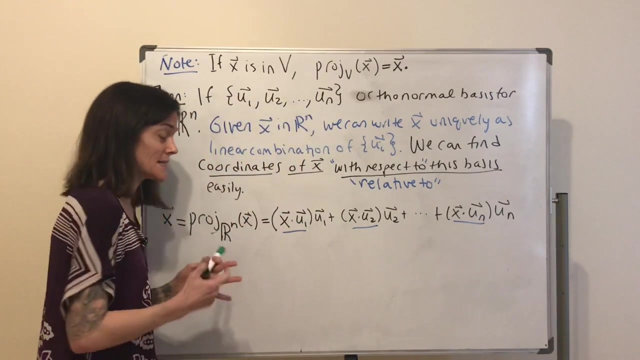 coordinate one, coordinate two, coordinate three. out to coordinate n. okay, because they are the coefficients that appear in front of the basis vectors um in this linear combination. it's very much like- and i'll do an example in a moment, but let me take you into. what is this like? 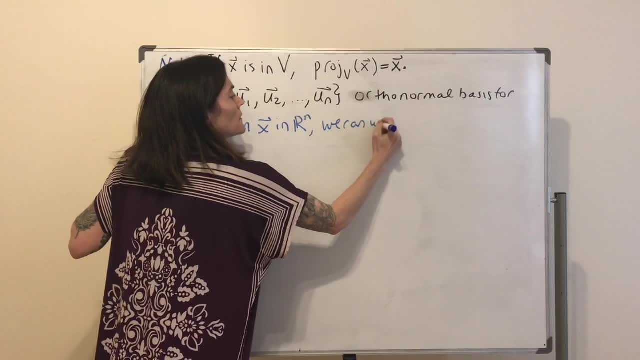 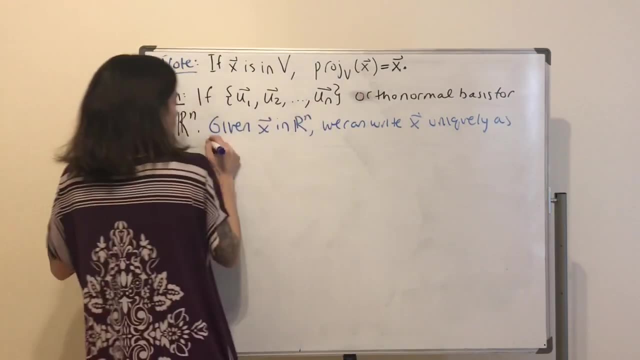 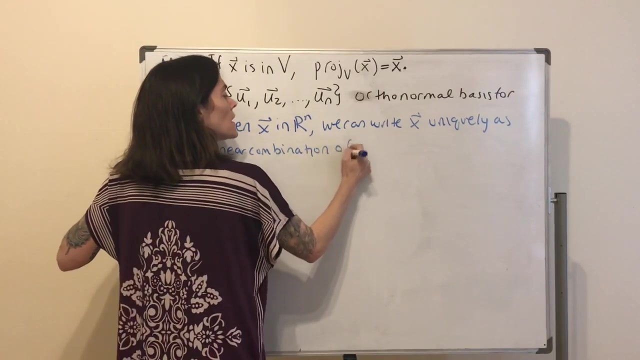 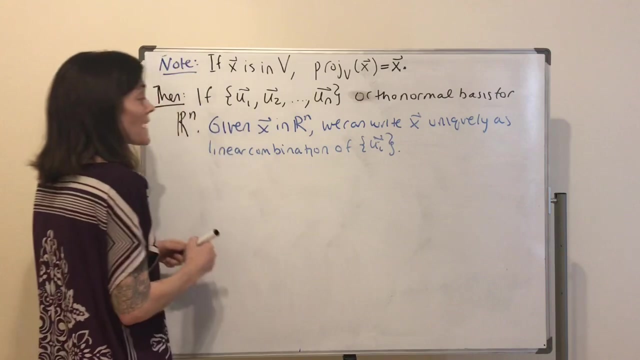 we know we can write x uniquely as a linear combination of ui. This is combination, This is combination Of this, that's what I just talked about. of this basis We can find this, so we can find this unique way to write it. 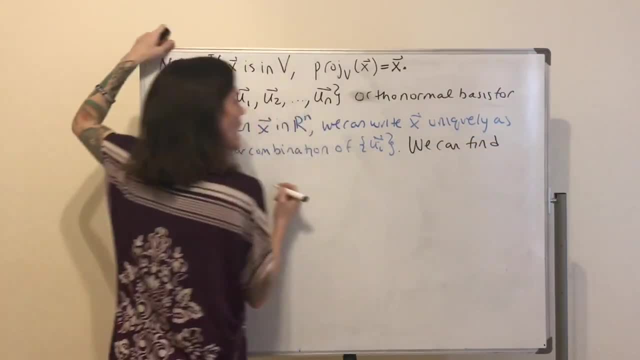 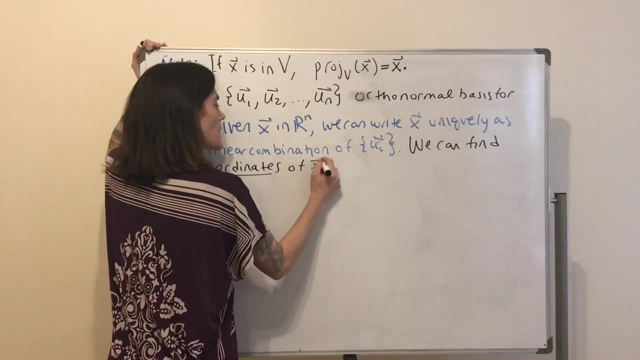 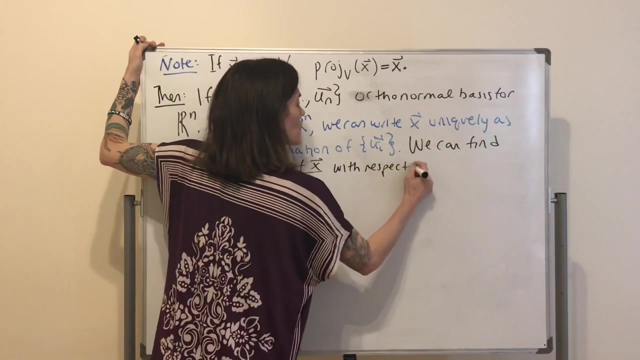 We can find, And I'll even tell you what it's called. They're called the coordinates of x with respect to this basis. So, for example, if we want to do well, let's say: x is equal to y. So this is: x is equal to y. 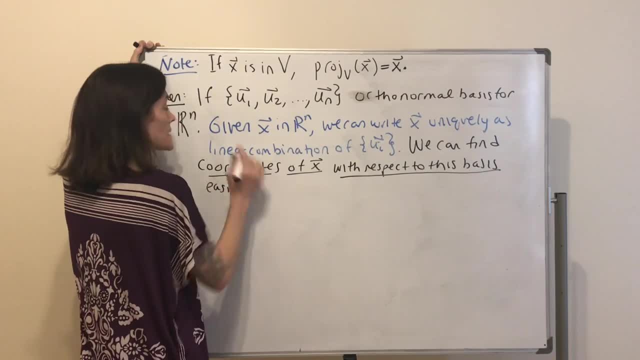 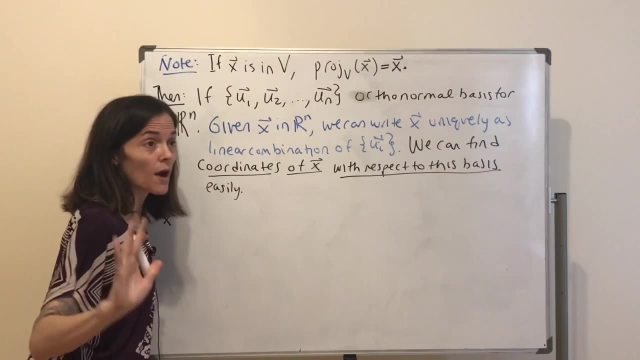 so, like I said, x is in our n, So I can write this. so, like I said, x is in our n, So I'm gonna use this as my last is gonna use this as my last, but let's. 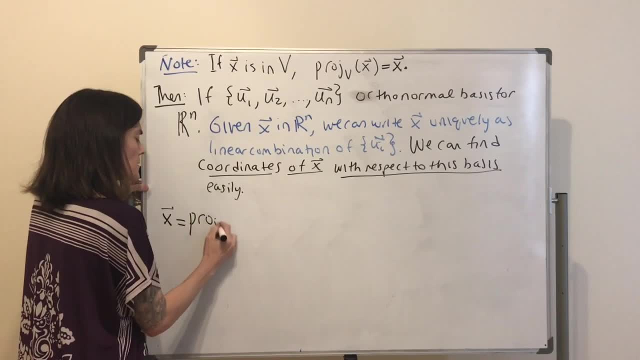 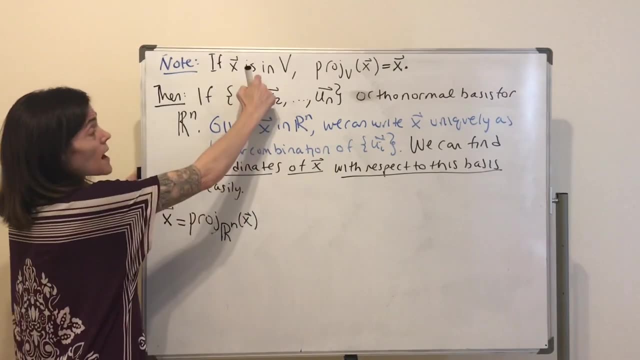 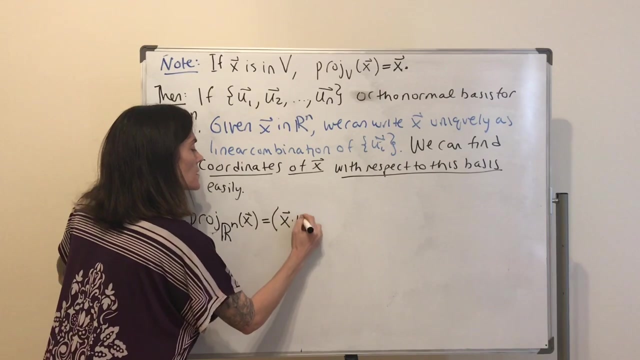 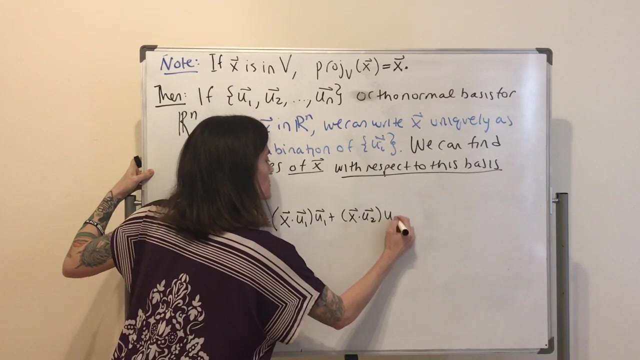 we don't even need the last one. I'm gonna use this as my last, just to get the last part of this, Easily, this observation right. And then this equals well, x dot u1, u1, plus x dot u2, u2, out. 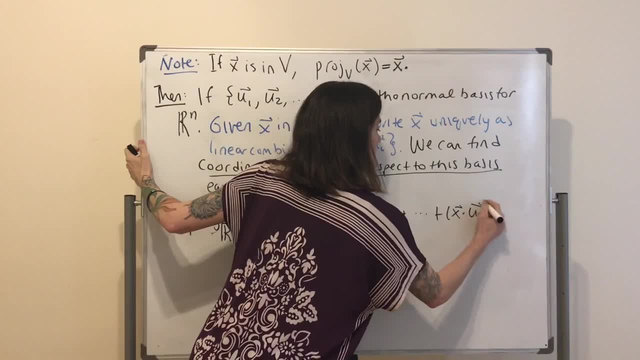 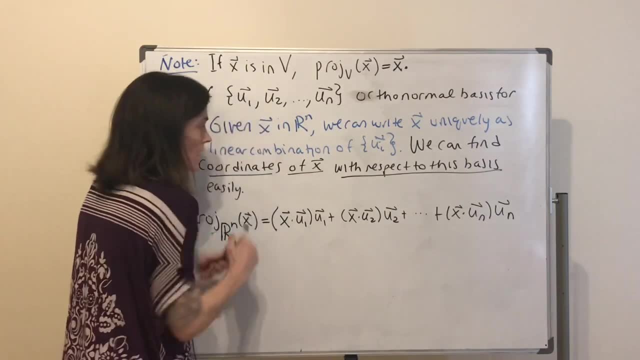 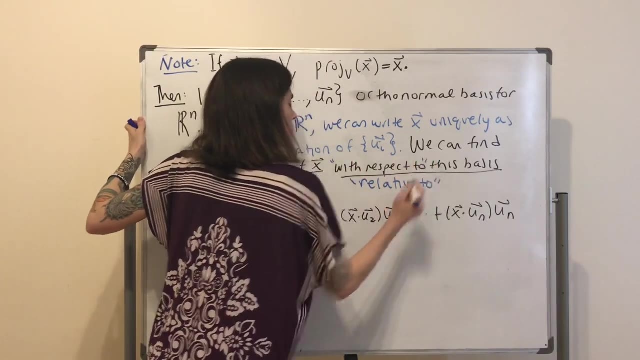 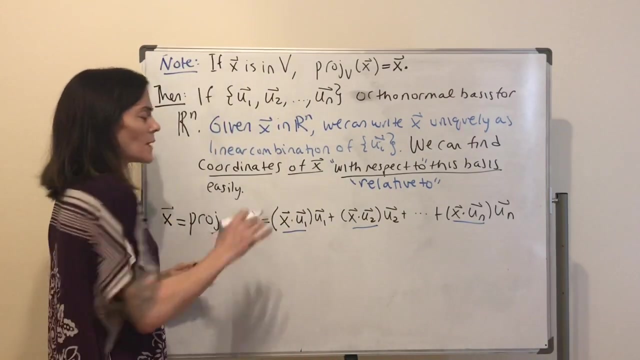 2, x, dot, un, un, And these are what's called the coordinates with respect to, or, you might also see, relative to this basis. This is coordinate 1, coordinate 2, coordinate 3.. Okay, well, excuse me. coordinate n. Coordinate 1, coordinate 2, coordinate 3, out 2, coordinate n. Okay. 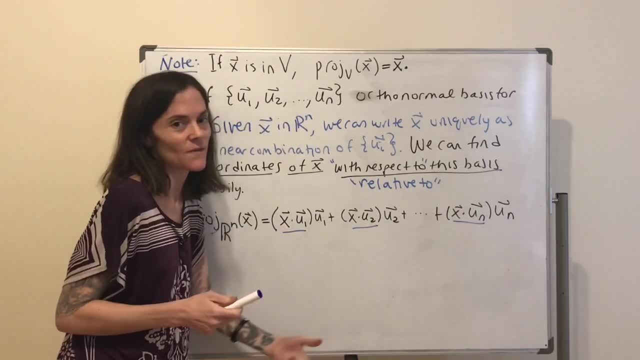 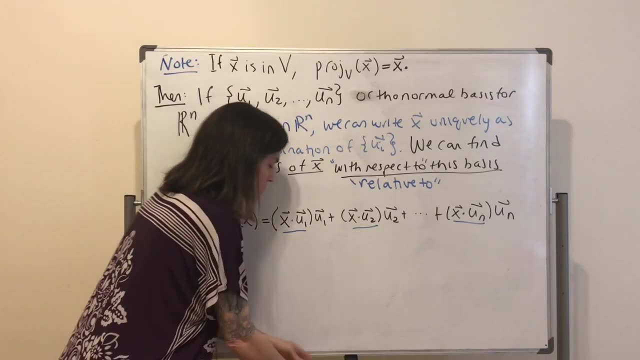 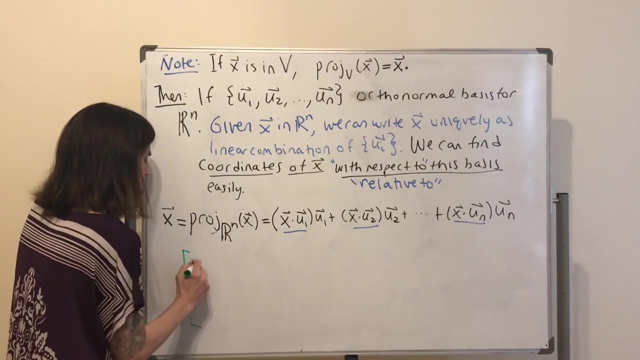 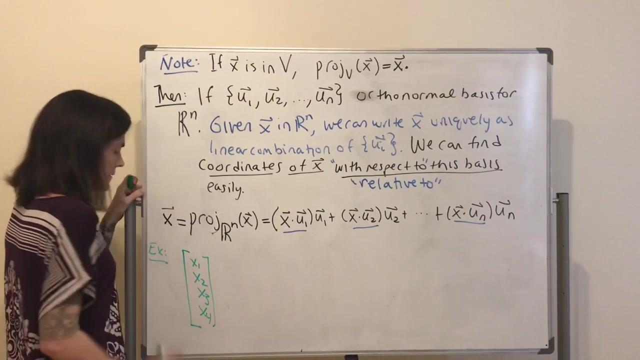 because they are the coefficients that appear in front of the basis vectors in this linear combination. It's very much like- and I'll do an example in a moment, but let me take you into what is this like. It's very much like this. We have this. Maybe I'll just do it in terms of 4.. We think of the coordinates. 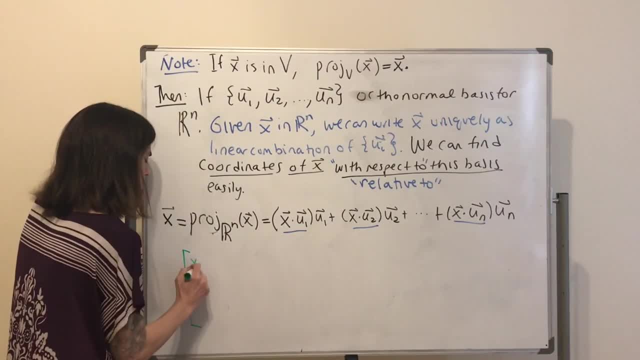 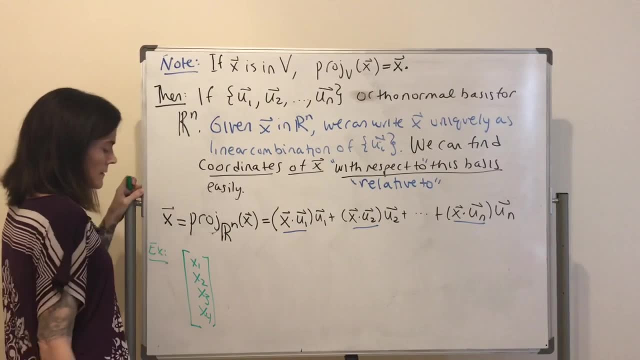 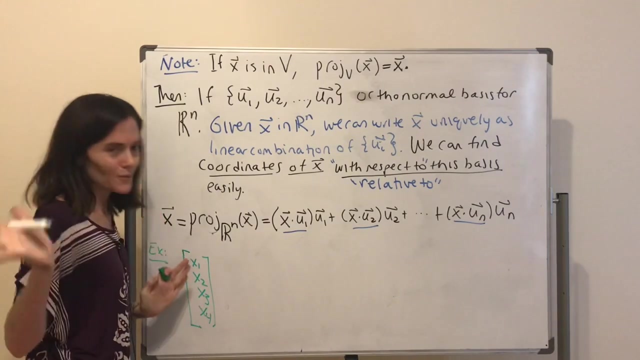 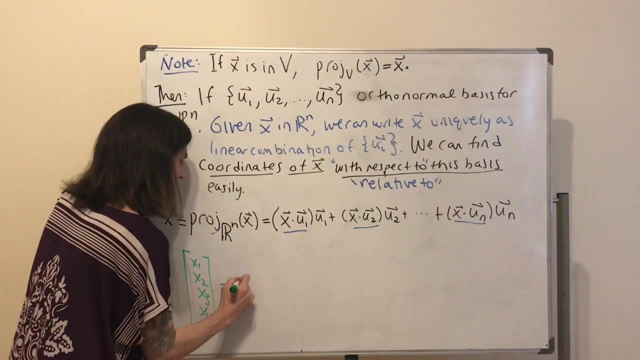 it's very much like this. we have this, maybe i'll just do it in terms of four. we think of the coordinates of this vector, as we are looking at it, as x1, x2, x3, x4. right, we're good, but in light of this observation, this is x1- e1 plus x2- e2. 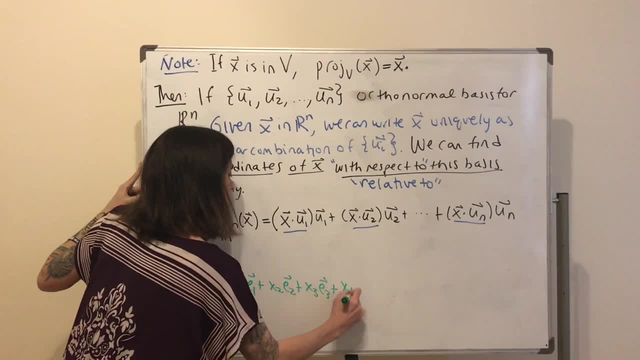 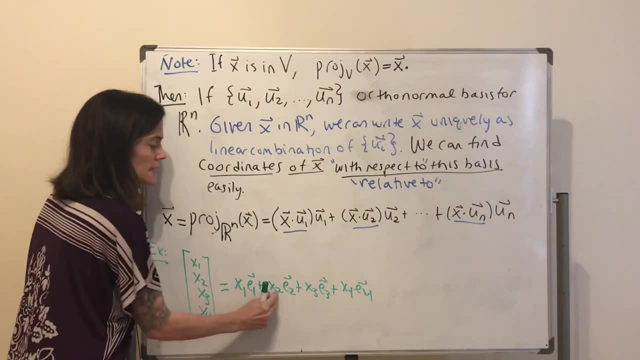 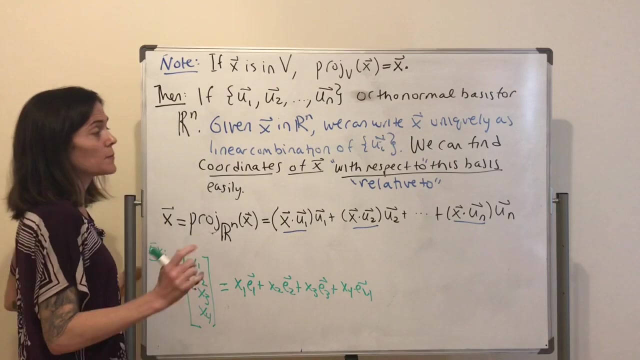 x3, e3, x4, e4. in fact, this is definitely the case, that these, this and this is equal. and so you see, these x1, x2, x3, x4 are the coordinates of this vector with respect to the standard vector basis, but if you have a different orthonormal basis, then whatever this coefficient is here. 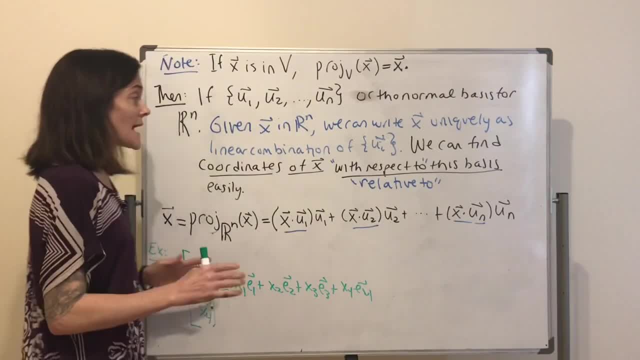 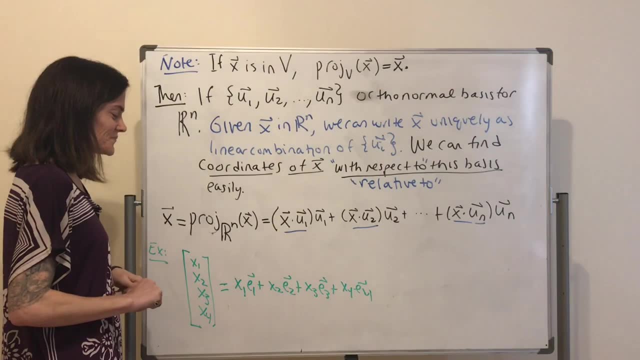 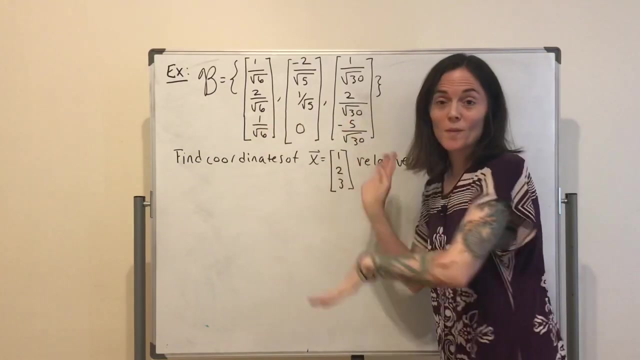 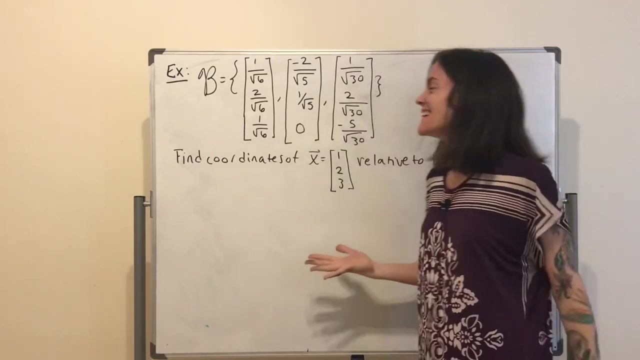 here, here, etcetera. it would just be called as the coordinates of x relative to, or with respect to, that basis. okay, now i'm returning back to this orthonormal basis. this was one that we did right, and i said i'm returning back to it here i have, but that this is an orthonormal basis. 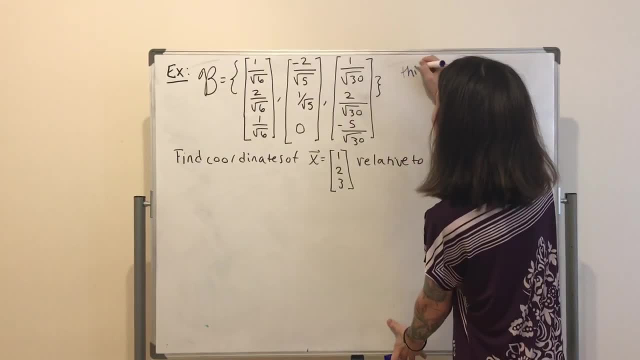 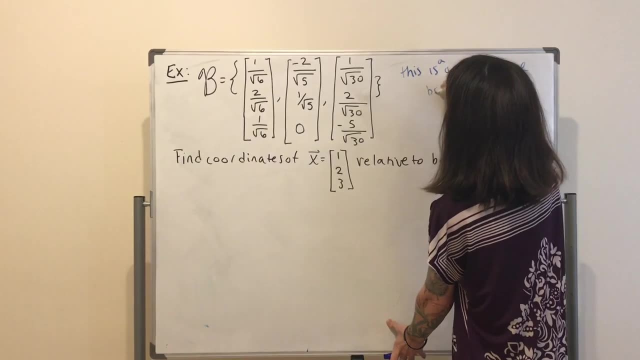 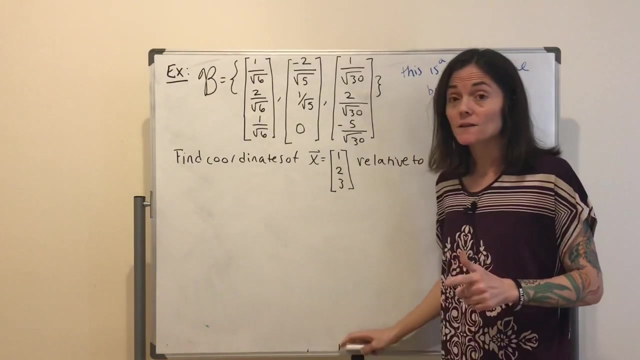 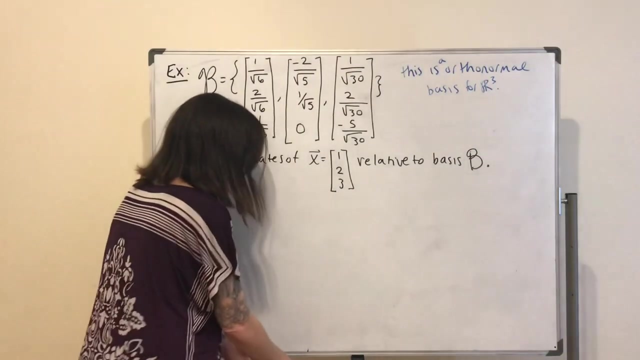 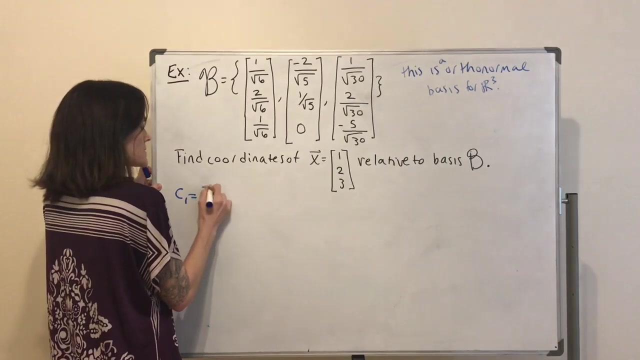 maybe i should write that we showed and we calculated this is orthonormal or is a orthonormal basis for our three. okay, then we're going to find the coordinates of this vector relative to this basis. okay, all we need to do is calculate. so maybe i'll say c1. the first coordinate is x. 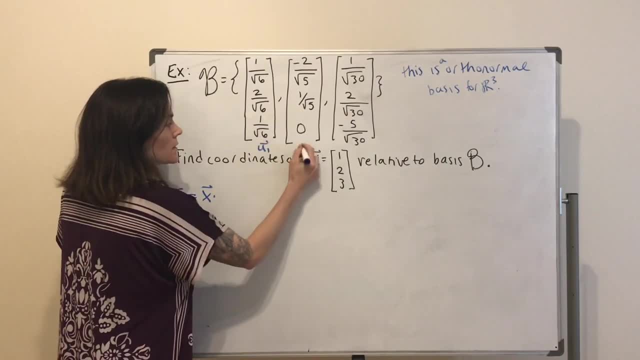 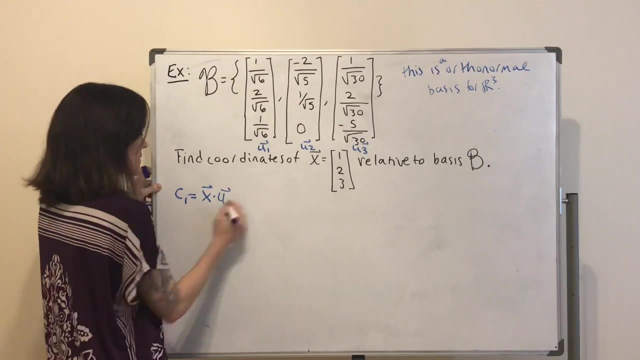 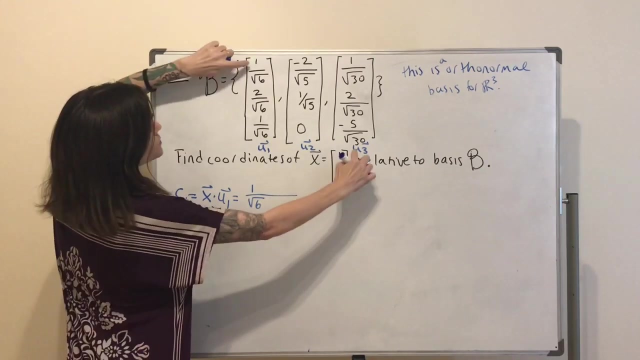 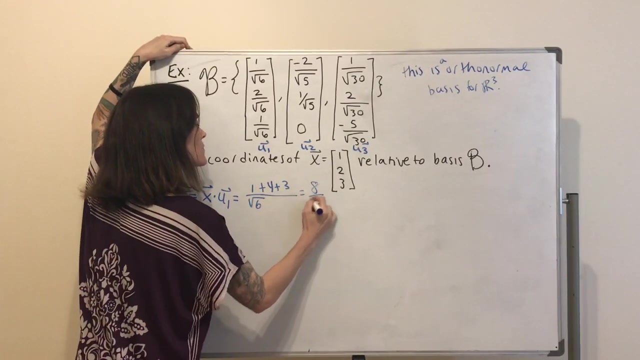 dot. oh, let's say this is u1, u2, u2, and u3,. like this, this would be x dot, u1.. And this is okay. here we go. It's 1 over square root 6.. Oh well, this is all over square root 6.. It's 1,, 4,, 3.. We have 8 over the square root of 6.. 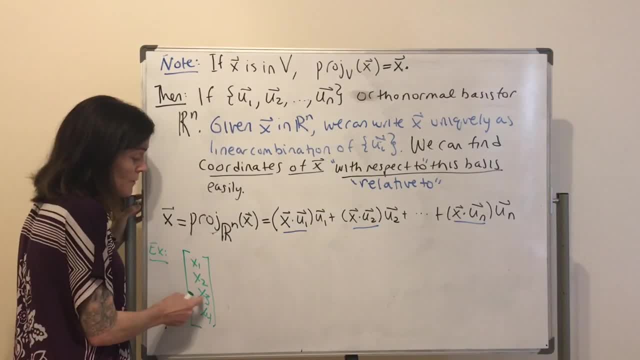 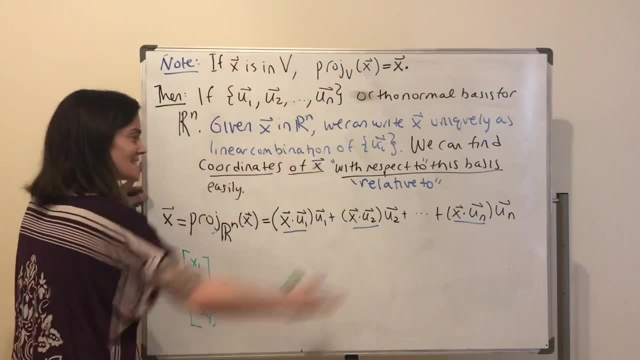 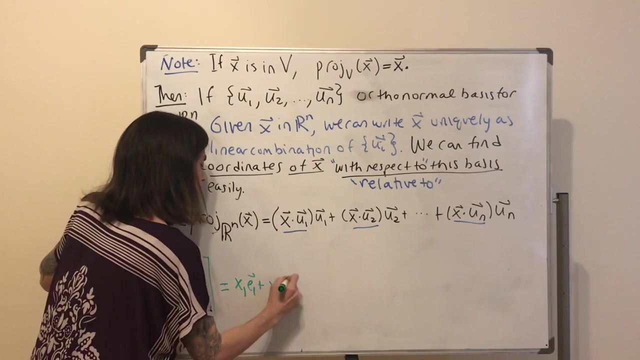 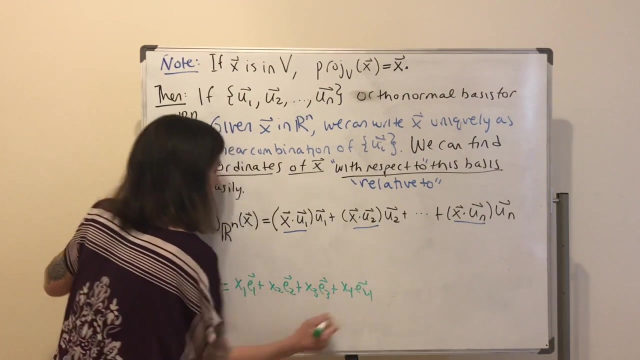 of this vector, as we are looking at it as x1, x2, x3, x4, right, We're good. But in light of this observation, this is x1. E1 plus x2, e2, x3, e3, x4, e4.. In fact, this is definitely the case, that this and this is. 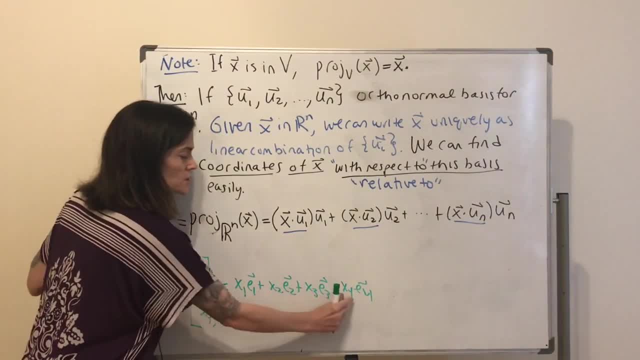 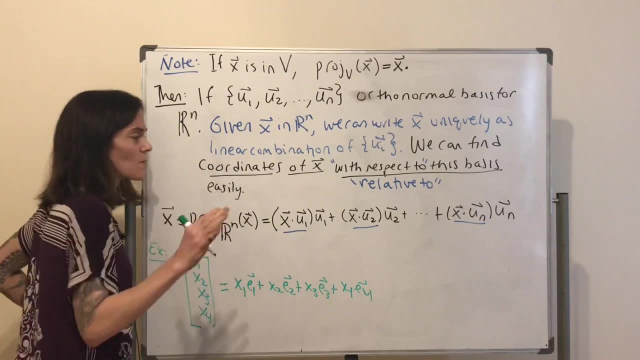 equal. And so you see, these x1, x2, x3, x4 are the coordinates of this vector with respect to the standard vector basis. But if you have a different orthonormal basis, then whatever this coefficient is here, here, here, et cetera, it would be a different orthonormal basis, And so 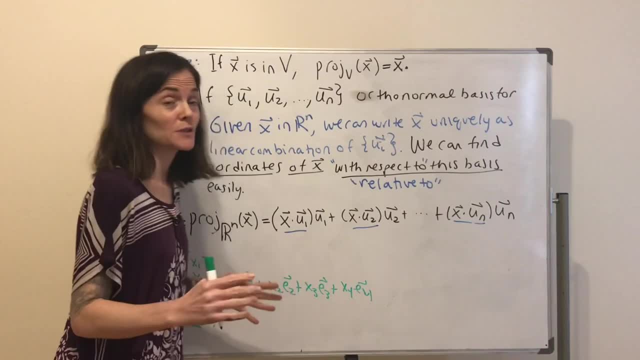 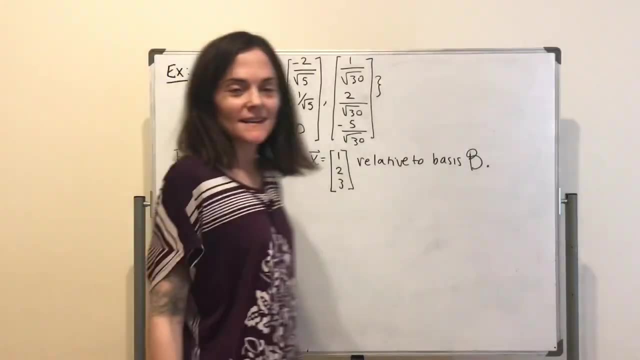 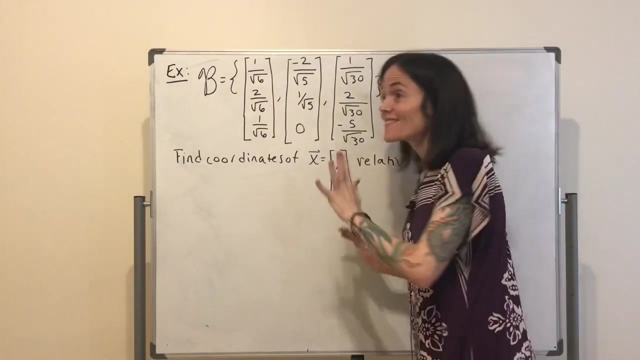 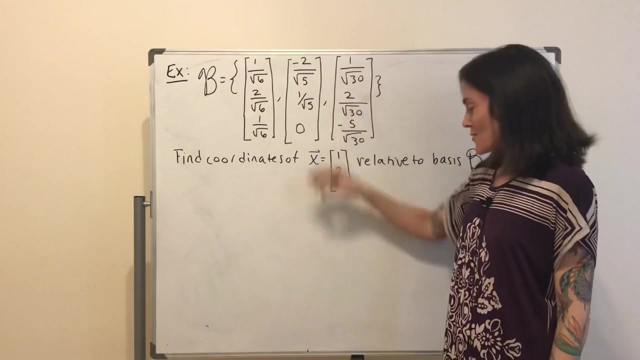 you would just be called as the coordinates of x relative to or with respect to that basis. Okay, Now I'm returning back to this orthonormal basis. This was one that we did right, And I said I'm returning back to it. Here I have, But that this is an orthonormal basis, maybe. 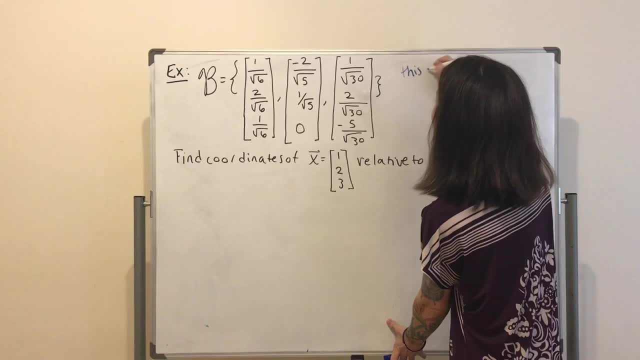 I should write that We showed and we calculated. This is the basic basis. So you can calculate here and there And then you can just go back to that and then you can look at the other things And then you can just look at it, and then you can go back and look at that And then 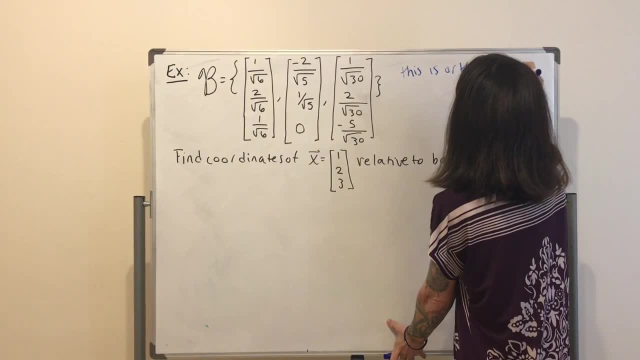 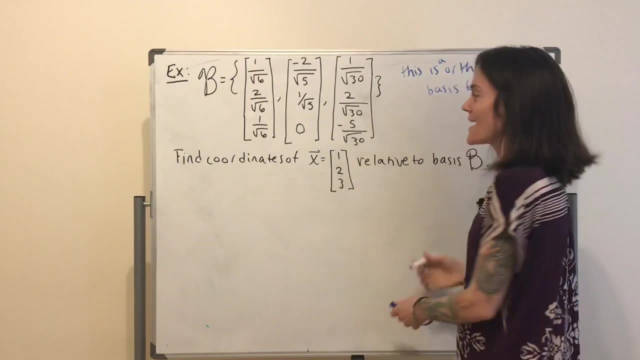 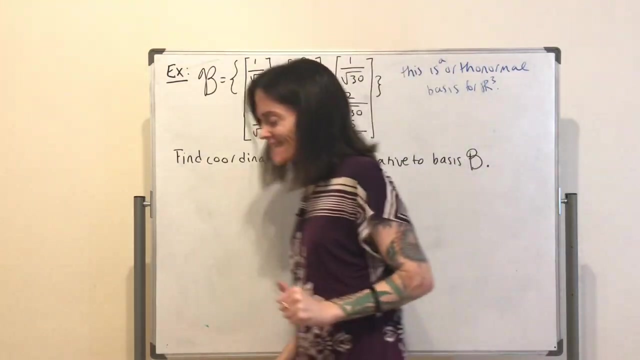 you can look at that, And then you can look at that, And then you can look at that. And orthonormal, or is a orthonormal basis for our three? okay, then we're going to find the coordinates of this vector relative to this basis. okay, all we need. 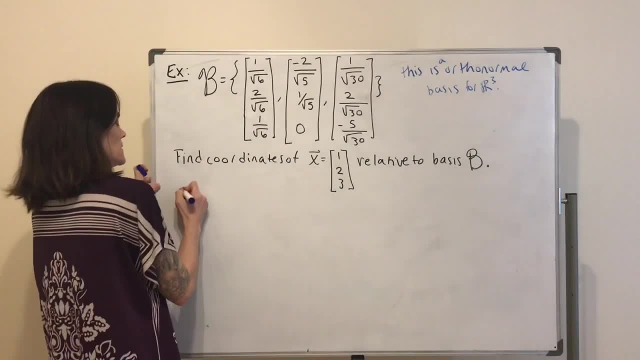 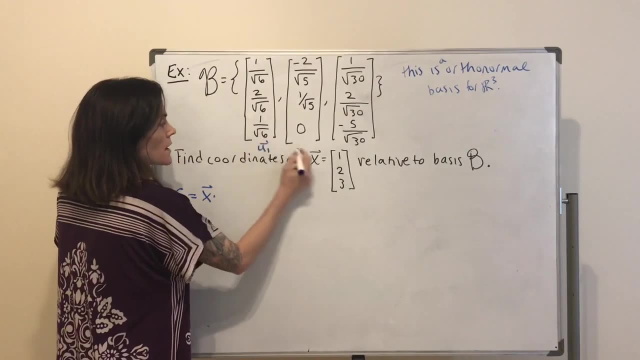 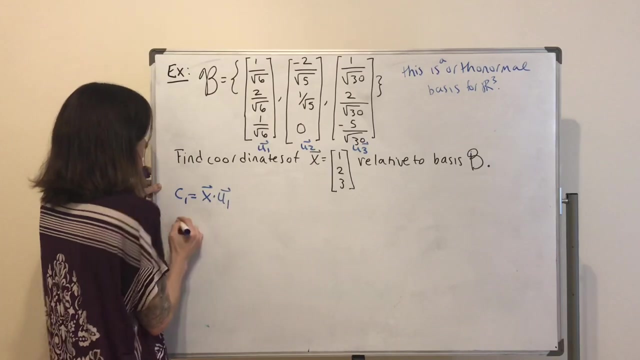 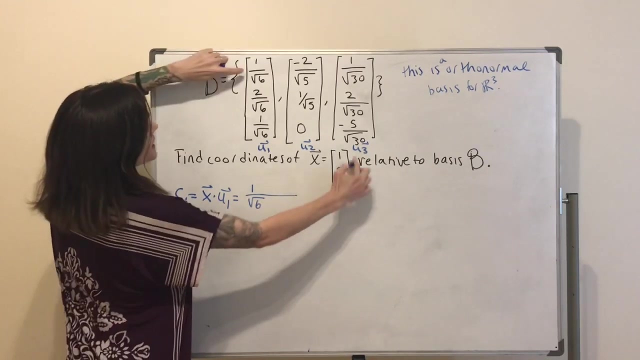 to do is calculate, so maybe I'll say c1. the first coordinate is X dot. oh, let's say this is u1, u2 and u3. like this, this would be X dot, u1 and this is okay. here we go. it's 1 over square root 6. oh well, this is all over square root 6. it's 1- 4. 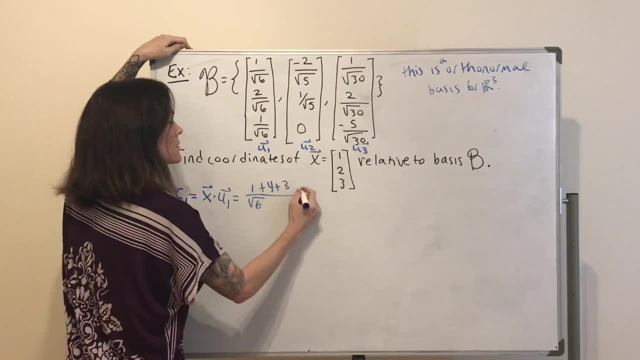 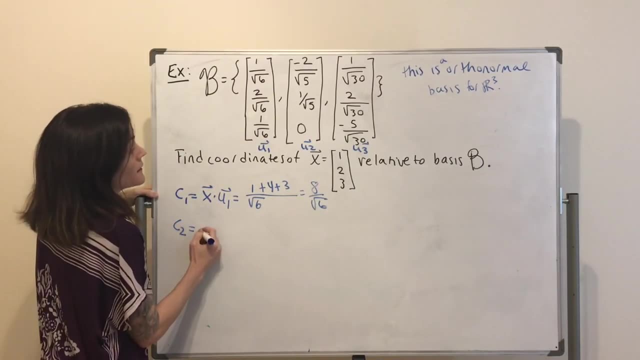 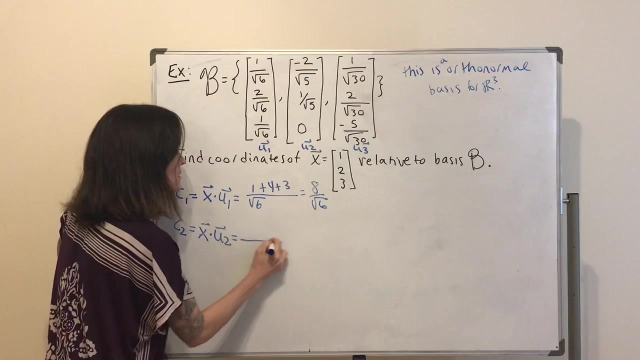 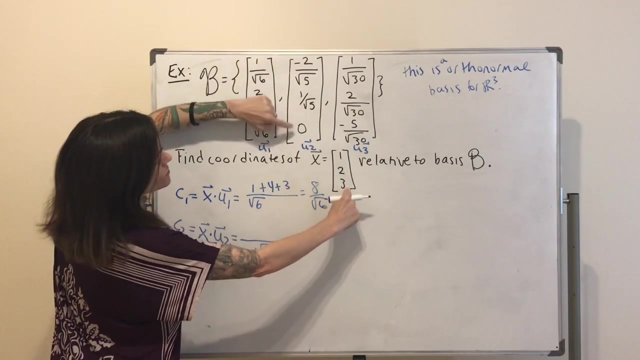 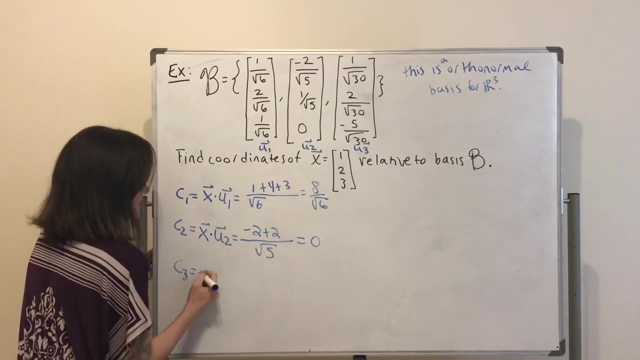 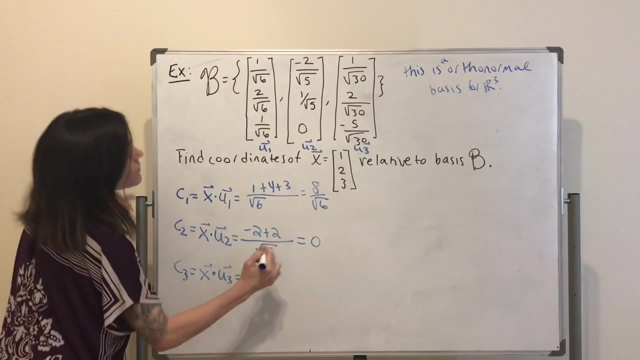 3. we have 8 over the square root of 6. and then see 2. this is going to be all over. well, I'll write it: x dot U 2. this will be all over the square root of 5. we get minus 2 plus 2. oh, this is just 0. and then see 3. this is x dot u 3. here we go. 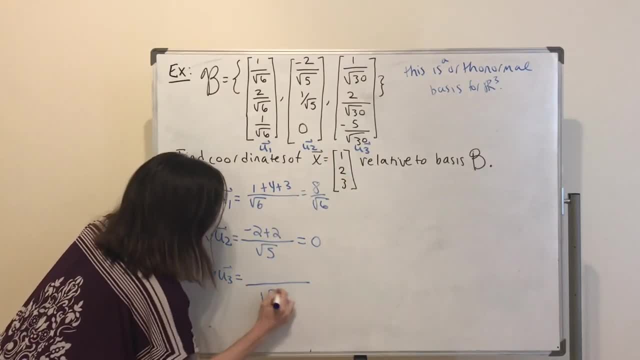 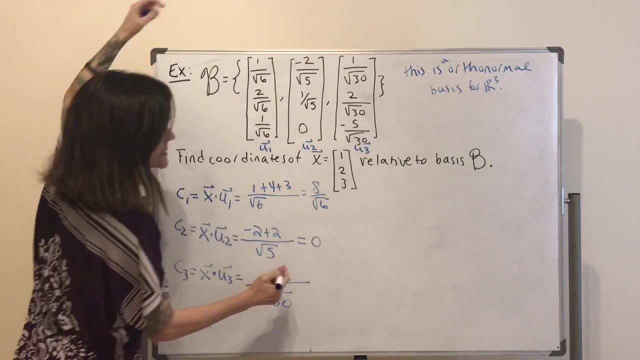 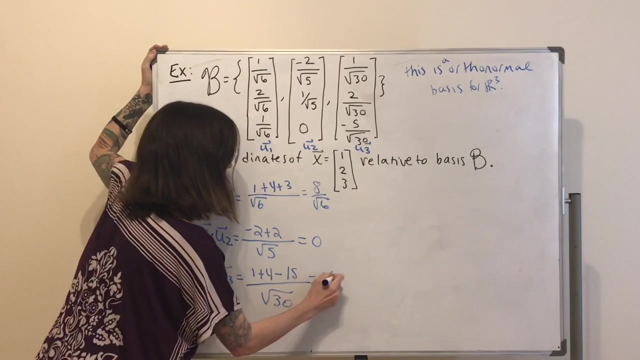 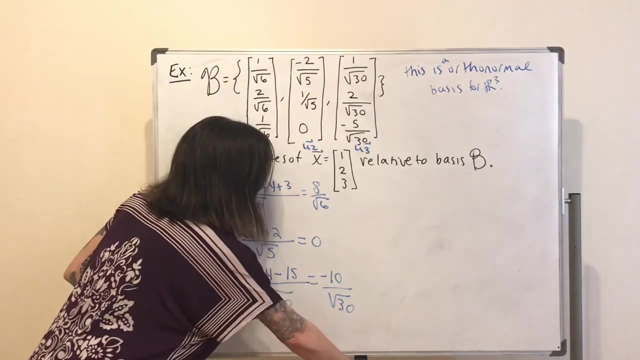 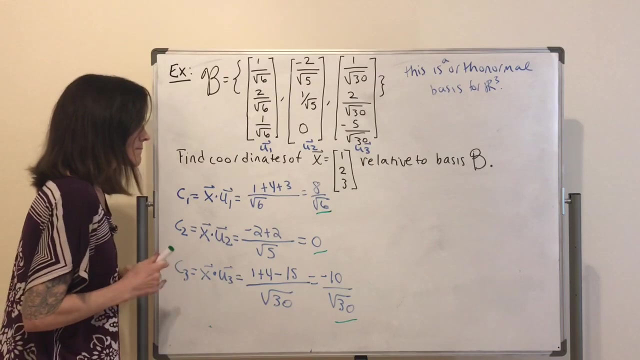 it's going to be all over the square of 30 and we get 1 plus 4 minus 15 negative 10 over the square root of 30. okay, so my coordinates with respect to this basis are here: this one, this one, this one- okay, in that order. maybe I'll just write as a final observation here: 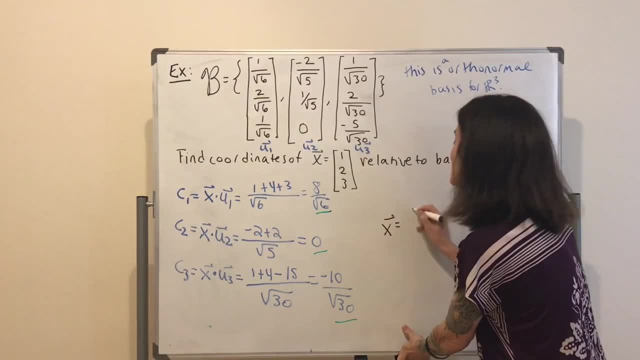 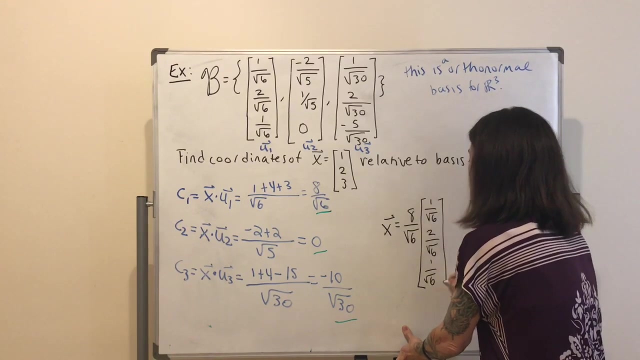 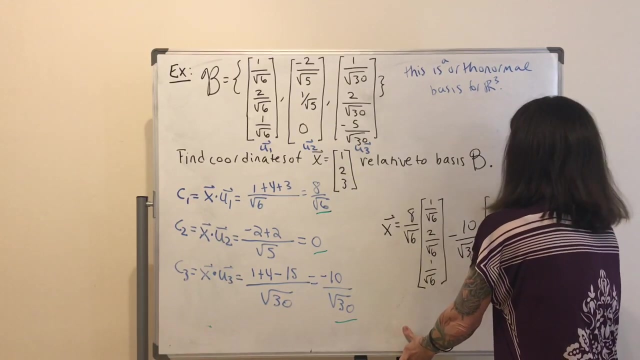 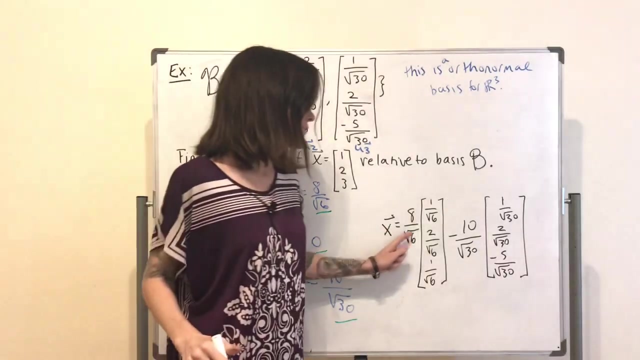 that X is equal to, we have 8 over the square root of 6 times this first vector, and then minus 10 over the square root of 30 times this third vector. like this, and you should in fact check. it's not even that hard, just if you add. 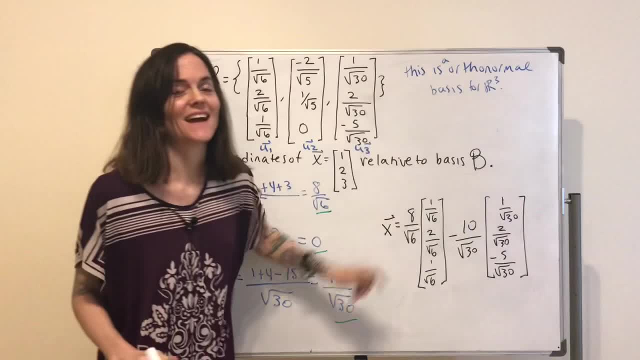 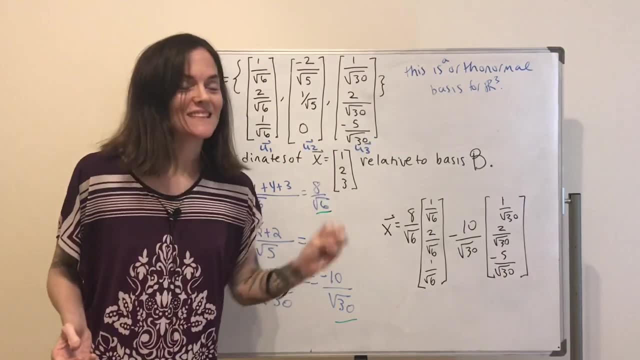 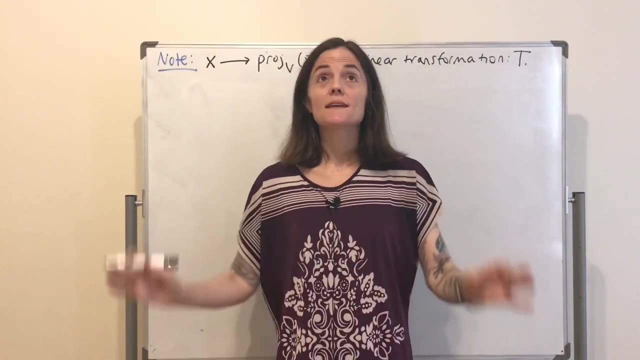 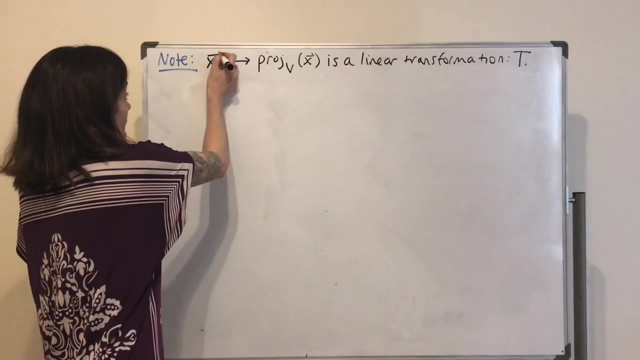 these up, you get X, you get 1, 2, 3 as the vector. so this is an example of finding these coordinates relative or respect to some orthonormal basis. let's make another note or comment about the projection onto a subspace, and that's that, if you take, this is for V. oh, I need my hat for V, a subspace of our n. 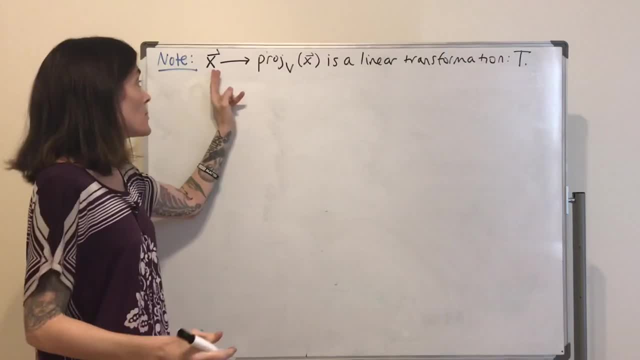 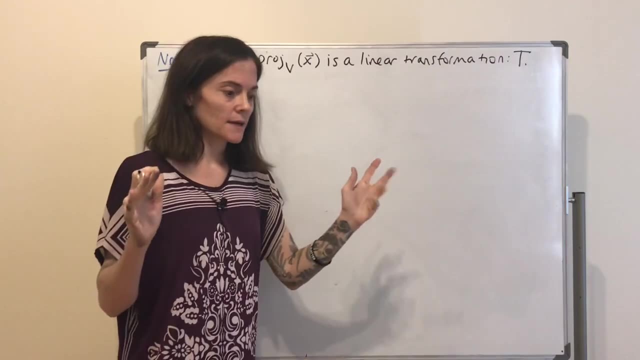 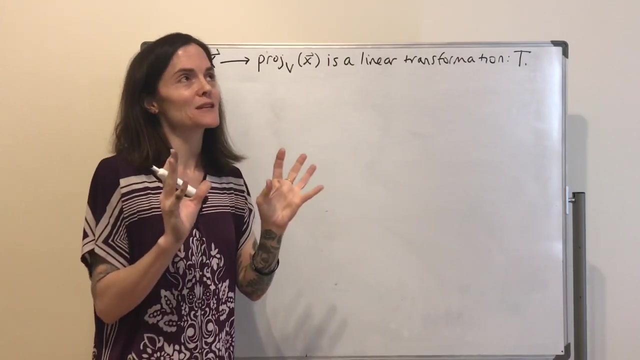 and X in our n. this map, which sends X to this vector, is a linear transformation, just like we had when, when V was just a line and and well, for instance, we found the matrix. we for well, we found the matrix when you're going from r2 to R, to 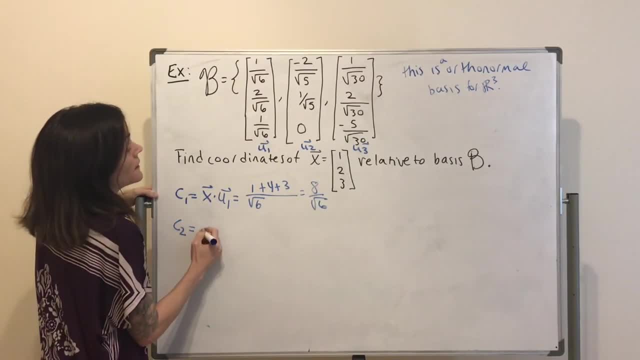 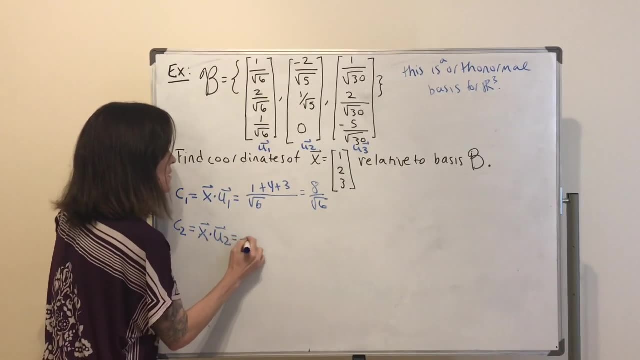 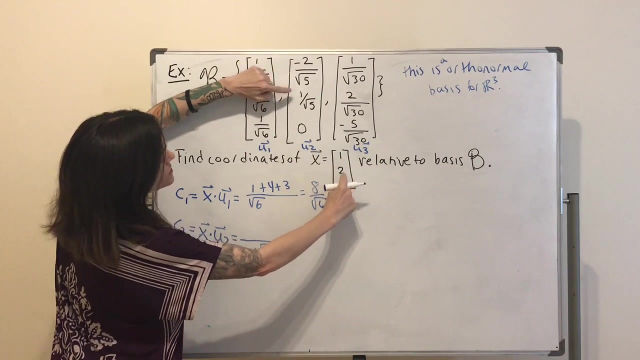 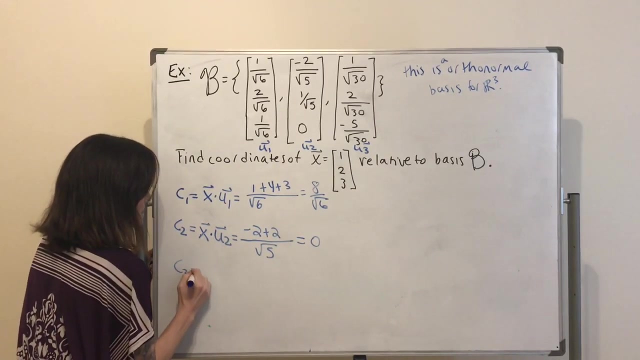 And then c2, this is going to be all over. well, I'll write it: x dot u2.. This will be all over the square root of 5.. We get minus 2 plus 2.. Oh, this is just 0.. And then c3, this is x dot u3.. 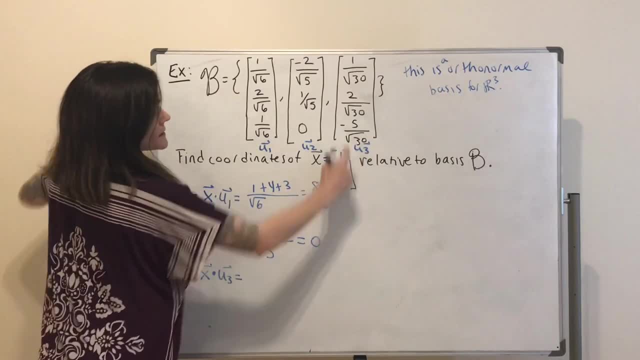 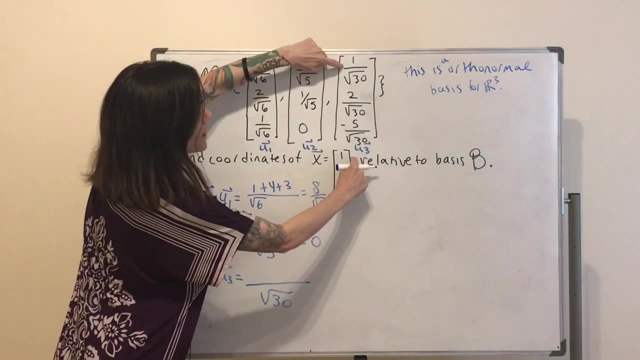 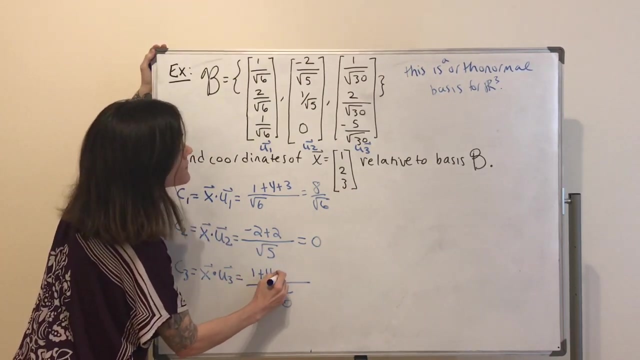 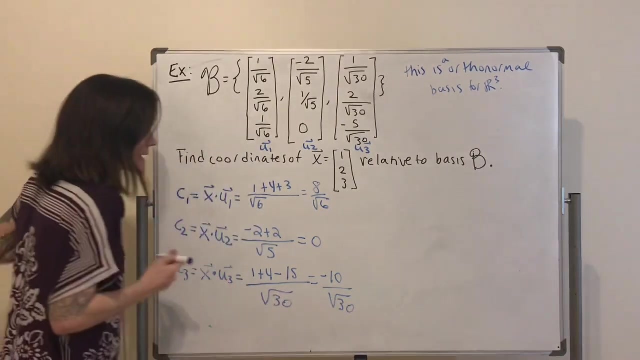 Here we go. It's going to be all over the square root of 30.. And we get 1 plus 4 minus 15.. Negative: 10 over the square root of 30.. Okay, so my coordinates with respect to this basis. 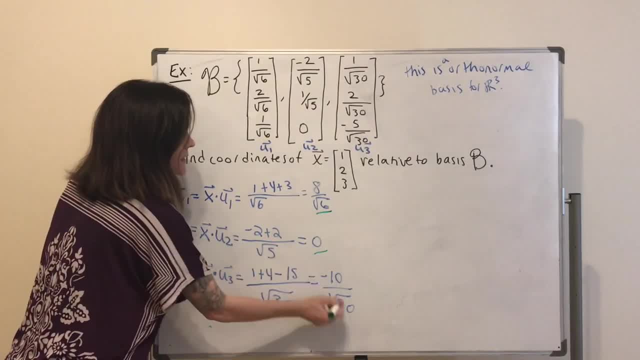 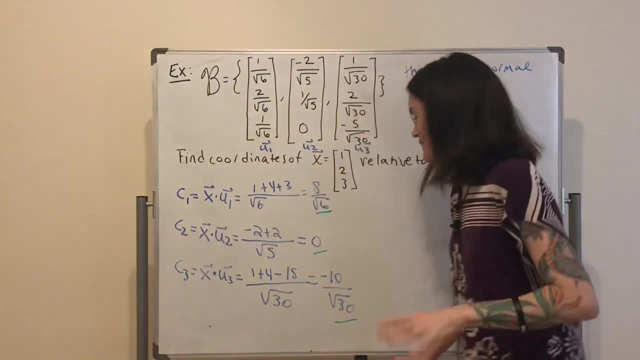 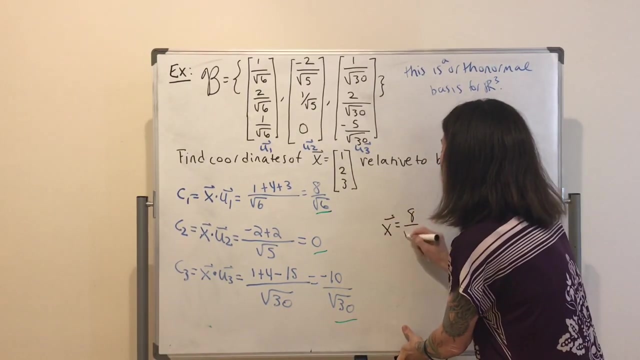 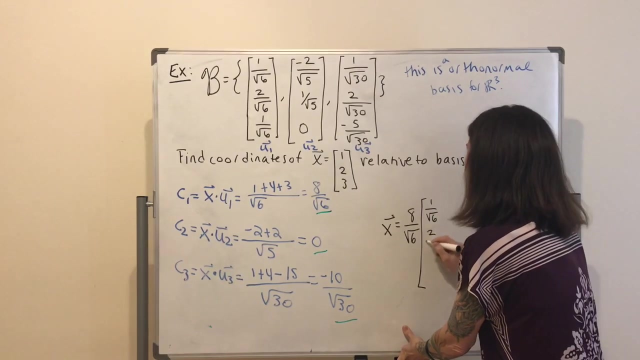 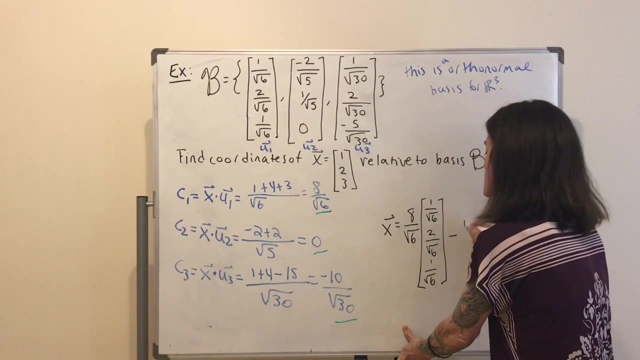 are here: This one, this one, this one- okay, in that order. maybe I'll just write as a final observation here that X is equal to: we have 8 over the square root of 6 times this first vector and then minus 10 over the square root of 30 times this third vector. 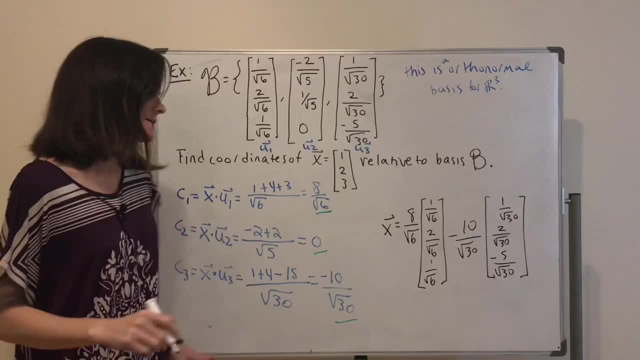 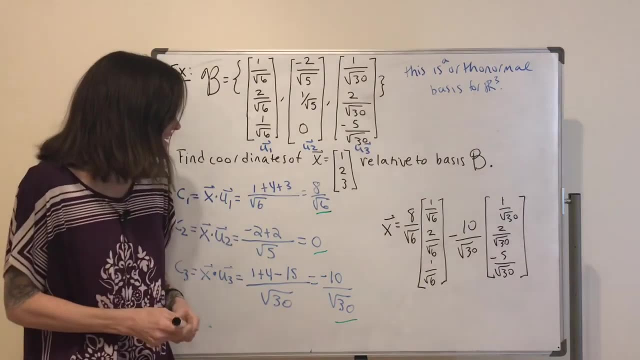 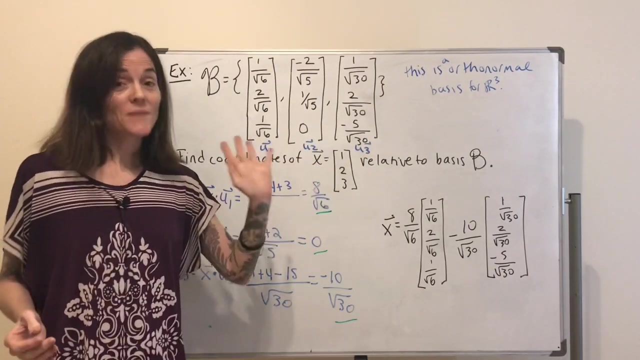 like this, and you should in fact check- is not like this and you should in fact check- is not even that hard. just if you add these up, you get x, you get one, two, three as the vector. so this is an example of finding these coordinates relative or respect to some orthonormal basis. let's make 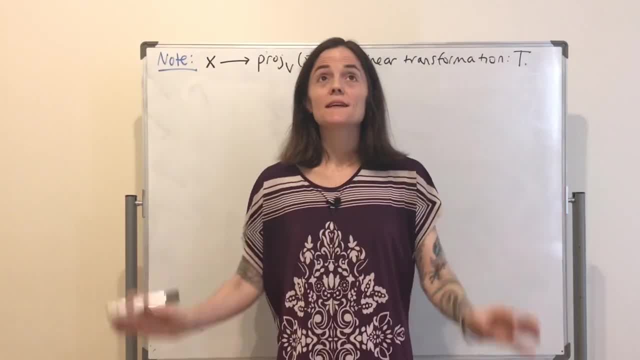 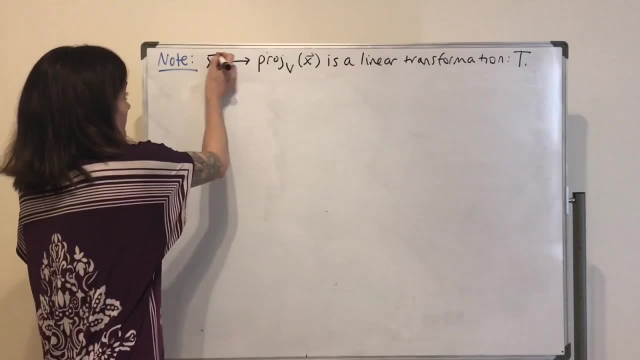 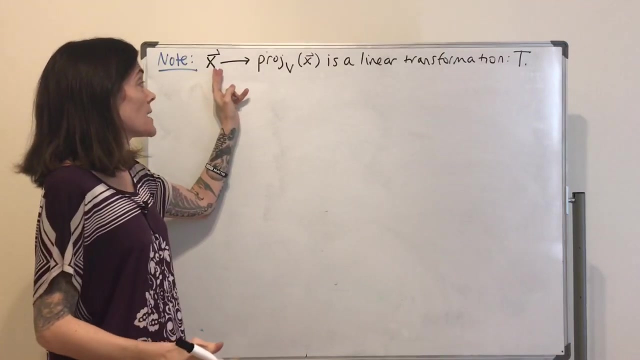 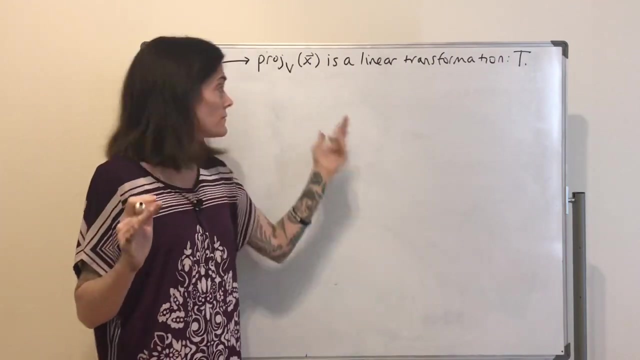 another note or comment about the projection onto a subspace, and that's that, if you take, this is for v- oh, i need my hat for v- a subspace of rn and x in rn. this map, which sends x to this vector, is a linear transformation, just like we had when, when v was just a line and and well, for instance, 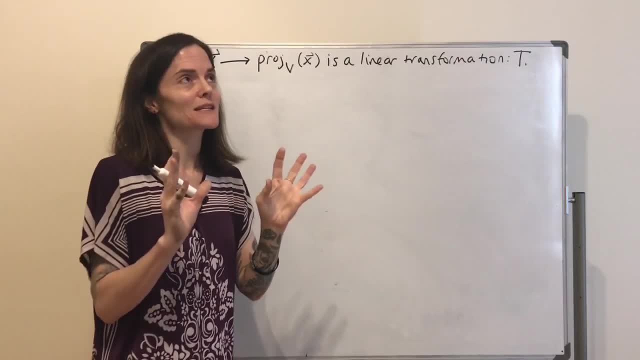 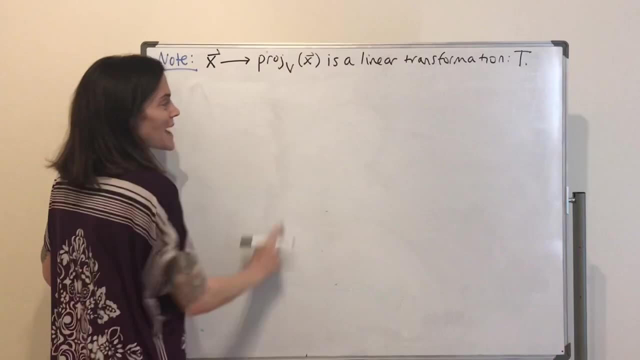 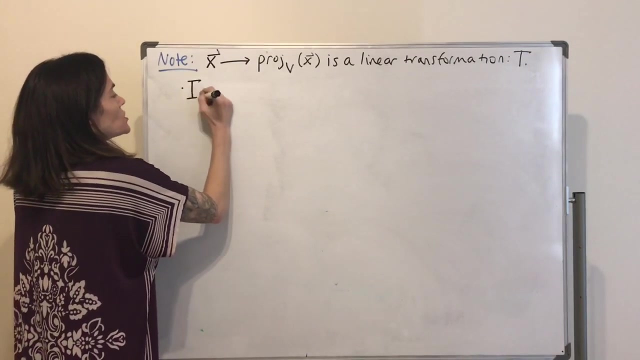 we found the matrix. we for, well, we found the matrix. when you're going from r2 to r2, we had this little two by two. in any case, generally, this map is a linear transformation. let's call it T, okay. what do we know? we know the image of T is V itself. but then, 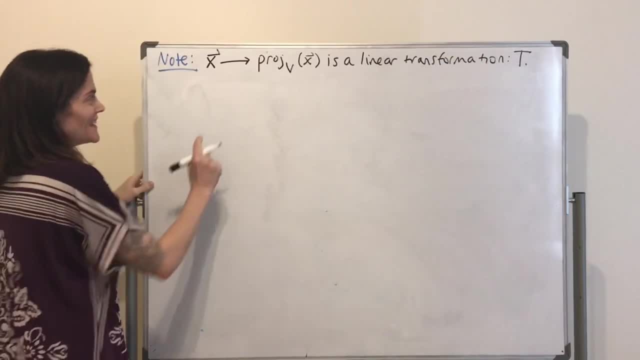 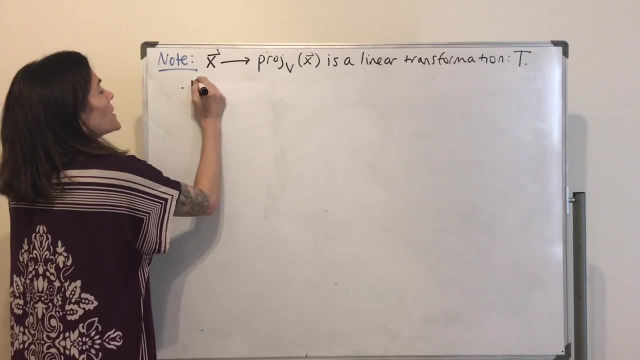 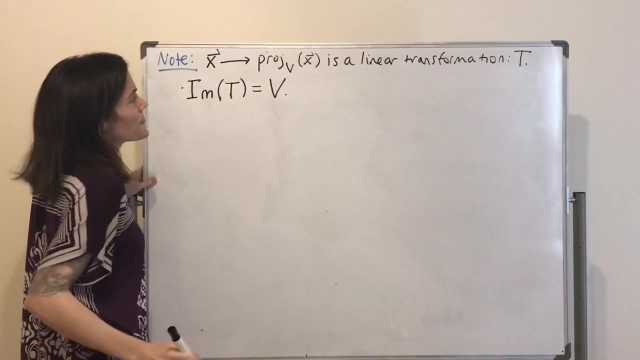 we have this little 2 by 2, and anycase, generally, this map is only a transformation. let's call it T. okay, what do we know? we know the image of T is V itself, but then what's interesting is the kernel. this has a name. the way this набt. I wanted this and let's see what happens when you find all of the collaborators. all of them have their own to its end. so what this does, I found, is the Magnesium-Base matrix, which is re- scratch image of this matrix, validates, and this is so important, with the prediction basis. we've Ellie, who represents the all of our ways of expression in both ways, and this is what it does. so what you can determine if you find what this slide достens on ты, если у тебя есть methodник呢. 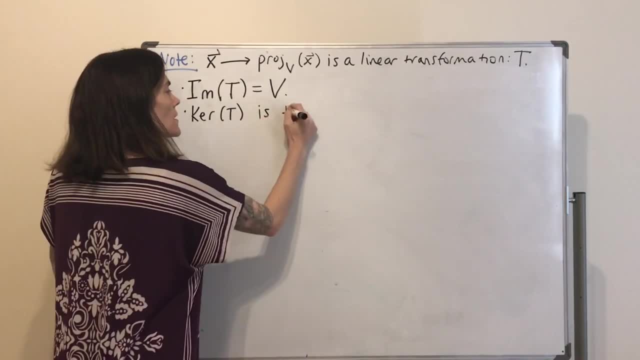 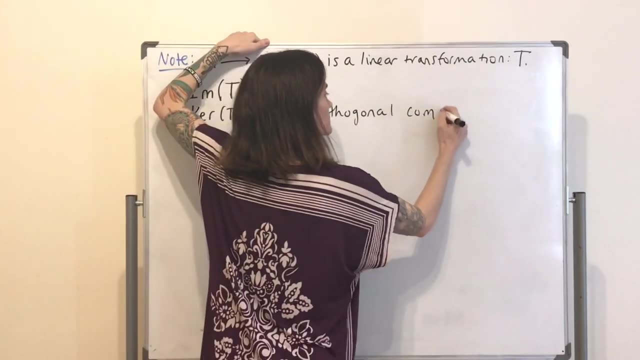 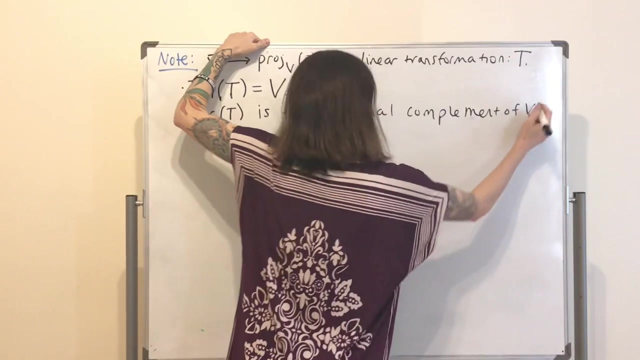 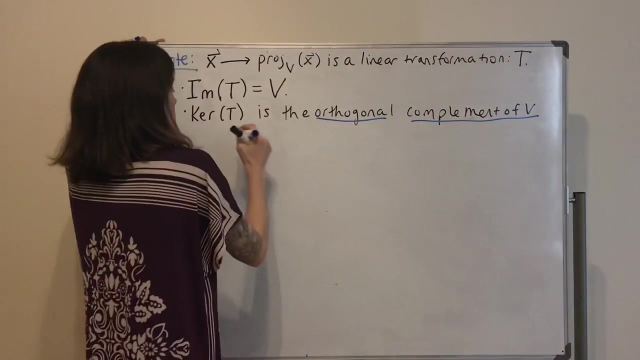 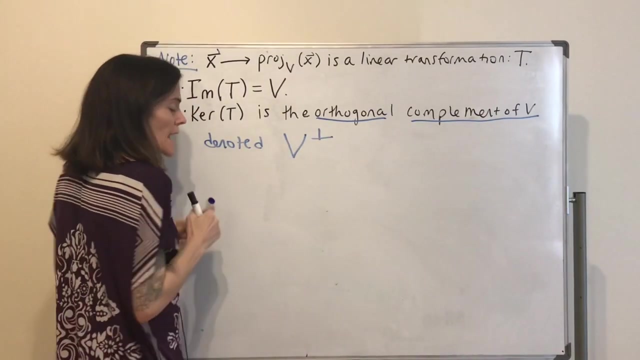 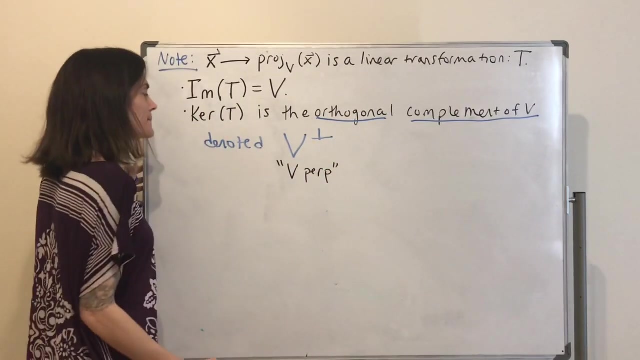 This is what's called the orthogonal complement of V, And this is what I'm defining here: orthogonal complement of V. And this is denoted like this, And this is read: V perp, V, perp. okay, And if we wanna write this as a set, 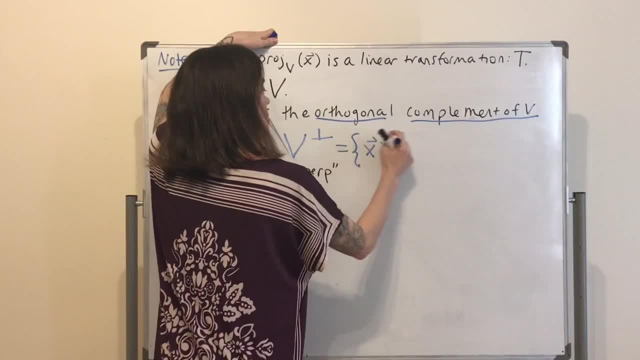 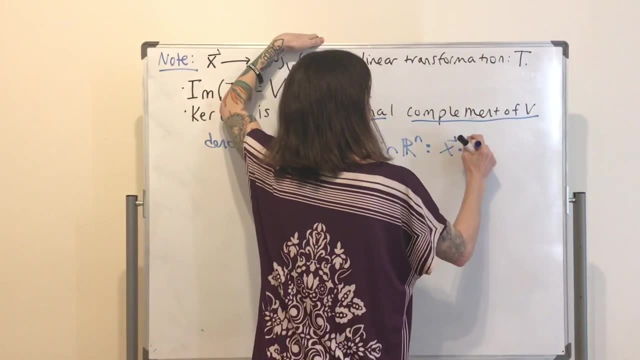 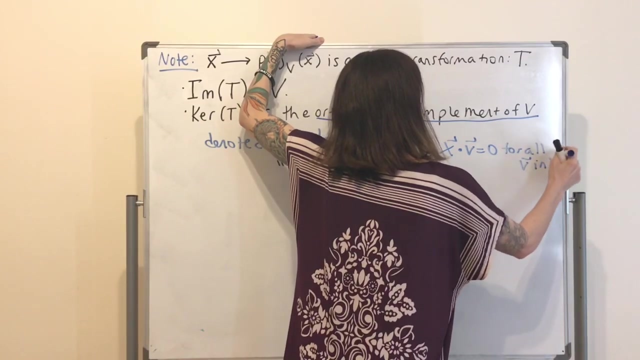 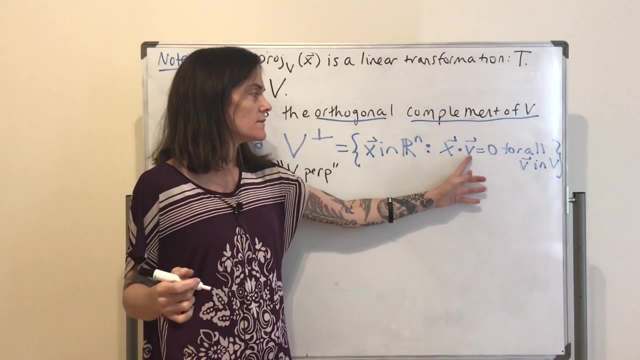 this is the set of all X in Rn, such that, well, XV is zero for all V in Rn, But just as we discussed, it's also equivalent to say that XV is zero for all V in a basis of V. okay, 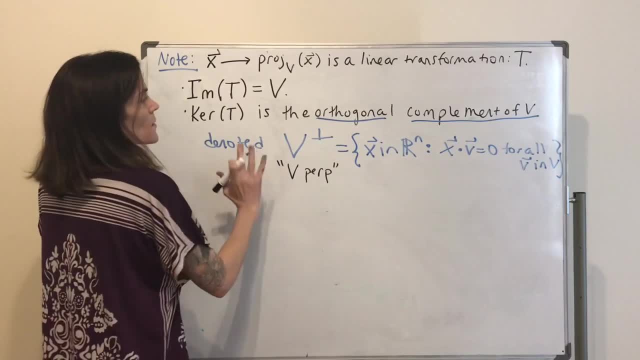 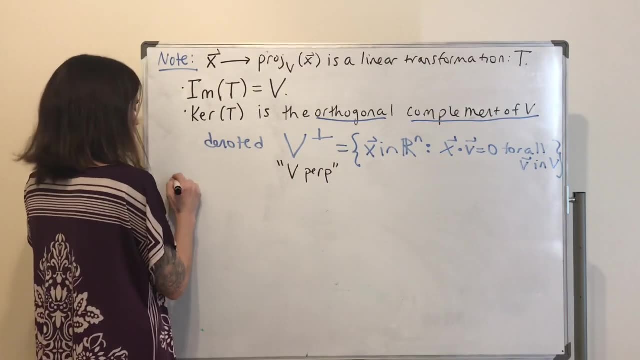 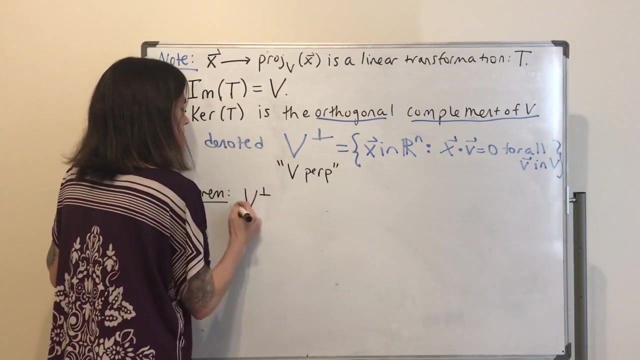 Might have been two examples ago, But this is what the orthogonal complement of a subspace is. Now, what can I say about this? Maybe I'll write this as a theorem. First of all, this one is a subspace of Rn. 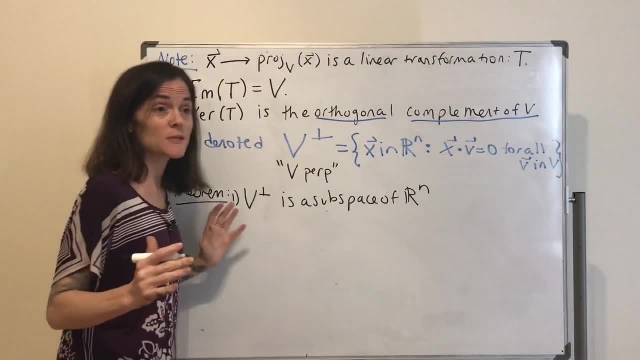 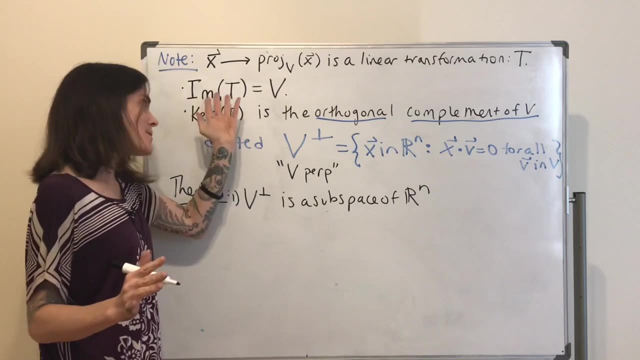 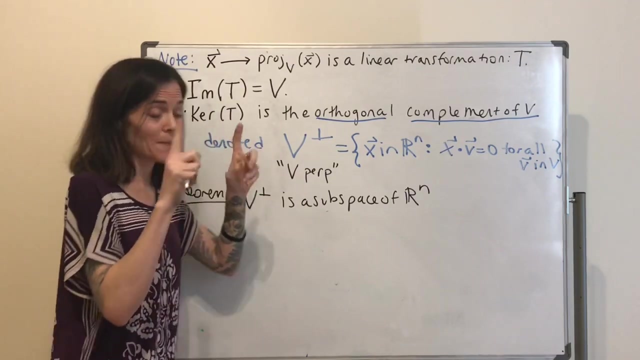 Why is it a subspace? Well, look, it's the kernel of a transformation, And we know kernels and transformations, and images of transformations for that matter, are subspaces, and this will be a transformation. The corresponding matrix is n by n. 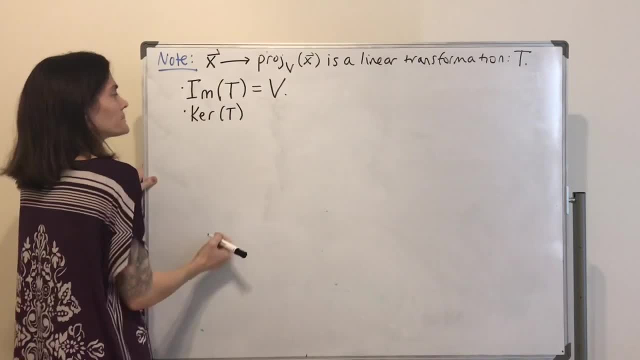 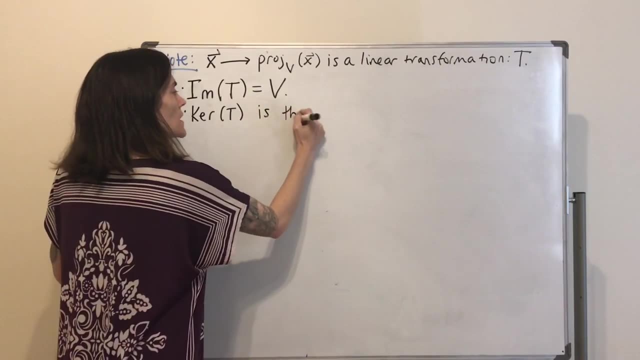 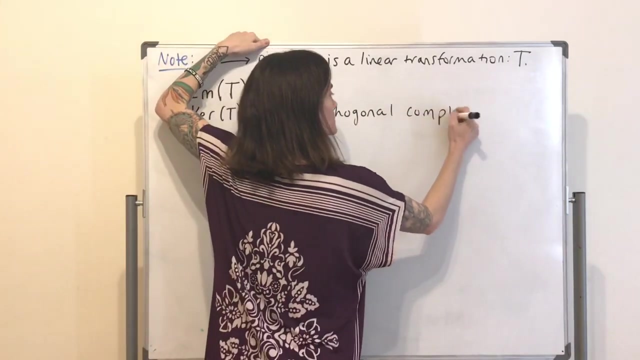 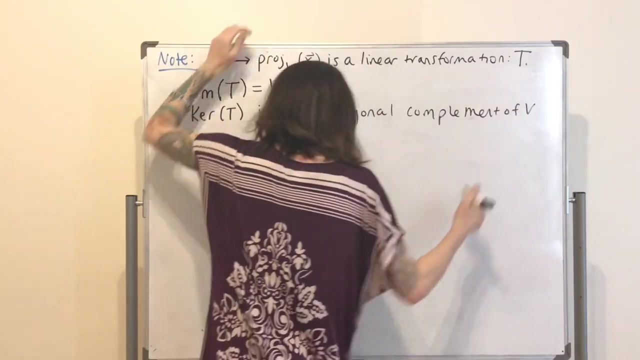 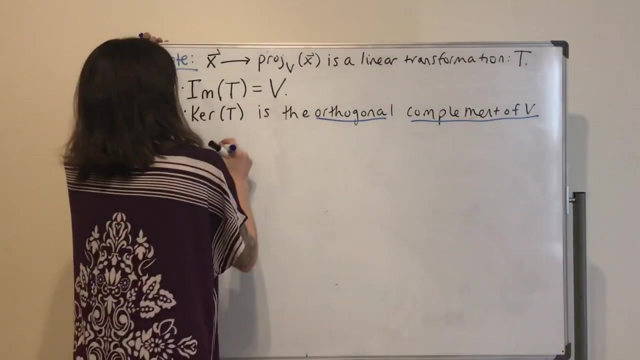 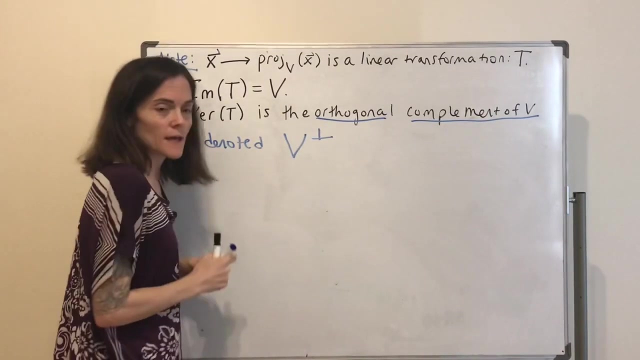 what's interesting is the kernel. this has a name. this is what's called the orthogonal complement. calm, I'm missing something. complement of V and this. this is what I'm defining here: orthogonal complement of V, and this is denoted like this, and this is red V- perp. 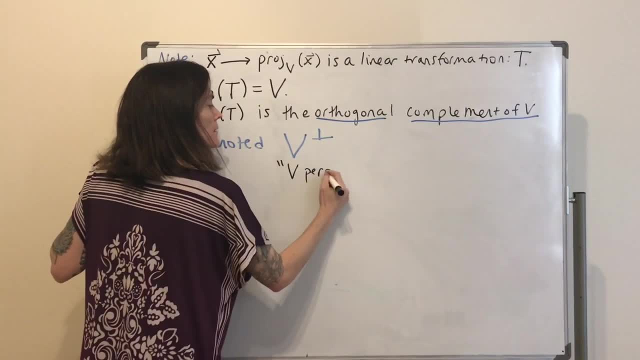 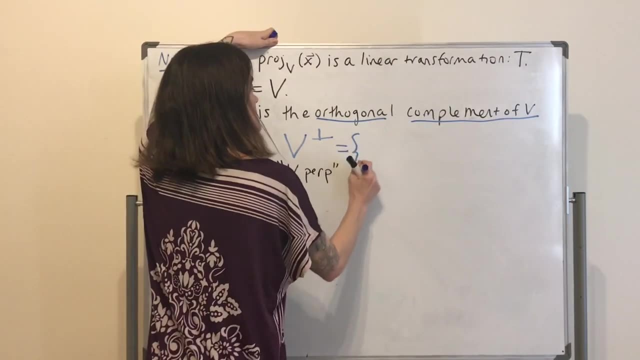 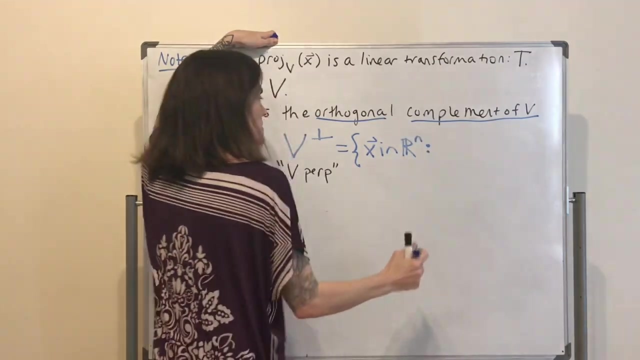 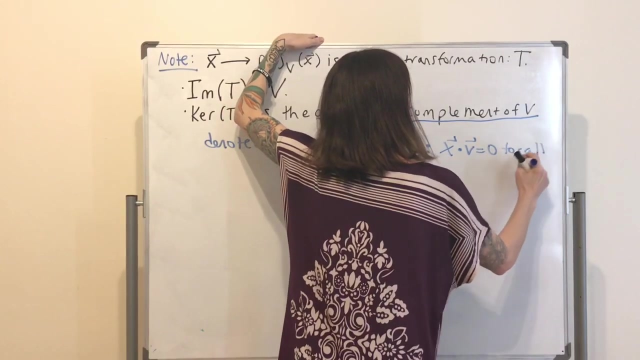 the perp, okay, and if we want to write this as a, as a set, this is the set of all X in our n, such that, well, x dot V is zero for all V in V. but just as we discussed, but just as we discussed, but just as we discussed. 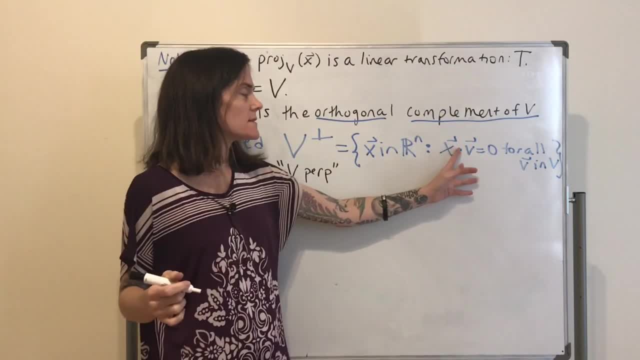 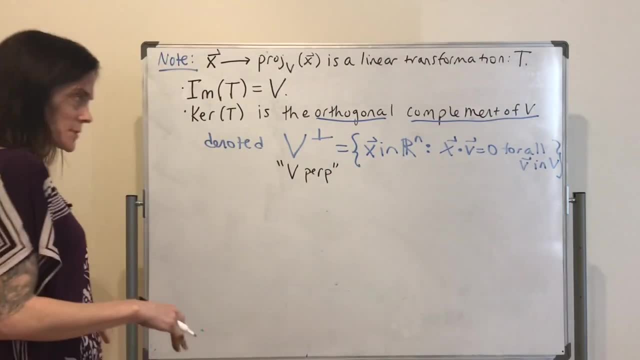 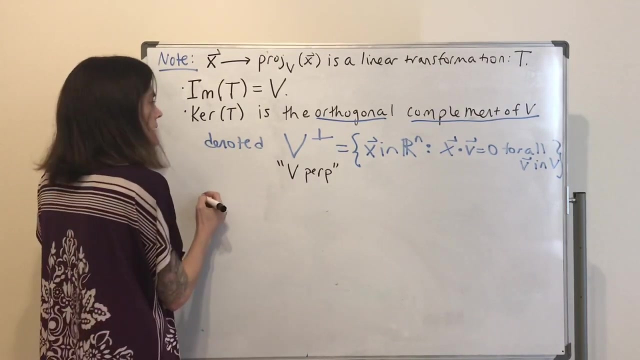 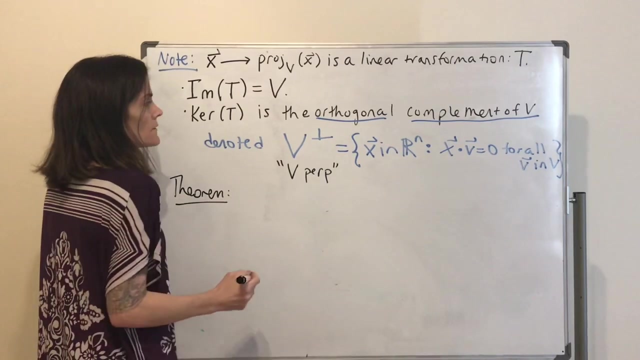 it's also equivalent to say that x dot v is zero for all v in a basis of v. okay, i've been two examples ago, but this is what the orthogonal complement of a subspace is. now. what can i say about this? maybe i'll write this as a theorem. first of all, this one is a subspace. 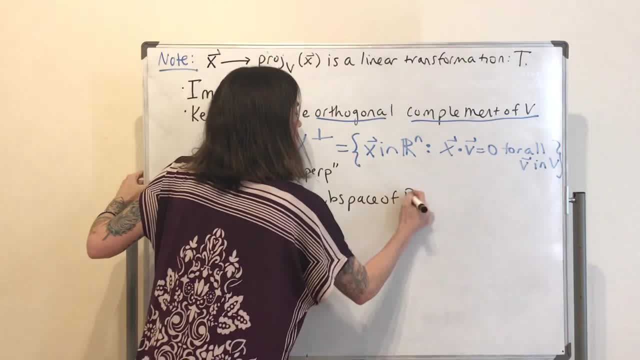 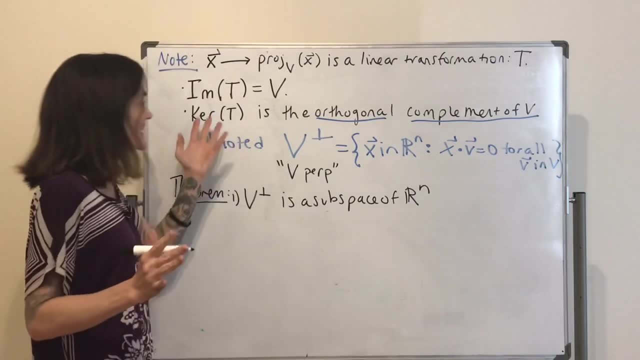 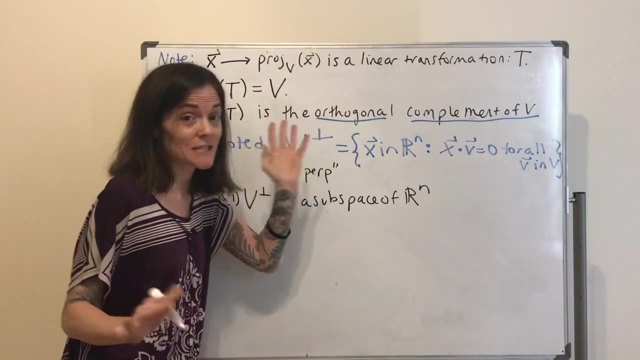 of rn. why is it a subspace? well, look, it's the kernel of a transformation, and we know kernels of transformations- and images of transformations for that matter- are subspace of rn. so what can i say about this? maybe i'll write this as a theorem: subspaces, and this will be a transformation. the corresponding matrix is n, by n, it's a. 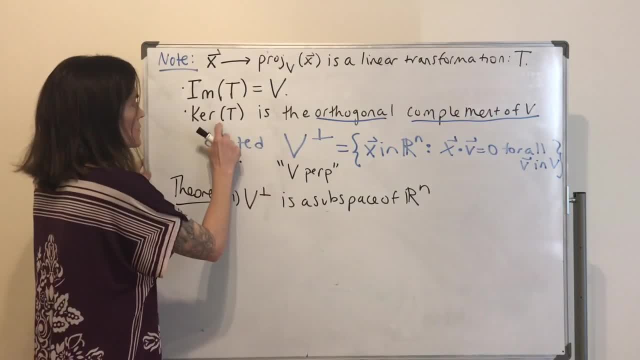 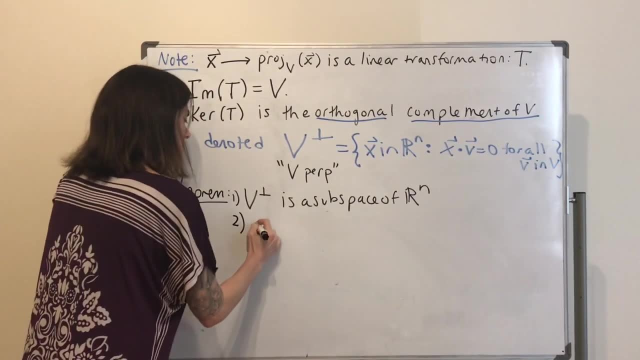 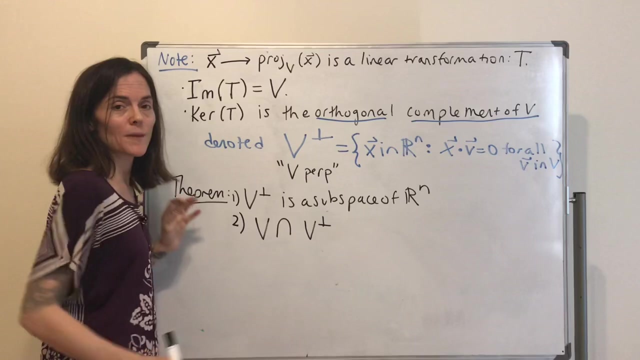 transformation from rn to rn, and so this is inside of rn and this is inside of rn. for example, what else do i have to say? if you take v intersect v, perp, if you have not seen what this is, this symbol means it's every element that is in both. so this is a set and well. 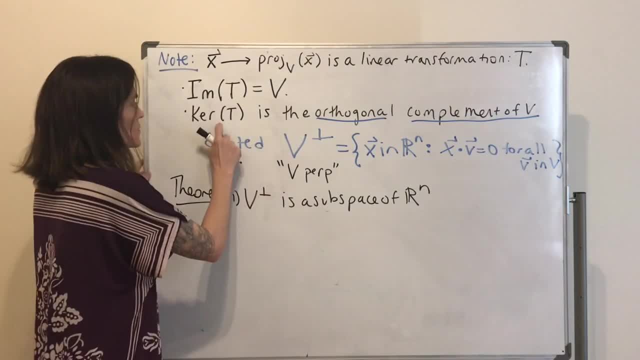 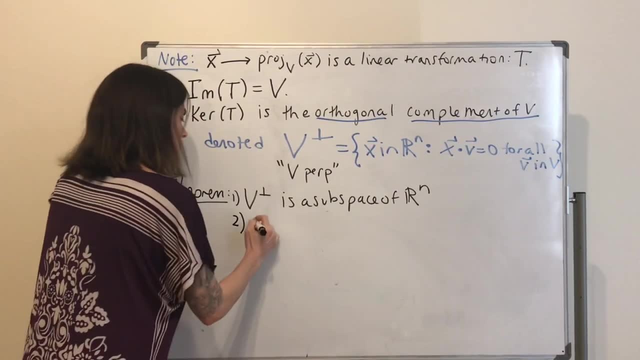 It's a transformation from Rn to Rn, Mm-hmm, And so this is inside of Rn and this is inside of Rn. For example, what else do I have to say If you take V, intersect V, perp, if you have not seen what this is. 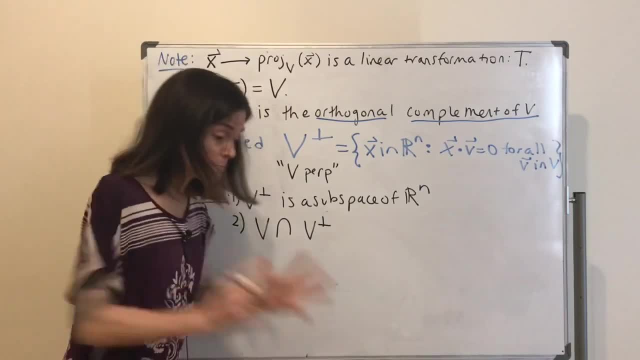 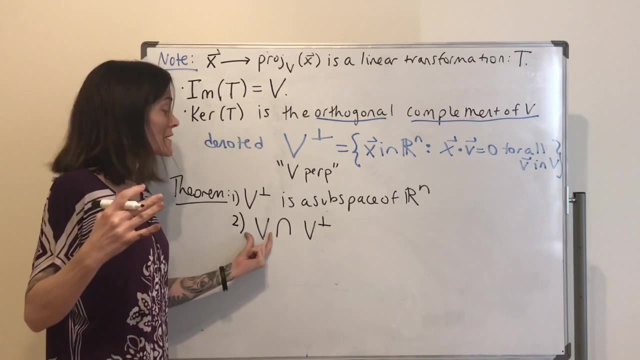 this symbol means it's every element that is in both. So this is a set. and well, to be in this set means you are in V and you are in the orthogonal complement of V or V perp. This is just zero. 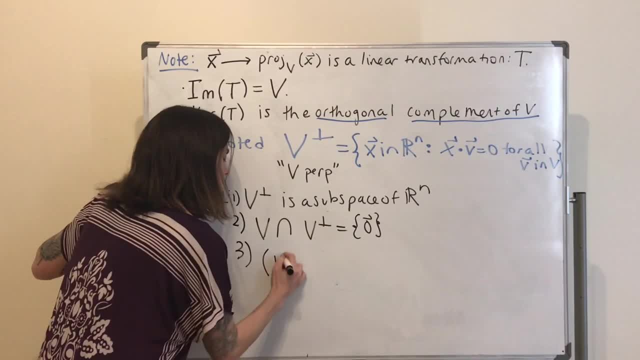 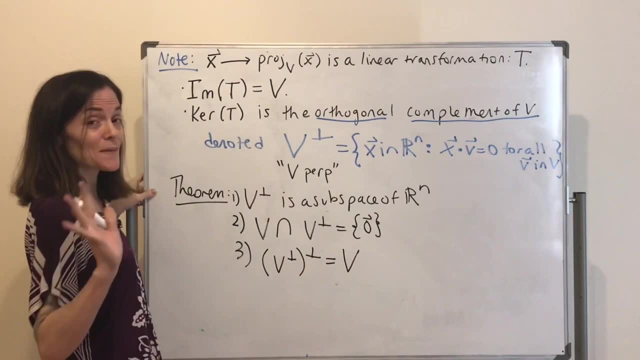 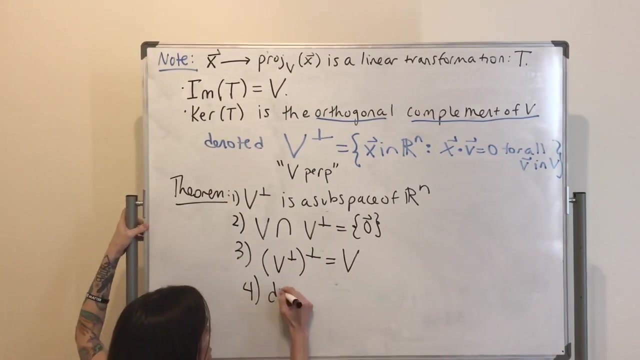 Okay, what else do I want to say about this? If you take an orthogonal complement and then you take its orthogonal complement, you get back the original subspace, And the final thing is about dimensions, That the dimension of V plus the dimension of V perp. 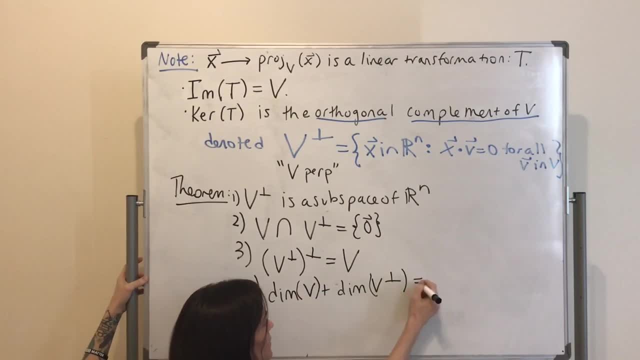 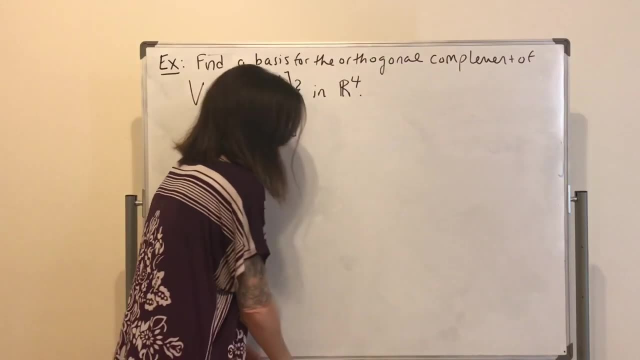 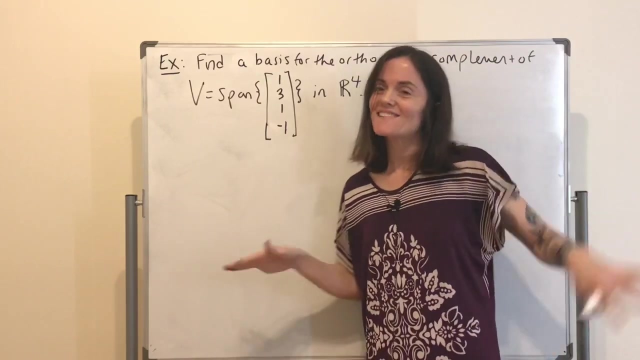 Maybe I need parentheses. Equals n. This one comes from rank nullity theorem. Here's our first example. This is a vector in R4.. V is one-dimensional. We are going to be looking for a three-dimensional subspace in R4,. 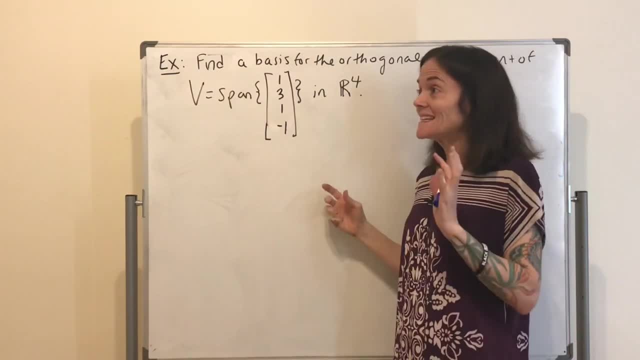 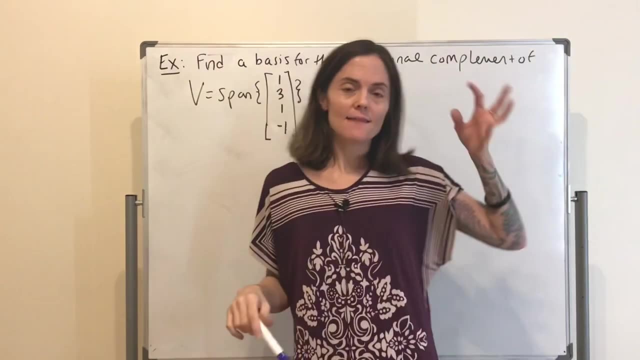 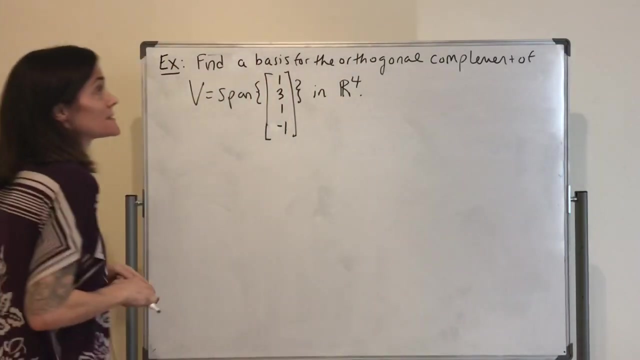 which is the orthogonal complement of V. So we need to find three vectors to have a basis- And you notice, I don't say anything about orthonormal basis or anything like that, Just some basis. So how could we possibly do this? Well, what do we know? 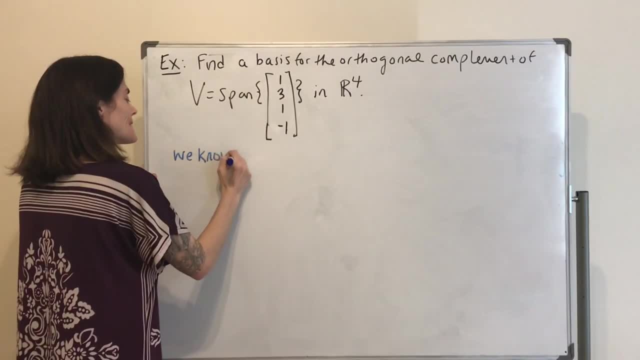 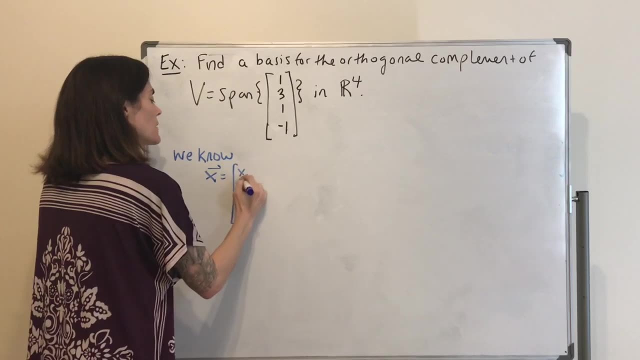 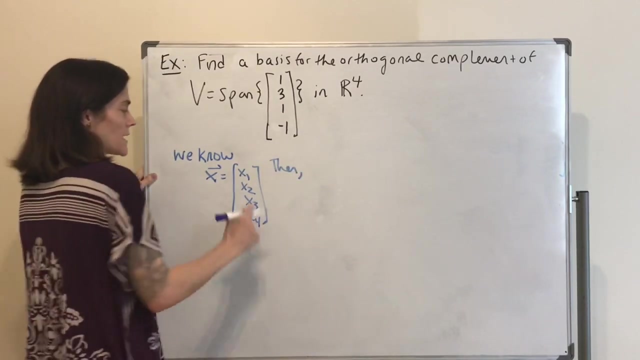 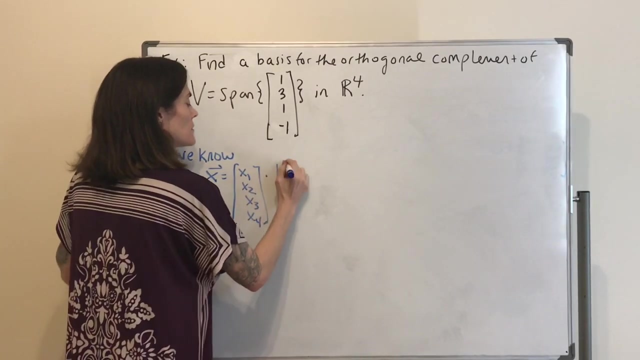 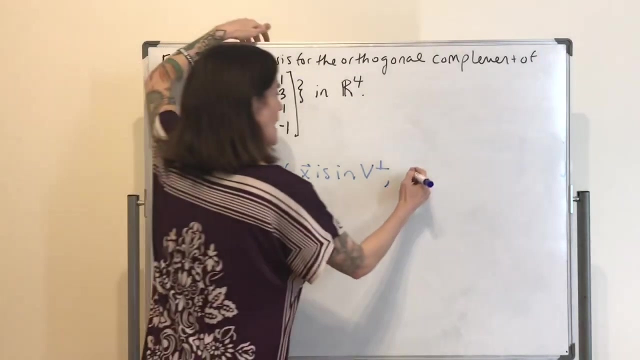 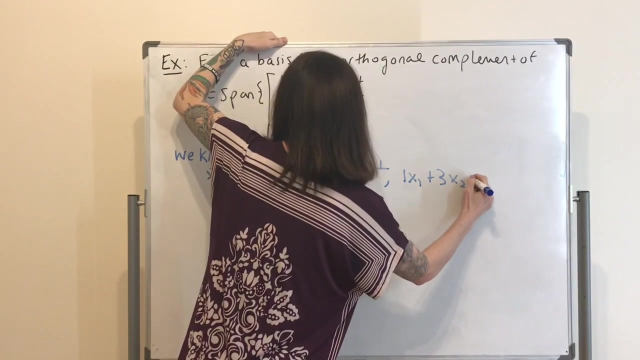 We know, let's say X is X1, X2, X3, X4.. Then we must have: If X is n, oh, I should put that: Oh, if X is n, V perp, We must have that 1X1 plus 3X2 plus 1X3 minus 1X4 is 0.. 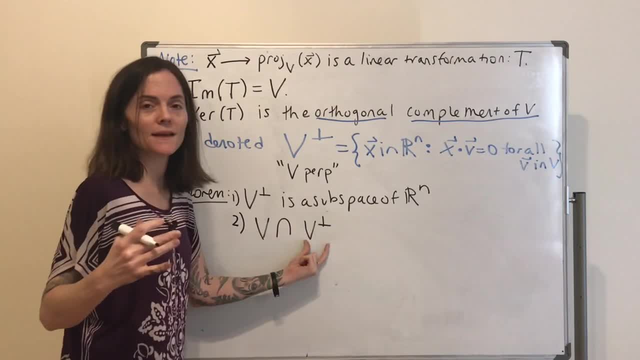 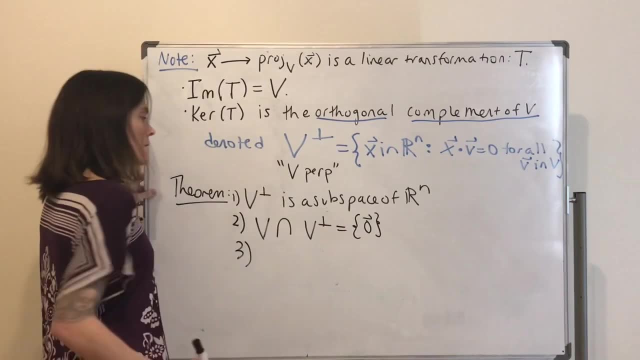 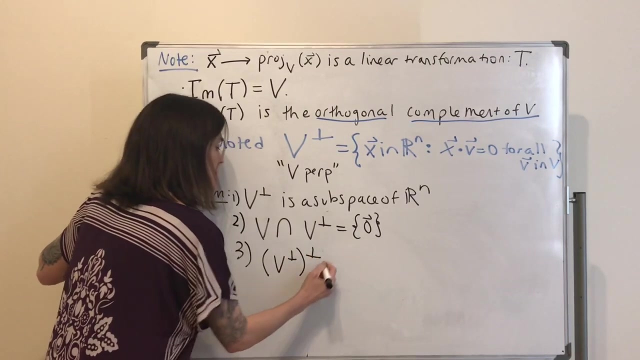 to be in this set means you are in v and you are in the orthogonal complement of v or v perp. this is just zero, okay. what else do i want to say about this? if you take an orthogonal complement and then you take its orthogonal complement, you get back the original subspace. and the final thing is about: 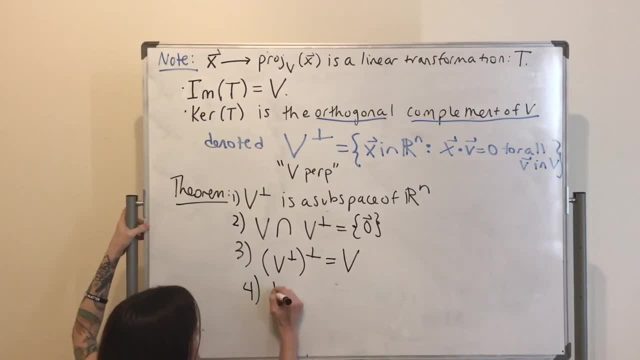 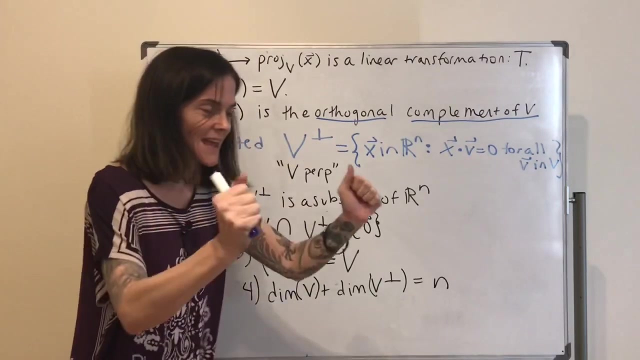 dimensions, that the dimension of v plus the original subspace is zero. so this is a set. and then you take the orthogonal complement, and then you take the orthogonal subspace, and then you take the orthogonal subspace, and then you take the orthogonal plus the dimension of v perp- maybe i need parentheses- equals n. this one comes from rank. 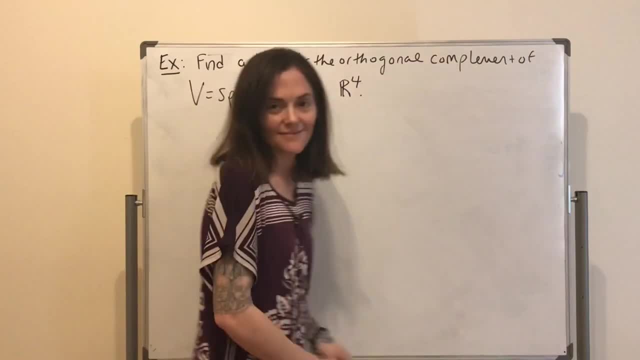 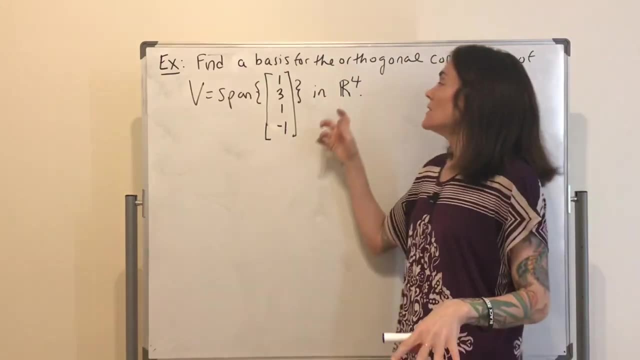 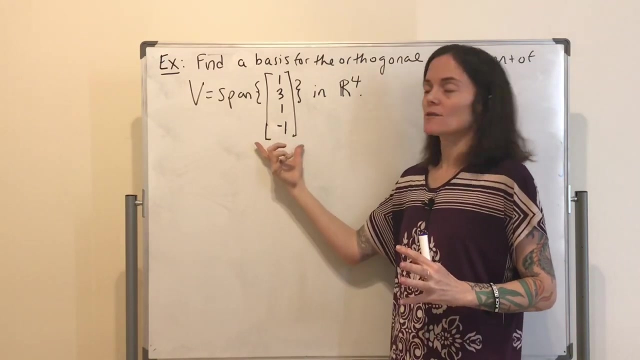 nullity theorem. here's our first example. this is a vector in r4. v is one dimensional. we are going to be looking for a three-dimensional subspace in r4 which is the orthogonal complement of v, and then we're going to take the orthogonal complement of v and we're going to take the orthogonal 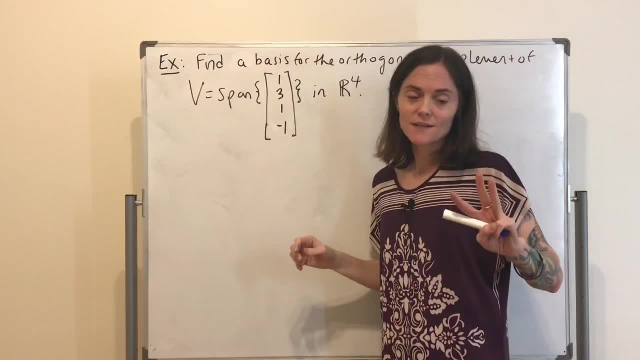 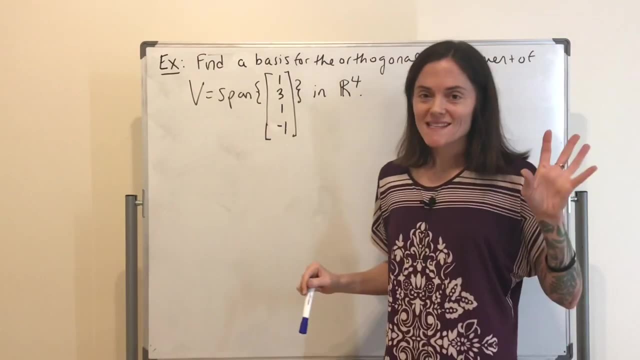 complement of v and we're going to take the orthogonal complement of v. so we need to find three vectors to have a basis- and you notice, i don't say anything about orthonormal basis or anything like that, just some basis. so how can we possibly do this? 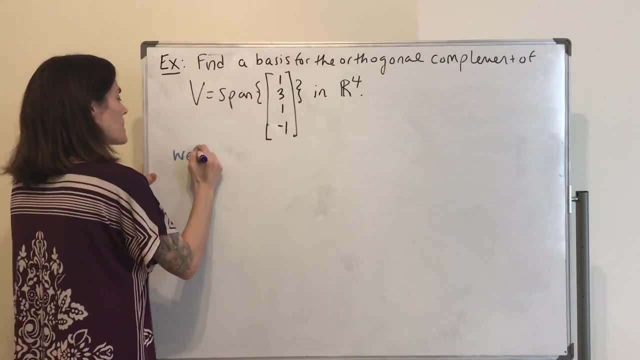 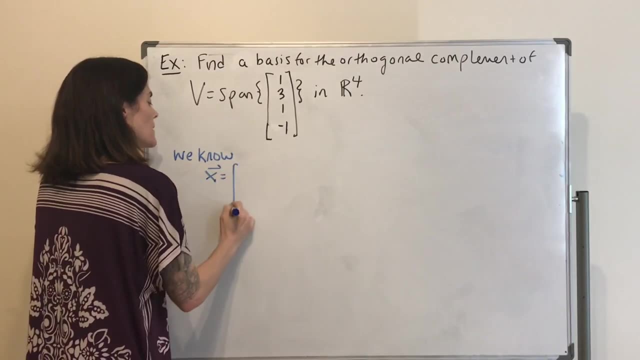 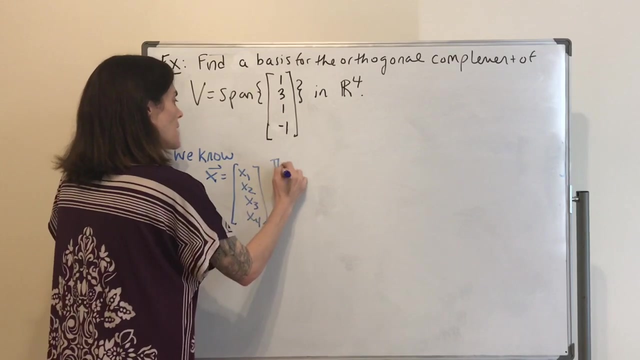 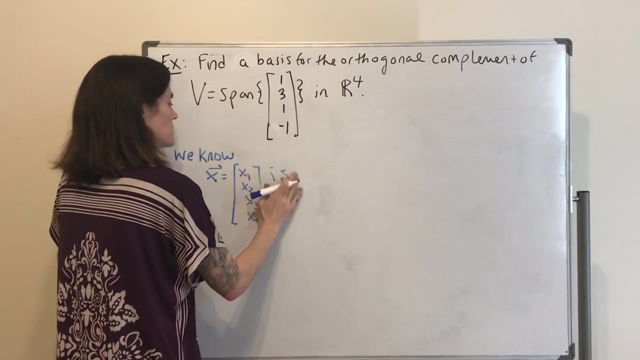 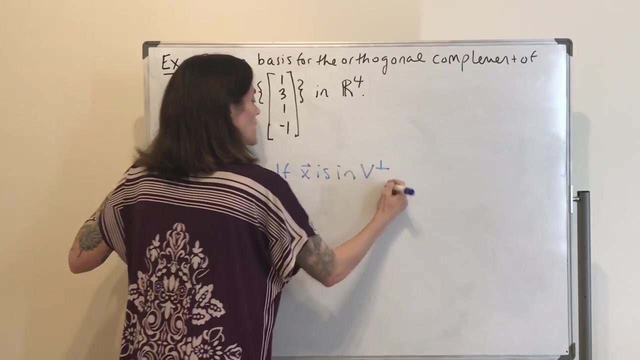 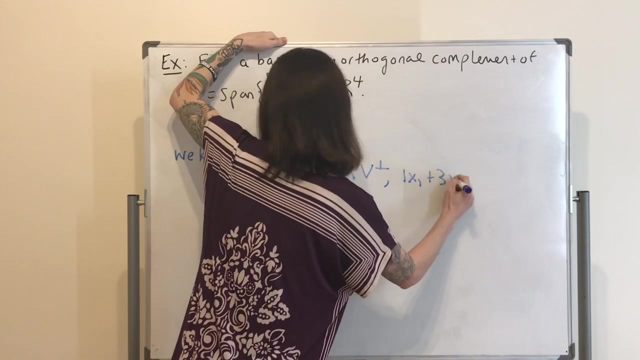 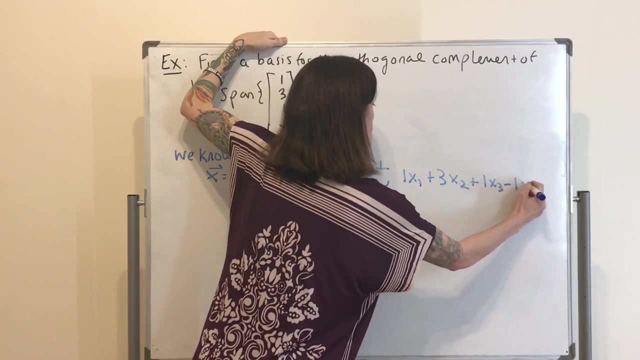 well, what do we know? we know, let's say x is x1, x2, x2, x3, x4, then we must have: if x is in- oh, I should put that- oh- if x is in the perp, we must have that 1x1 plus 3x2 plus 1x3 minus 1x4 is 0.. This is the dot product of this. 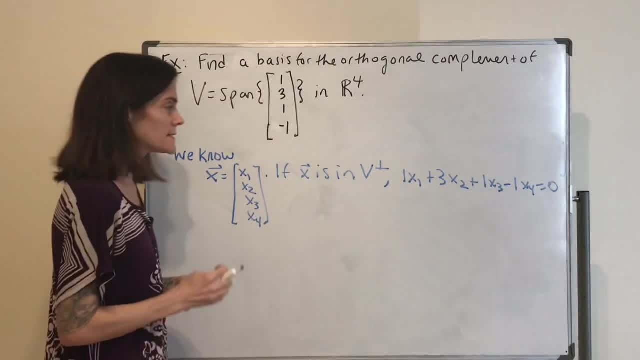 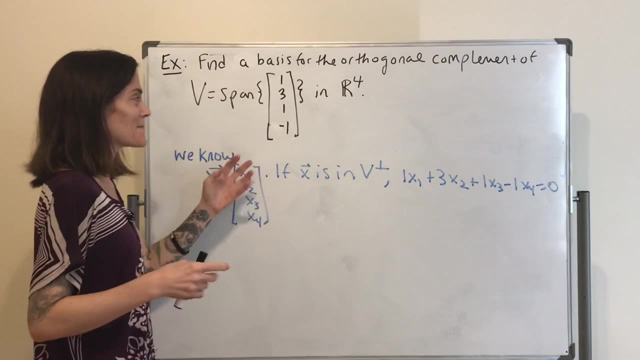 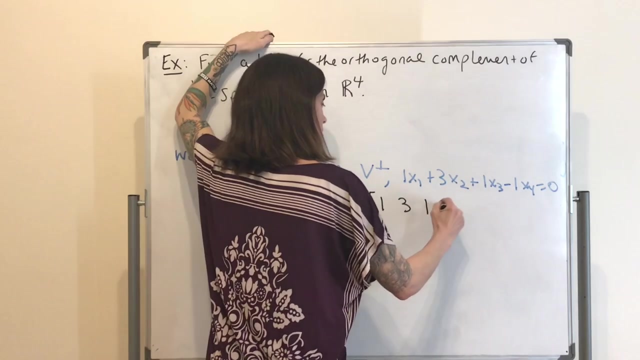 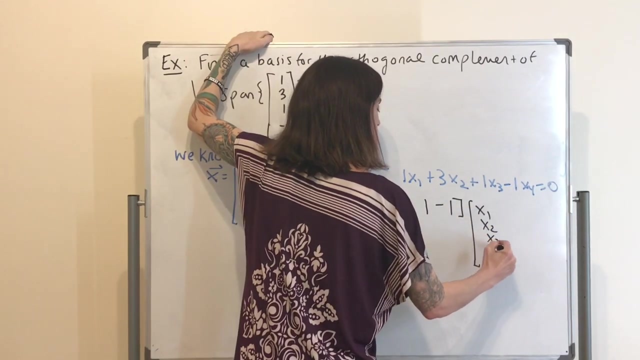 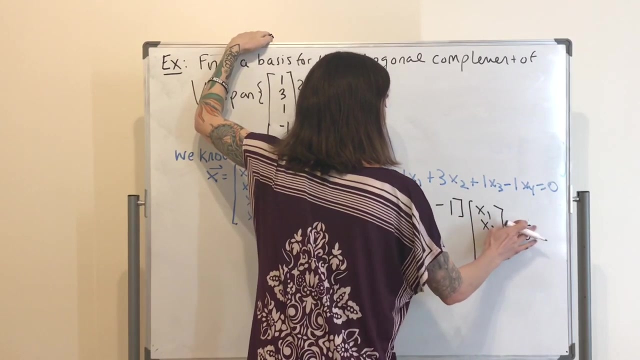 This is the dot product of this And this right, Okay, Well, because I'm going to be moving into more than just a one-dimensional subspace, V notice. this is this. This is this. Well, Okay, I won't put a hat because it is just a number in this case. 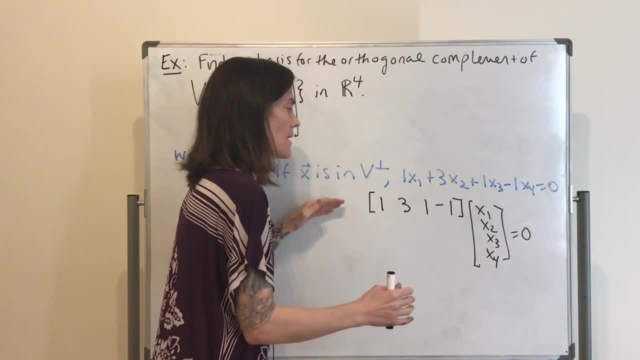 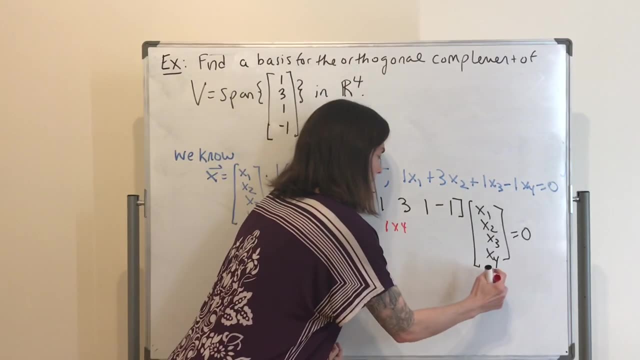 But what we see here, look, this is really, if you want to think about it, you can think about it, as this is a 1 by 4 matrix And this is a 4 by 1 vector, And it's saying that this vector is in the kernel of this matrix, right? 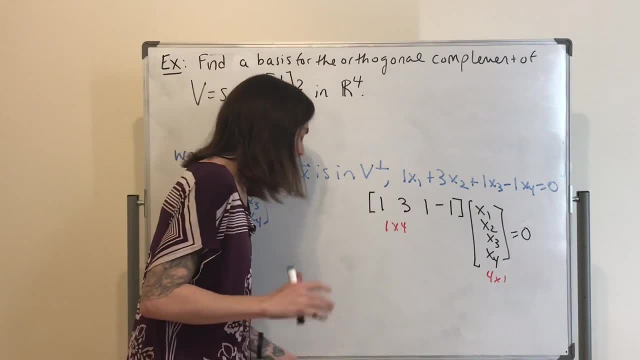 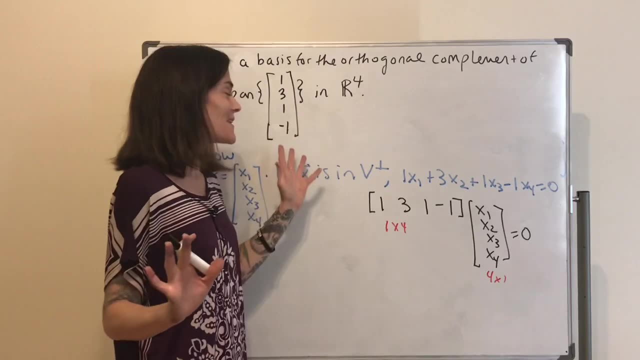 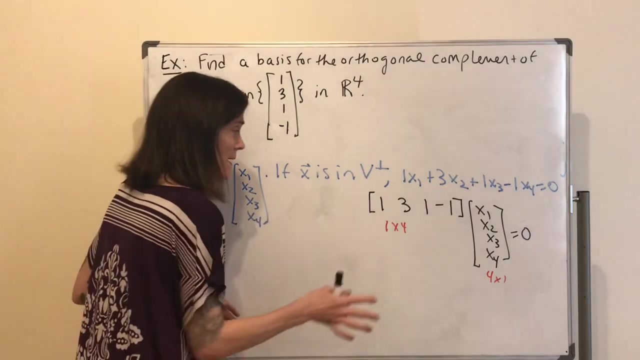 Even though it's just a vector- this one, But, But I will move to one where it's not just one vector. Okay, Let's Now, if we think about this as a matrix and we think about finding its kernel. 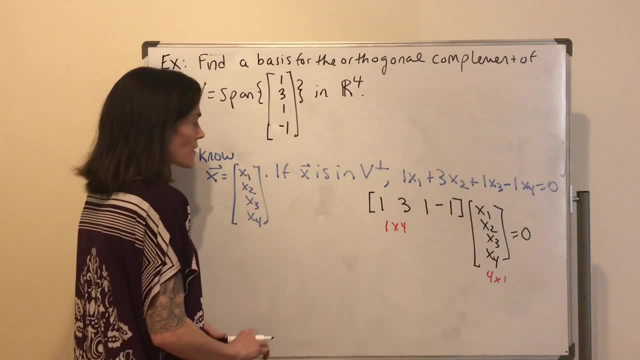 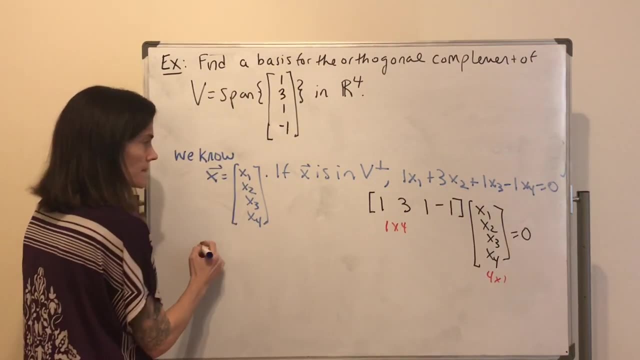 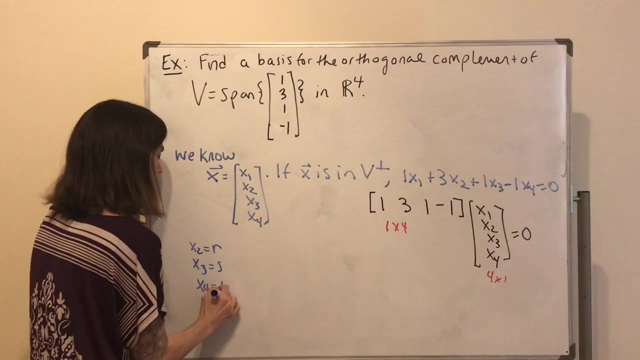 we have 1,, 2,, 3 free variables. So I would just- Maybe I'll do this here- Say X2 is R, X3 is S, X4 is T, And then I know X1 must be. Well, here's the equation. 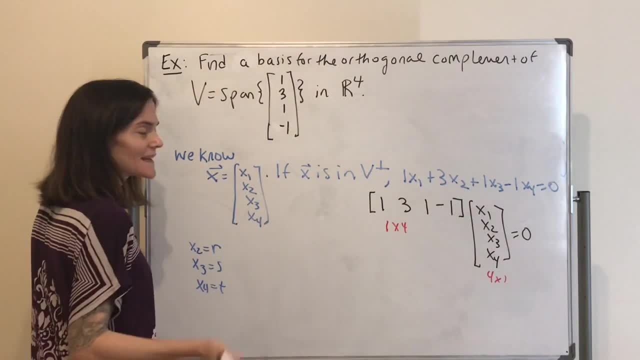 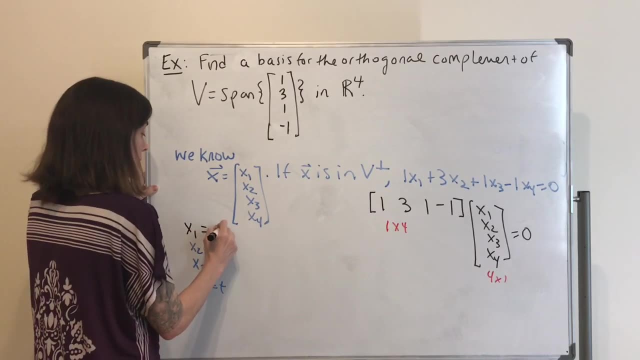 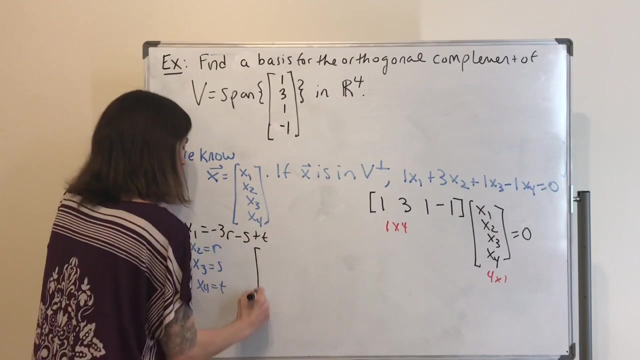 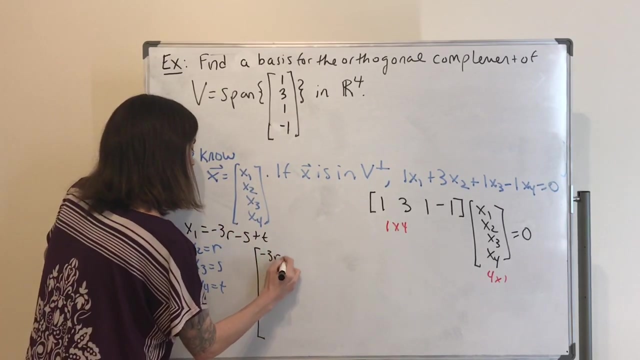 I can even look here. I was just interpreting it in terms of a matrix product below. I would know that X1 better be minus 3R, minus S plus T. So a general vector in the perp Okay Is minus 3R minus S plus T. 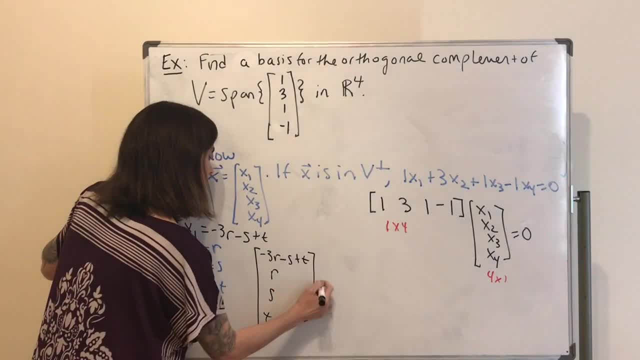 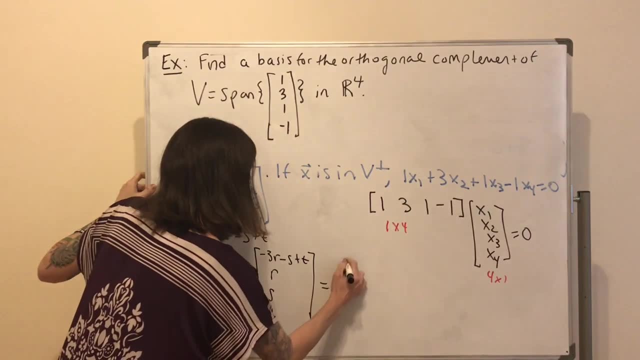 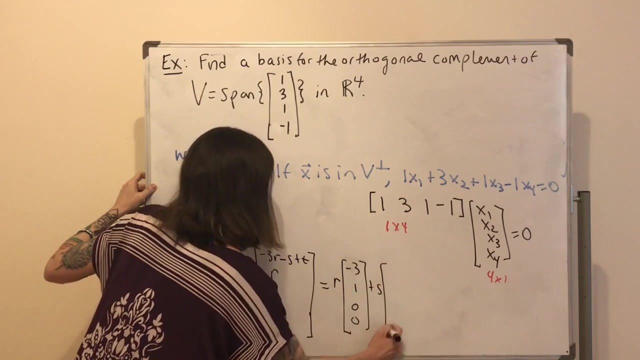 R S T And then to find the basis. Oh, this doesn't look all that great. I can just break this as R times minus 3, 1, 0, 0.. Plus S times minus 1, 0, 1, 0.. 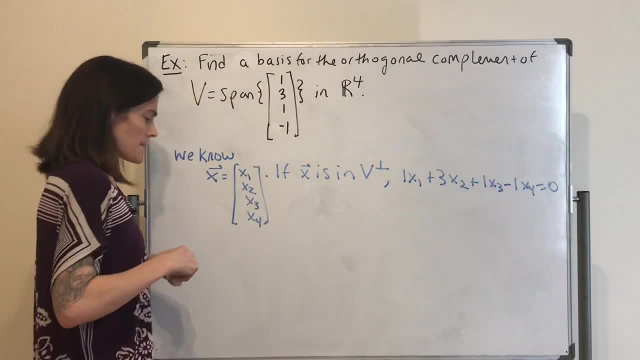 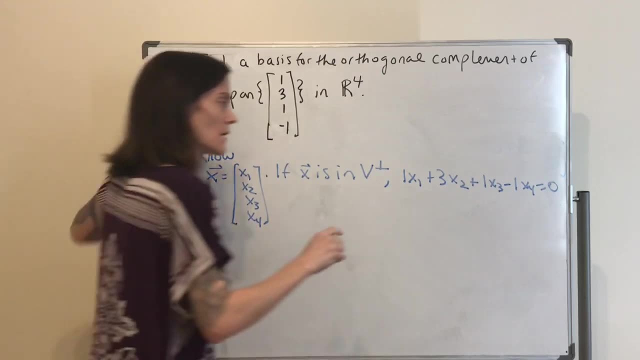 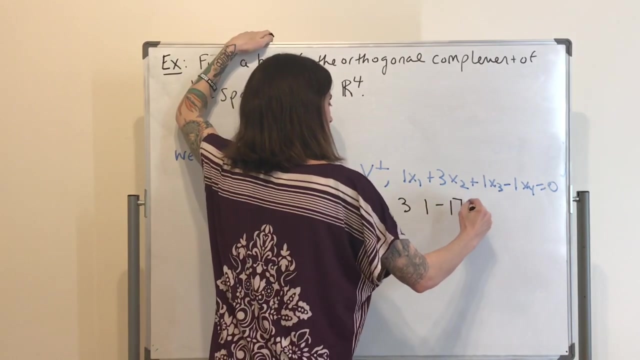 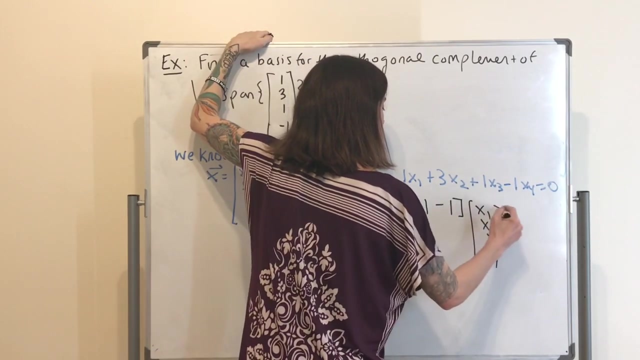 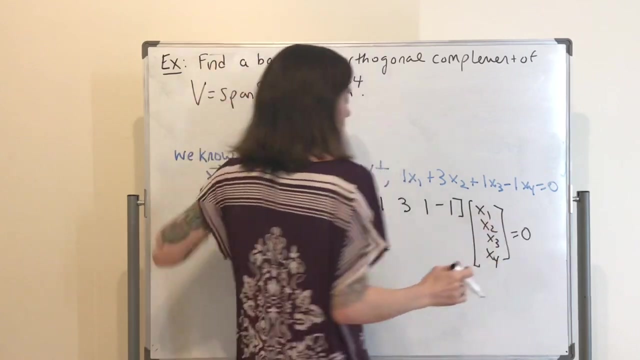 and this, right, Okay, well, because I'm going to be moving into more than just a one-dimensional subspace. B notice: this is this. Well, okay, I won't put a hat because it is just a number in this case, but what we see here, 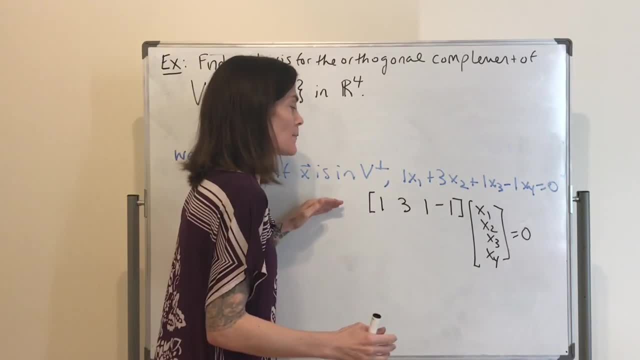 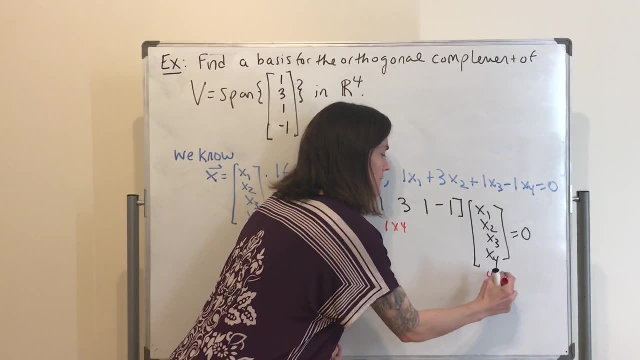 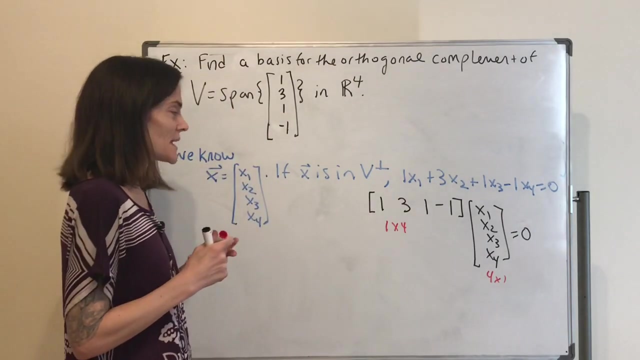 look, this is really, if you want to think about it, you can think about it, as this is a 1x4 matrix and this is a 4x1 vector, and it's saying that this vector is in the kernel of this matrix, right, Even though it's just a vector, this one. but 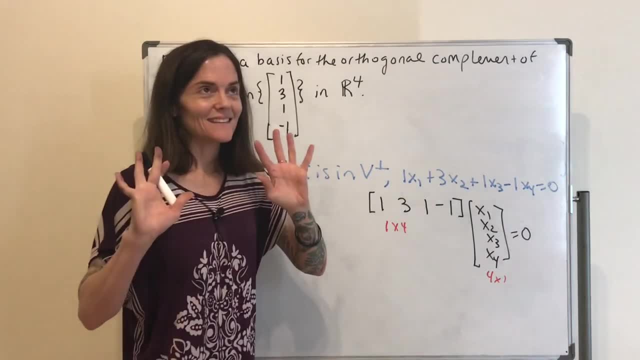 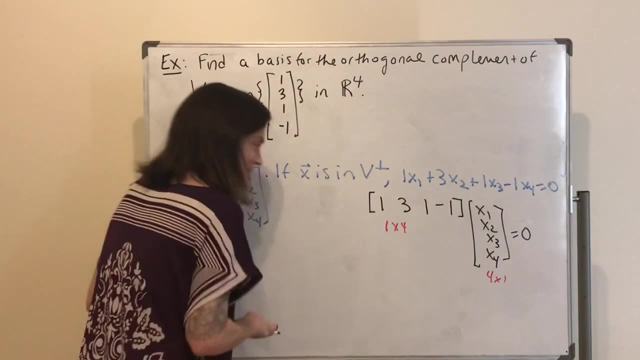 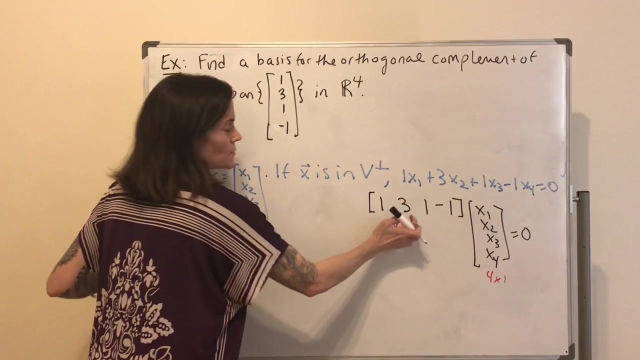 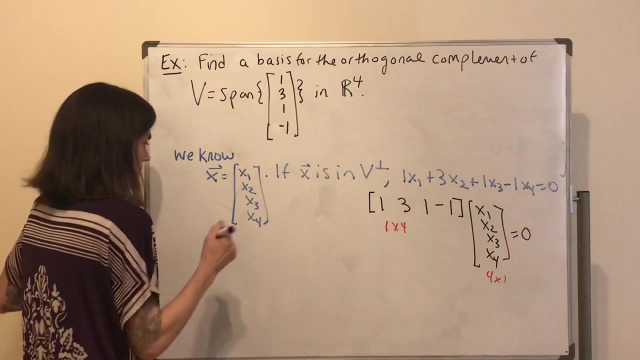 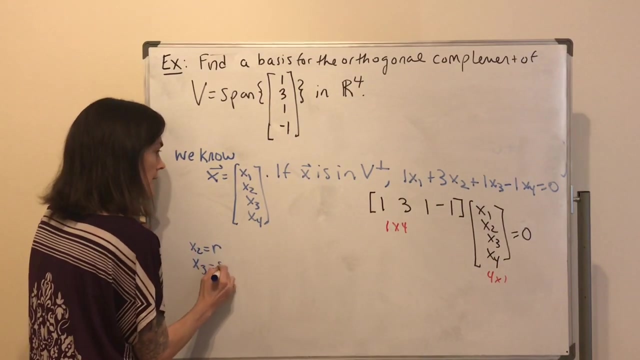 I will move to one where it's not just one vector. Okay, let's, let's now. let's think about this as a matrix and we think about finding its kernel. We have 1,, 2, 3 free variables. So I would just- maybe I'll do this here- Say: x2 is r, x3 is s, x4 is t, And then I: 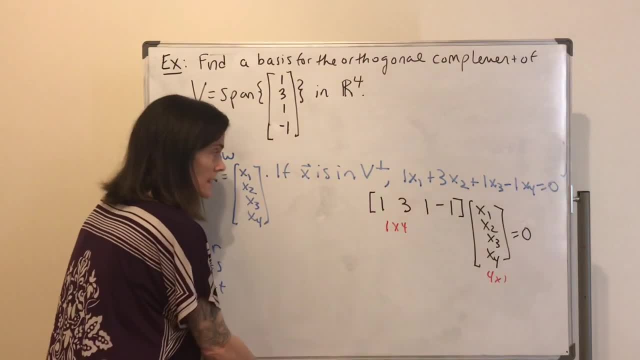 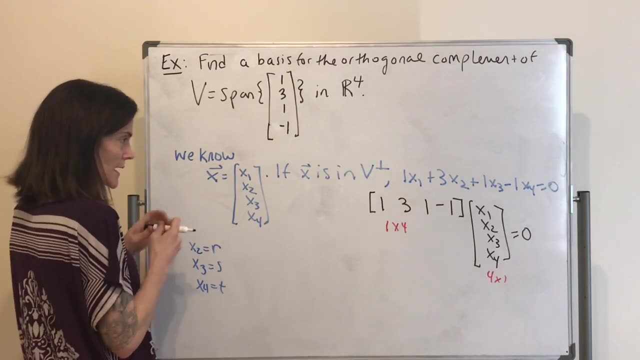 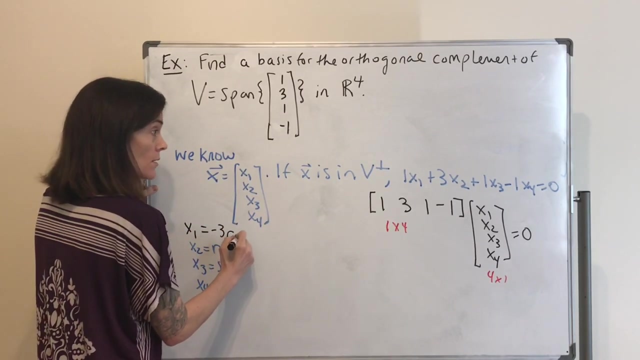 know x1 must be. well, here's the equation. I can even look here. I was just interpreting it. but in terms of a matrix product below, I would know that x1 better be minus 3r, minus s, plus t. 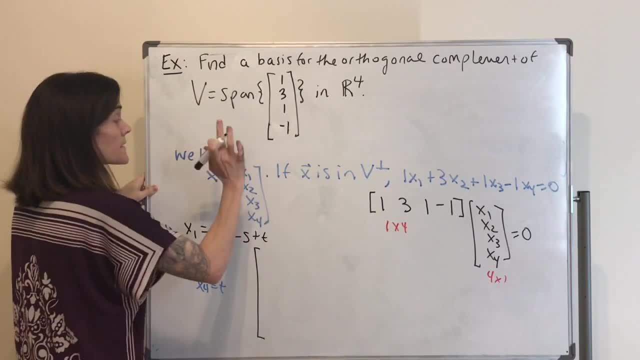 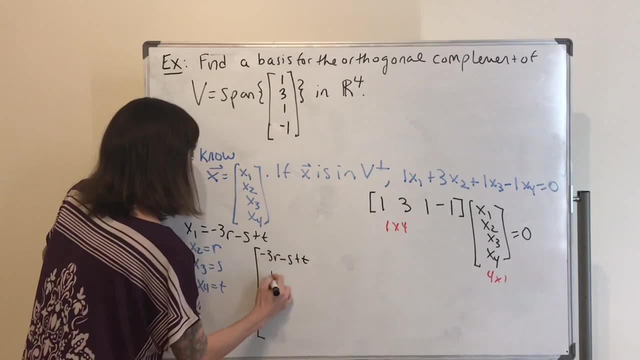 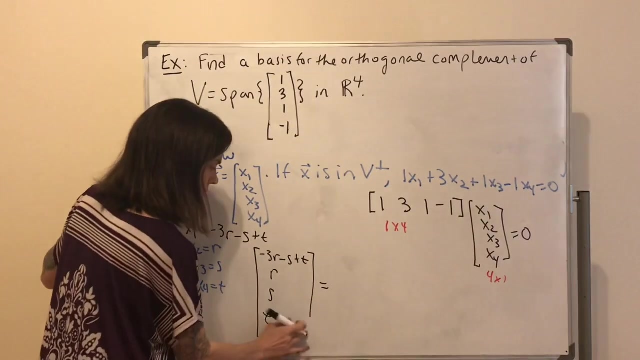 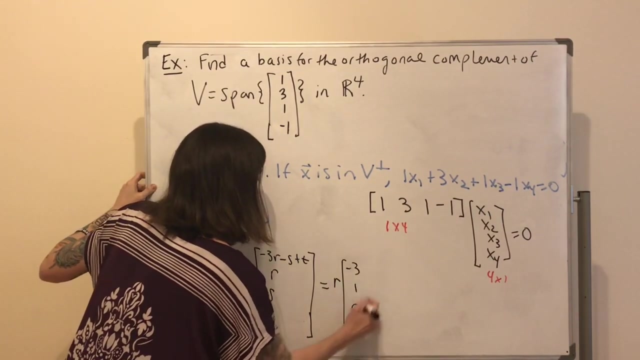 So a general vector in the perp, okay, is minus 3r minus s plus t r s t. And then to find the basis: oh, this doesn't look all that great. I can just break this as r times minus 3,, 1,, 0, 0, plus s times. 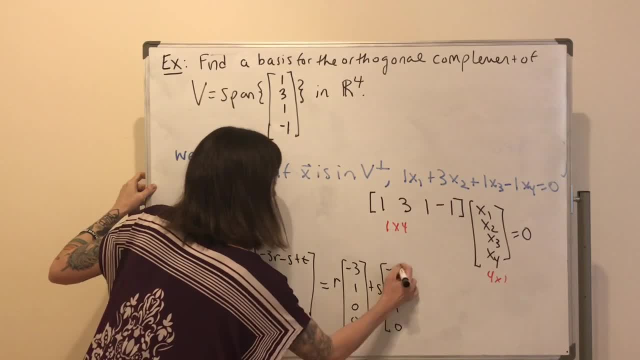 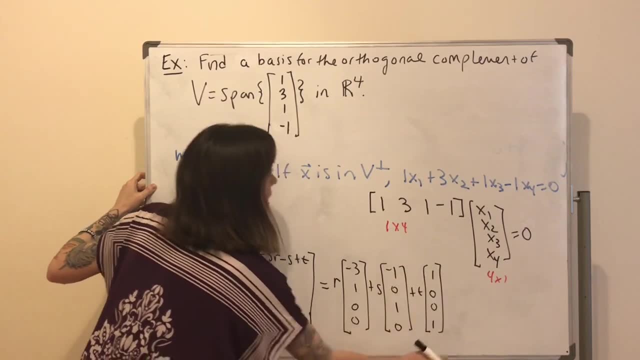 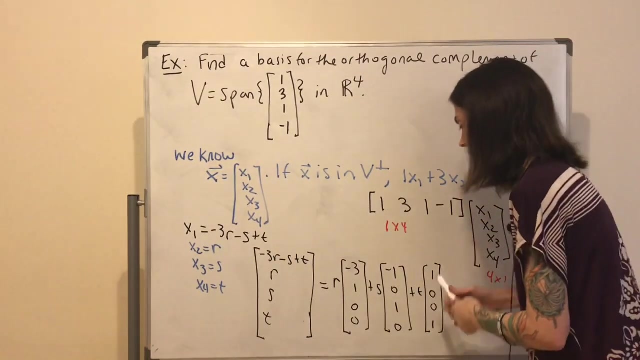 minus 1, 0, 1, 0.. And then plus t times 1, 0, 0, 1.. Okay, So in fact that I do still have room on the board, I can put it right here What we see here. is that my basis? 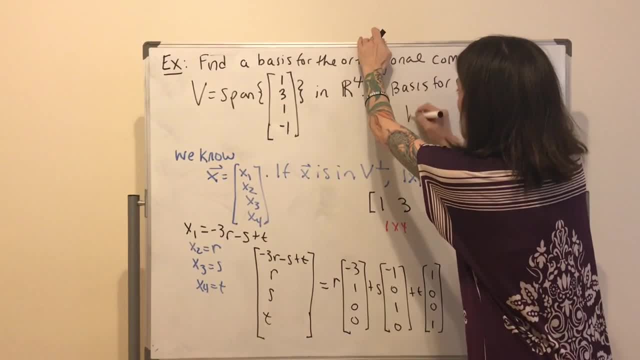 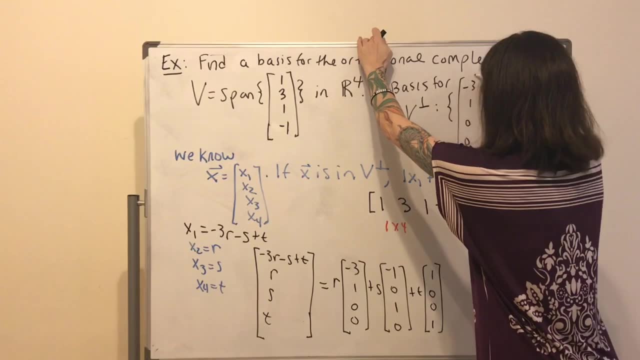 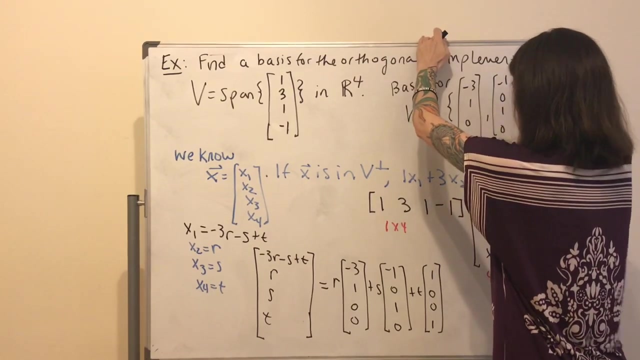 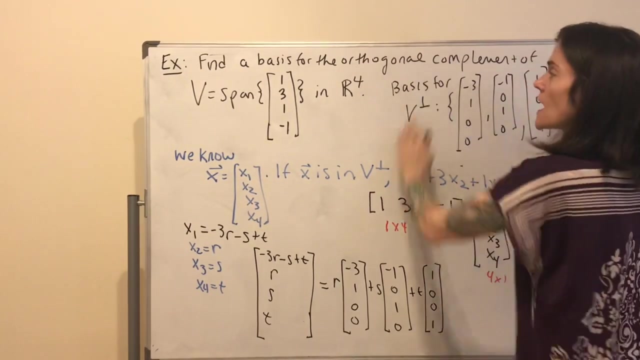 for the perp is minus 3, 1, 0, 0, minus 1, 0, 1, 0, and 1, 0, 0, 1.. And you can check. maybe we should minus 3, plus 3.. Okay, 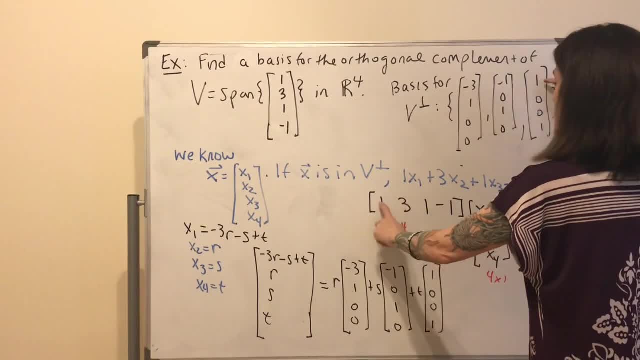 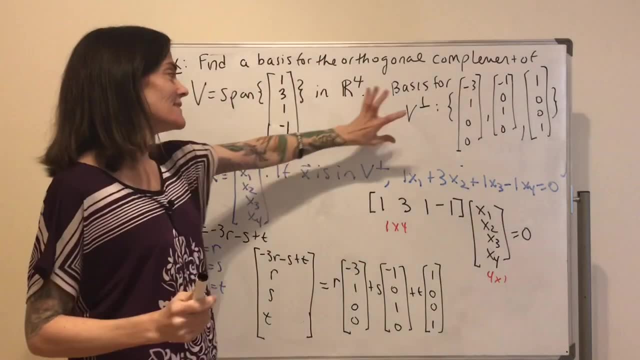 Minus 1, plus 1.. Okay, 1, 0, 0.. Minus 1.. Okay, Those are all definitely in this orthogonal complement, And then we have three of them, And then you can argue: they're literally. 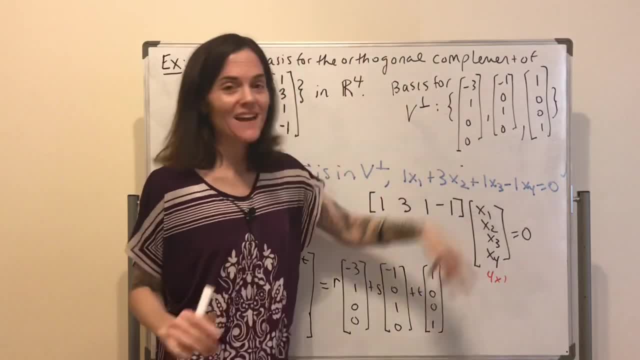 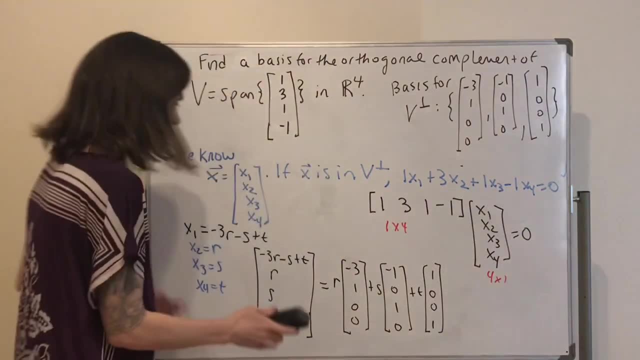 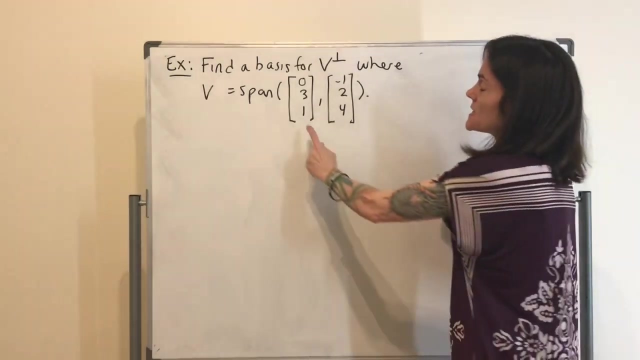 independent, for example, by looking at their pattern of zeros, as we have done before. So in fact, this is a basis for the orthogonal complement. Let's do one more example like this. Well, here's another example, And if we just look at this, these two vectors are literally independent. 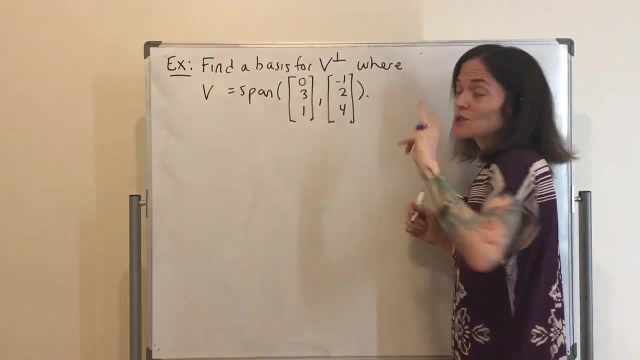 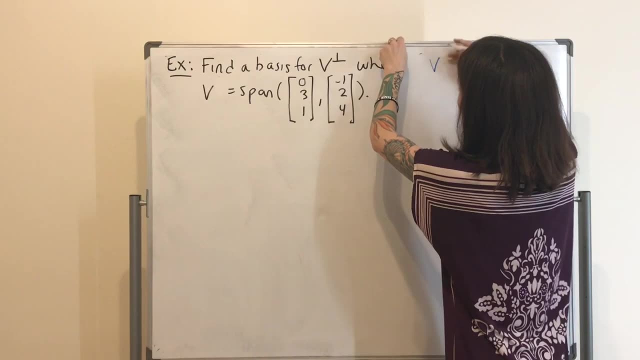 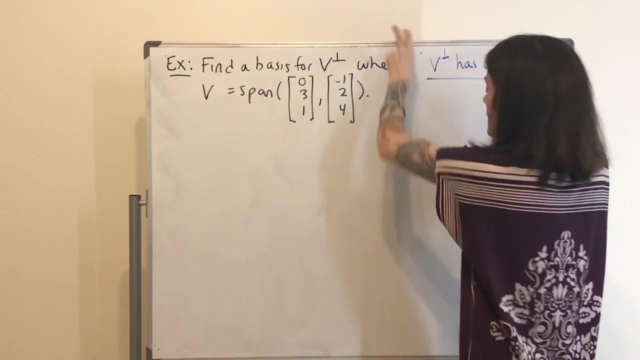 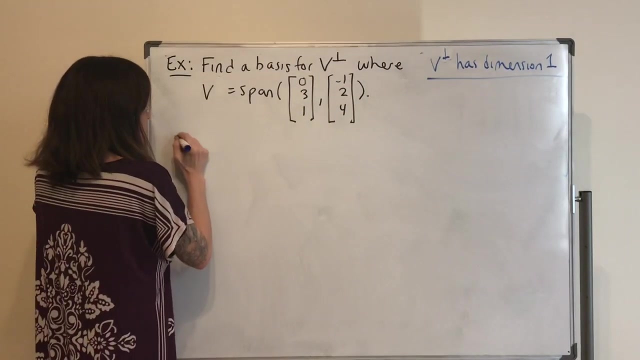 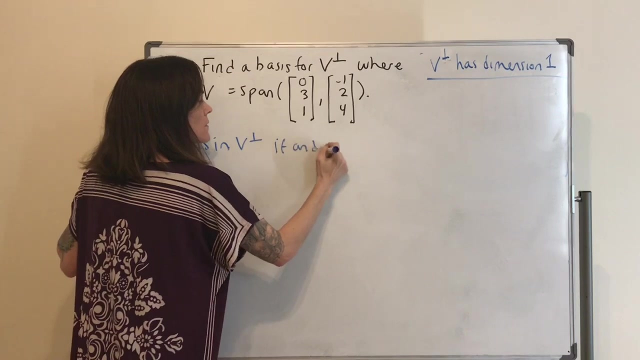 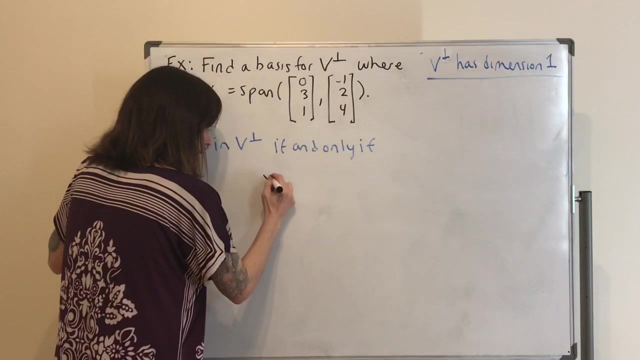 So v is going to have dimension 2, and it's in R3.. We should expect that v perp has dimension 1.. 1. Okay, And the other observation to make is that x is in v perp if, and only if. Okay, Put x here. Well, I want to have the dot. 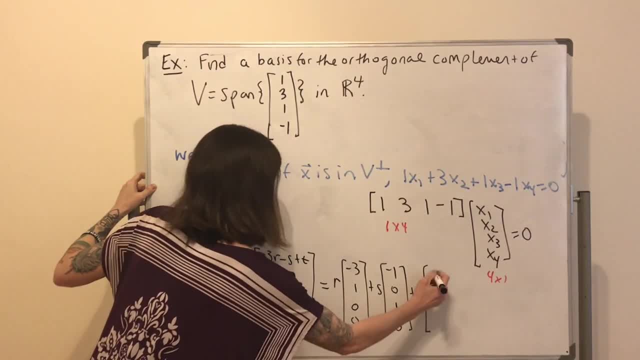 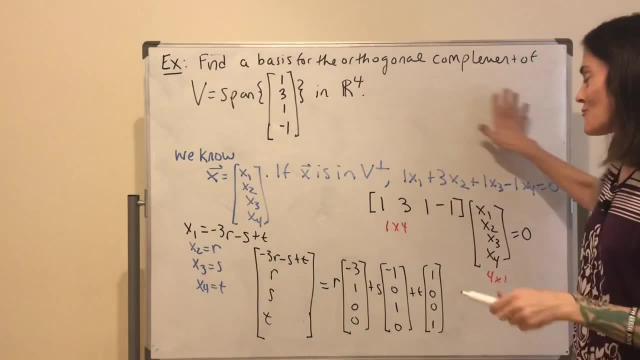 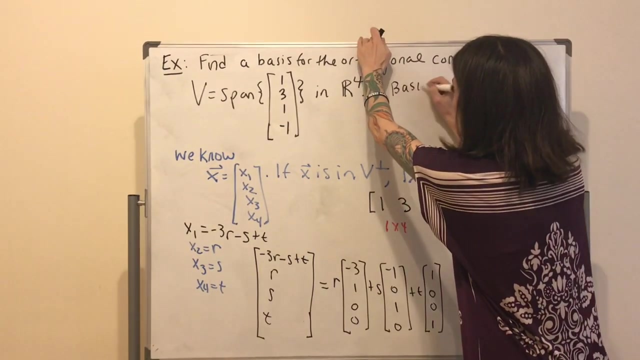 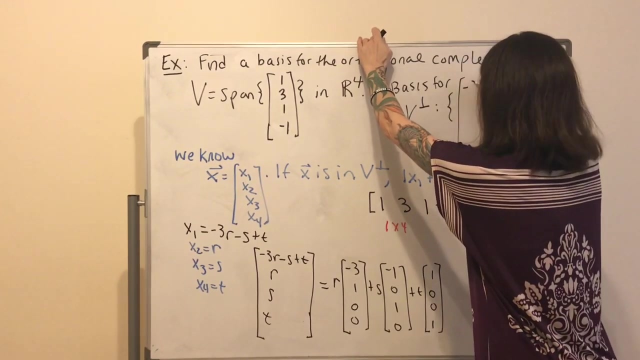 And then plus T times 1.. 0, 0, 1.. Okay, So in fact- and I do still have room on the board- I can put it right here: What we see here is that my basis for the perp is minus 3, 1, 0, 0.. 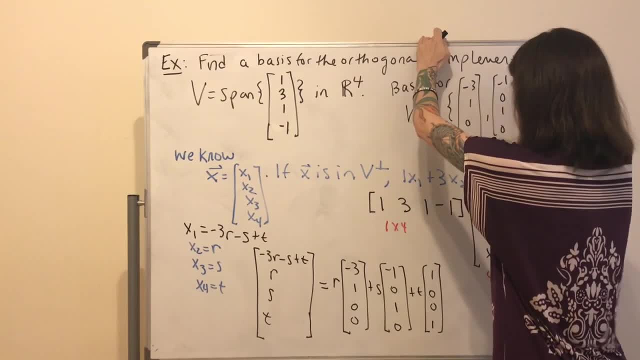 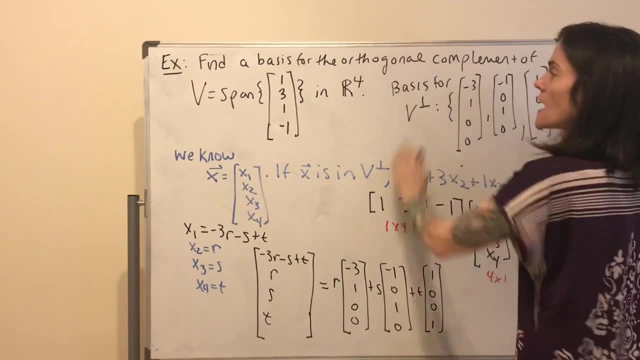 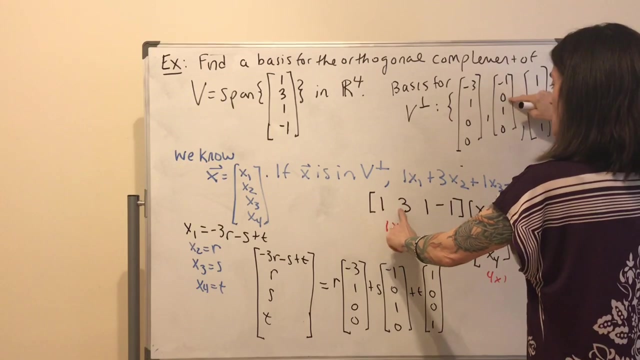 Minus 1, 0, 1, 0.. And 1, 0, 0, 1.. And you can check, Maybe we should: Minus 3 plus 3.. Okay, Minus 1 plus 1.. 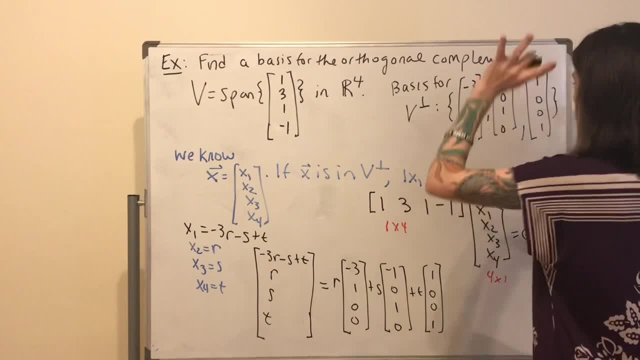 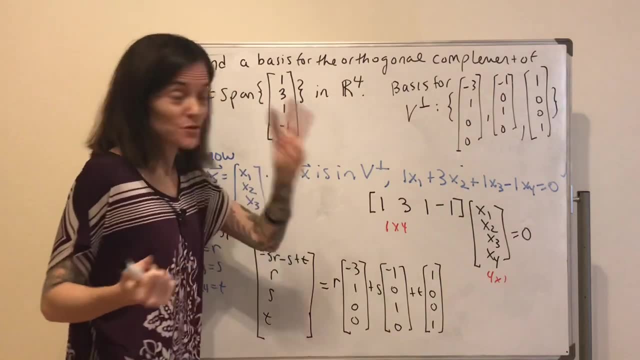 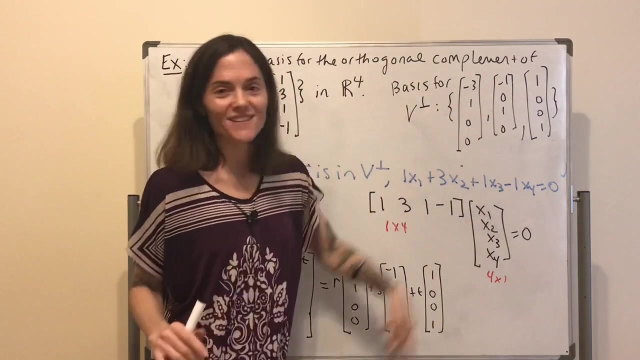 Okay, 1, 0, 0. Minus 1.. Okay, Those are all definitely in this orthogonal complement. And then we have three of them, And then you can argue they're literally independent, For example by looking at their pattern of zeros, as we have done before. 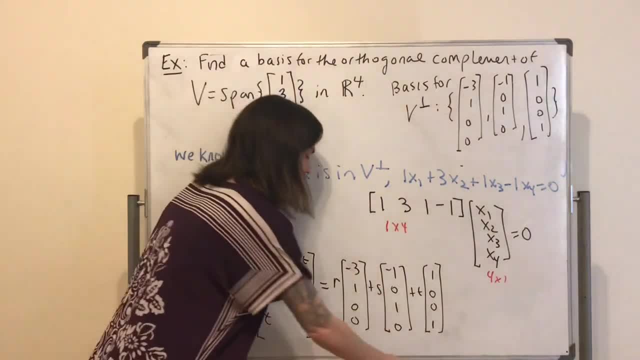 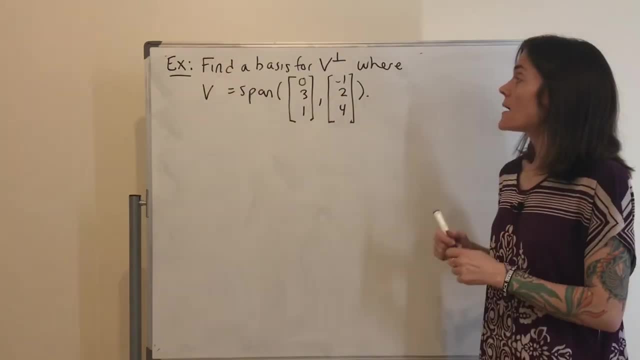 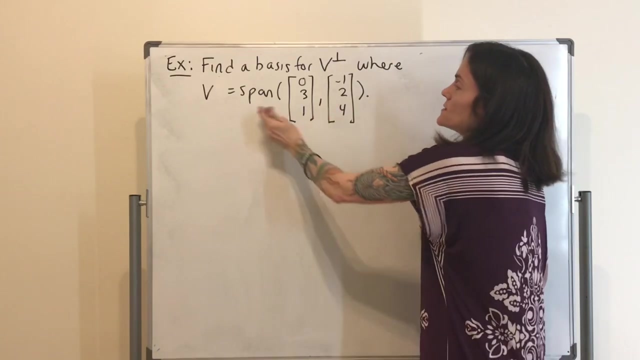 So in fact, this is a basis for the orthogonal complement. Let's do one more example like this. Well, here's another example, And if we just look at this, these two vectors are literally independent. So V is going to have dimension 2.. 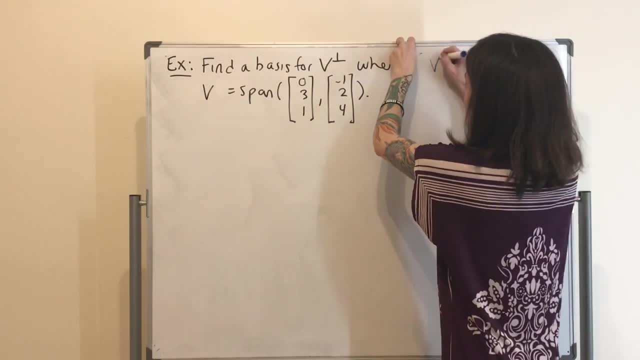 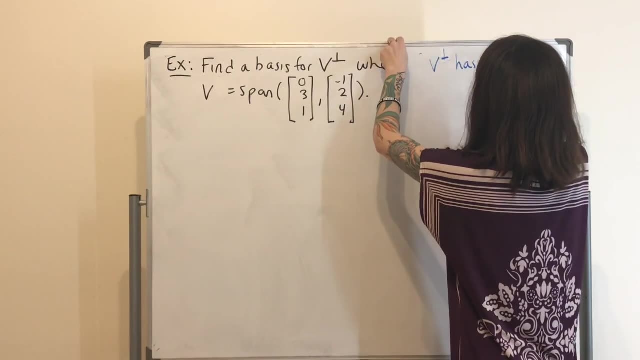 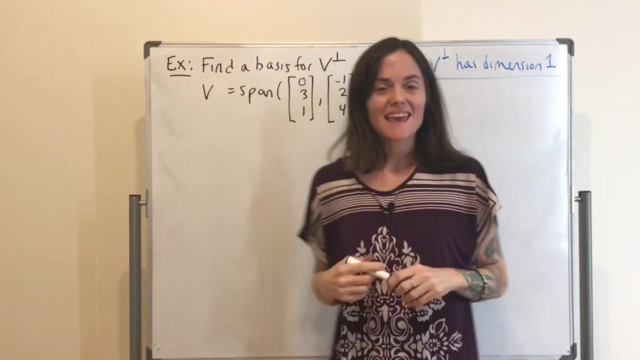 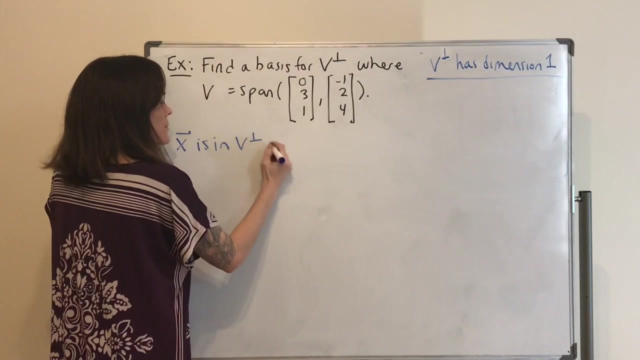 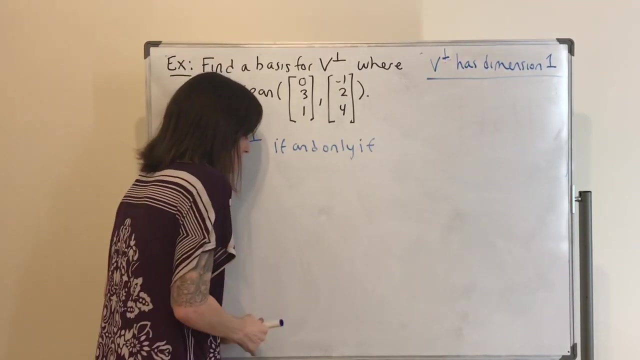 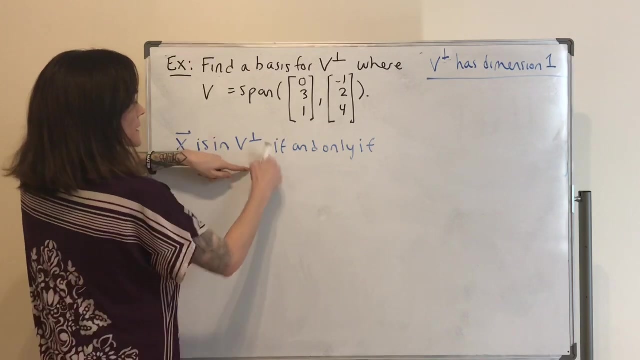 And it's in R3.. We should expect that V perp Has dimension 1.. Okay, And the other observation to make is that X is in V perp If, and only if. Okay, Put X here. Well, I want to have the dot product like this: 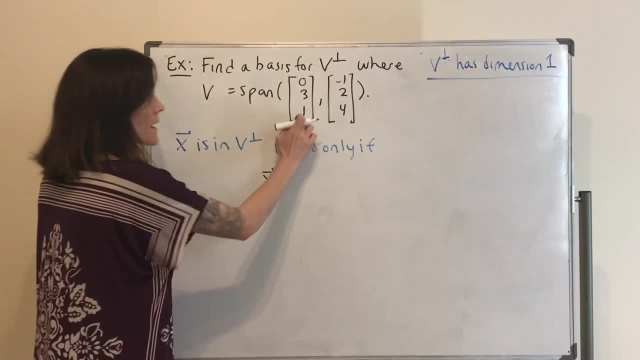 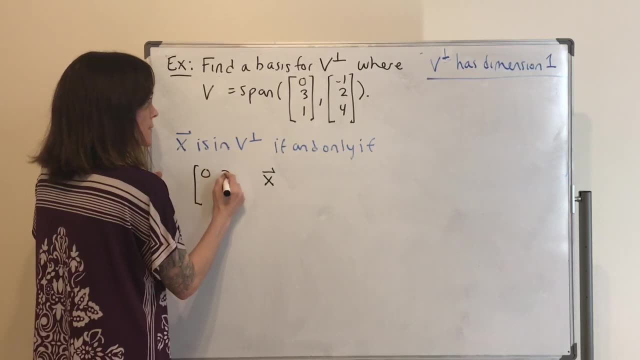 Like this, Just like in the last example. right, I know that X dot this is 0 and X dot this is 0. But I can translate that if I 0,, 3,, 1. And then minus 1,, 2, 4.. 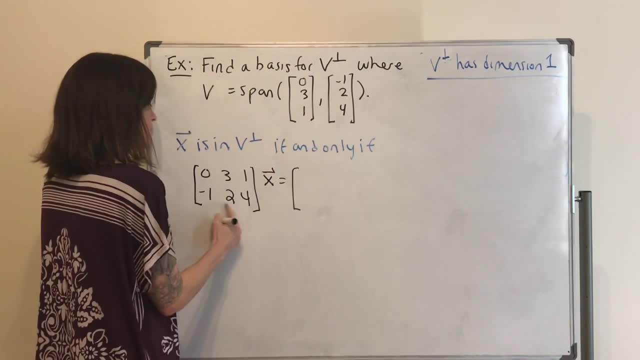 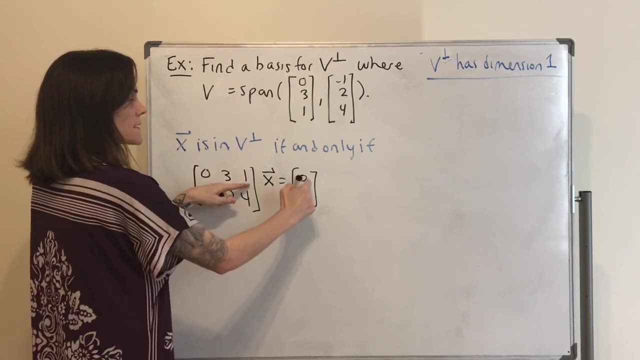 Right, Because this is 2 by 3, 3 by 1. This would be 2 by 1.. But here, dot product with this gives you this entry 0.. Dot product with this: this entry 0.. 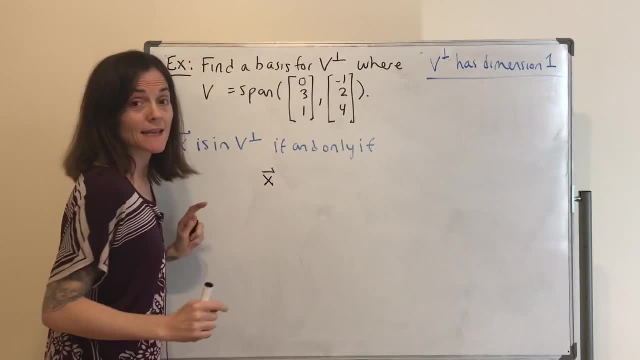 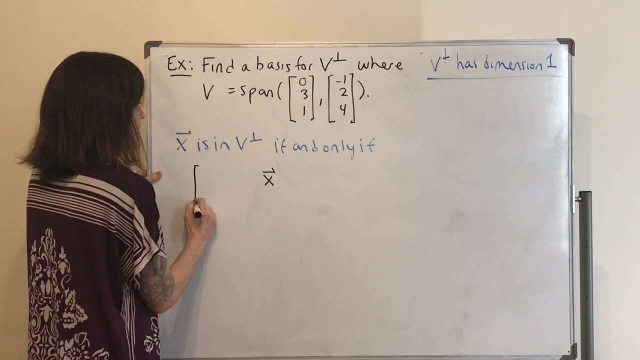 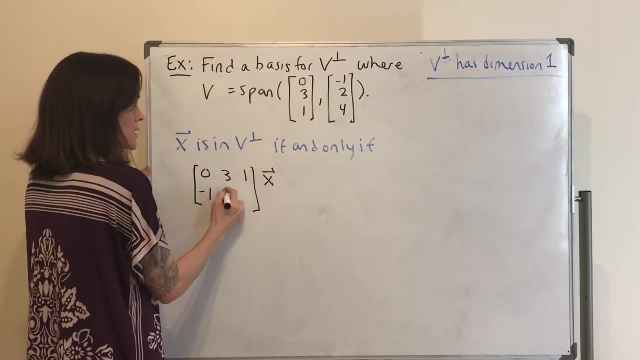 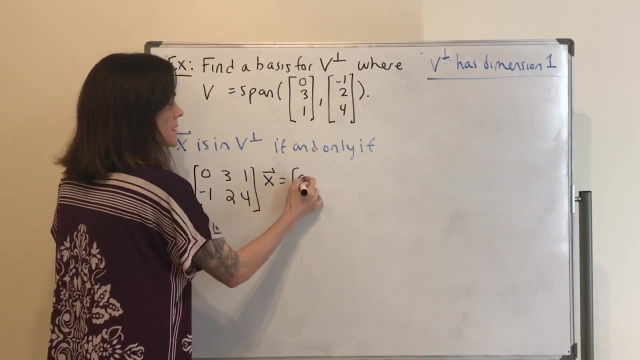 product with like this, like this, Just like in the last example, right, I know that x dot this is zero and x dot this is zero, but I can translate this into the dot product. So I can translate that if I 0,, 3,, 1, and then minus 1,, 2,, 4,, right, Because this is 2 by 3,, 3 by 1,. 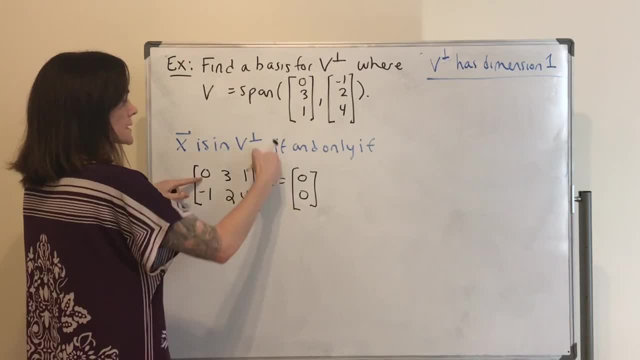 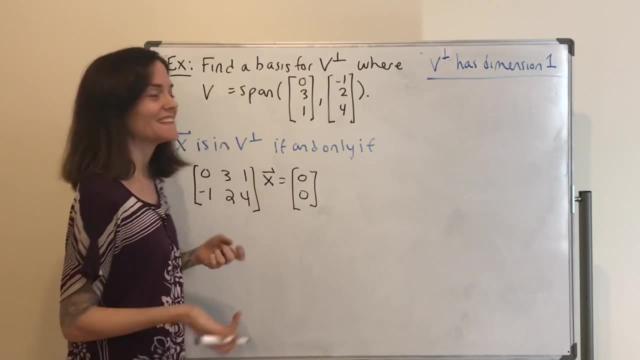 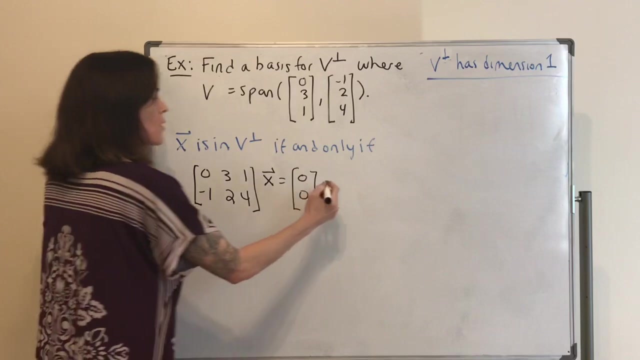 this would be 2 by 1.. But here, dot product with this gives you this entry 0.. Dot product with this, this entry 0, right, This is what I need. if, and only if, This matrix times this vector x equals 0, or equivalently. 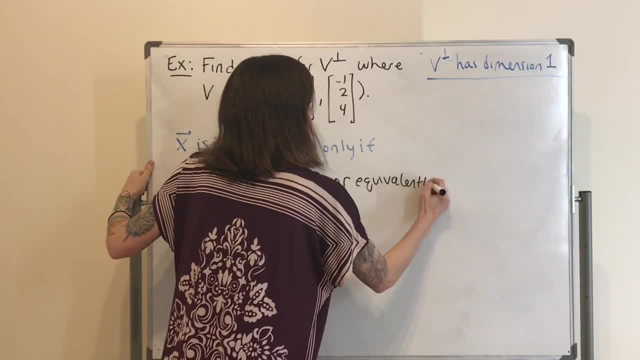 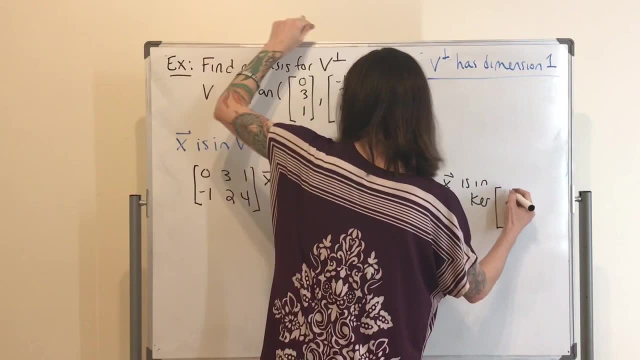 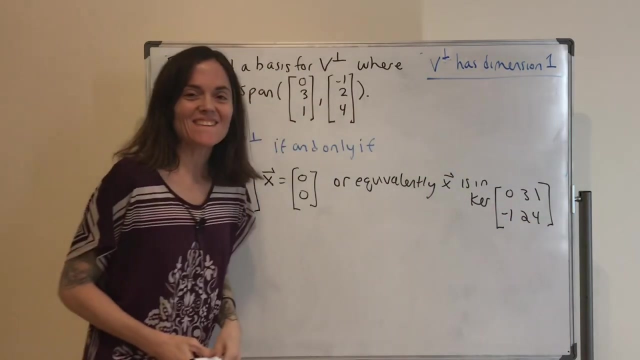 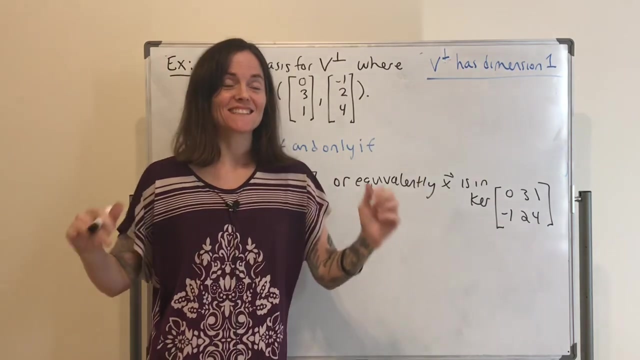 x is in the kernel of this matrix: 0, 1, 3, minus 1, 2, 4.. Okay, This is why I was thinking about the last example, even though my matrix was 1. which is really just a vector. but I wanted to think about it like that because when you have 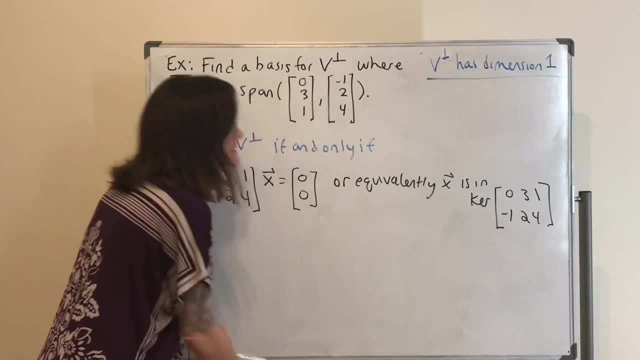 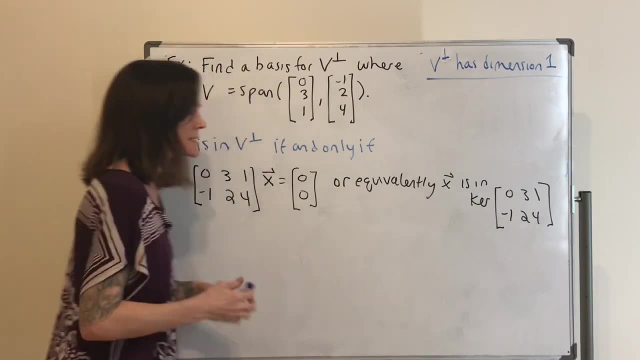 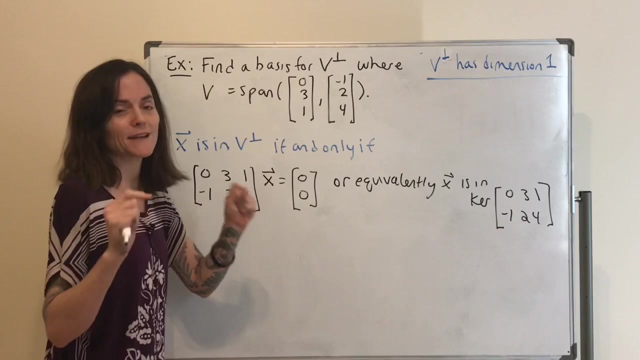 more than one vectors. it's very similar. Now the nice thing is we know how to find bases or a basis for a kernel of a matrix. Okay, I need to perform elementary row operations to get this into reduced row echelon form. Then I can figure out a basis for the kernel. So the first thing I'm 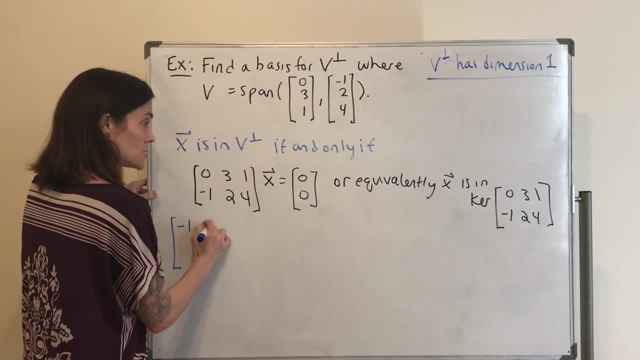 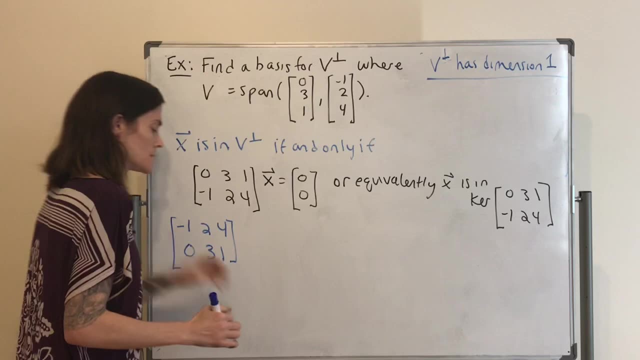 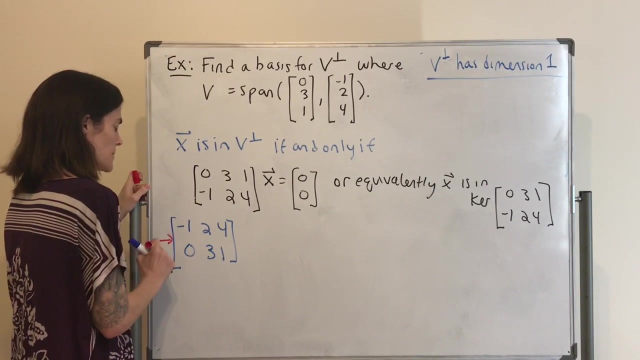 going to do is: I'm just going to interchange my row so that I have a non-zero entry in the 1, 1 position. So technically, I have already done something here. It went from here to here. Oh, okay, maybe I'll write it. Well, no, I'll just do this. I've done something. Okay, I interchange row. 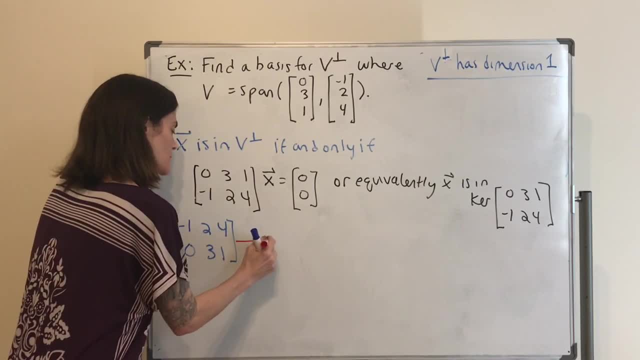 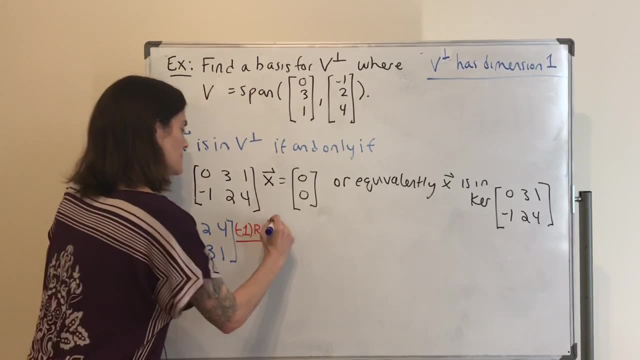 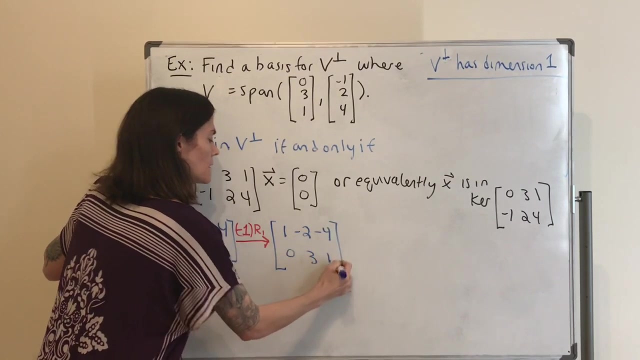 2 and row 1.. Now I'll do my first step, that I write what it is. I multiply row 1 by minus 1.. This becomes 1 minus 2 minus 4.. This has not changed. Now I need to multiply row 2.. I could. 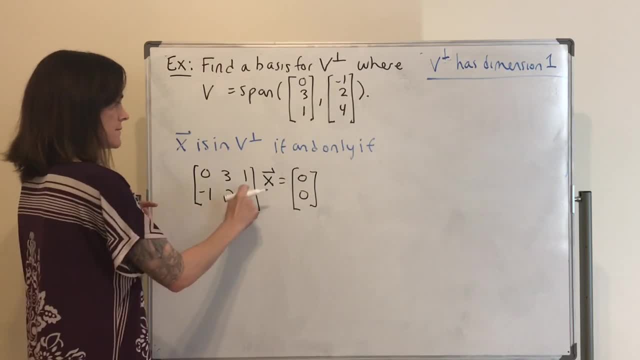 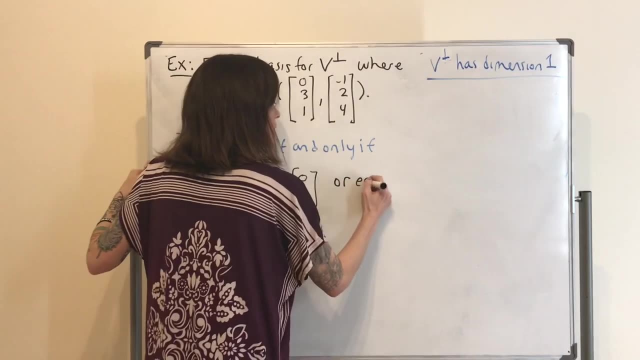 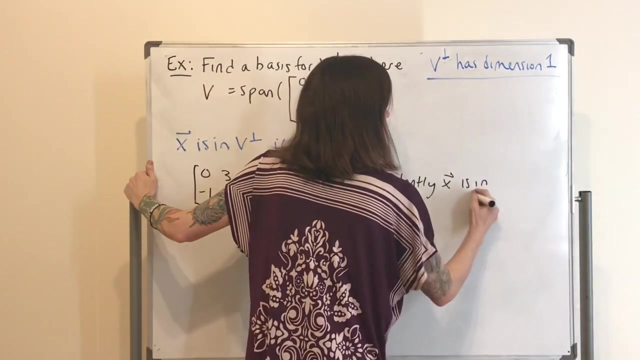 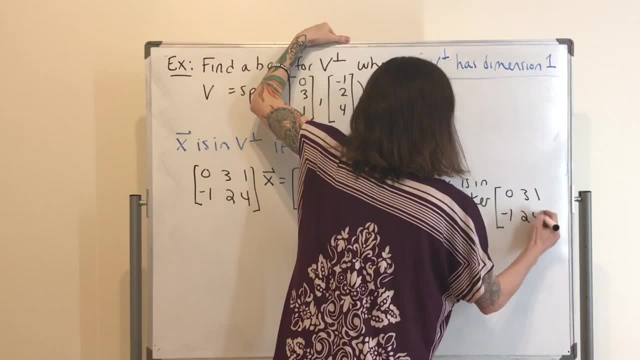 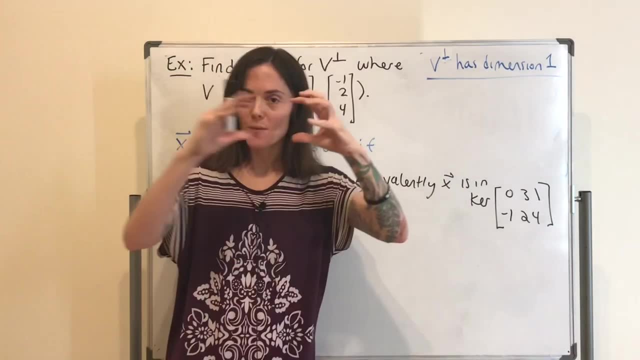 0.. 0.. 1.. 3. Minus 1,, 2, 4.. Okay, This is why I was thinking about the last example, even though my matrix was 1 by 4, which is really just a vector. 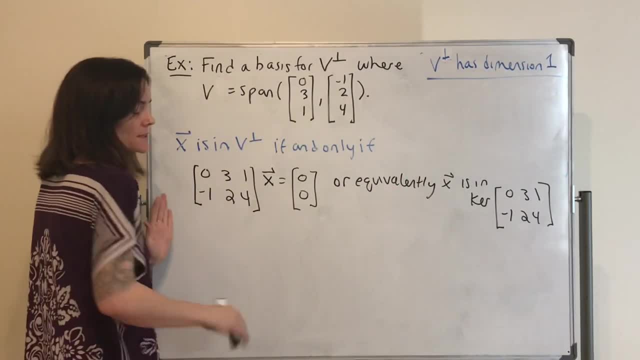 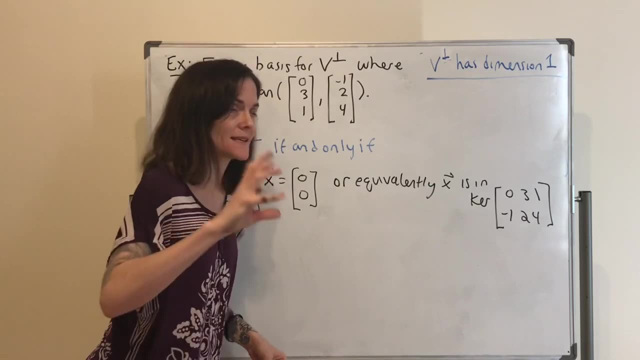 But I wanted to think about it like that, because when you have more than one vectors, it's very similar. Now the nice thing is, we know how to find bases, or a basis for a kernel of a matrix. Okay, I need to perform. 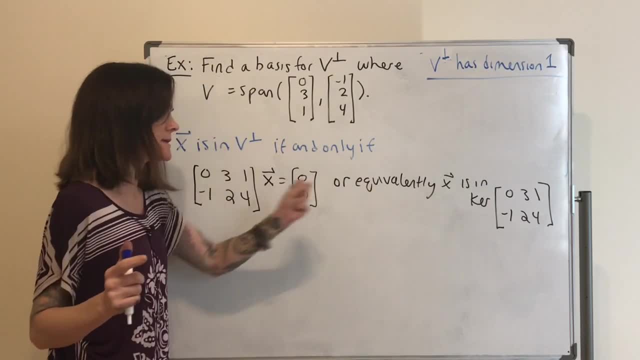 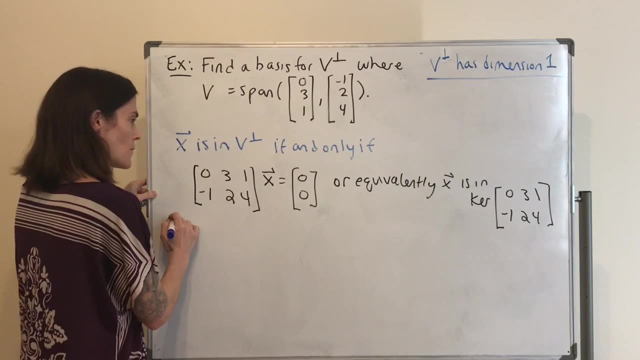 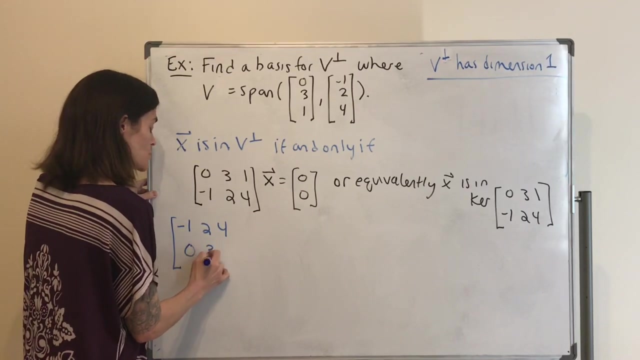 I need to perform elementary row operations to get this into reduced row echelon form. Then I can figure out a basis for the kernel. So the first thing I'm going to do is I'm just going to interchange my row so that I have a non-zero entry in the 1, 1 position. 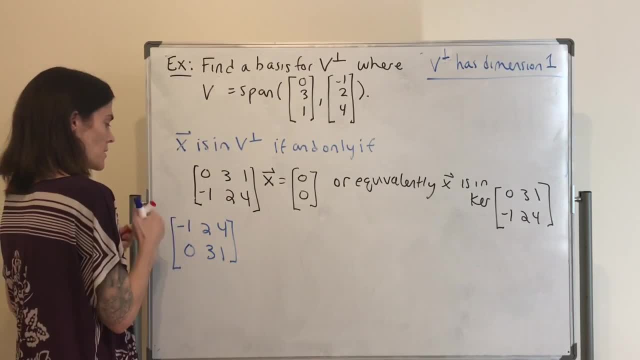 So technically, I have already done something here. It went from here to here. Oh okay, Maybe I'll write it. Oh no, I'll just do this. I've done something. Okay. I interchange row 2 and row 3.. 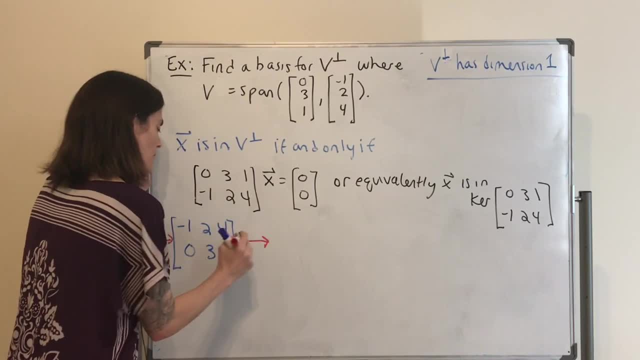 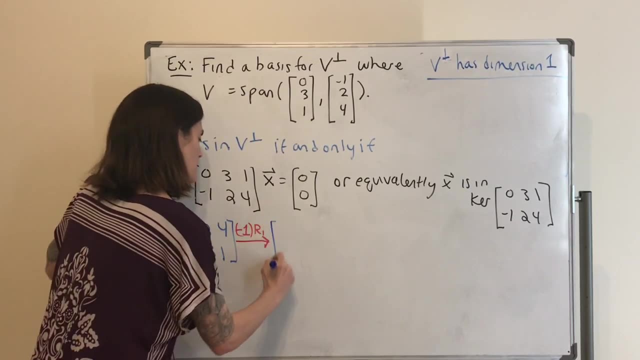 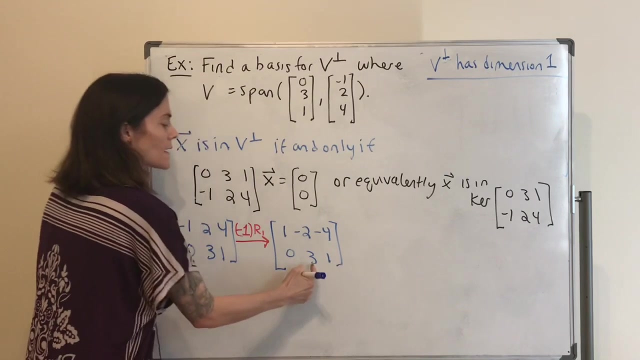 Row 1.. Now I'll do my first step, that I write What it is. I multiply row 1 by minus 1.. This becomes 1 minus 2 minus 4.. This has not changed. Now I need to multiply row 2.. 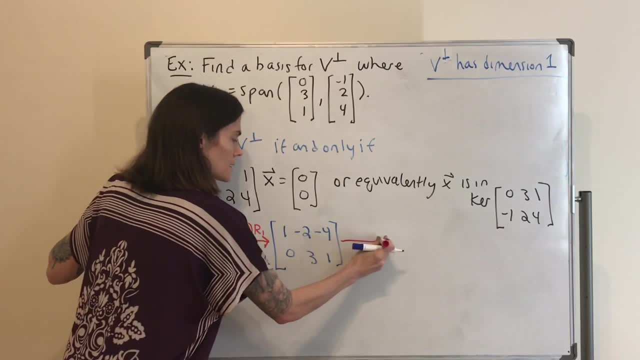 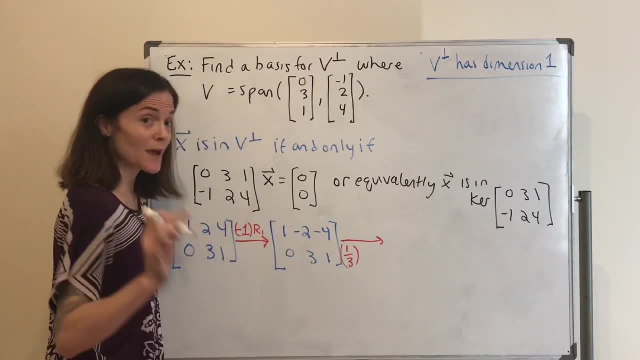 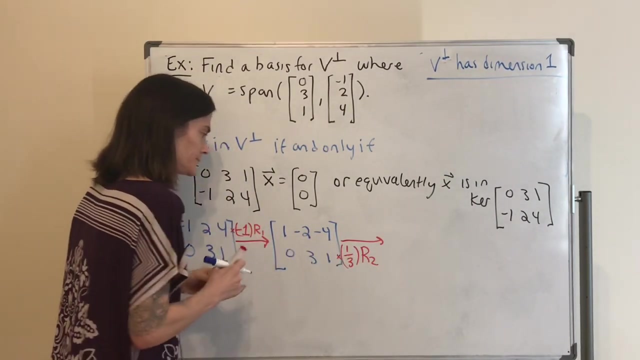 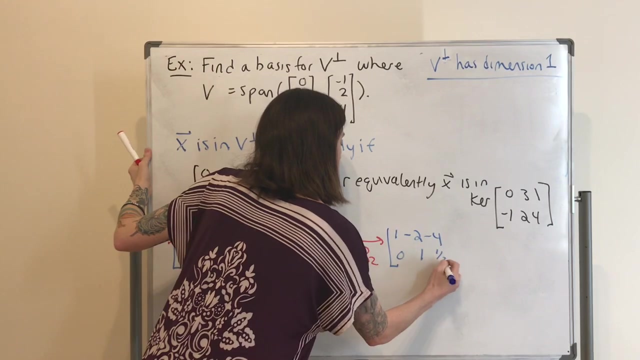 I could have technically done it in the same step. Okay, It's fine, I'll do it in two steps. Multiply row 2 by a third, And this will turn this into 8.. And I'll multiply row 2 by a 1, 1 third. row 2, times and times, okay, and then I have 1, minus 2, minus 4, 0, 1, 1 third. 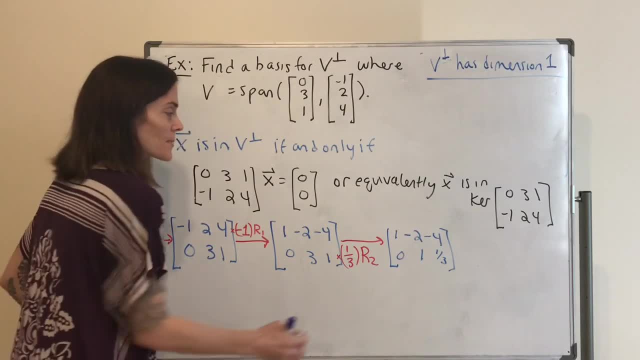 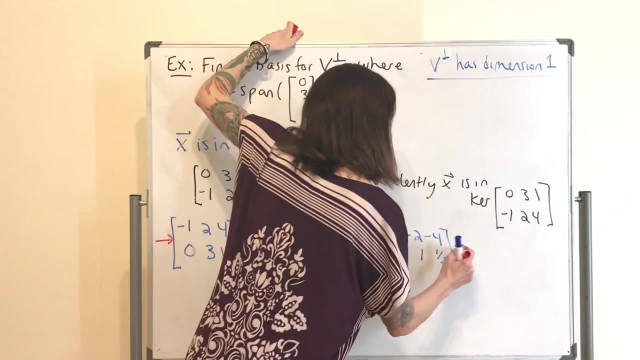 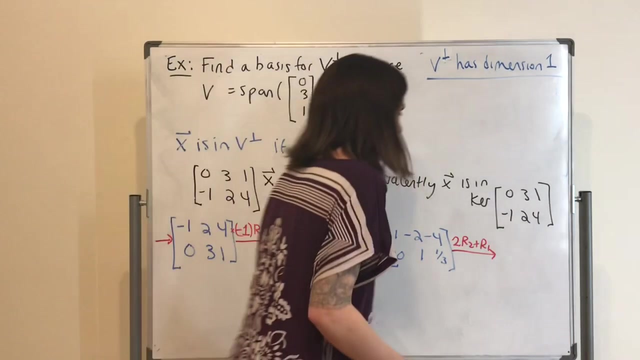 Well, I'm almost to reduce row echelon form. I just need to make this minus 2, that's above this 1 a 0. So I can take 2 times row 2.. Add it to row 1. And then I will be reduced. 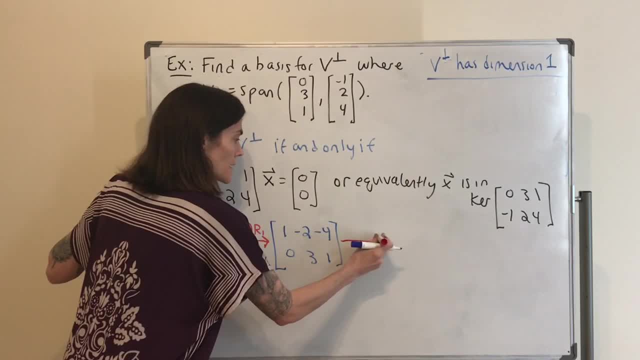 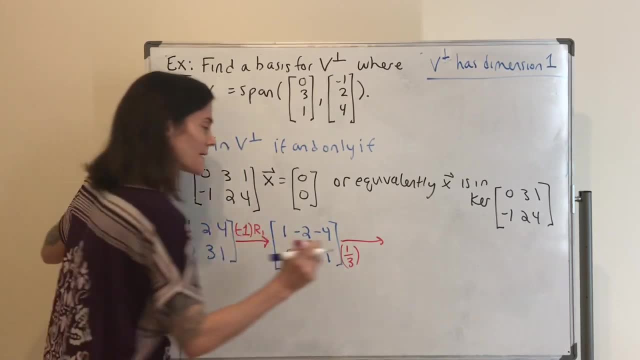 have technically done it in the same step. Okay, it's fine, I'll do it in two steps. Multiply row 2 by a third and this will turn this into a 1. One-third row, 2 times and times. Okay. 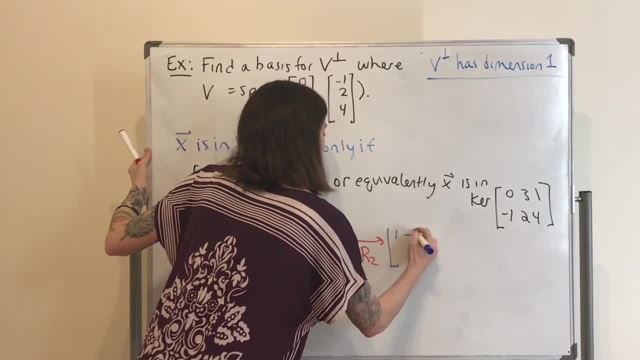 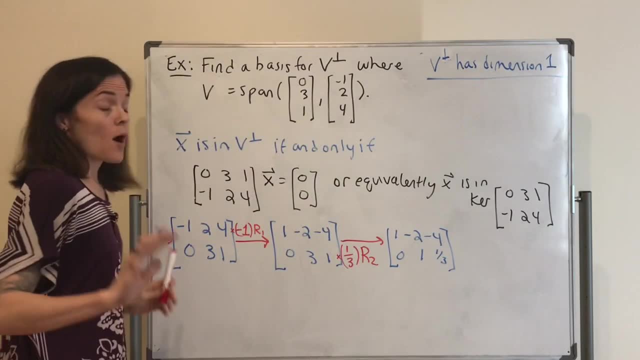 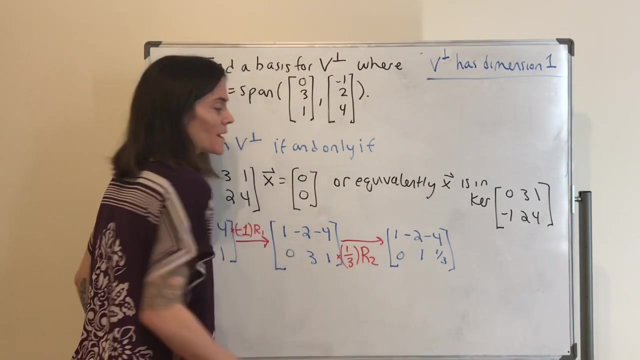 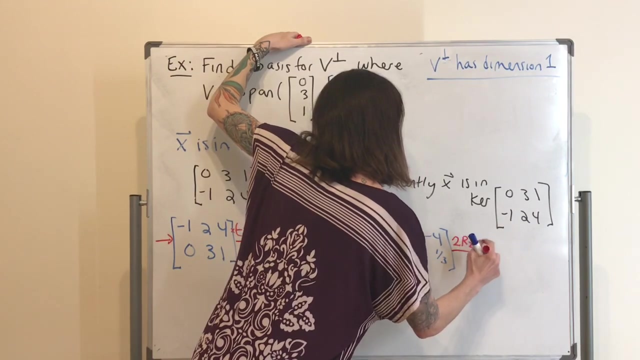 and then I have 1. Minus 2 minus 4. 0, 1. One-third. Well, I'm almost to reduced row echelon form. I just need to make this minus 2, that's above this 1 a 0. So I can take 2 times row 2, add it to row 1, and then I 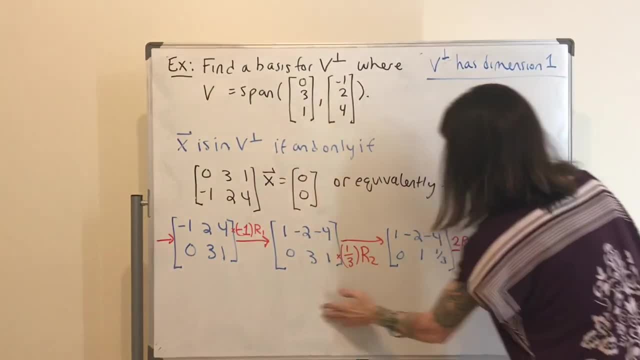 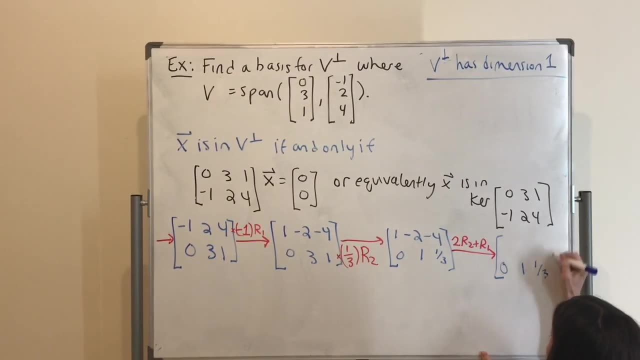 will be reduced. Oh goodness, Row echelon form. So row 1, oh, row 2 has not changed. Row 1, 1, 0, and now comes fractions. Well, it's going to be 2-thirds minus 4.. This is 12-thirds minus 10 over 3.. Okay, so this is this entry here. 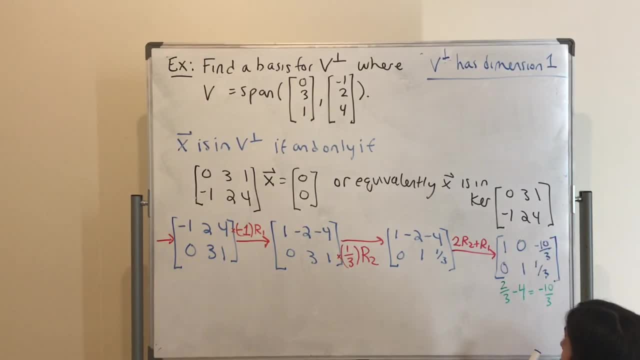 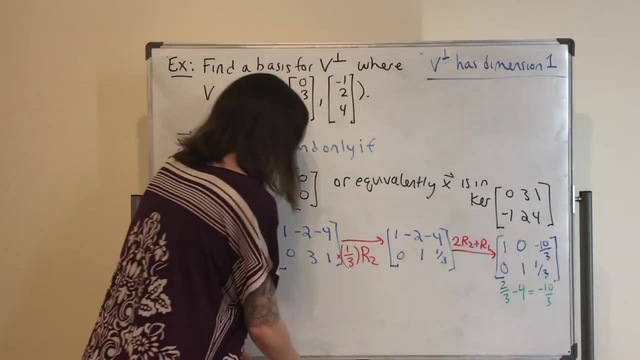 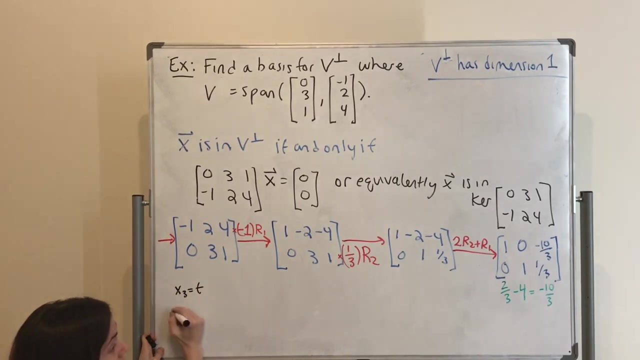 Minus 10 over 3.. You see I have my third column corresponds to a free variable. So if I set, let's say I set x3 to be t, and then I get x1 is 10-thirds t and I get x2 is minus a third t, So an element in the 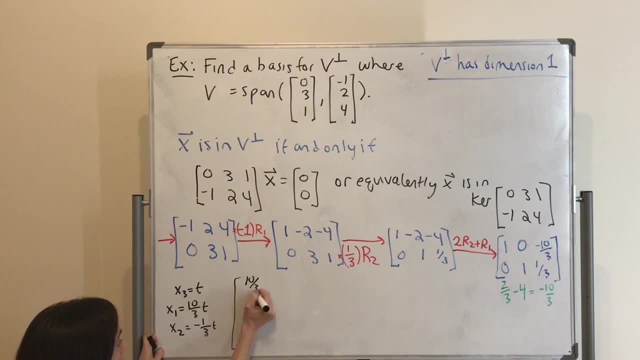 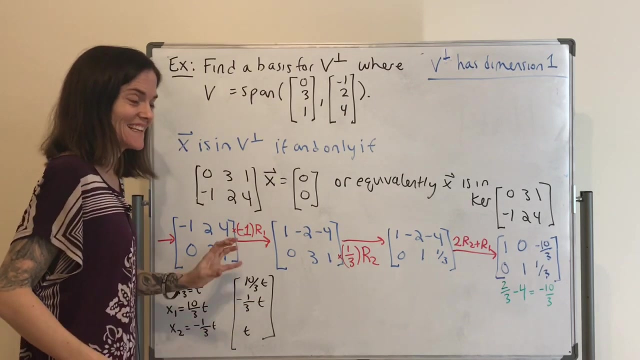 kernel of this matrix is 10-thirds t minus a third t and t. Okay, now I can use this to get a basis. I just need one of these. It's not zero, because this is one-dimensional And you see, I had only one free variable. 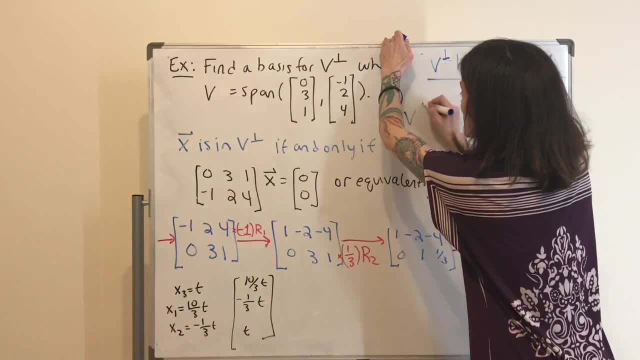 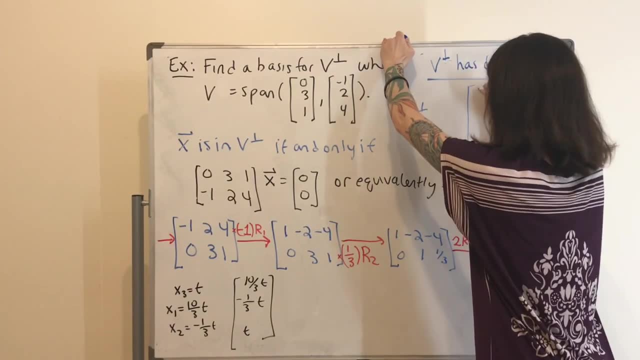 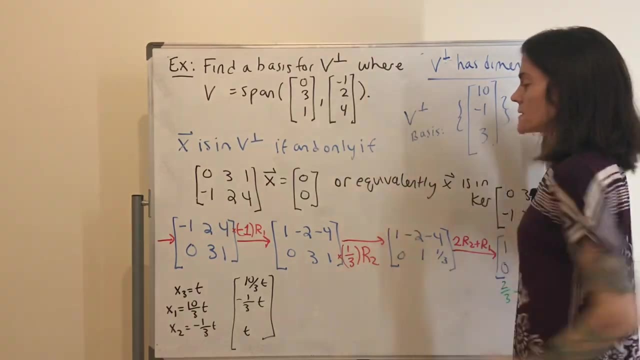 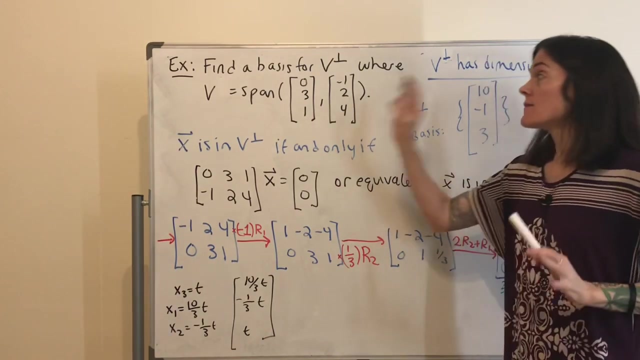 I'll write it up here. I could also just use 10. Minus 1 and 3. Sort of avoids having a fraction And this will be a basis for the orthogonal complement of this v And in fact you can check. 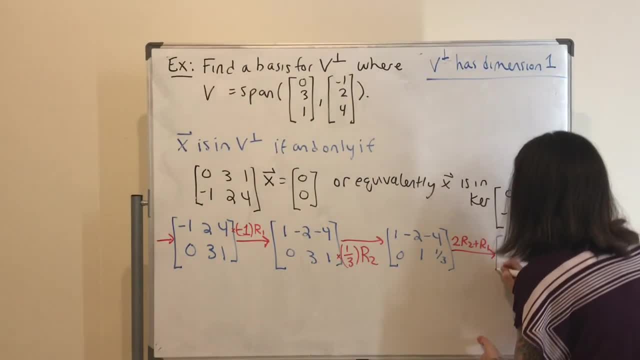 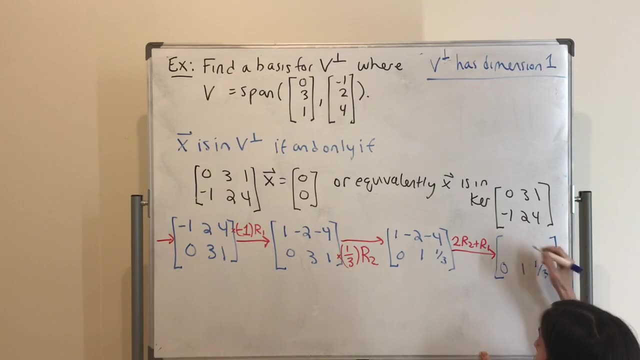 Oh goodness, Row echelon form, So row 1.. Oh, row 2 has not changed. Row 1, 1, 0.. And now comes fractions. Well, it's going to be 2 thirds minus 4.. 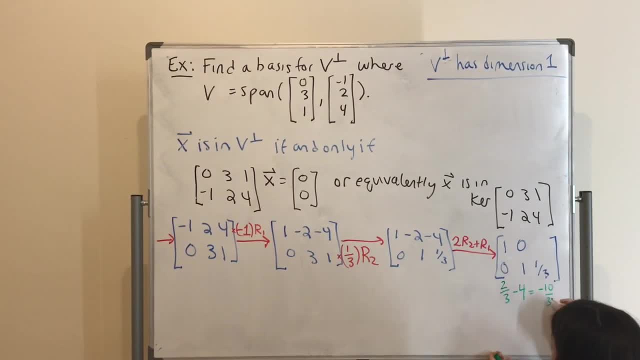 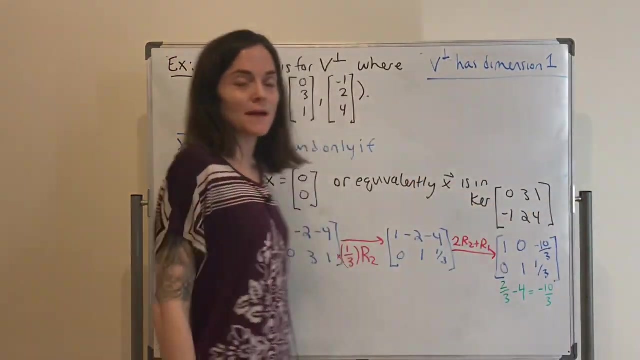 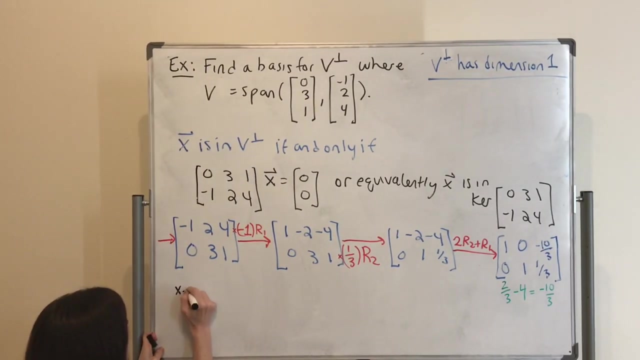 This is 12 thirds, 2 thirds minus 10 over 3.. Okay, So this is this entry here, minus 10 over 3.. You see I have my third column corresponds to a free variable. So if I set, let's say I set- X3 to be T and then I get, X1 is 10 thirds. 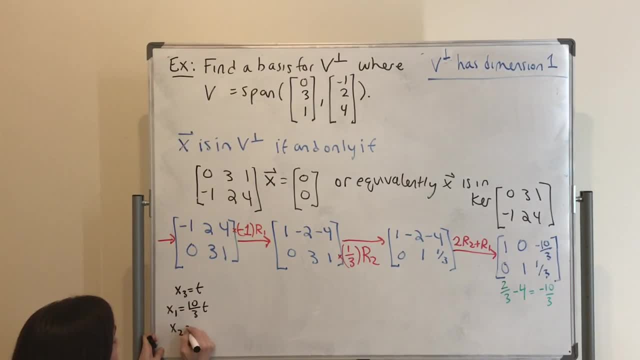 T and I get X2 is minus a third T, So an element in the kernel of this matrix is 10 thirds T minus a third T and T. Okay, Now I can use this to get a basis. I just need one of these. 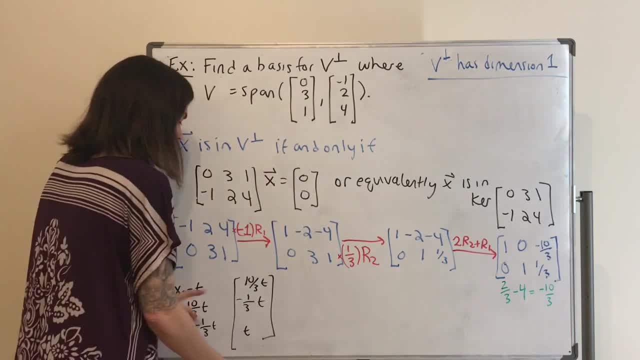 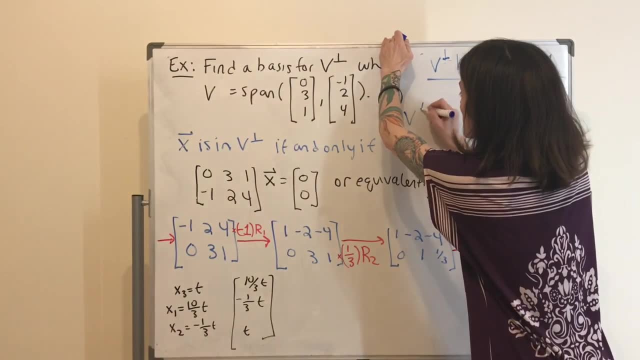 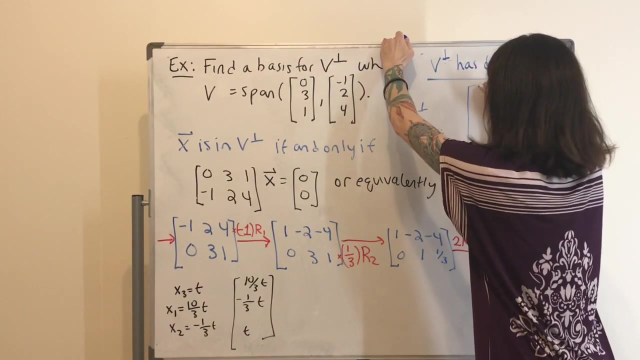 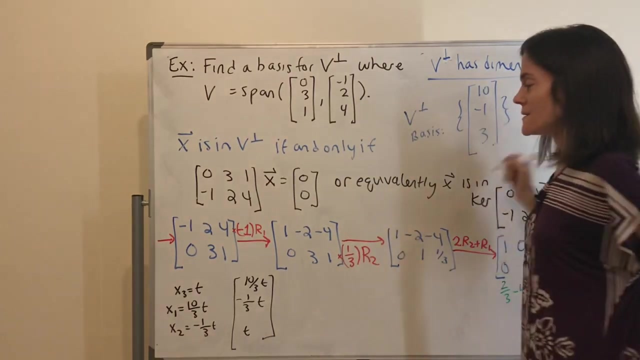 It's not zero because this is one dimensional And you see I had only one free variable. I'll write it up here. I could also just use 10, minus 1, and 3. Sort of avoids having a fraction. 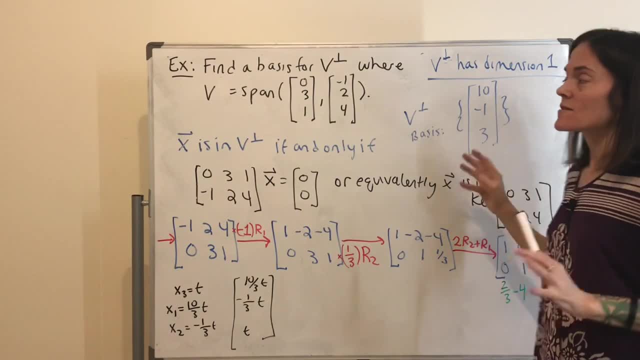 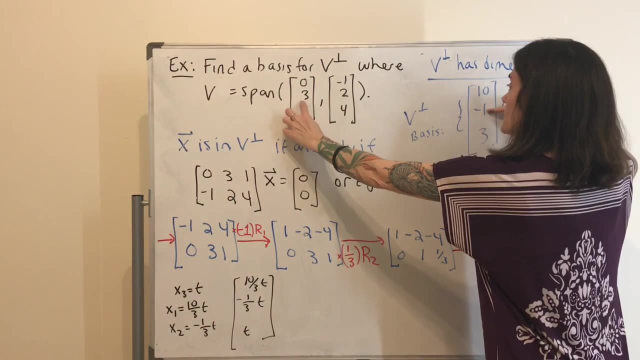 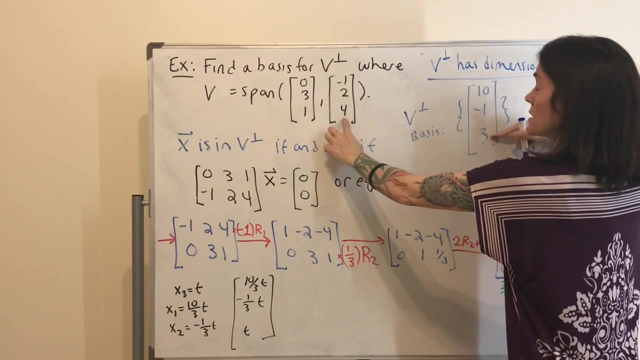 And this will be a basis for the orthogonal complement of this V. And in fact you can check dot product here: Zero Minus 3, plus 3, zero, And then this is going to be minus 10, minus 2 is negative. 12, plus 12, zero. 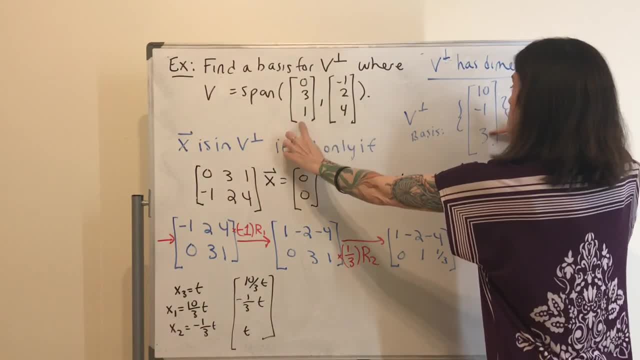 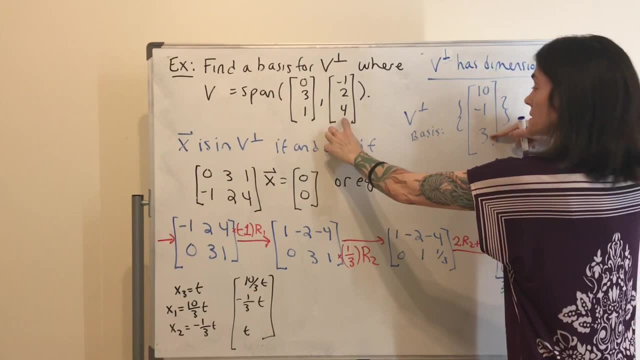 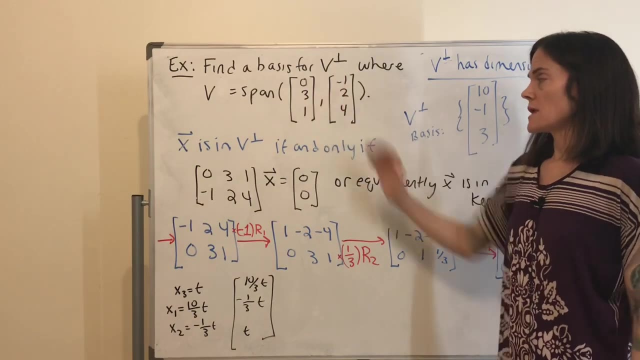 Dot product here: 0, minus 3, plus 3, 0. And then this is going to be minus 10, minus 2 is negative, 12, plus 12, 0. So this is 1.. Non-zero vector, linearly independent, is perpendicular to both these. 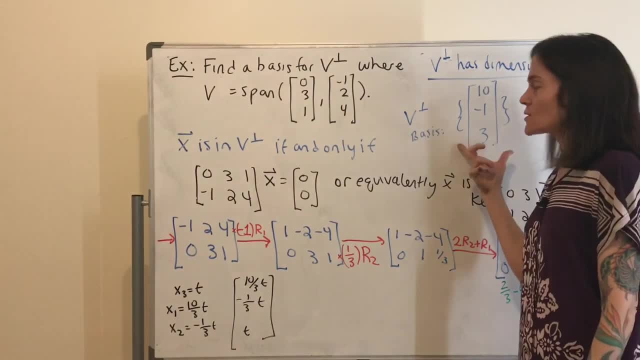 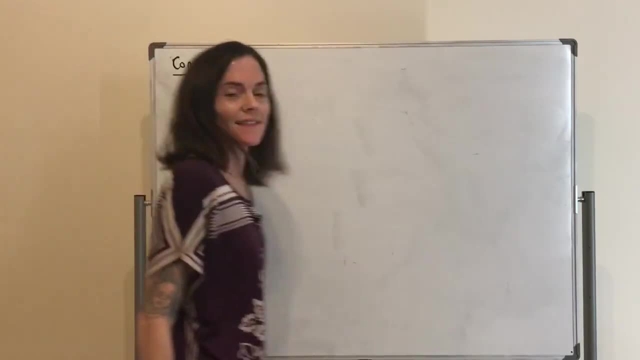 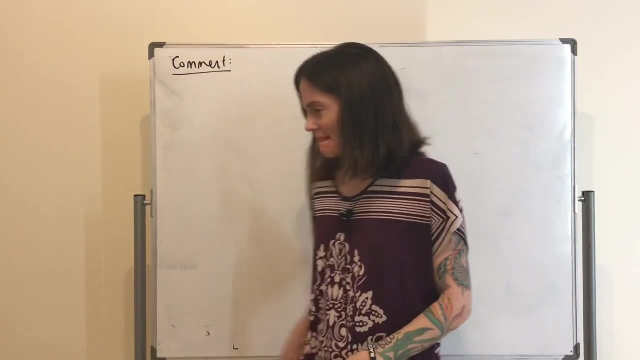 Well, and we're looking for something of one-dimensional, So we have found a basis for the orthogonal complement of v. There is a comment that I want to make here which we have observed in these two examples- And then I'm going to do an example that that seems really different than the ones we've just been doing. 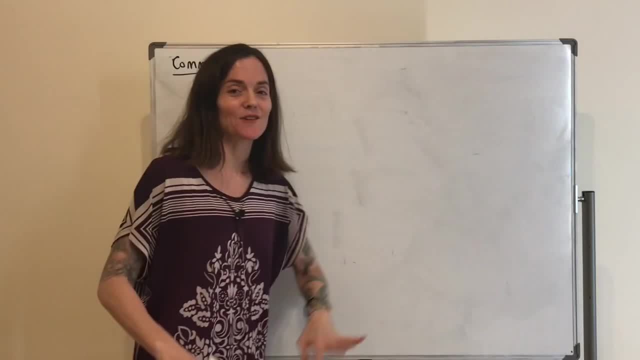 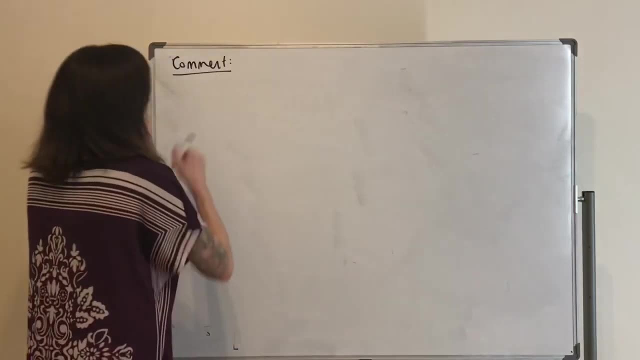 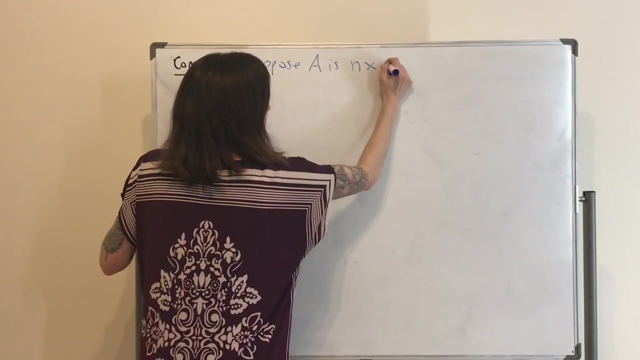 But it's very much like one of your homework And uses that Cauchy-Schwartz inequality that I started the lesson with today. Okay, so what's my comment? Well, suppose A is n by m matrix. Okay, I think that's. maybe I don't need to write that. 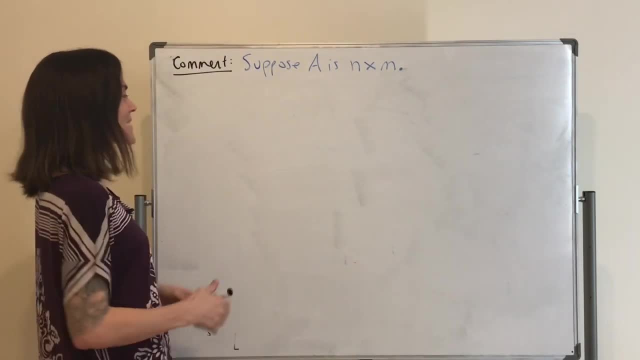 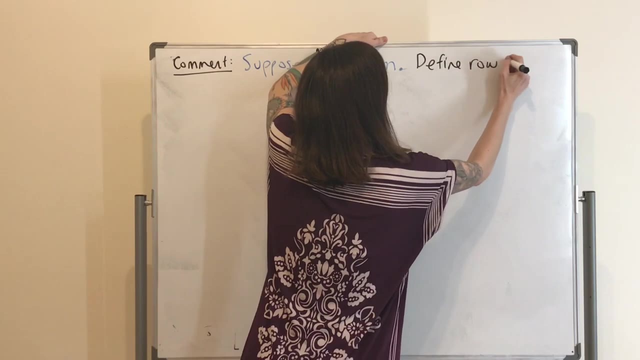 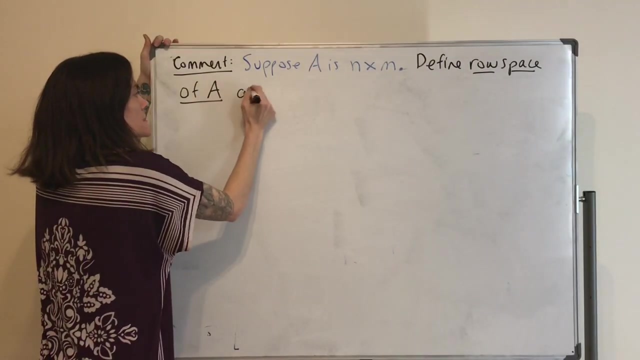 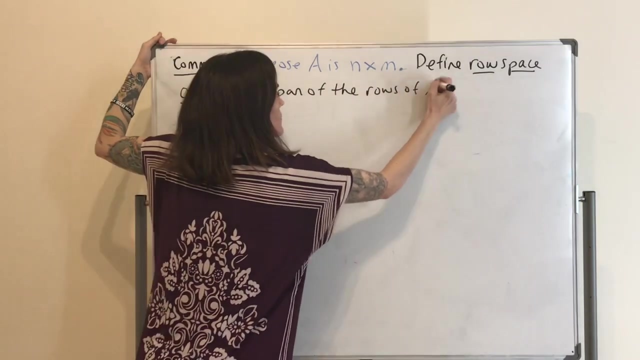 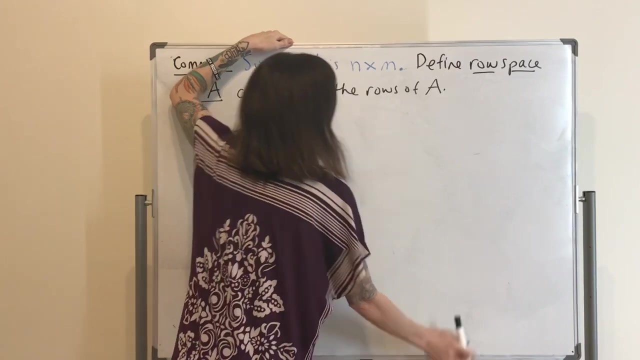 It's a matrix And it's n by m, N rows, m columns. We can define, I will say, the row space of A as the span of the rows of A, Or I should say the row vectors. Oh, I'll just say it this way: 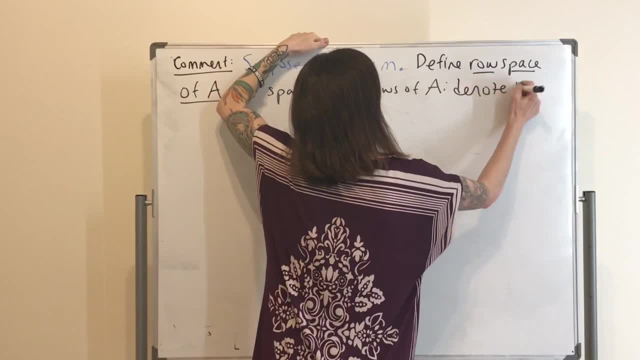 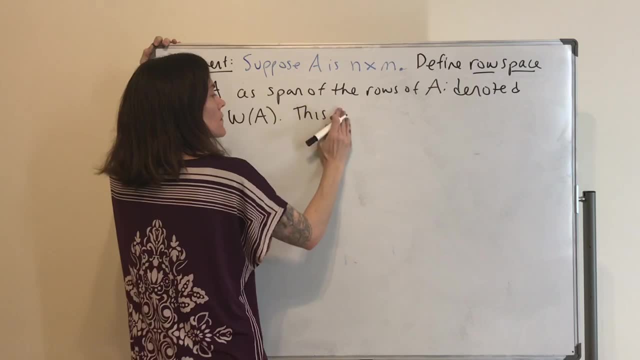 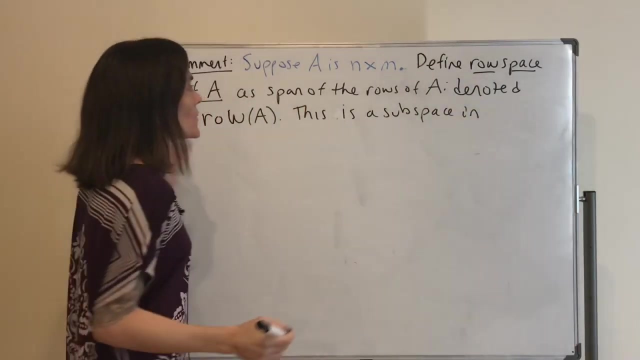 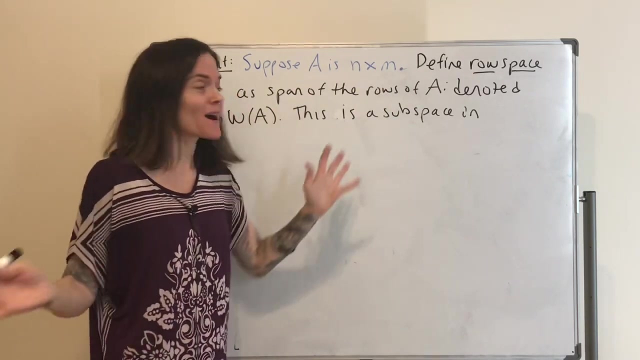 And this is denoted like this: Row Of A. This is a subspace In. Well, let's see, We have n rows. Each row lives in r? m Because we have m columns. So this is a subspace in r? m. 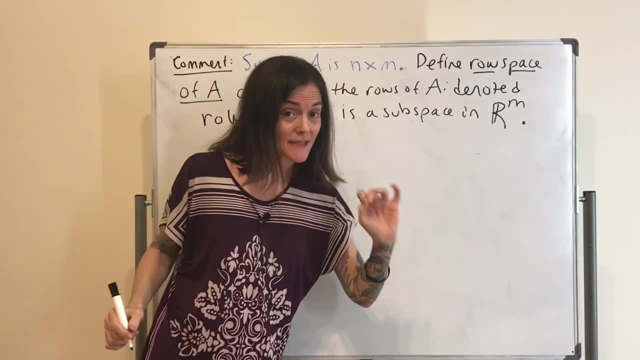 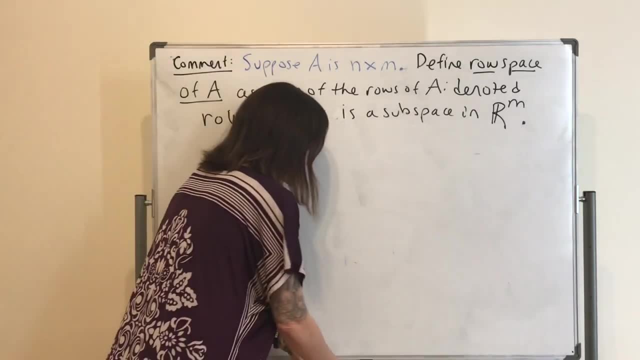 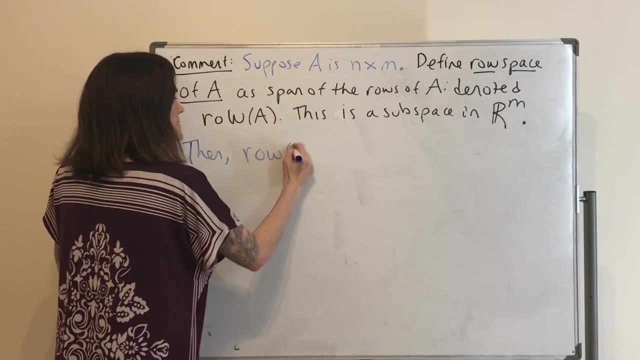 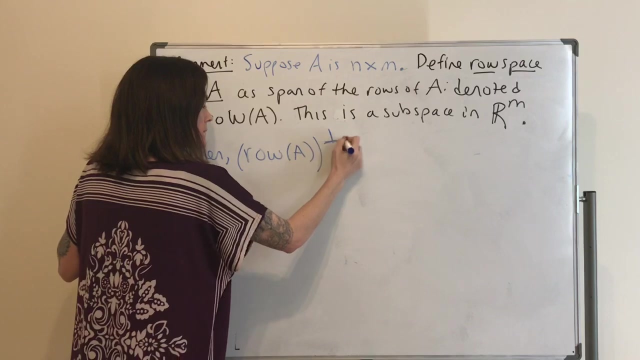 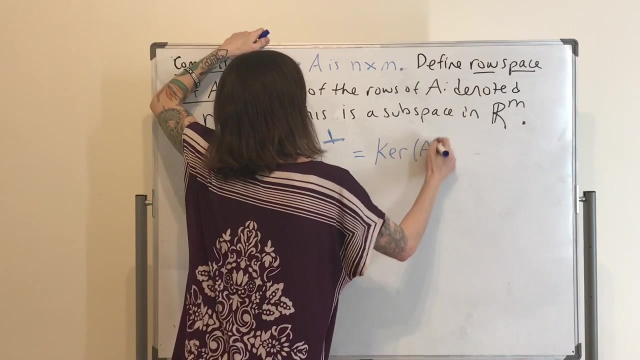 Okay, Now what we see in the last two examples Is much more More general. So what we saw in the last two examples is the following: Then, if you take this subspace And you take its orthogonal complement, This is the kernel of A. 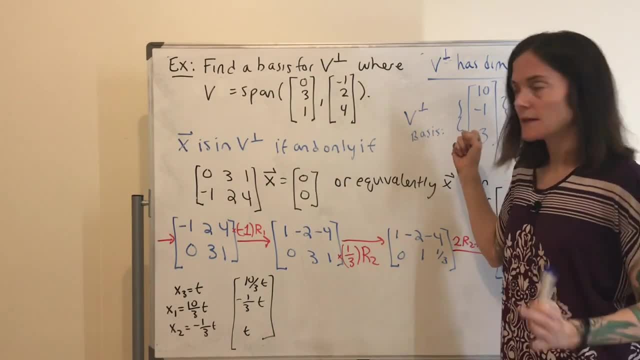 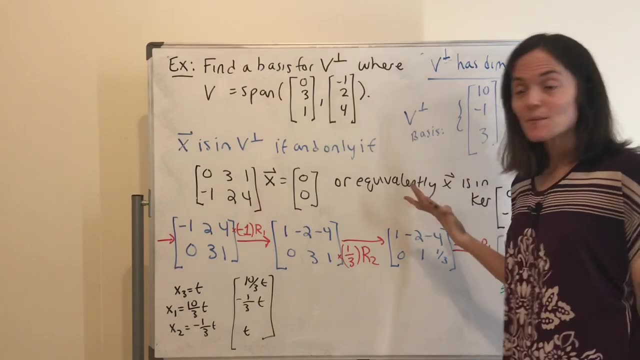 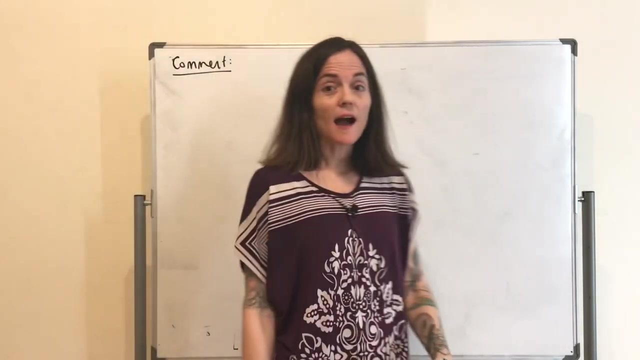 So this is one non-zero vector. linearly independent is perpendicular to both these. Well, and we're looking for something of one dimensional. So we have found a basis for the orthogonal complement of V. There is a comment that I want to make here. 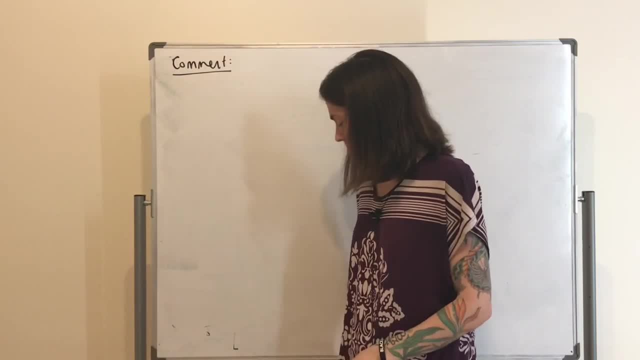 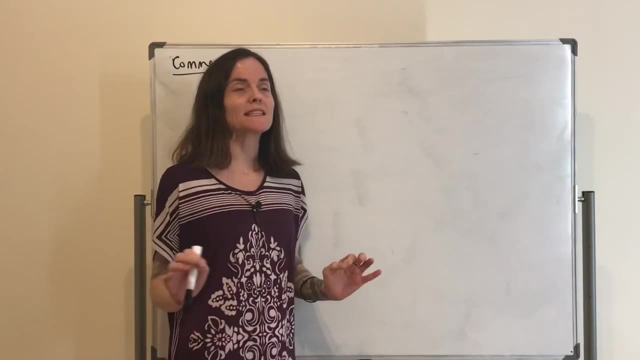 which we have observed in these two examples. And then I'm going to do an example that seems really different than the ones we've just been doing, But it's very much like one in your homework and uses that Cauchy-Schwarz inequality. 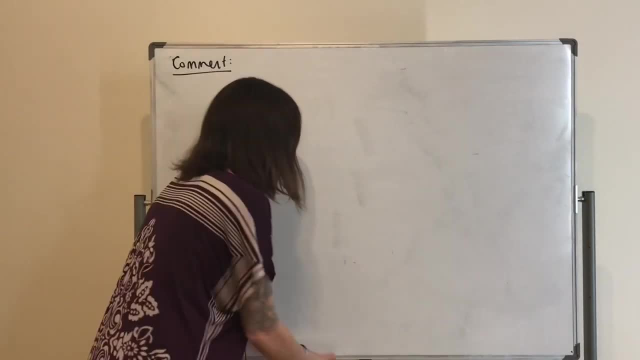 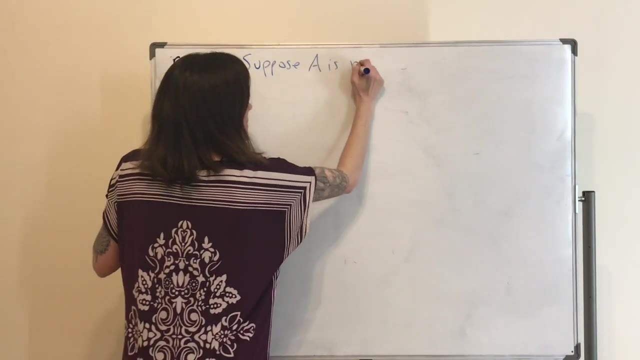 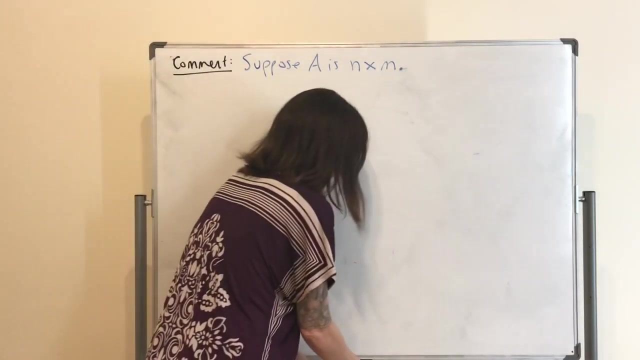 that I started the lesson with today. Okay, So what's my comment? Well, suppose A is N by M Matrix. Okay, I think that's. maybe I don't need to write that. It's a matrix and it's N by M. N, rows N, columns. 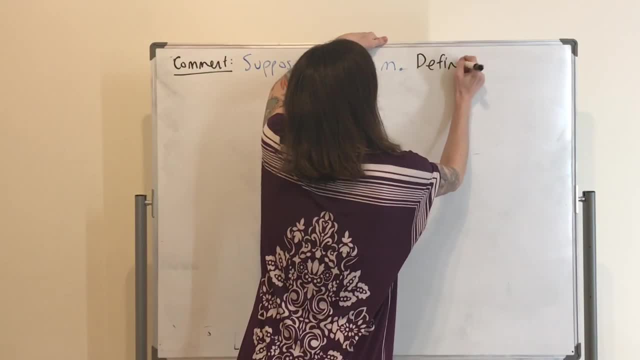 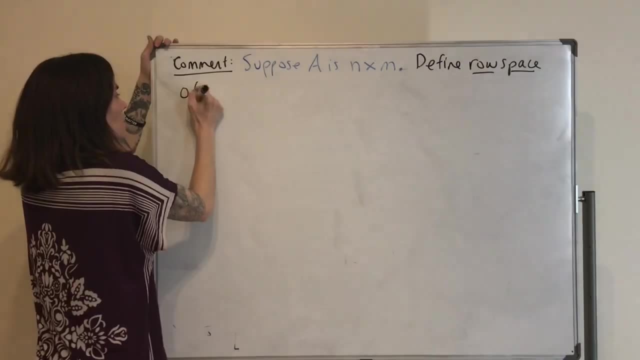 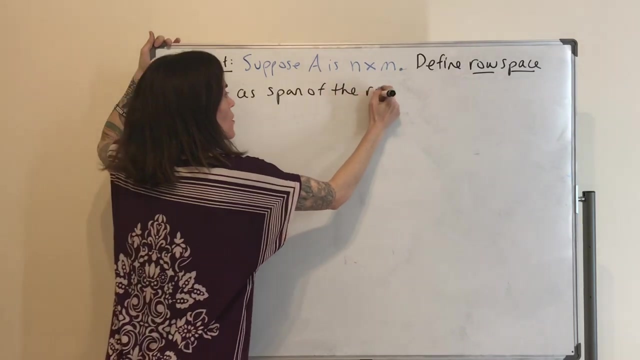 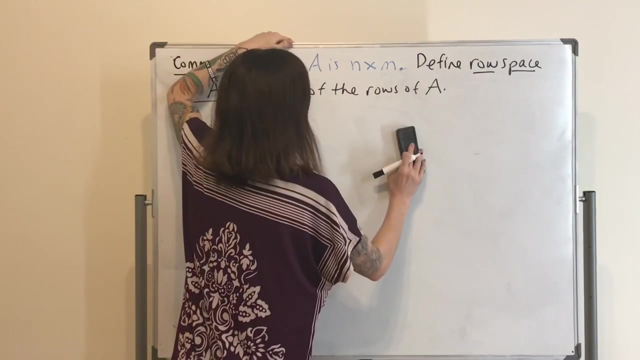 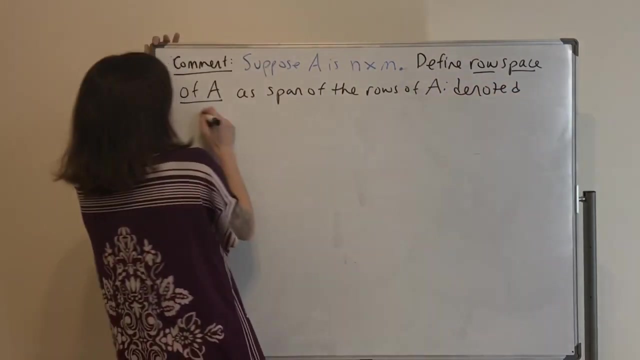 We can define, I will say, the row space of A as the span of the rows of A, Or I should say the row vectors. Oh, I'll just say it this way, And this is denoted like this: row of A. 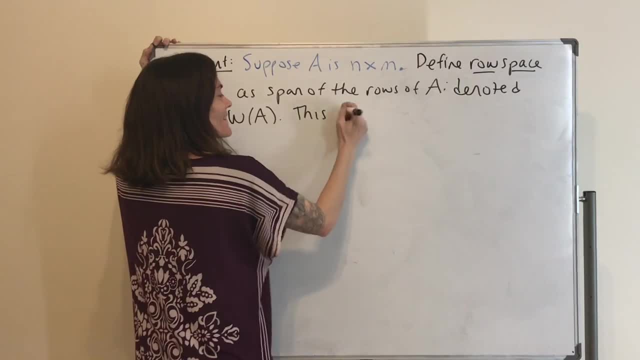 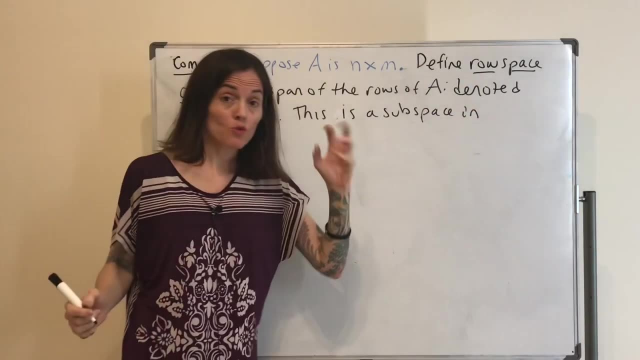 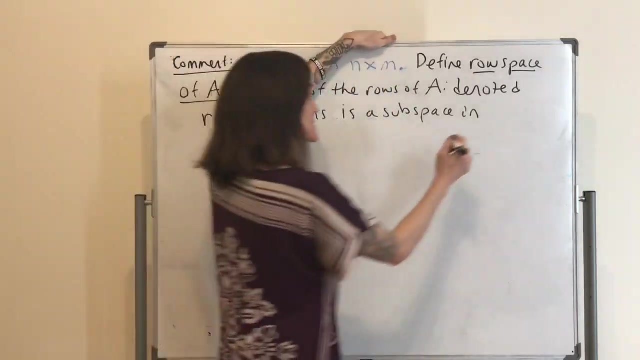 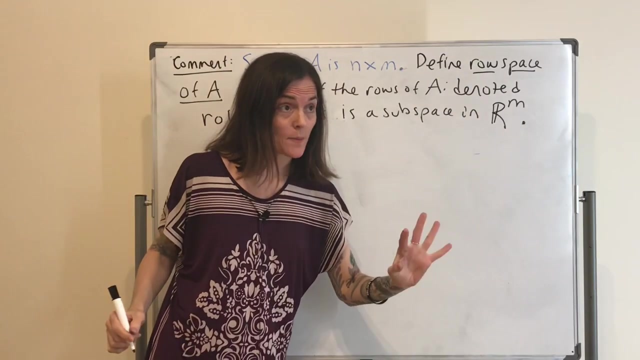 This is a subspace N. well, let's see, we have N rows. each row lives in our M because we have M columns. So this is a subspace in our M. Okay, Now, what we see in the last two examples is much more general. 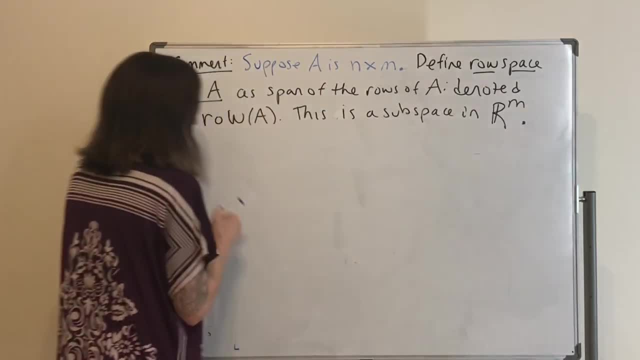 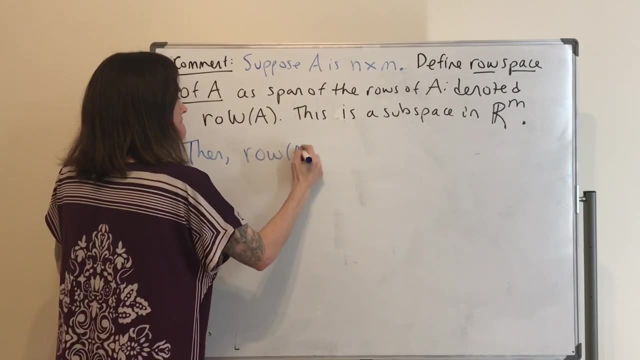 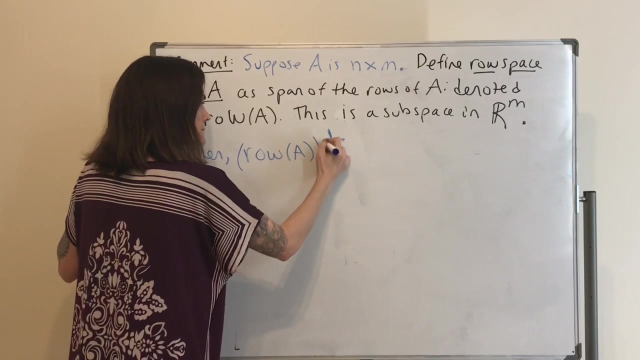 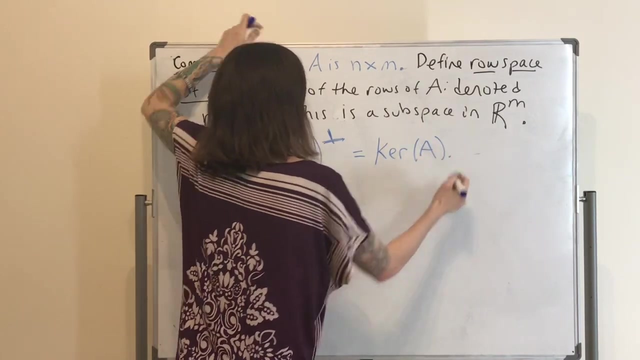 So what we saw in the last two examples is the following: Then, if you take this subspace and you take its orthogonal complement, this is the kernel of A. In fact, this is how we just had a vector, or two, depending on the example. 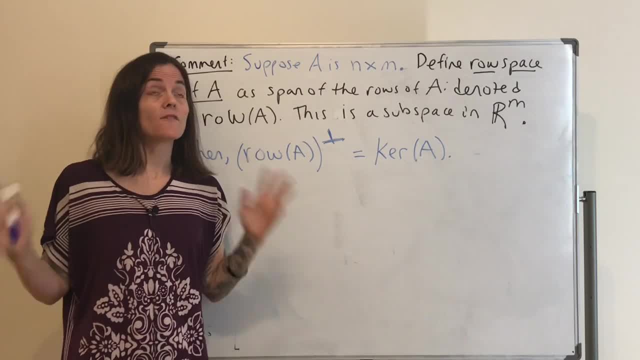 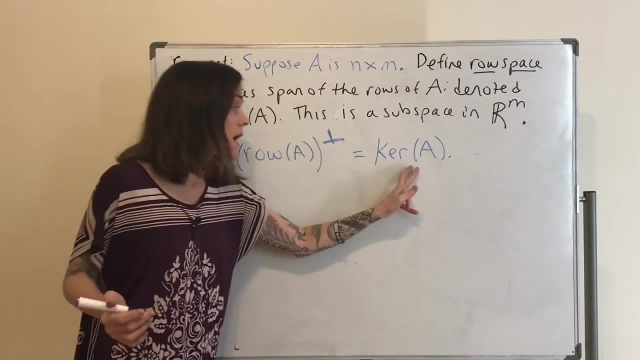 how we actually found a basis for its orthogonal complement. We just put it in the rows of a matrix and then we found the kernel of that matrix. But this is sort of an observation. I wanted to make One more example that, like I said, 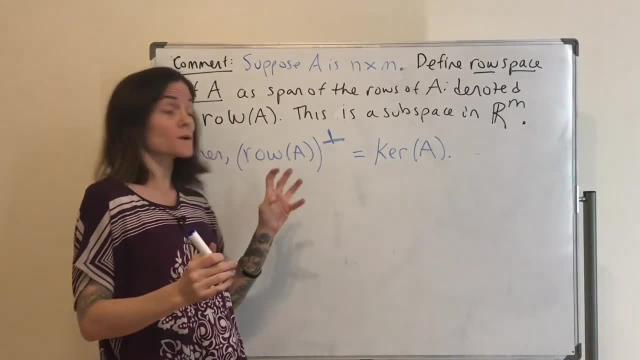 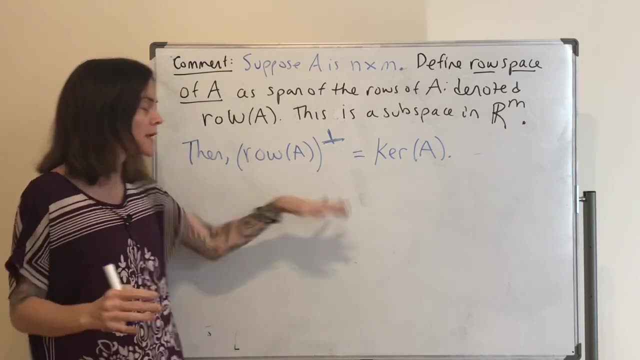 In fact, this is how we just had a vector or two, Depending on the example, How we actually found a basis for its orthogonal complement. We just put it in the rows of a matrix And then we found the kernel of that matrix. 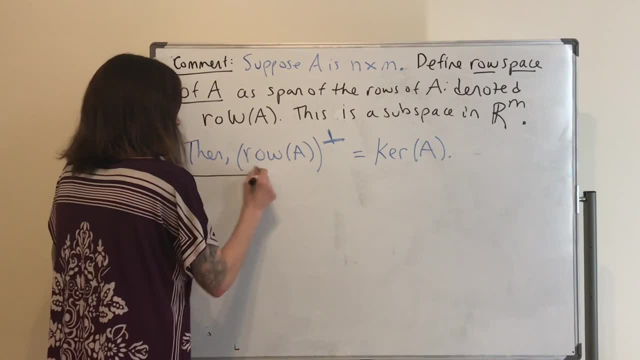 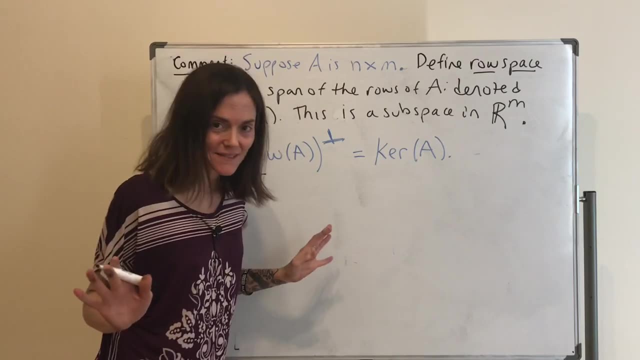 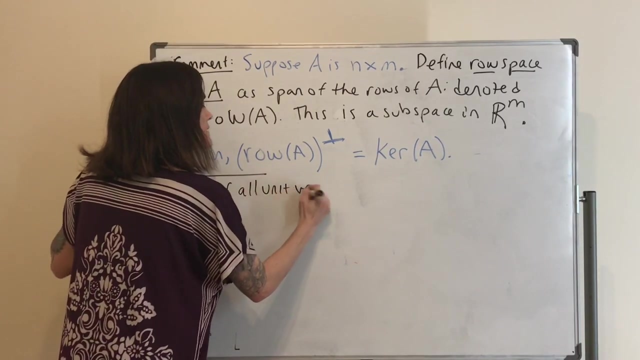 But this is sort of an observation. I wanted to make One more example that, Like I said, it seems different than the ones we have done today, But it's similar to one in your homework Of all unit vectors, And let's look at this one. 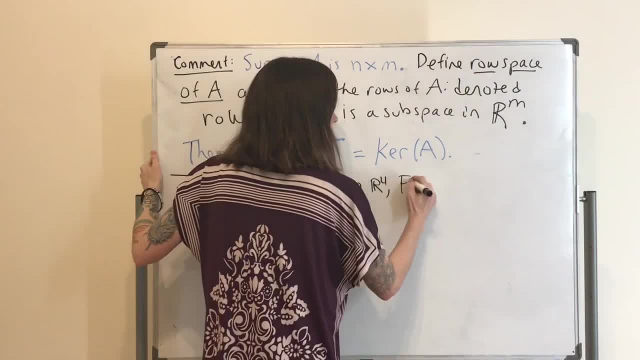 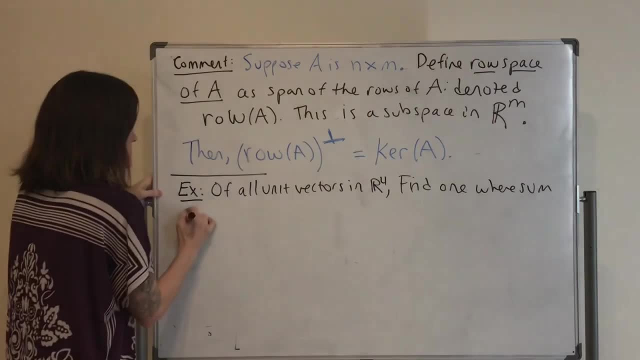 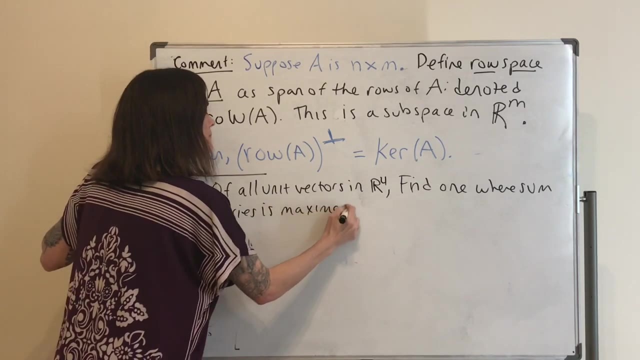 One, Two, Three, Four, Seven Eight, 10., 11., 12., 13., 13., 14., 16., 15., 17., 16., 19., 20. 22.. 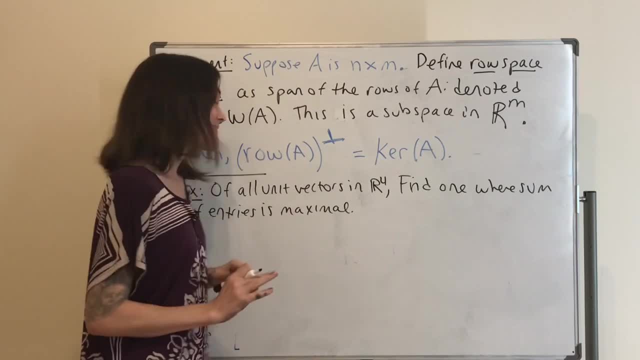 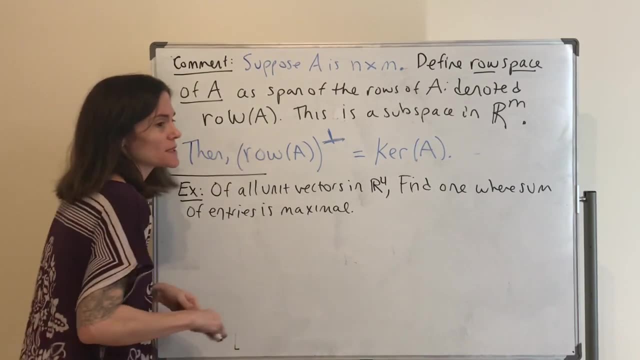 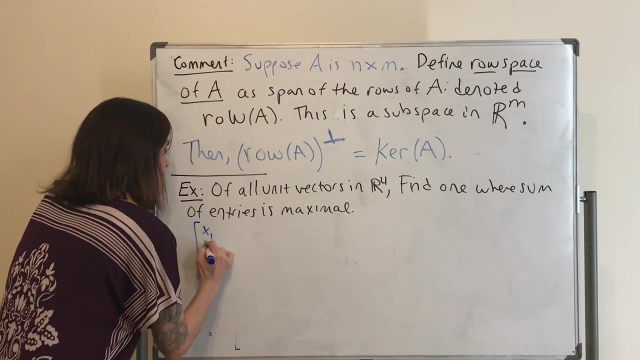 24. 25., 28., 24., 25., 26., 24., 36., 27., 29. Cauchy-Schwartz, and we will be able to figure this out. So let's suppose we have x1,, x2, x3, x4.. 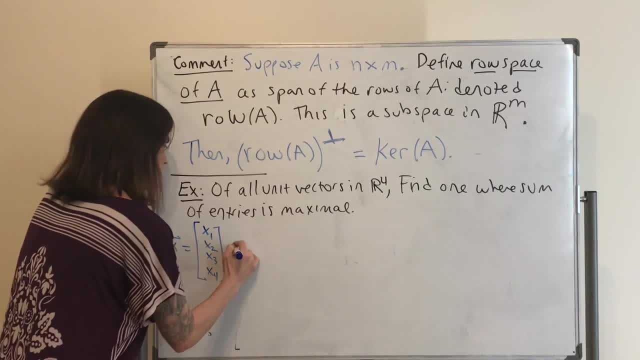 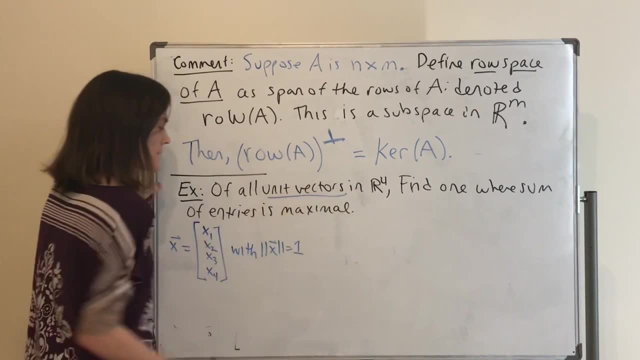 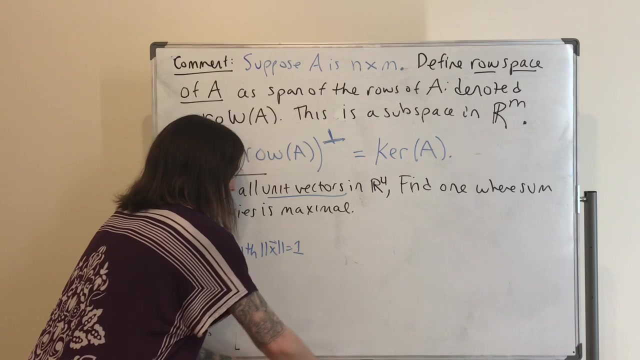 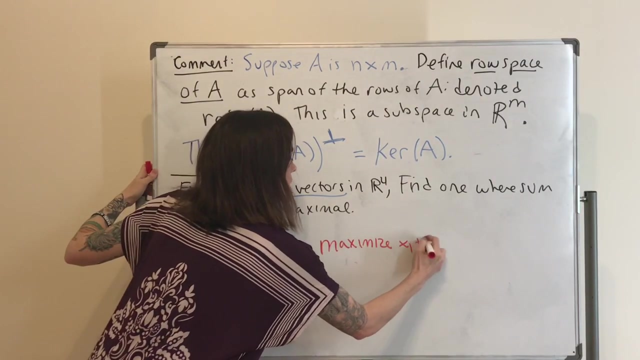 Say: this is here. Maybe I should have called it u, but I'll just make it unit by here, because we're really only looking at unit vectors here. What does this say? We want the sum of the entries to be maximal. We want to maximize this: x1 plus x2 plus x3 plus x4.. We want to find the. 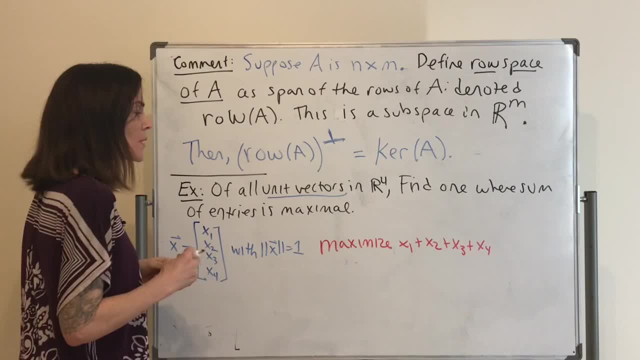 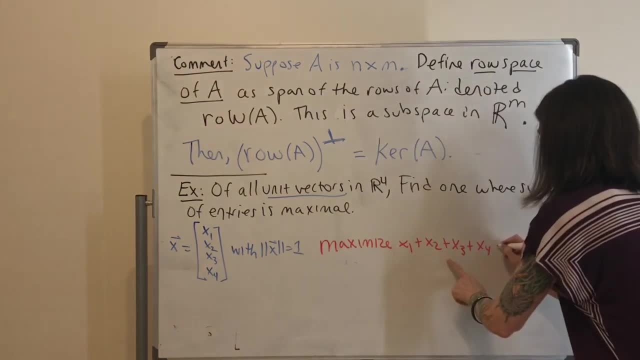 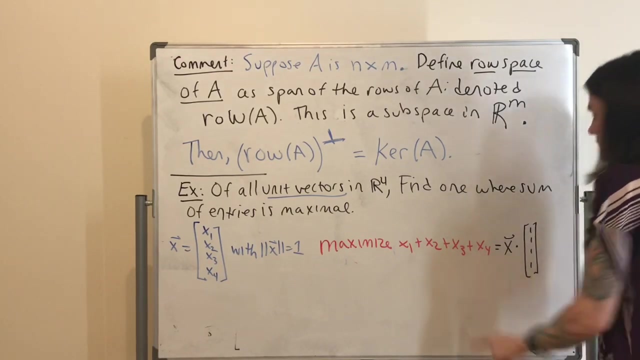 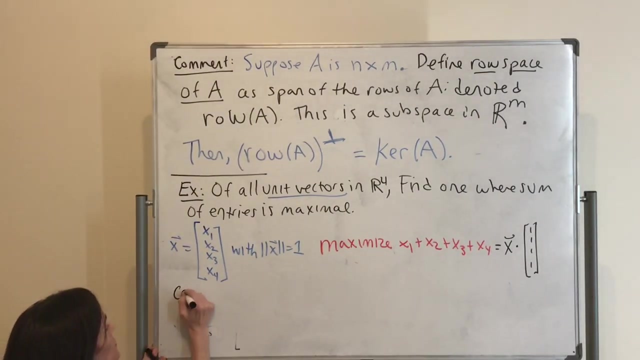 vectors such that this is maximal. But if we notice, here this is a dot product, So this is just x dotted with here 1, 1, 1, 1.. Okay, And then what else can we know, We know or can use. 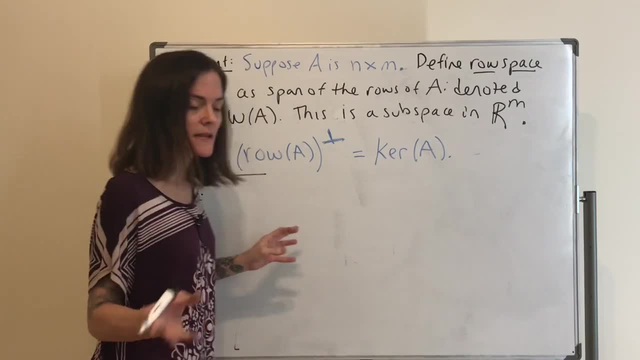 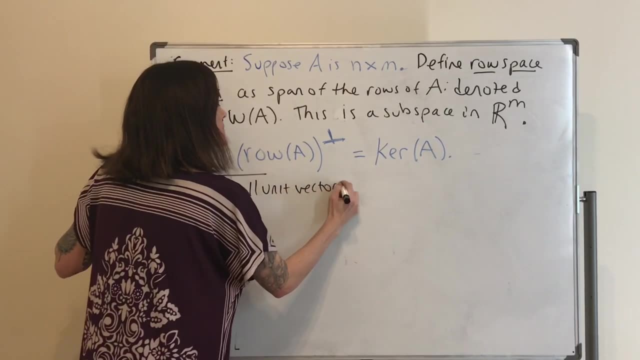 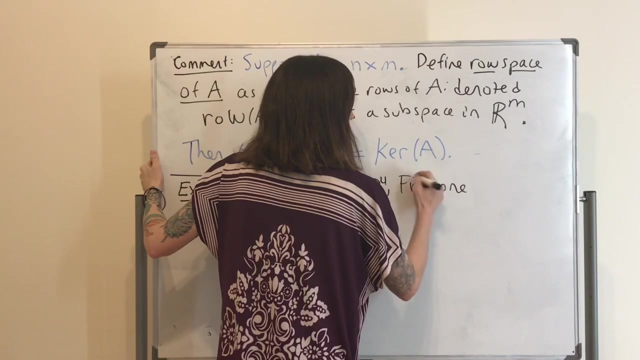 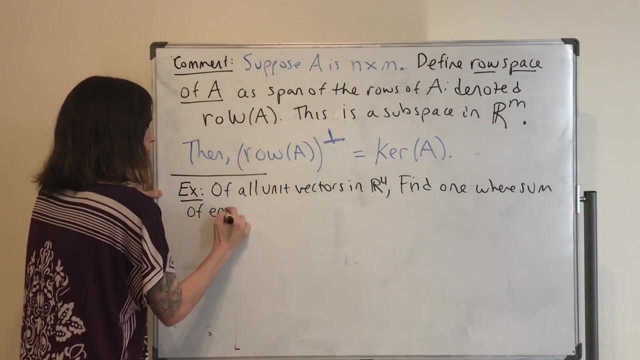 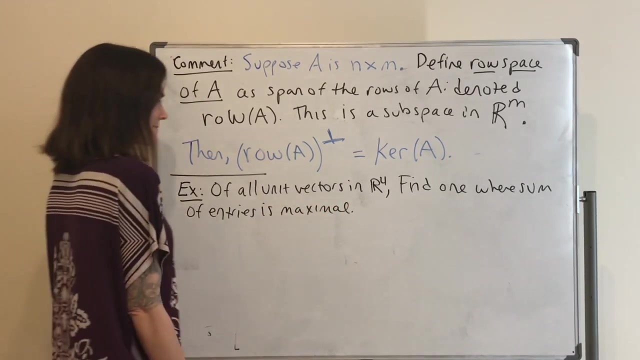 it seems different than the ones we have done today, but it's similar to one in your homework. Of all unit vectors in R4, find one where the sum of the entries is maximal. Well, we have to think, because it seems strange. 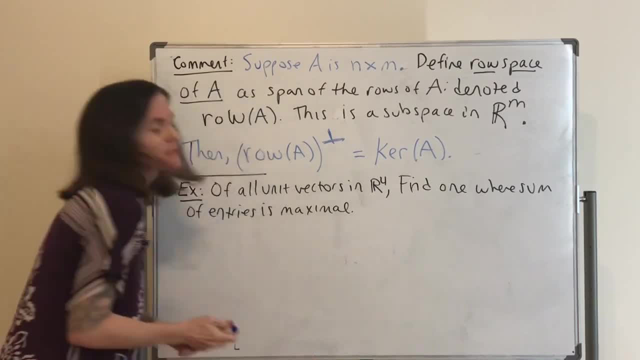 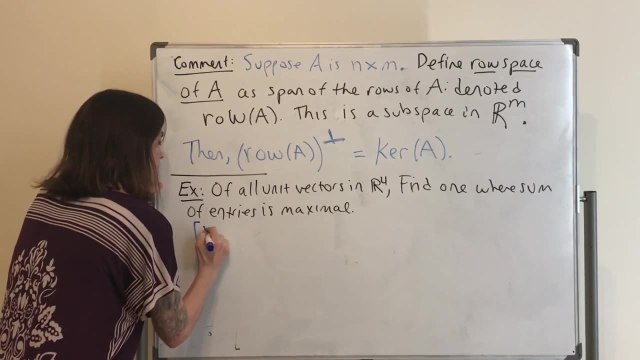 So let's just write down some things And, as I mentioned, this will use Cauchy-Schwarz and we will be able to figure this out. So let's suppose we have X1,, X2,, X3, X4.. 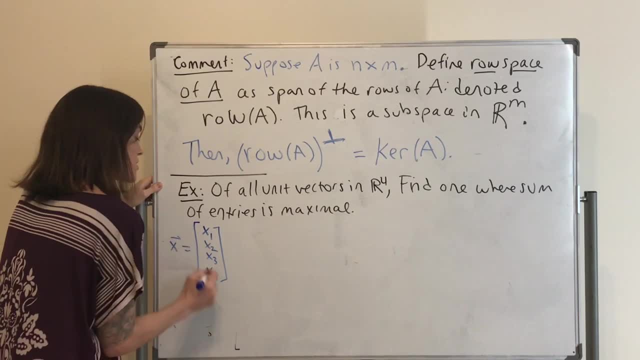 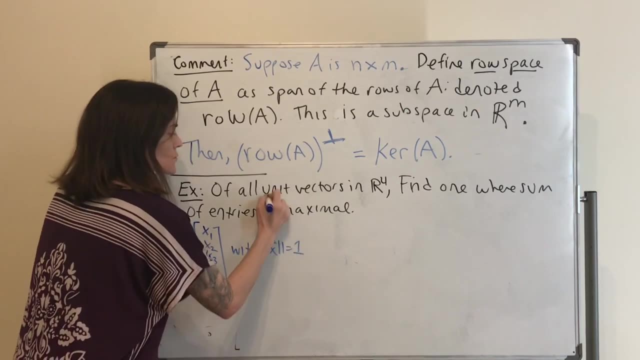 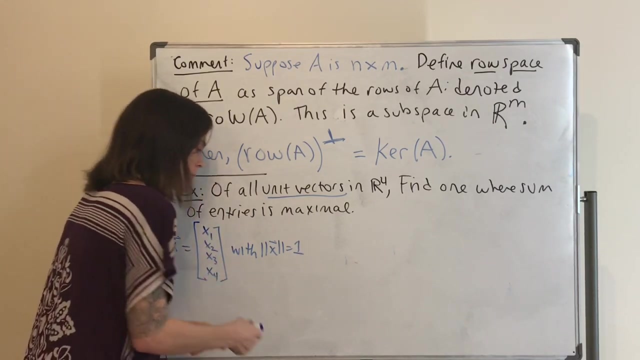 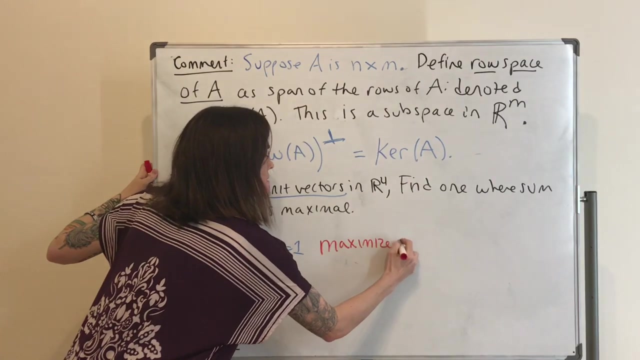 Say: this is here. Maybe I should have called it U, but I'll just make it unit by here, Because we're really only looking at unit vectors here. What does this say? We want the sum of the entries to be maximal. We want to maximize this: X1 plus X2 plus X3 plus X4. 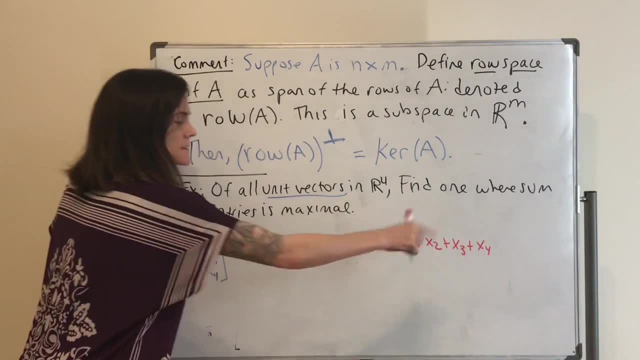 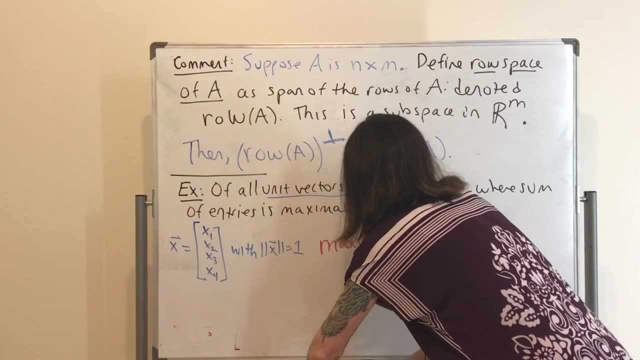 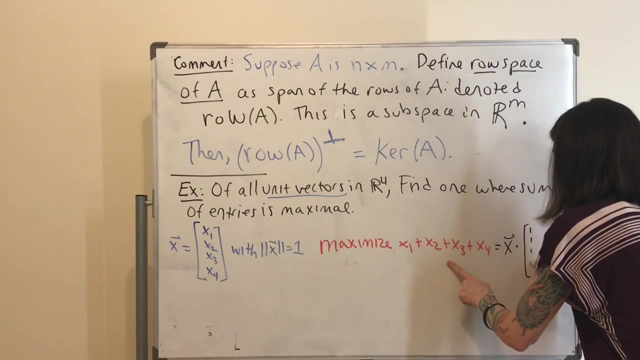 And we want to find the vectors such that this is maximal. But if we notice here, this is a dot problem, This is a product. So this is just X dotted with here 1, 1, 1, 1.. 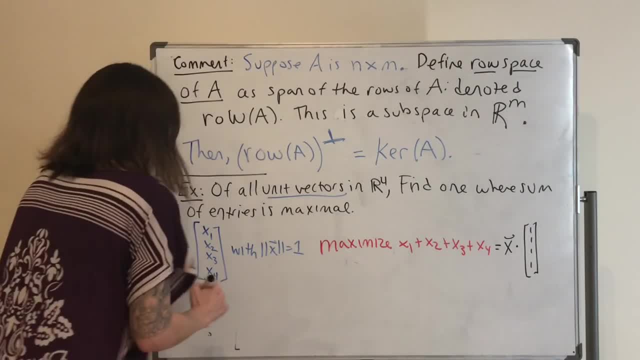 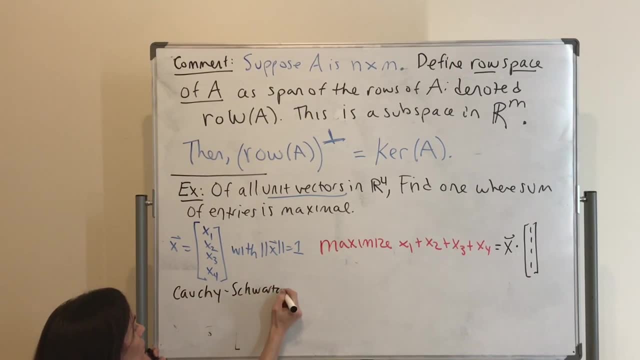 Okay, And then what else can we know? We know, or can use Cauchy-Schwarz, which says: any time you have a VW, an absolute value, it's going to be less than or equal to length of V times. length of W. 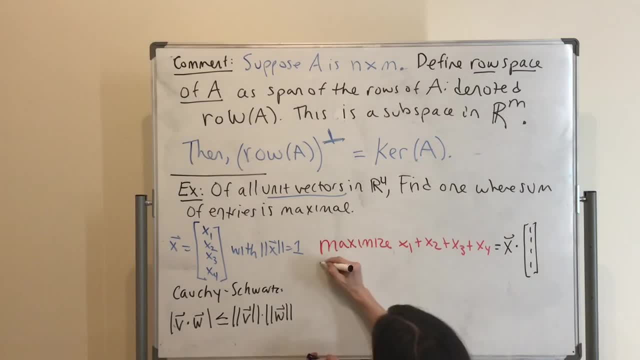 Right, Mention this at the beginning. This, which is X dot, an absolute value, is going to be less than, or equal to well, the length of X times what's the length of this Square root of 4, which is 2.. 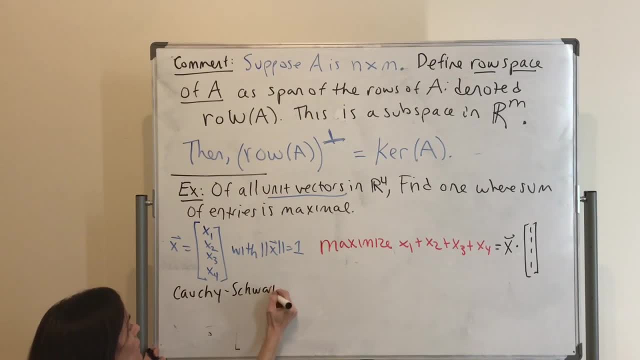 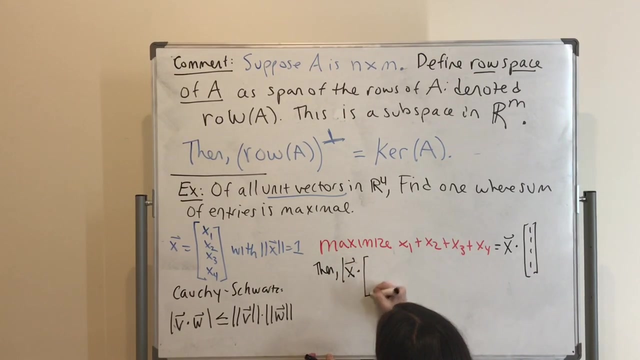 Cauchy-Schwartz, which says: anytime you have a vw an absolute value, it's less than or equal to length of v times length of w. Right Mentioned this at the beginning. This, which is x dot, an absolute value, is going: 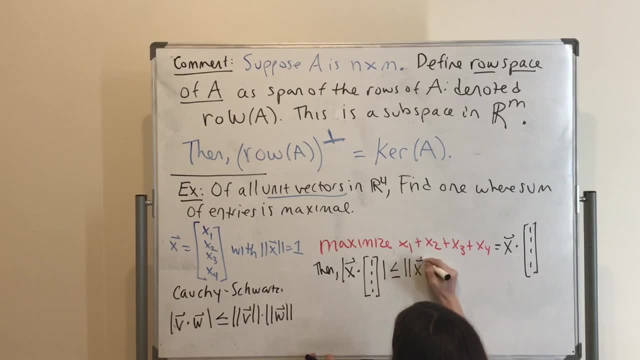 to be less than, or equal to well, the length of x times. what's the length of this square root of 4, which is 2?? Well, maybe I'll write it in two steps: 1 plus 1 plus 1 plus 1.. And this is the length of x is 1 and this is 2.. So the biggest 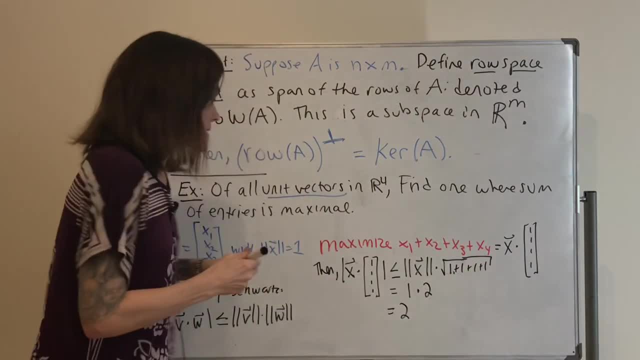 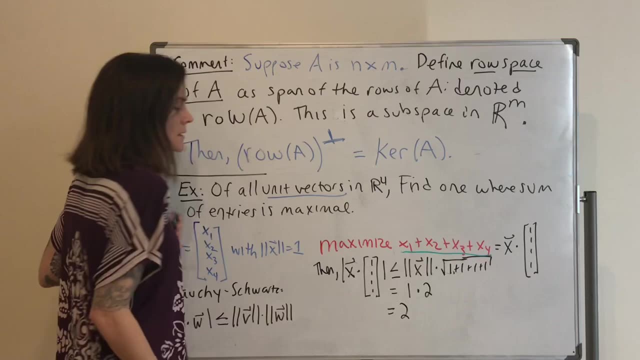 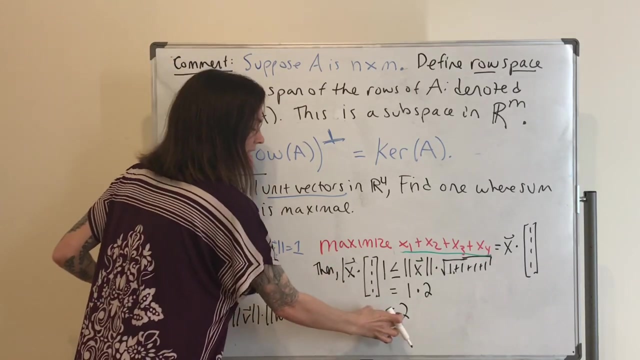 an absolute value that this can be. the biggest this can be here is 2. And the smallest it can be is minus 2.. Right, Because if absolute value of x is less than this, it means that this number itself sits between minus 2 and minus 5.. Okay, And then? what else can we know? We want to maximize this: x1 plus x2 plus x3 plus x4.. So this is 1 and this is minus 2.. Okay, Mentioned this at the beginning. This is x dot, an absolute value of x plus x3 plus x4.. 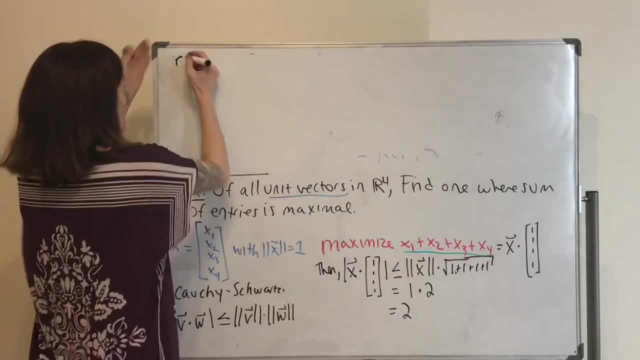 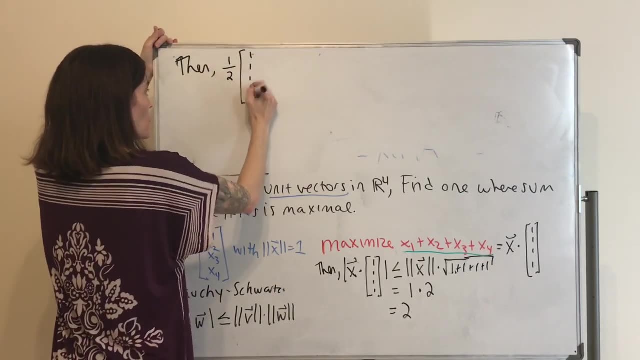 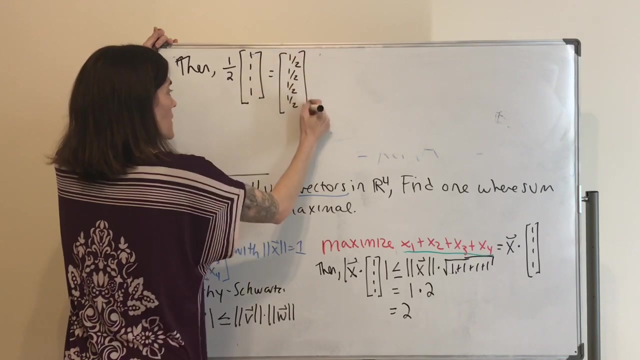 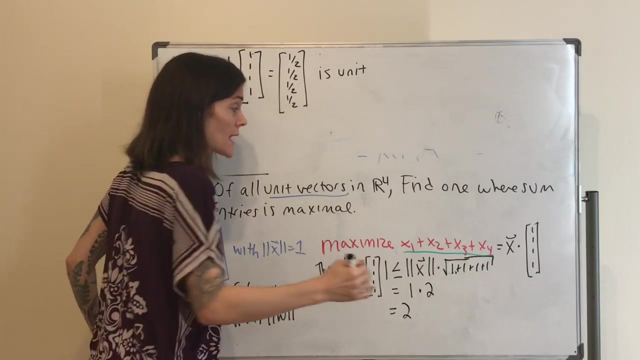 is 2 and 2.. So the biggest this sum can be is 2.. If we take a half, 1, 1,, 1, 1,, this vector is unit. Well, you can either calculate the length or just realize we took a vector. 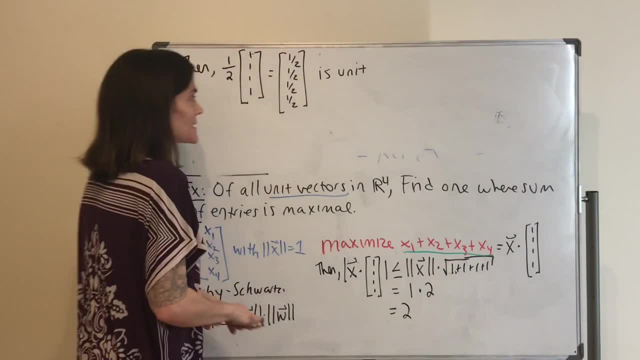 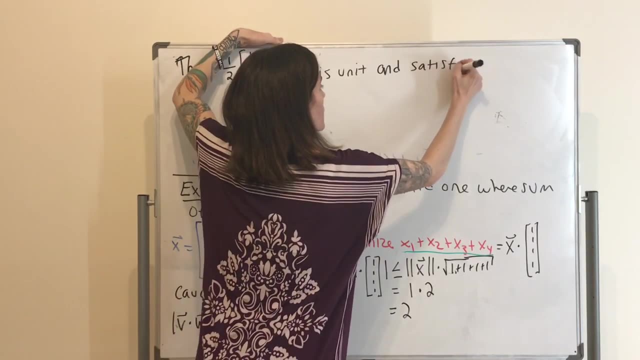 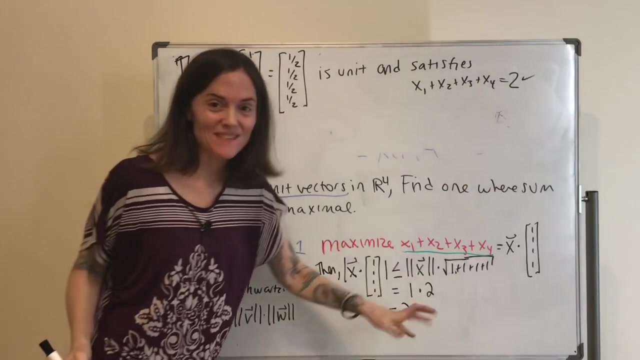 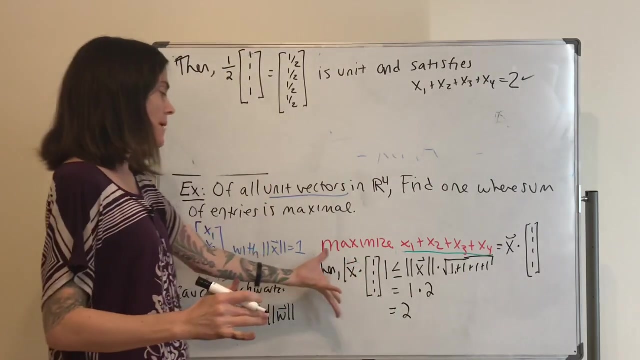 non-zero divided by its length, of course, it's unit and satisfies 2,, which is the maximal Satisfies. if you add up all the entries, you get 2,, which is the biggest this can possibly be by this Cauchy-Schwarz. So this would be the answer. To the question.